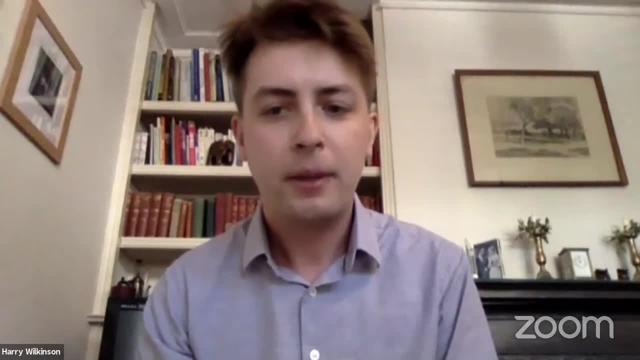 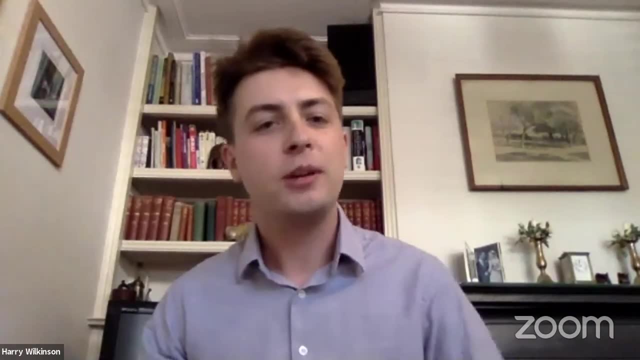 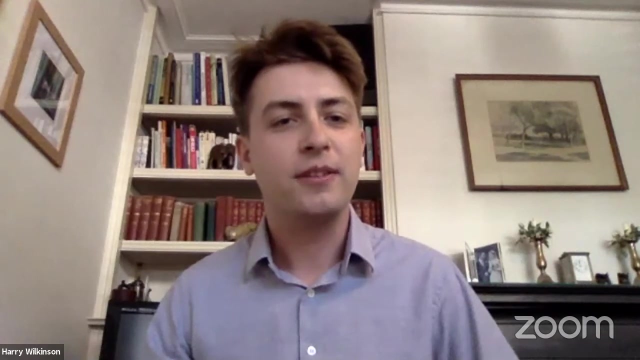 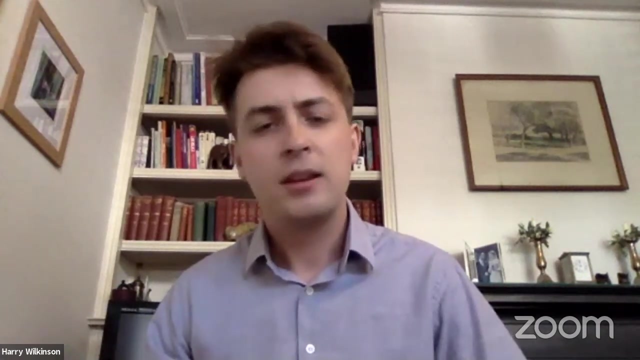 pardon me, and then they're indeed playing a vitally important role in the modern world. Indeed, we could not plan how an aeroplane worked, or indeed test whether flood defences would be able to cope in the most severe and rare storms. So what models are doing in so many practical examples is helping. 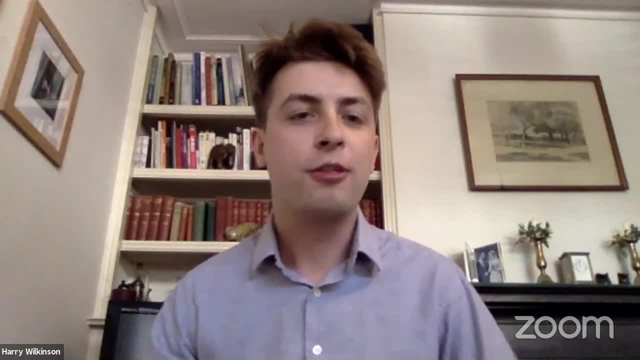 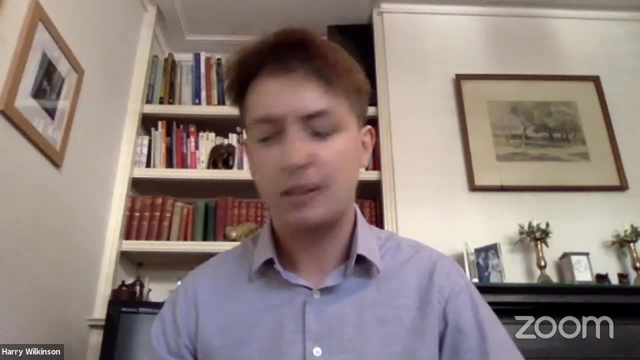 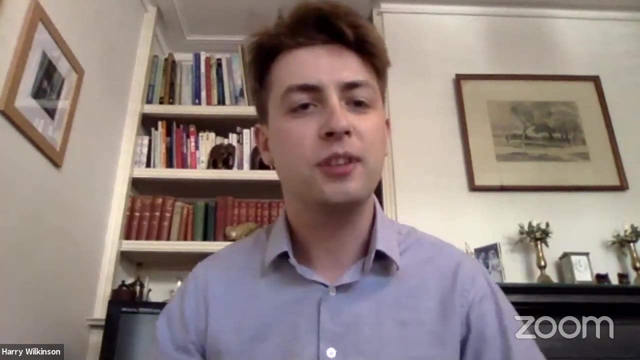 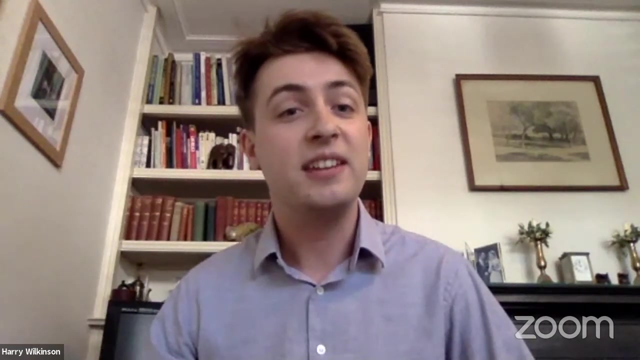 us translate the findings of theoretical physics, of mathematics, into practical applications, and there are indeed so many positive uses for those. However, the story about modelling isn't all so positive, and indeed it's a very important topic, So let's get started. Indeed, when it starts getting political, that's when we see some of the dangers getting involved. 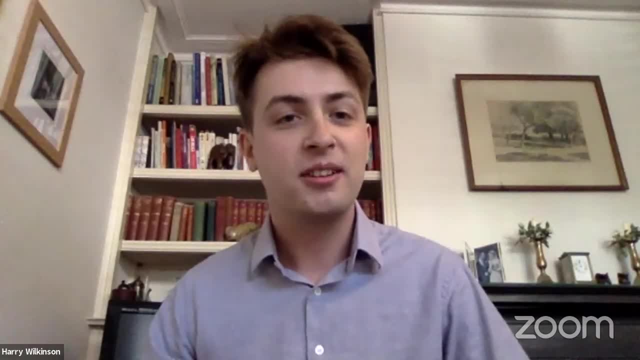 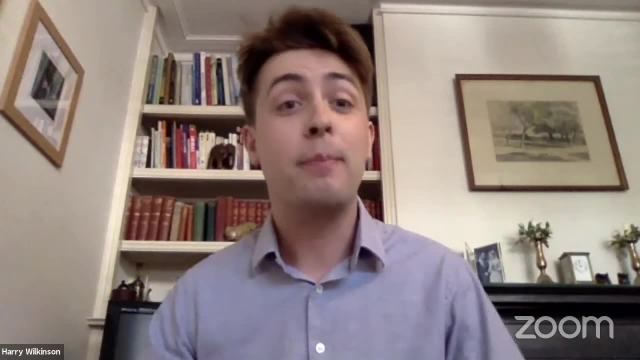 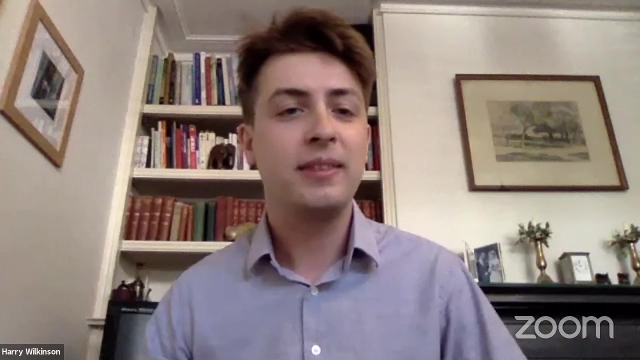 and just if you have some good modelling results, it doesn't mean necessarily that you're going to have some good policies from that. And if you have some bad modelling results, then you'll probably have some even worse policies at the end of that. So we've got to be thinking very carefully about. 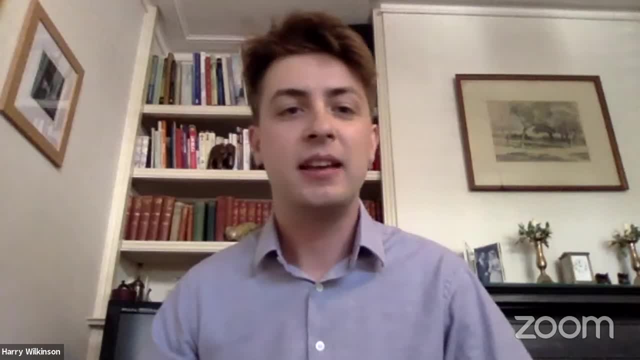 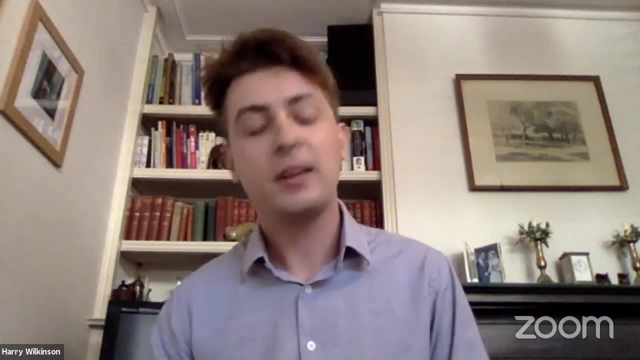 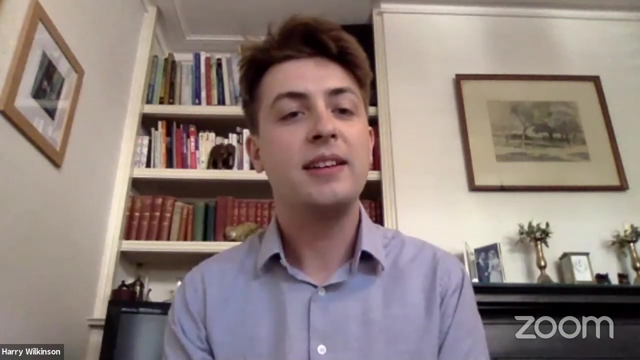 models and how we use them, How they're formulated and what we've learned from them. And our first guest today to talk about that is Professor Chris Essex. Now he's a Professor and Associate Chair in the Department of Applied Mathematics at the University of Western Ontario in Canada, And he's the perfect. 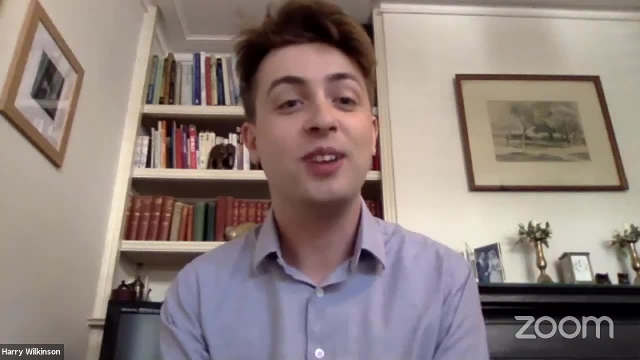 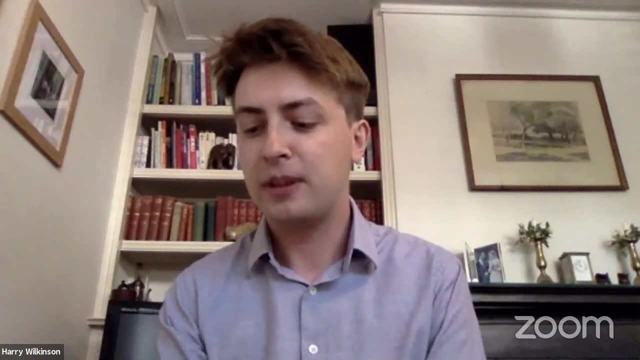 person to talk about this today, because he has indeed taught an undergraduate course on the subject of modelling And he's going to bring that up, So let's get started. Well, thank you very much, Chris. He's got an excellent approach by the всё South of the UK and we've heard from many of you. 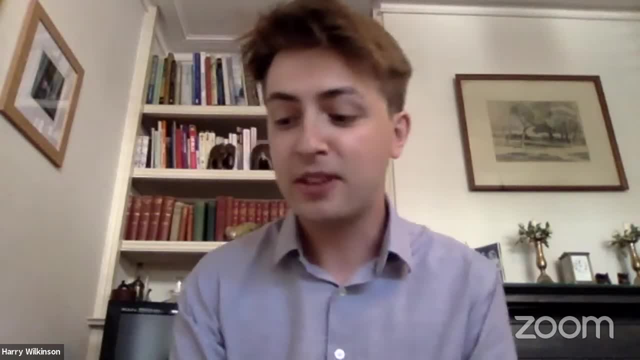 that you've had key insights on that today and he's very much something that you really appreciate. Yes, thank you. Thank you, Professor. Thank you, Professor. I think it's just fantastic that you've shared a little bit of that insight to us today. 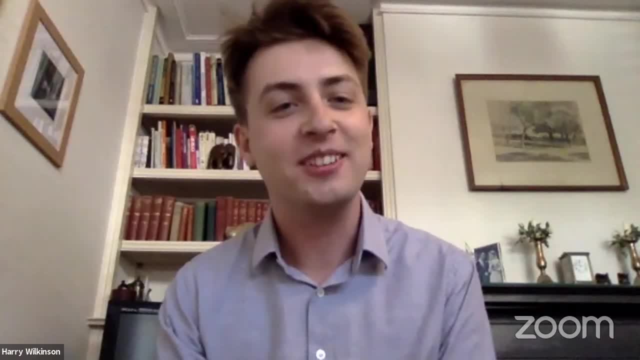 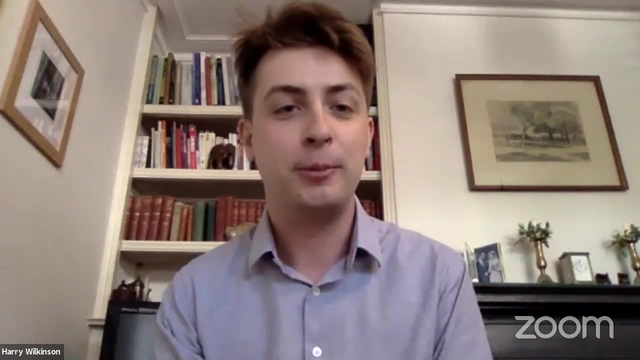 And he indeed co-discovered the entropy production paradox. In plain terms, he's a genius, And we're also very fortunate to have him as the Chairman of our Academic Advisory Council here at the GWPF. So without further ado, Dr Chris Essex, I'll pass it over to you. 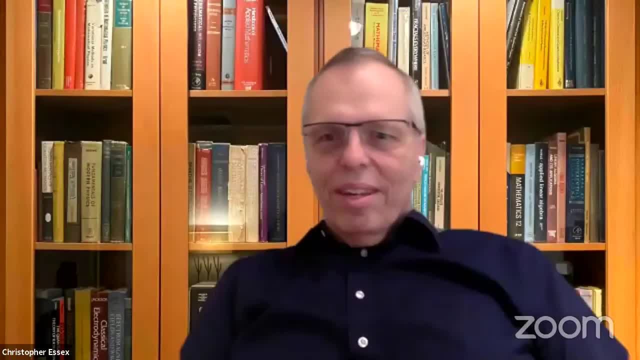 Thank you, Professor. It's a pleasure to be here. Thank you very much, Chris. Okay, so thanks, Harry. This is my first of these webinar settings, and so I'm getting used to the world of Zoom. Yeah, so we're talking about modeling today. There's a lot. 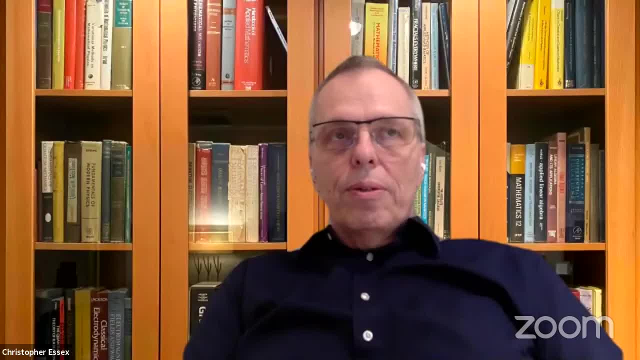 to say about the subject because modeling is used. the term model and modeling is used in many different ways And in recent times the term has come forward because of its interaction with politics And unfortunately politics does things to other subjects that one would 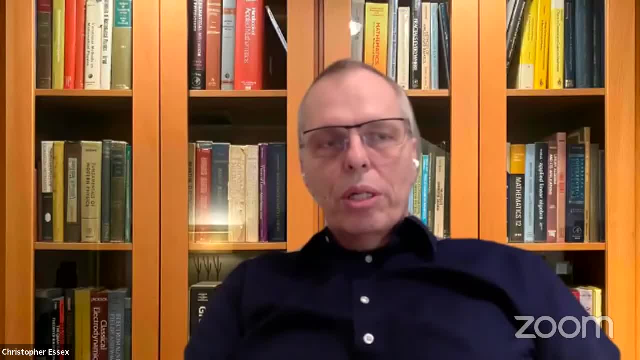 rather not do. But in any event, what I'm going to do is I'm going to talk a little bit about it from a mathematical and a scientific point of view, And then I'll work my way into talking about its connection with policy and what's special about it. 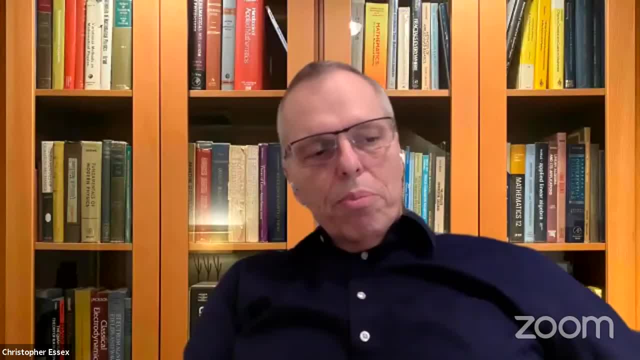 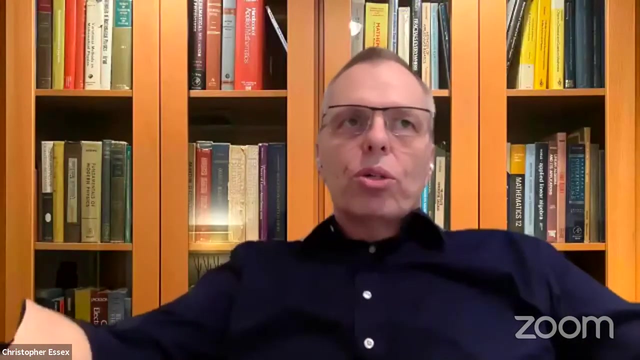 So the word modeling is used in many cases. So it's used in many in a range of scientific contexts. So, for example, we have in theoretical physics, we have something called the standard model. It's quantum field theory, And that is its intent: is to actually try to capture. 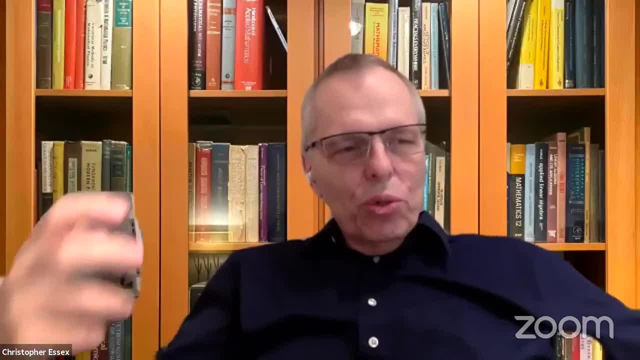 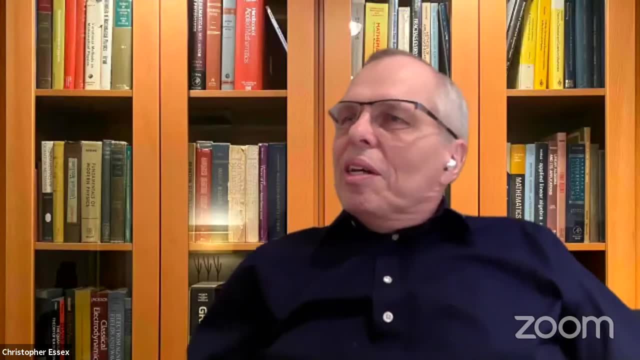 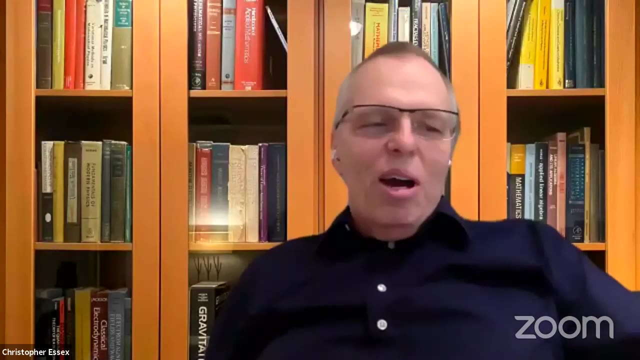 the laws of nature, And so there's a kind of different or unique agenda to that. But the term model is used in that respect And undoubtedly, even though one of my department colleagues used to say I have a lot of faith in the standard model. chances are it's probably. 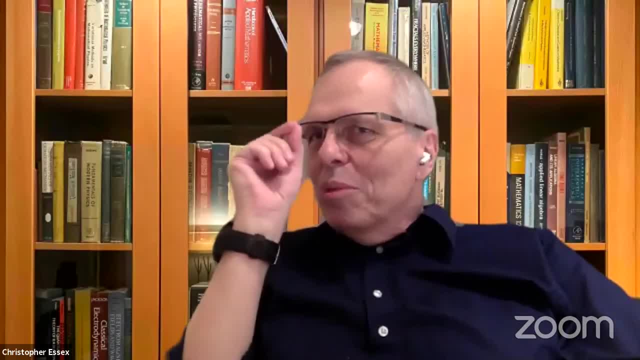 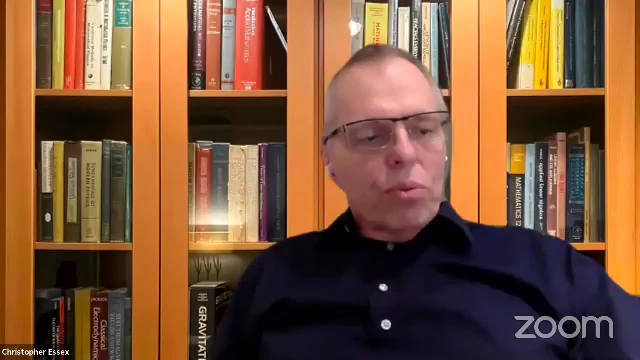 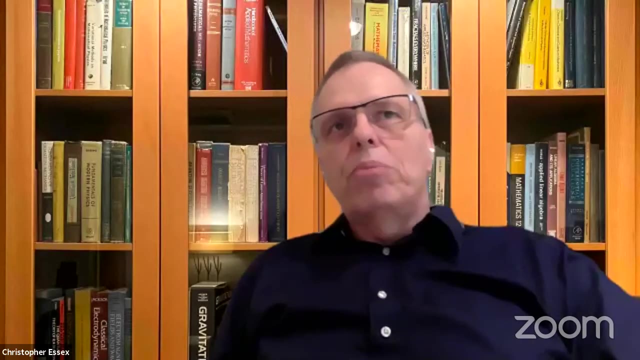 wrong. It's wrong to a very minuscule degree. It's a remarkable accomplishment in many ways. Then there are other models which scientists use to try to understand the world, And in those kinds of models there's no attempt to try to generate a comprehensive theory. 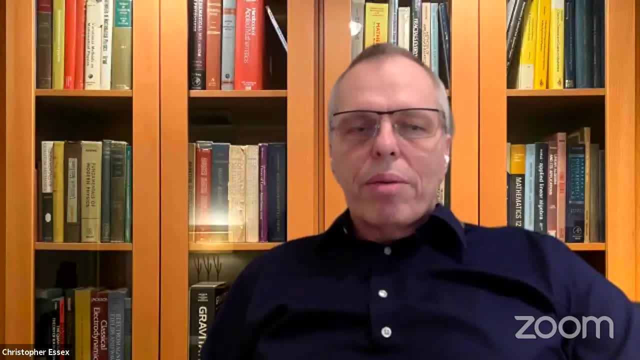 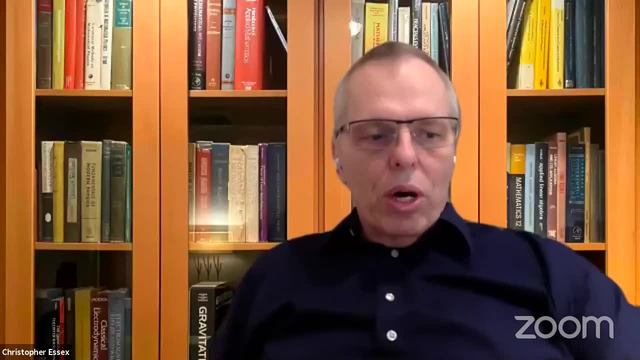 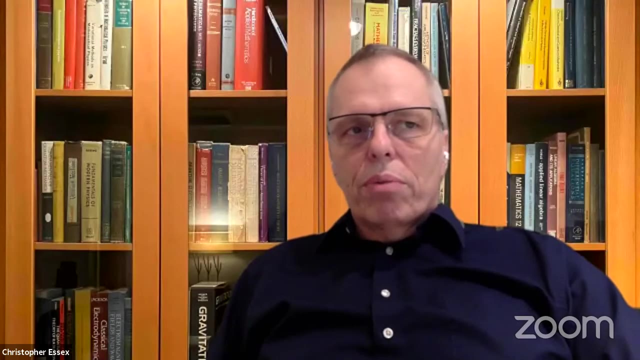 for all things. What they do is they create mathematical cartoons, And these cartoons are designed to help people develop their intuition about what's going on, And so a good example of something like that is the population models. They're the simplest version, being that the rate of population growth is proportional to the population size, And so 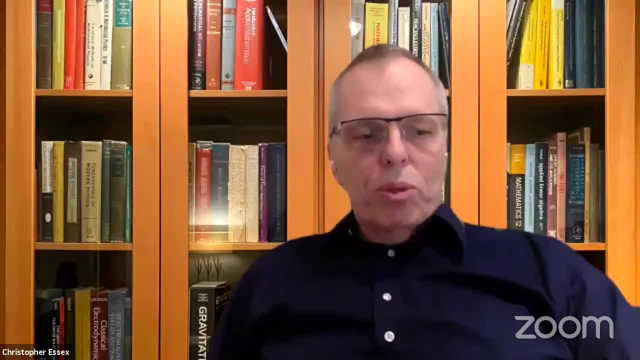 they're proportional to the population. That's the simplest possible model And that leads to exponential growth. So people have taken that very simplistic model and they've gotten very concerned about it And of course people are worried about the population of the earth. 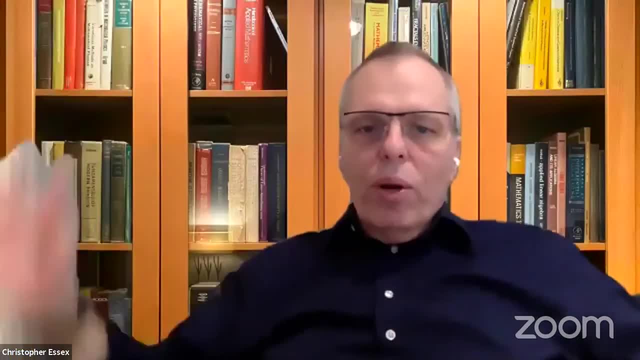 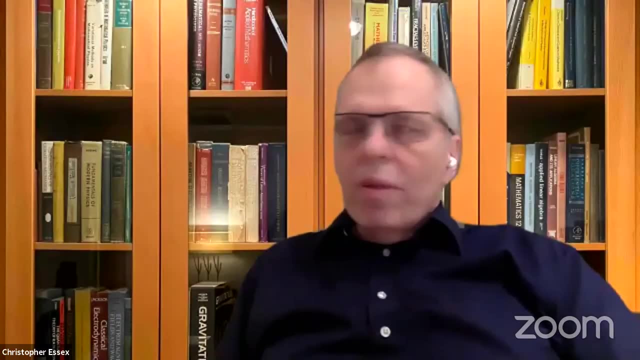 exploding because an exponential is a rapidly growing function, starts off really small and then boom off, it goes right. So there was a lot of anxiety about it. There was even a book on it, I think, called The Population Bomb. because the exponential is like a bomb: It takes off. 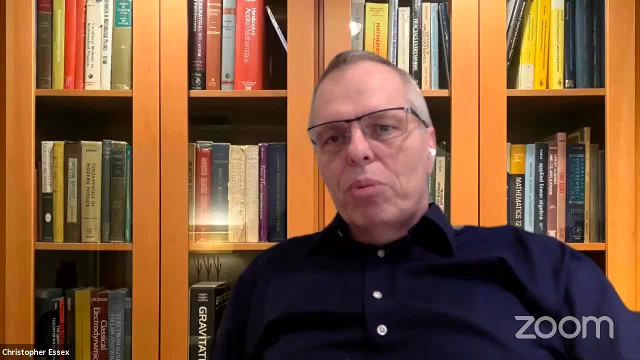 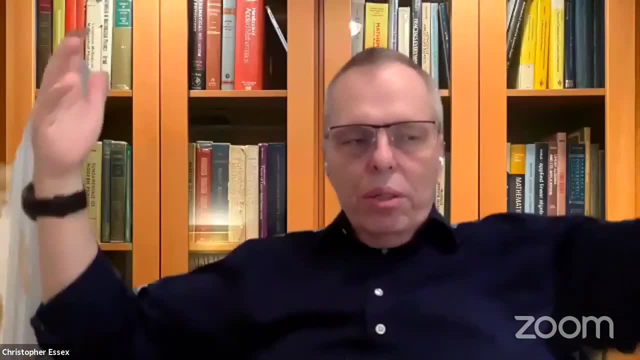 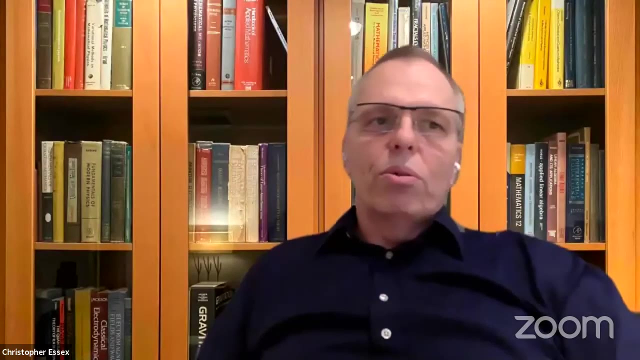 like that. But in the real world exponentials have some kind of limiting principle and they never go off forever, right? So there's always some process external to the model that limits it. So epidemiologists came up with a simple way to fix that, or population theorists. 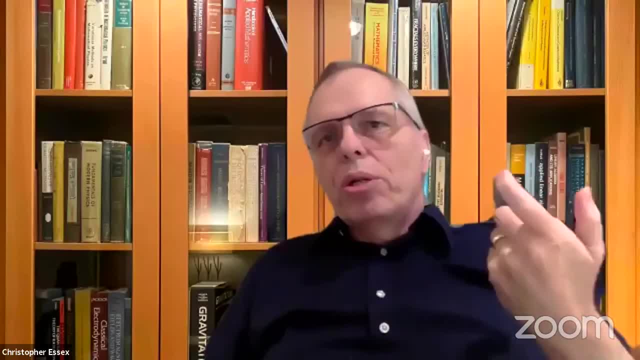 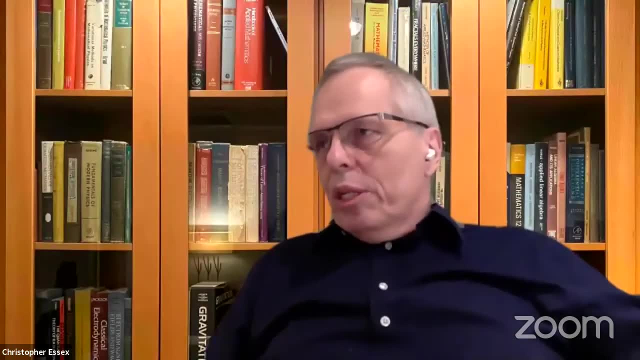 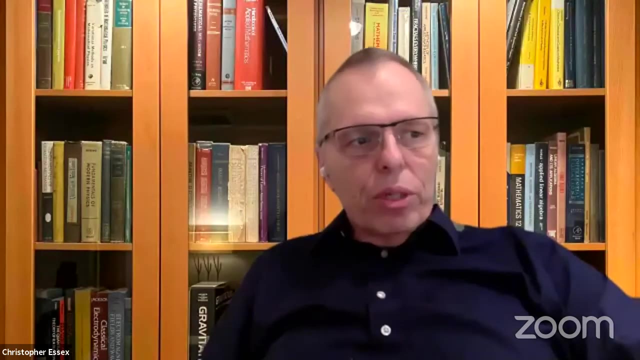 And you would turn it into a nonlinear differential equation. you put a difference that would be proportional to population. It's proportional population times some population minus some kind of fixed value- And this is now a nonlinear differential equation and it changes the solution. So instead of the population growing exponentially, 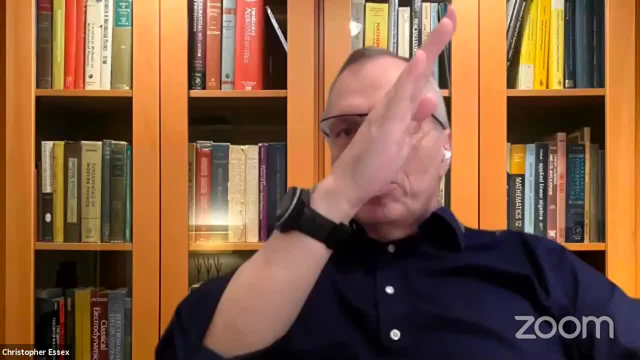 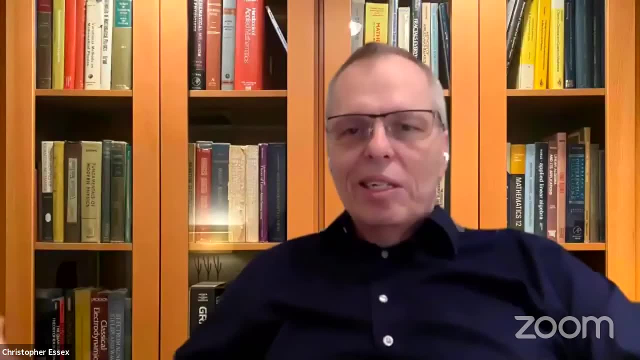 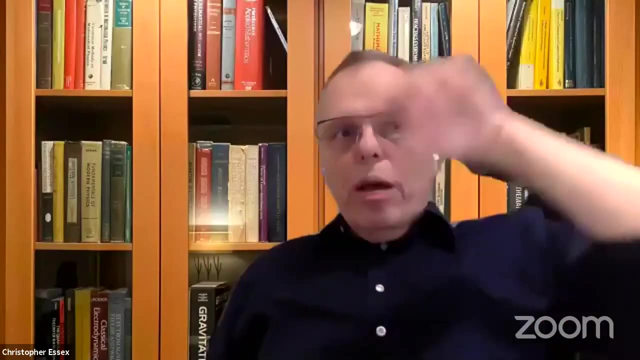 it still is exponential and grows exponentially, But eventually it starts leveling off And this kind of curve- it's a rather famous curve, It's referred to as sigmoidal And it's become very well known as a very effective way to model epidemics and so forth. 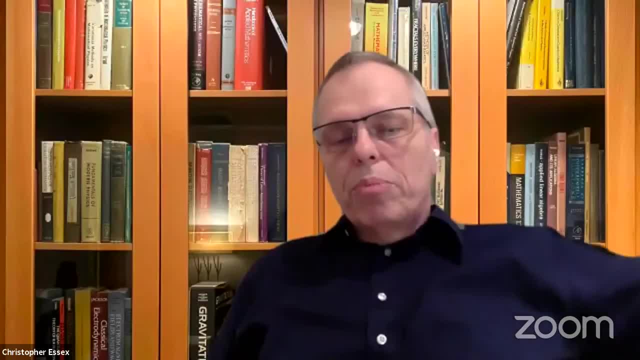 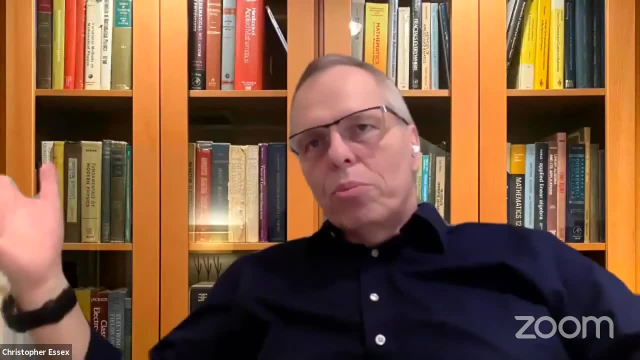 in many cases you have the growth and then you have the turnover at the top, And it's a very simple thing. Now I really wanted to talk about that particular differential equation, And don't be concerned about words like differential equations, just the rule that. 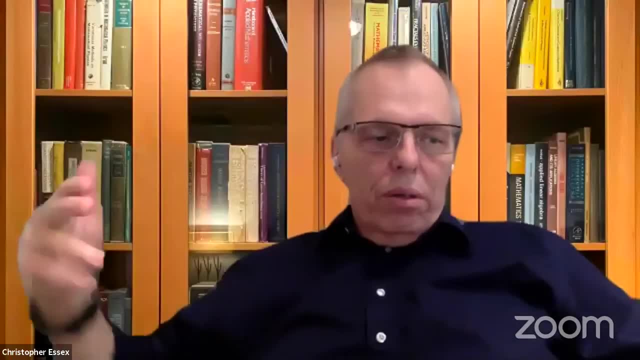 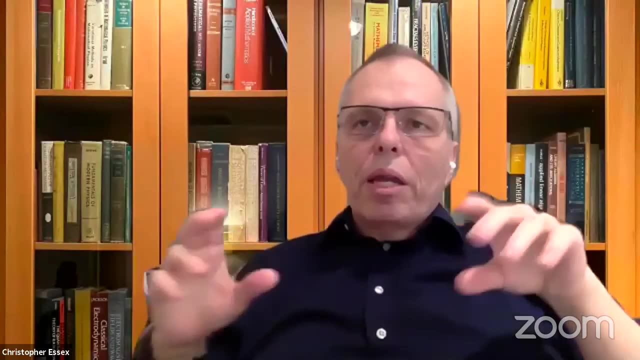 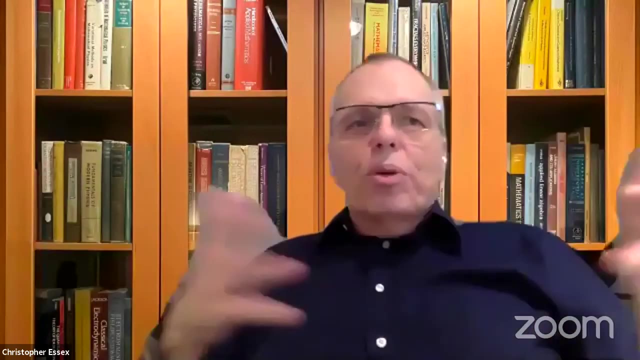 relates one thing to another, involving certain properties and calculates and so on. In any event, if you take that differential equation and you want to put it onto a computer, this is a very important thing- is that you discover that you can't. You can't put differential 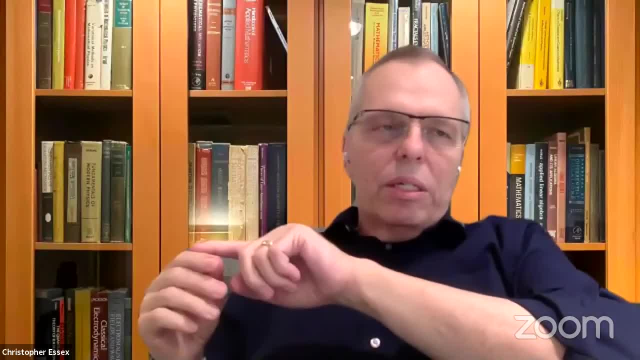 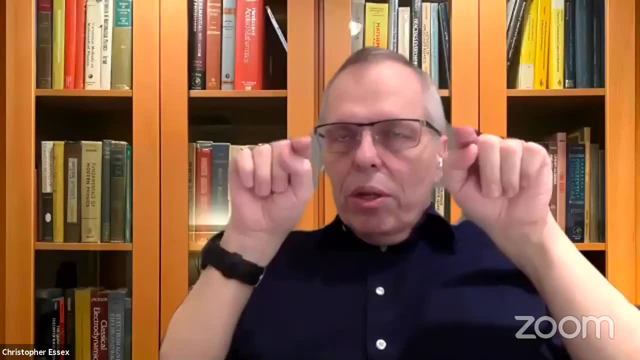 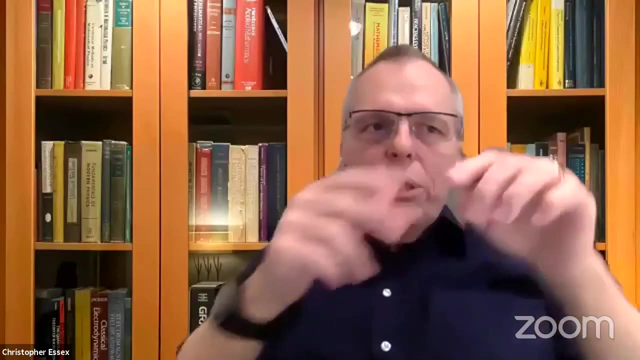 equations onto computers because of the fact that differential equations are continuous- in this case continuous in time- And the computer only has individual values. And so what you have to do is you have to take the differential equation and kind of cut it up into little pieces. 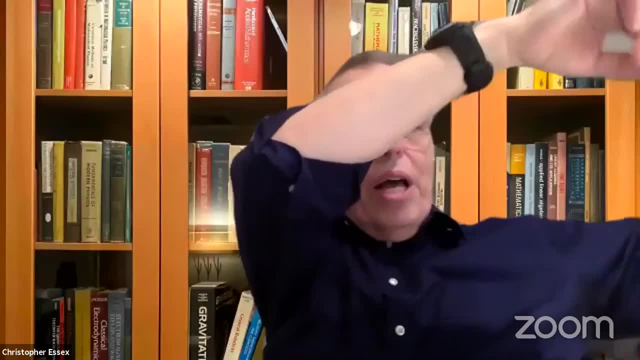 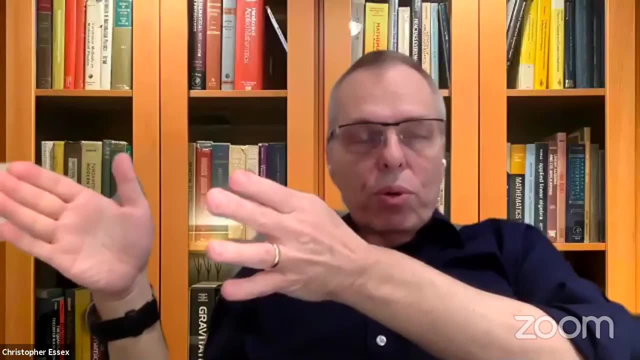 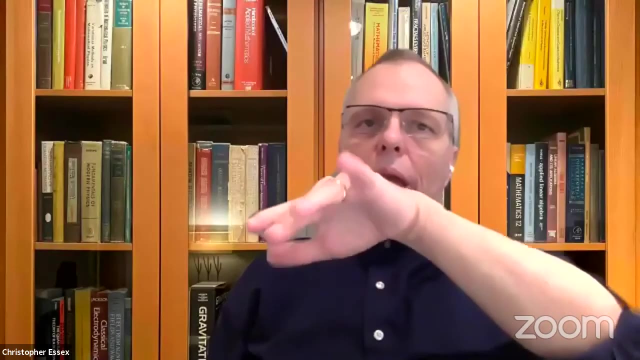 And then drape it over the individual values that the computer can generate, And so you actually have a different object. in this case, the logistic equation- which is what it's called because it's so famous- gets converted into the logistic map. So it's a discrete map, And this discrete map has 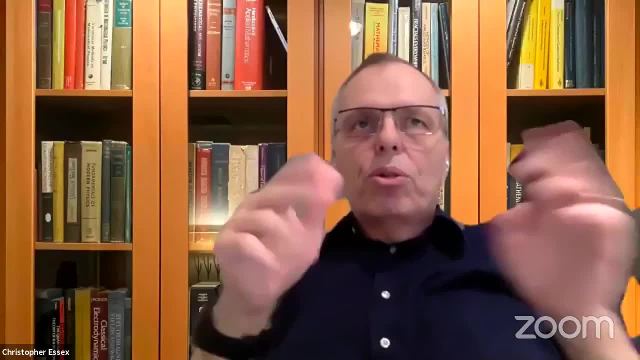 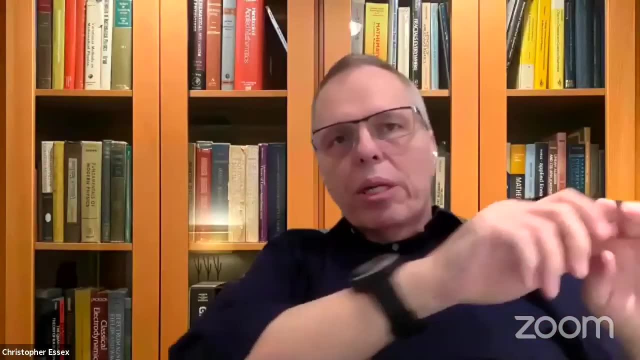 properties that match the differential equation. That's why we put things on computers. We want to get them as close as we can. the discrete map to the continuous differential equation. But if you push it a little bit it starts exhibiting completely new behaviors. And, of course, 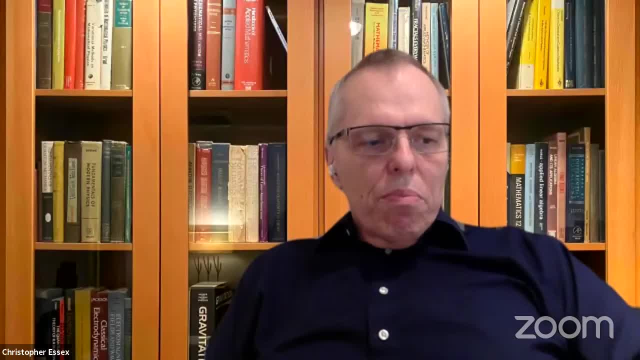 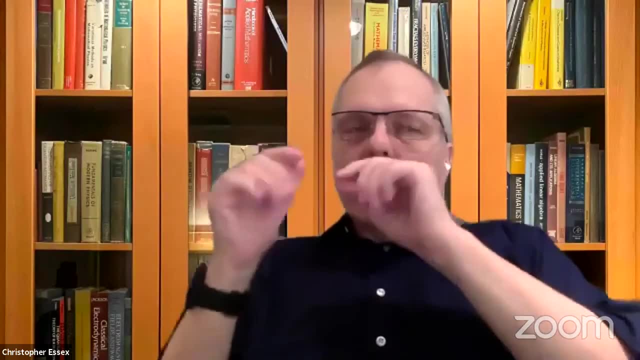 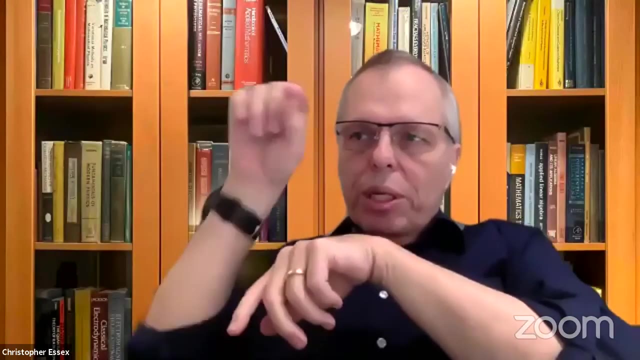 it's famous to study for a lot of reasons. But it also pertains to the issue of predictability. And if you take that discrete map and you modify it a little bit and push it into its extreme ends, you can get a situation where you get a value, you perform the operation, get the next value. 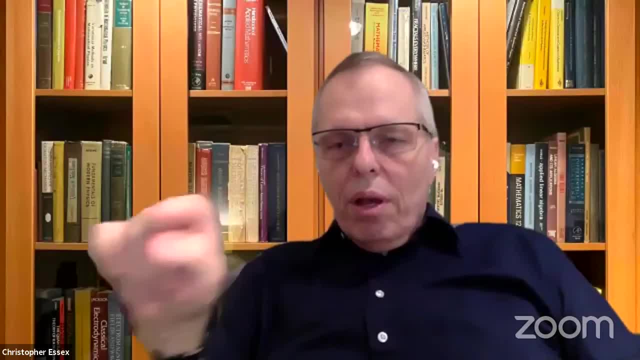 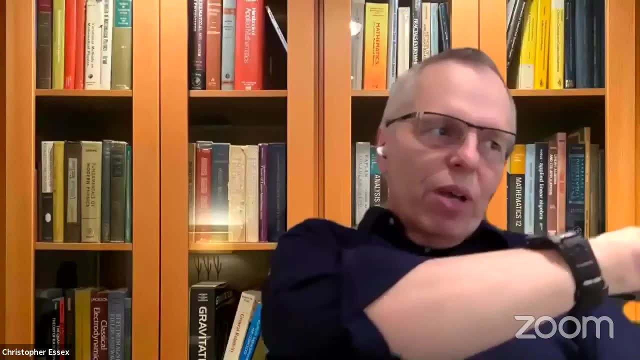 perform the operation, get the next value, And what you'll get is you get a value and then you do it and you get the same value, and then you get the same value, and you get the same value, and the same value and the same value, And so it's completely. 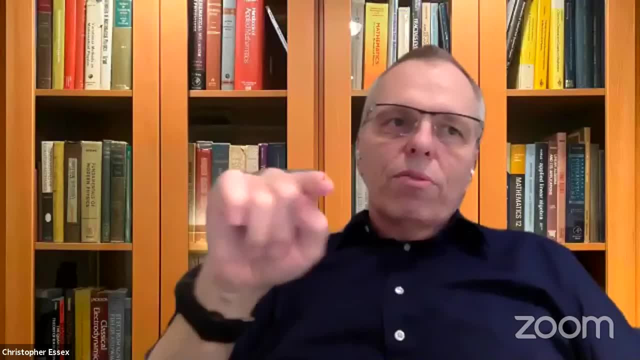 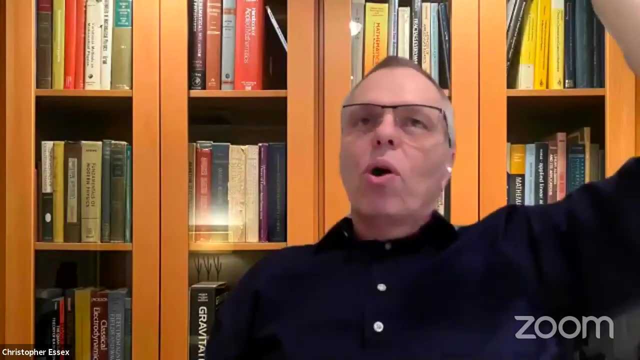 constant, And you can do this all day long until you basically fall asleep And then at some point, boom, it switches to a new value, And it will go on and on like that. And so people have this idea that, because there's this constant behavior, suddenly a jump. 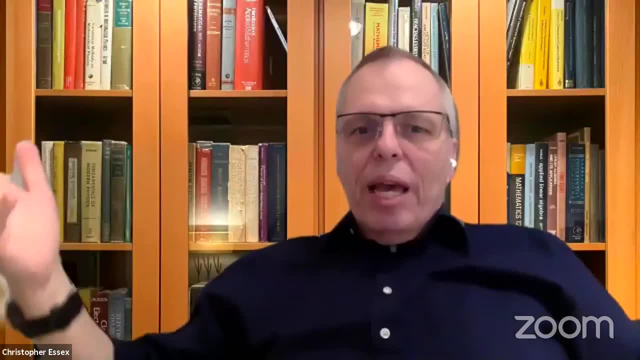 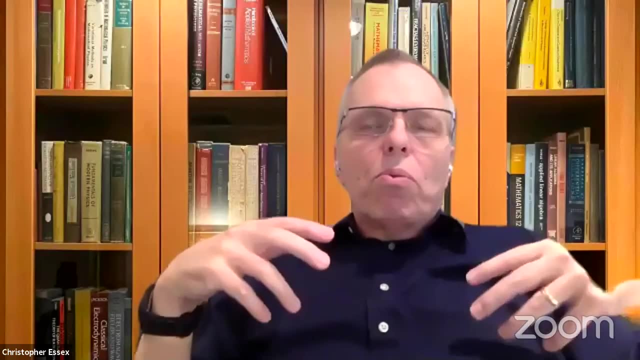 that there's some external cause that made that. But there's no external cause, It's a property of the internal dynamics that actually causes that jump. So what that model does, it provides for us, it provides a new conceptual window, It allows us to 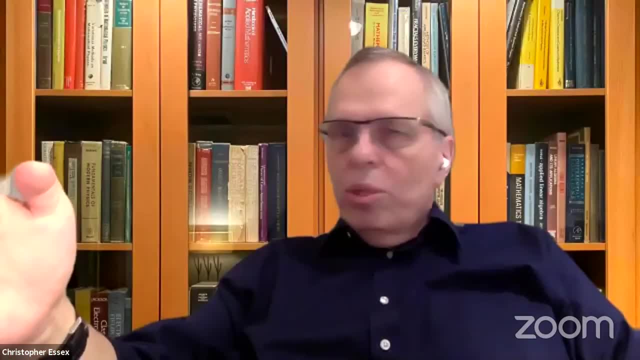 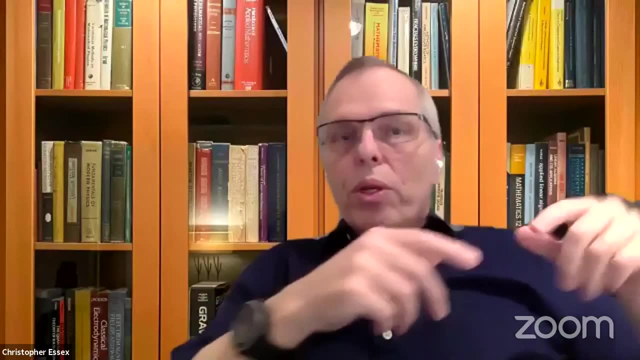 think of the world in a different way than we thought was even possible in the world. And that's what a lot of these models do. They're not used for predicting what some policymaker wants. They're used to broaden our minds. So we have the case of one differential. 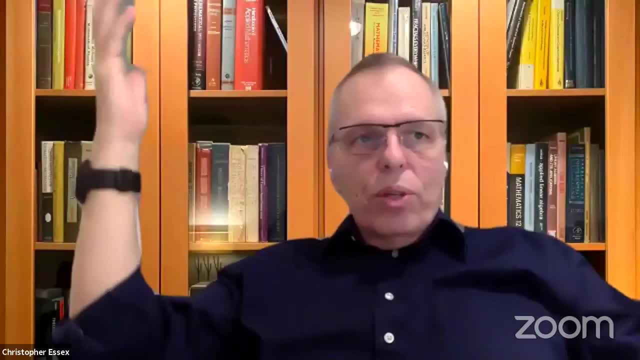 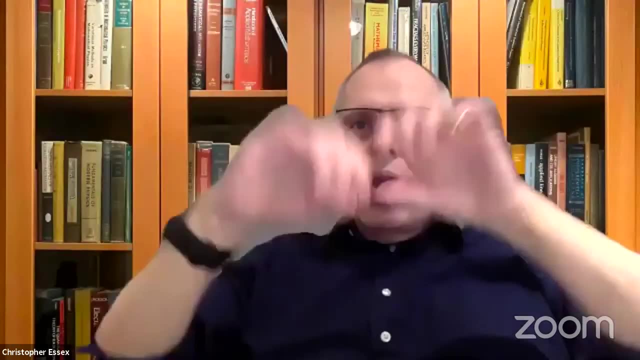 equation And you can make more complicated models, say of the weather, for example. And you, for example, if you have one differential equation, you can't get this unpredictability. If you have two differential equations, you can't either. 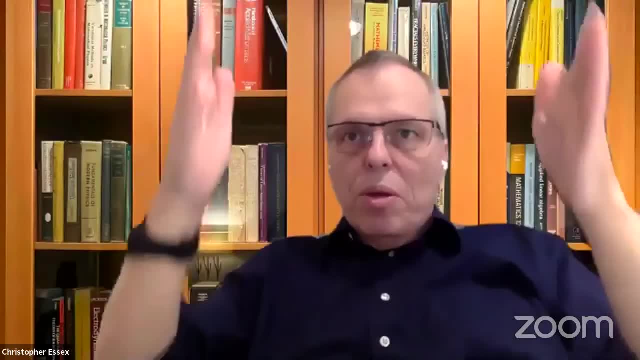 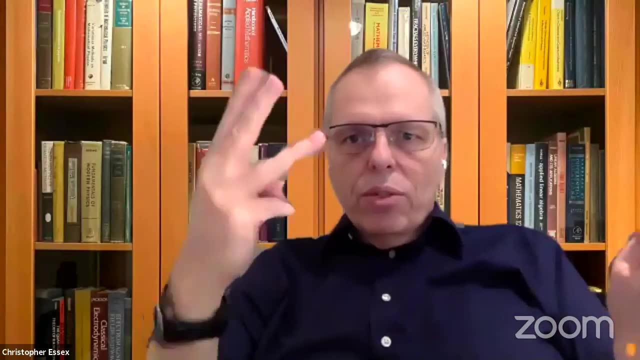 And there's a famous theorem called the Poincare-Bendixson theorem that says that with only two differential equations you can't get this unpredictability, But if you have three, then you can. So in fact, you've probably all heard of Lorentz's butterflies. 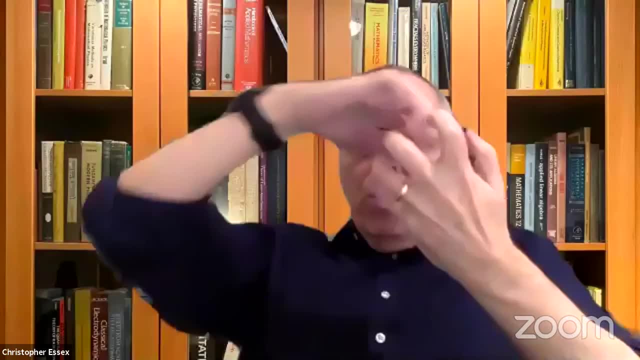 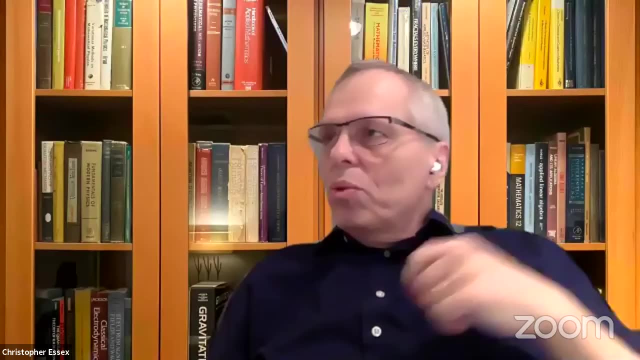 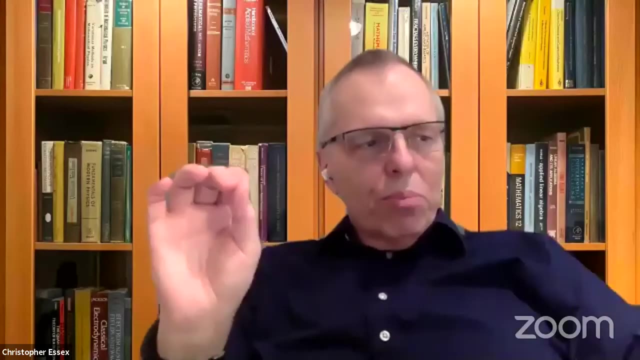 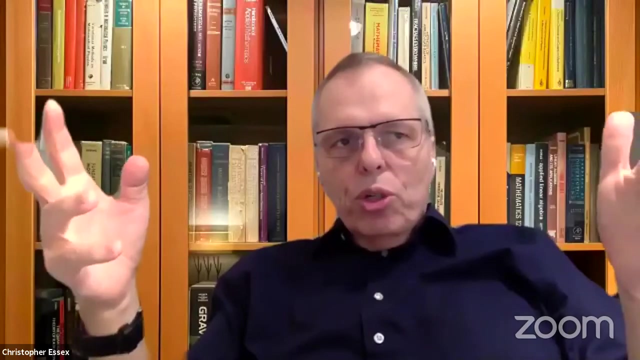 There's a system of these differential equations. They're all coupled together And these exhibit the differential equation. That's not really the point. The point is that you can have a model which has absolutely no value for predicting the future. Lorentz's equations don't predict anything that's useful for us. 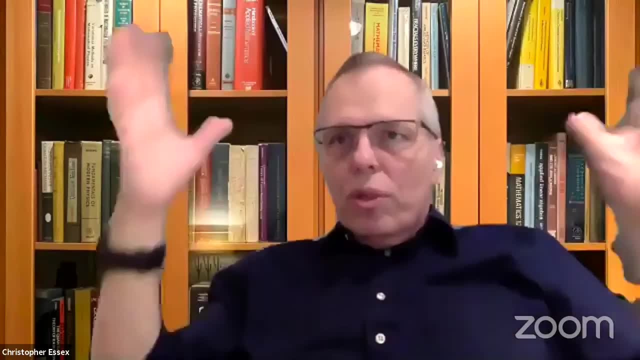 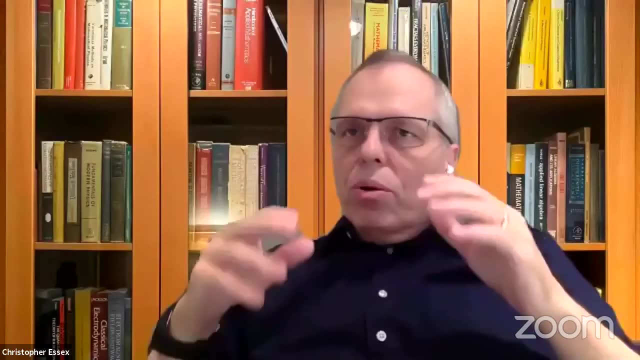 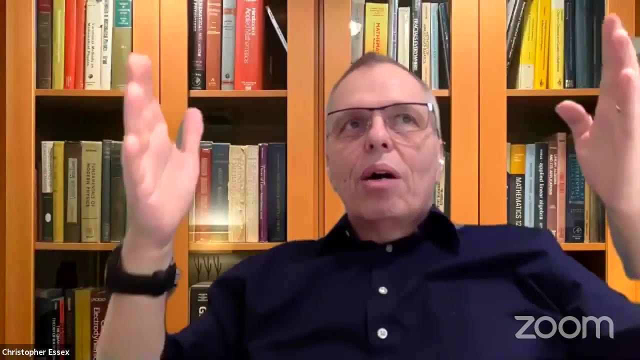 But what they do do is they in essence they cause a kind of revolution in the 1980s and 90s And 2000s in how we think of the world. So it's probably the most profoundly influential, important model. that's of no use for predicting anything, And so it's important you understand. 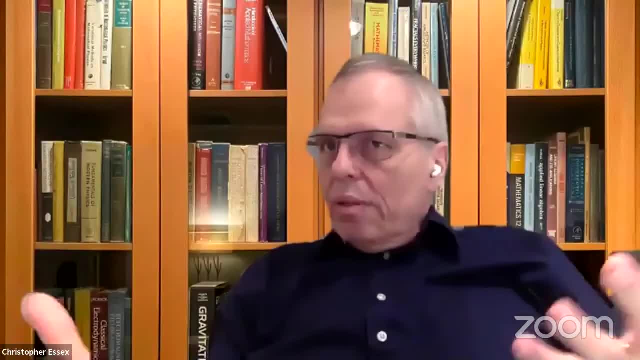 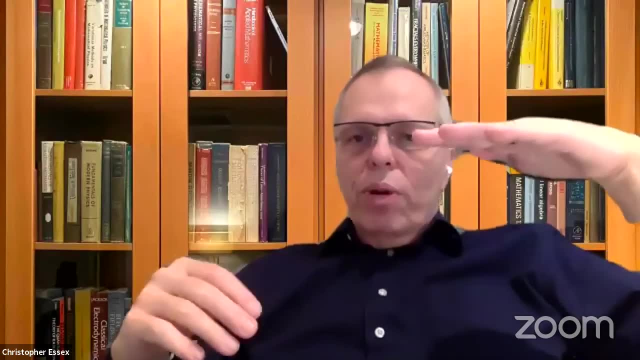 the nature of what you want to get out of a model. So that's this example. Now if we push on on the population point of view, if you do mathematical biology, you will find that you work with these kinds of mathematical objects. You have systems of these. 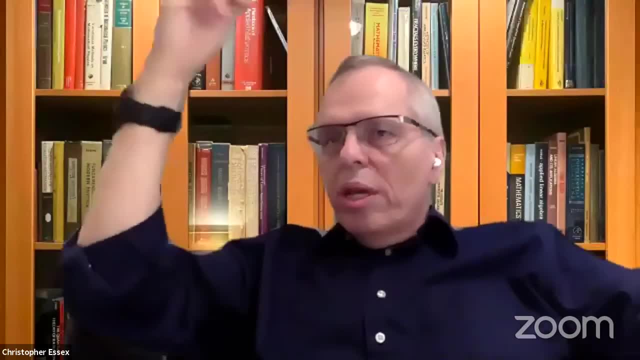 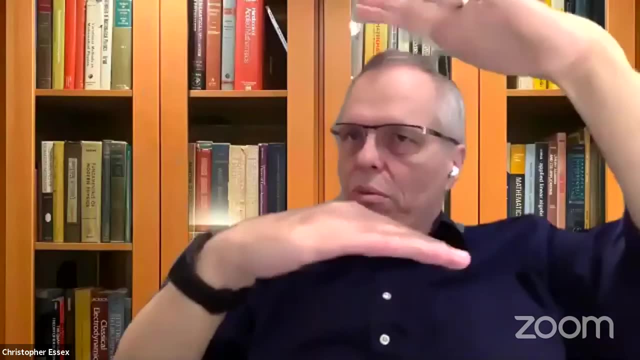 equations, talking, for example, about, say, infection, And you'd have a system that could be very complex. You have maybe 10, 20 equations- you could have hopefully smaller- And they're all coupled together And you'd have to use a computer to figure out what's going on. 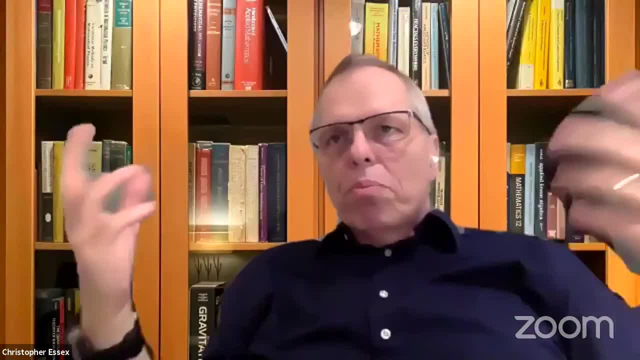 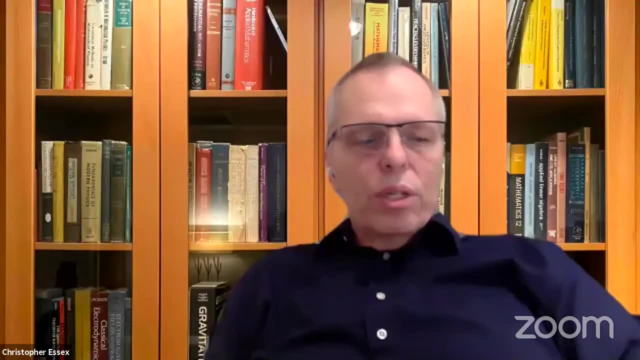 But these models are still ultimately incomplete. There are approximations of what's going on, but they're very important. One of the famous cases is the issue of AIDS. Probably you all remember about HIV. Well, in the beginning, people used to think that 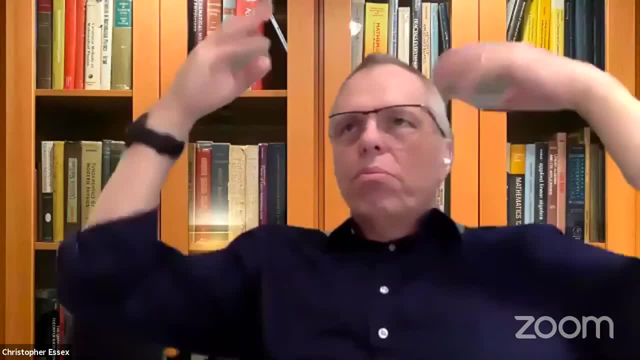 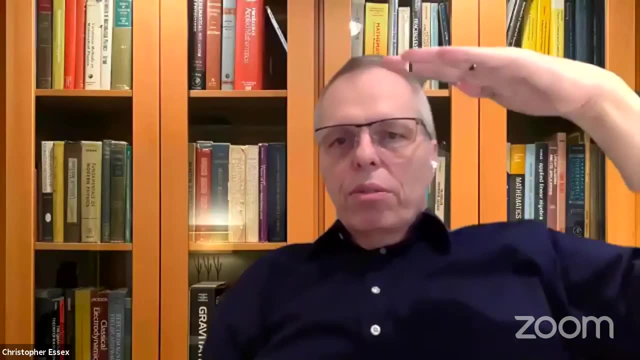 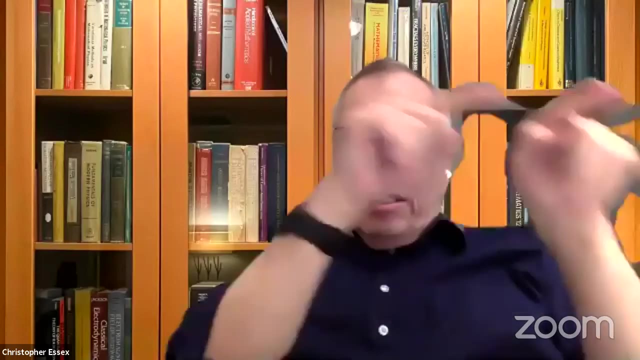 the HIV virus would just sleep. You'd get the HIV and it would sleep for 10 years and suddenly it would wake up. But there's a guy by the name of Perelman and his team. they used the system of differential equations, They used the data and they put them in. 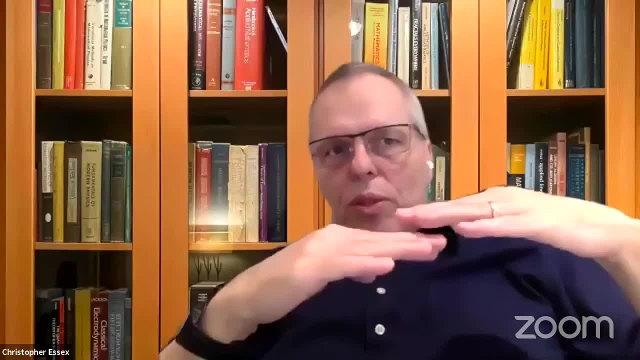 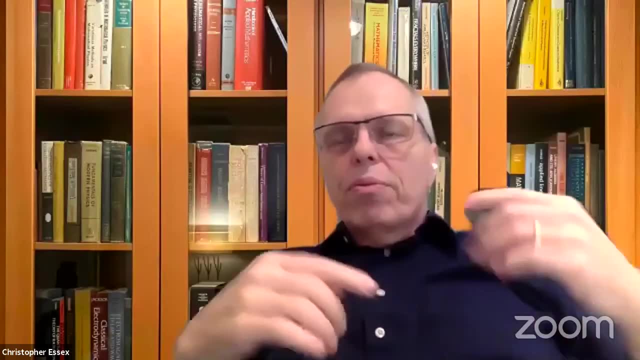 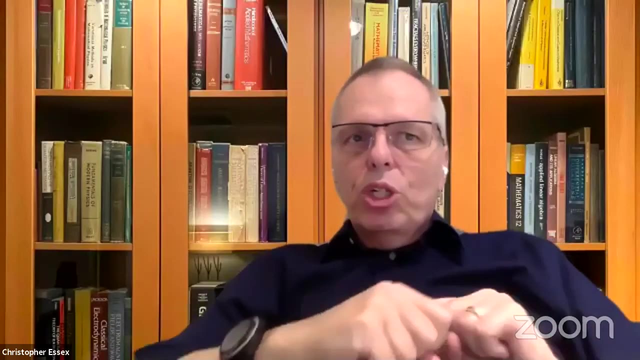 and they were able to figure out that what was going on wasn't what people had thought. HIV wasn't sleeping, It was ferociously active and the body's immune system was suppressing this activity and keeping the virus numbers really low, But eventually. 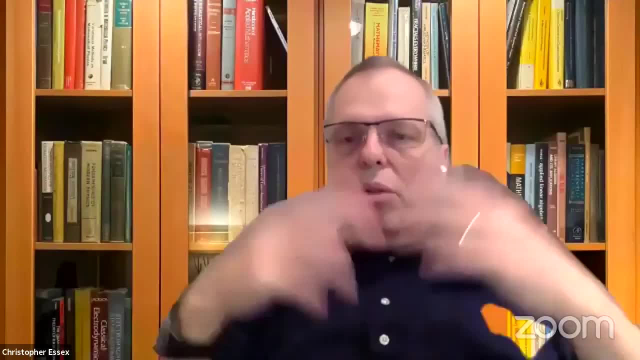 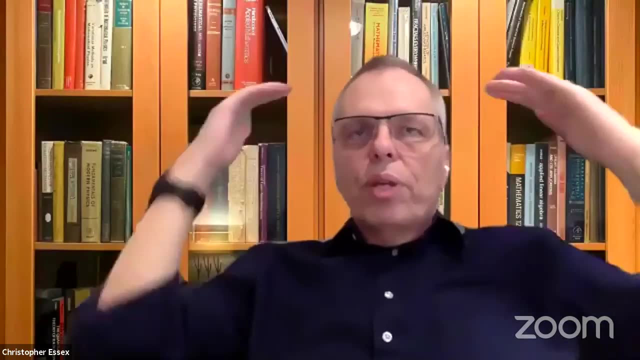 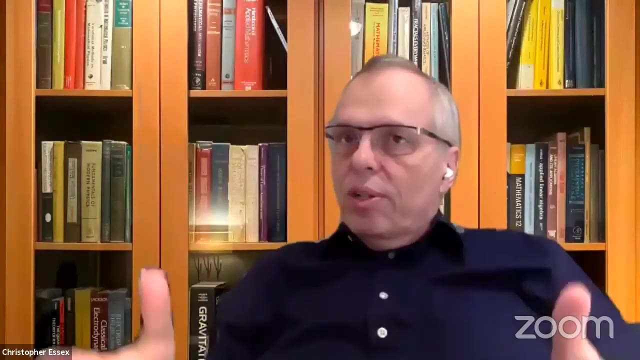 it just became overwhelmed, and then that's what would happen. So it's a completely different picture, And so, in essence, there was a confusion that existed in people thinking that a small number would correspond to a small rate, a small activity, And this system model proves. 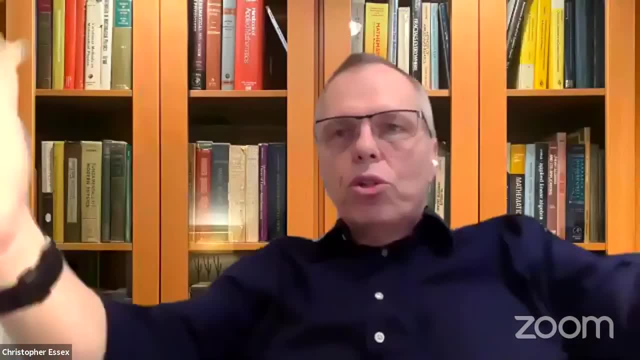 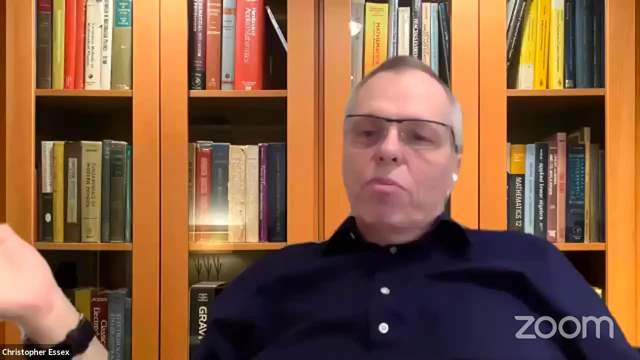 that wasn't the case, So it's nothing to do with prediction of the future, but this led to multi-drug treatments, full spectrum treatments that saved many lives. So it's important to understand that models have this important utility, which doesn't involve just predicting. 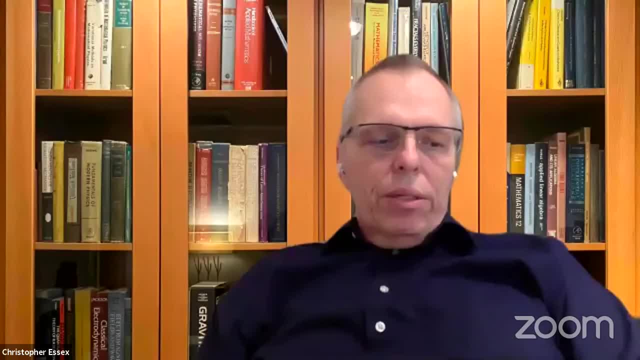 the future and so on. Now, if we want to get into things like climate models, we have a different creature. Originally, climate models also are based on kind of cartoons and they're sort of quasi-empirical cartoons And if you use 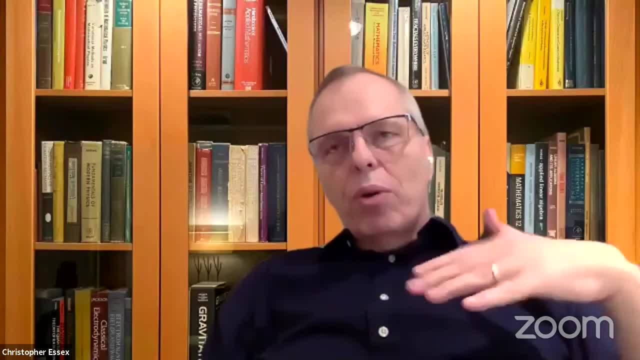 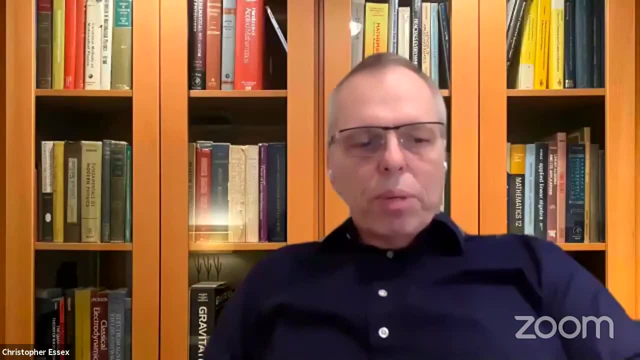 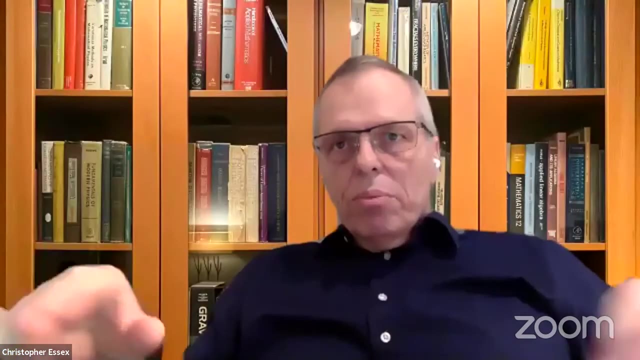 these models in such a way that you're trying to answer scientific questions like the ones that I kind of have sketched out. there's some value to them. The problem comes in is when you start trying to use them for policy purposes and you're trying to forecast with them. 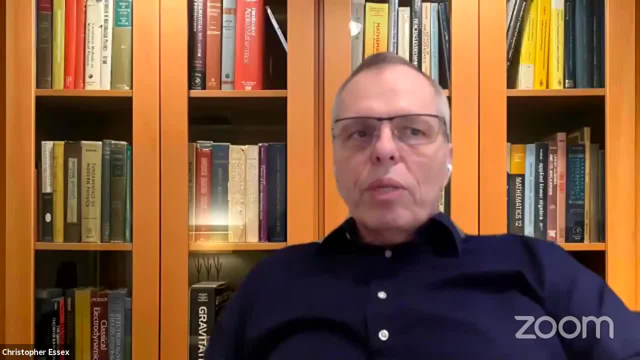 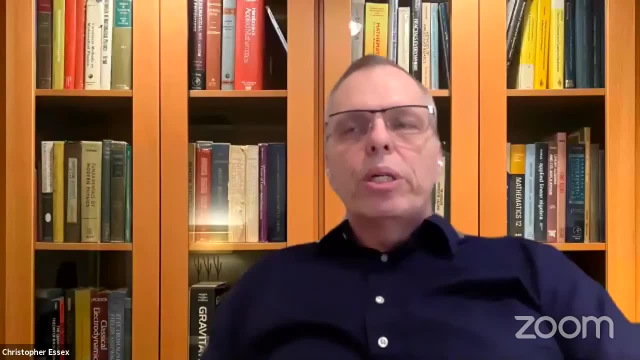 the way you would with a meteorological model, then you're in a very different world, Because the questions that are being asked or answered, apparently are policy questions, And this is something that has to be kept separate in people's minds. There's the scientific world. 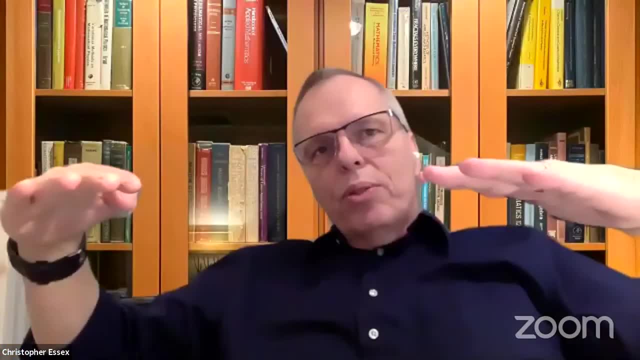 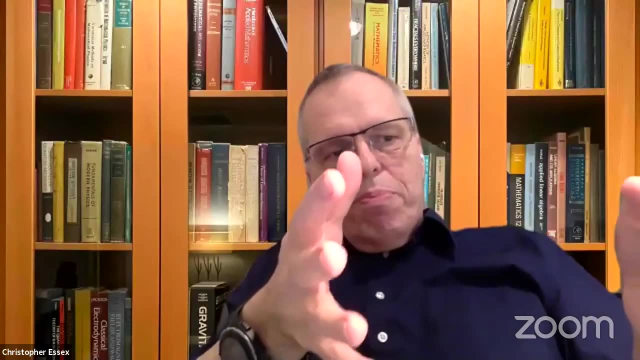 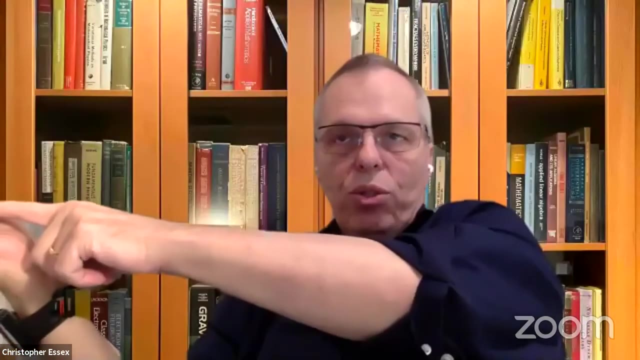 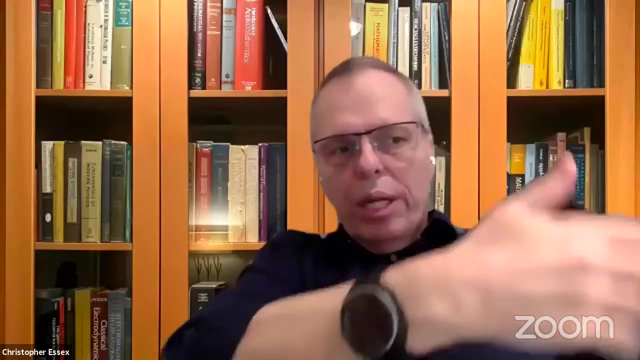 and there's the political world And unfortunately, what happens in the use of these policy questions applied to these models is it tends to paralyze the field. The field becomes locked into the need to provide answers to the policy people, which then stops questions being answered or asked, particularly about the nature of the 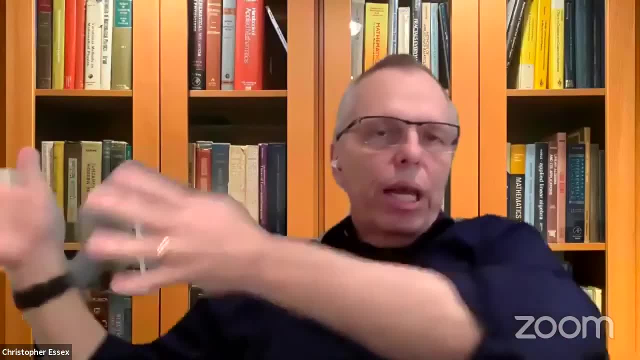 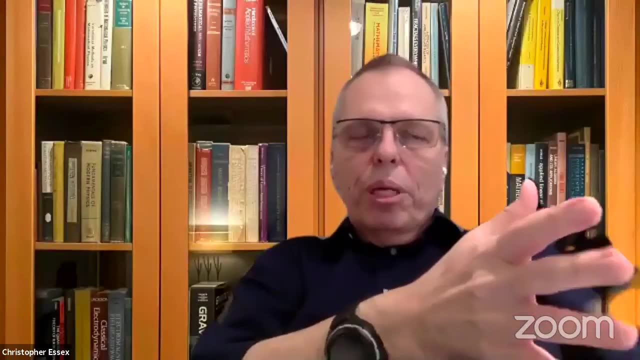 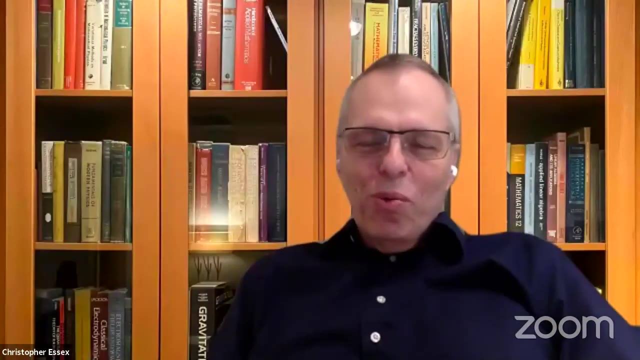 science, And the concern is always: how does that play into the policy issues? And I think that ends up distorting both things. The science becomes distorted and the politics becomes. well, it's always distorted, but it becomes distorted in its own way. So there's a range of 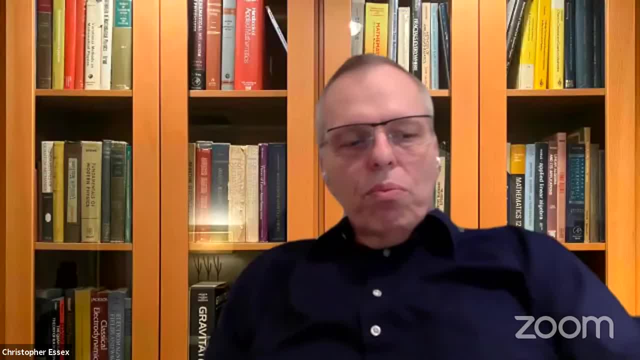 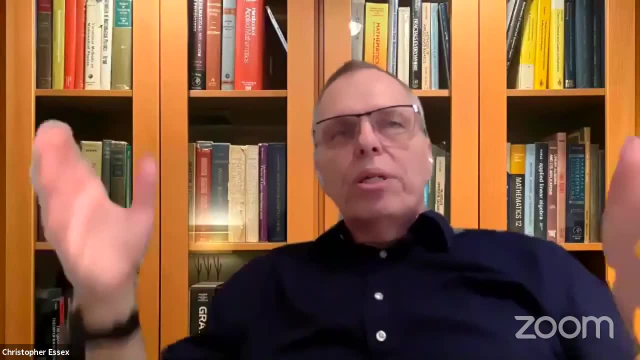 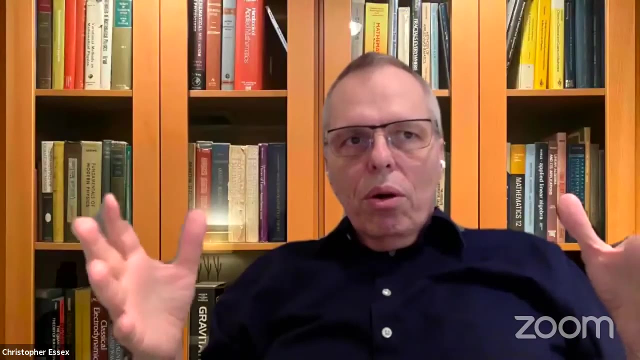 issues here And, ultimately, these modeling issues are well, models are basically cartoons and they're not something that should be treated like commandments engraved in stone. They are wobbly, wonky things And the people who use them for making policy decisions. 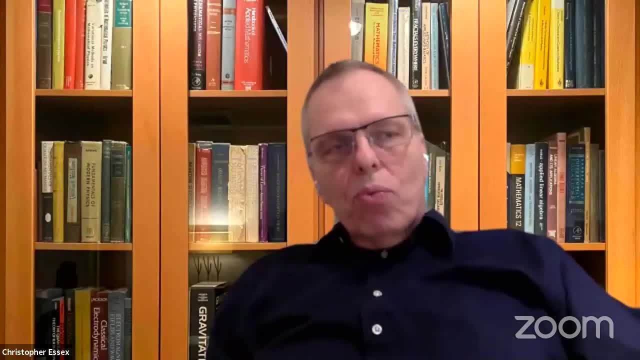 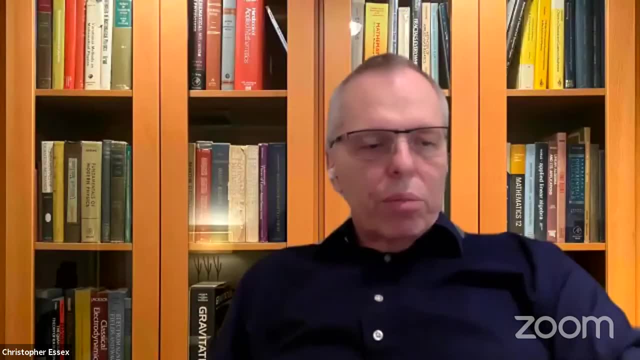 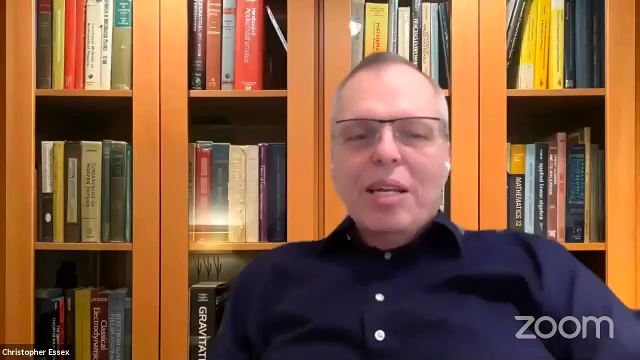 have to start asking questions about what the weakness is in these models. So, for example, we recently had a big discussion about a certain model in connection with virology recently, and everyone's now saying, oh, the model's really bad. Well, 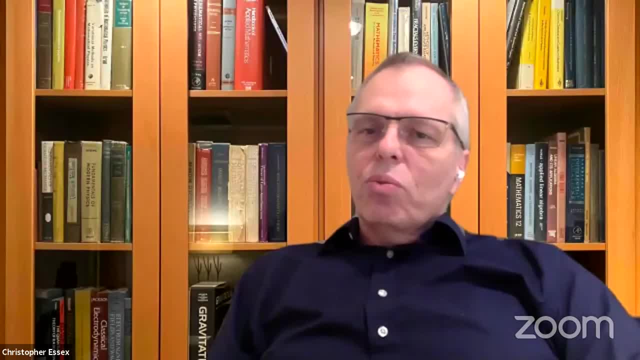 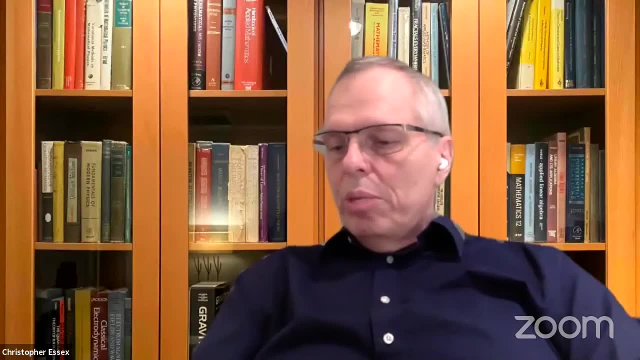 models are often bad in some respects. The question is, what do they actually do? And if you, for instance, were to ask certain questions, if you're going to do an epidemiology type question, you know that there are going to be exponentials in there And you can easily ask. 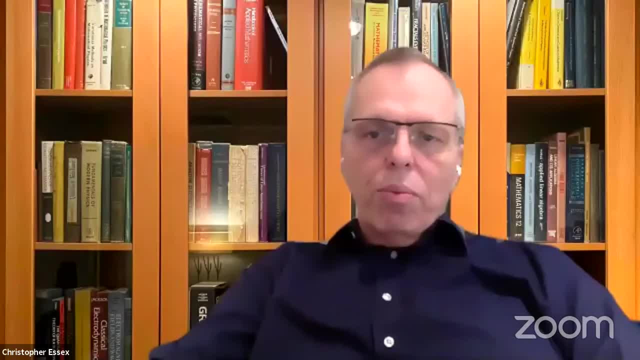 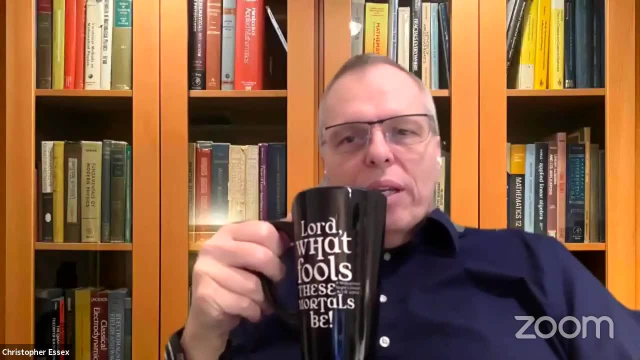 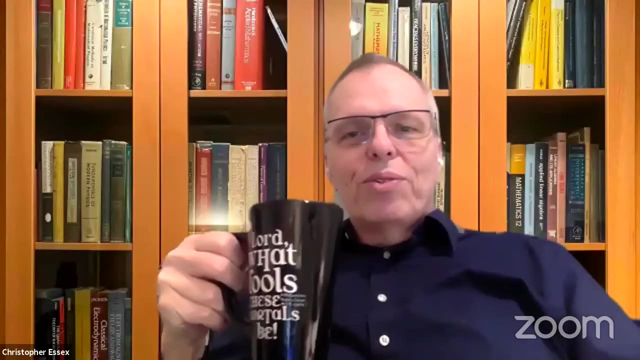 if you tweak some parameter this way or that way, how much does it change the outcome? And I think in this case it turns out it changes things a lot, And that would be something that a policymaker should be immediately cautious about. But, as you know, that's not how things work. 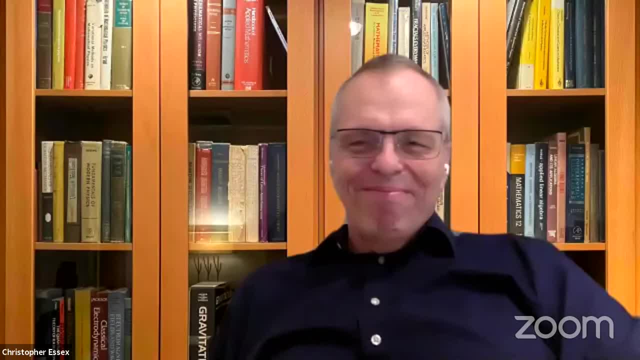 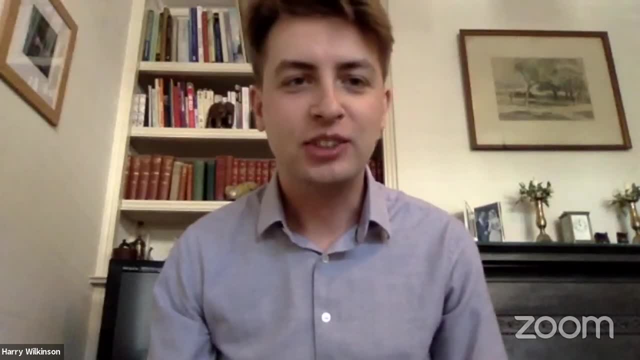 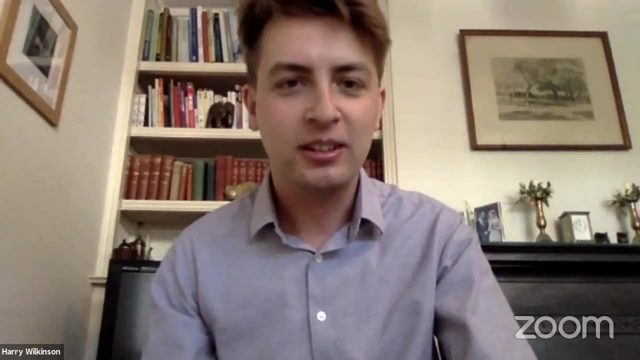 Okay, that's all I have for my opening remarks. Thank you very much, Chris. Right In a slight change to how we have done things in previous webinars, rather than me question Chris individually, we're going to have each panelist in turn and then we're going to come back at the end. 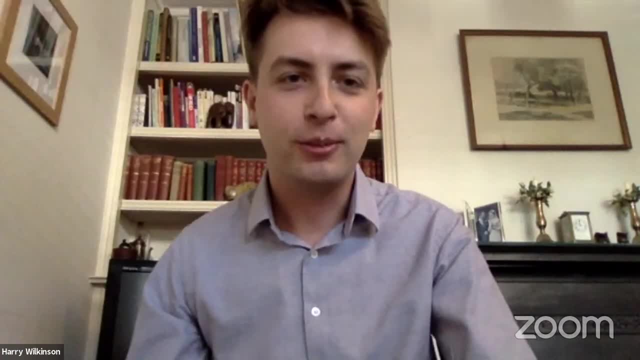 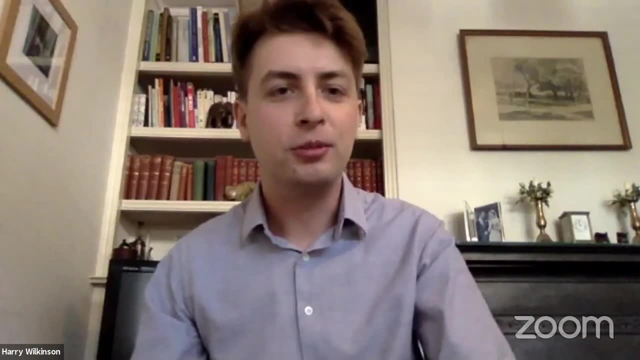 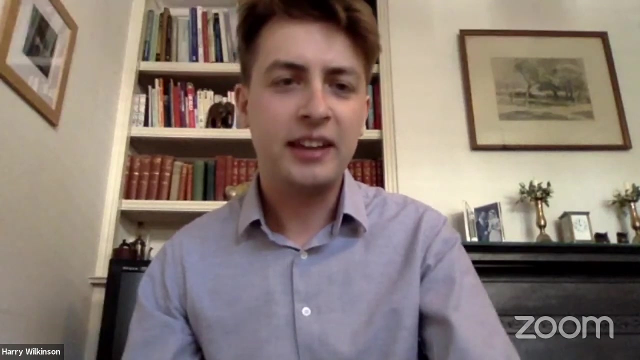 and try and have as many questions from the audience as possible, So I'm going to introduce our next guest, which is Professor Gordon Hughes. Now. I thought it would be very important to have an economist with us today, Because so often the applications of science in policy terms don't always. 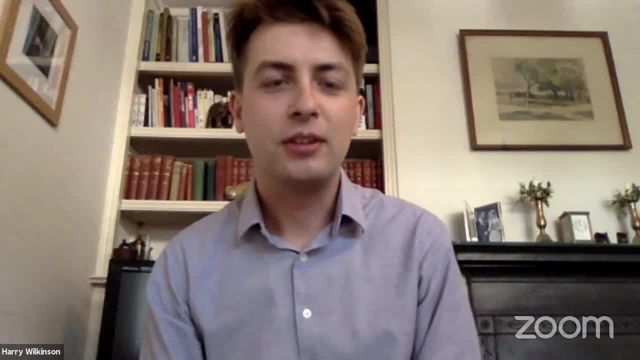 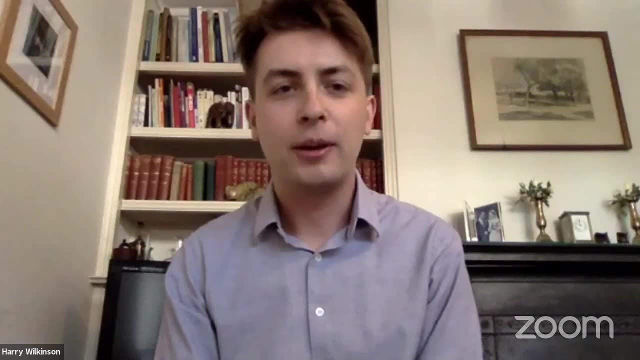 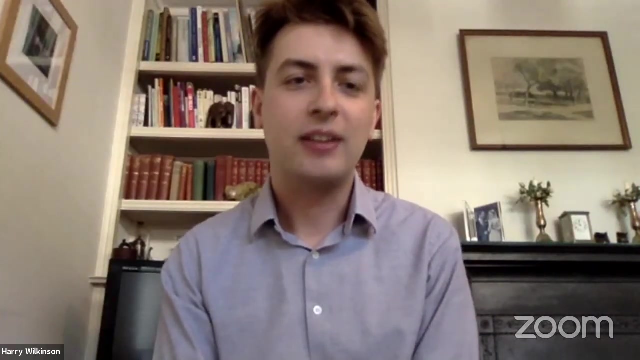 work out, as perhaps scientists or even politicians themselves had first anticipated, And understanding how markets work, how economies work, is often so important to be able to have a sense of what makes it better. So we're going to have a first question from Professor. 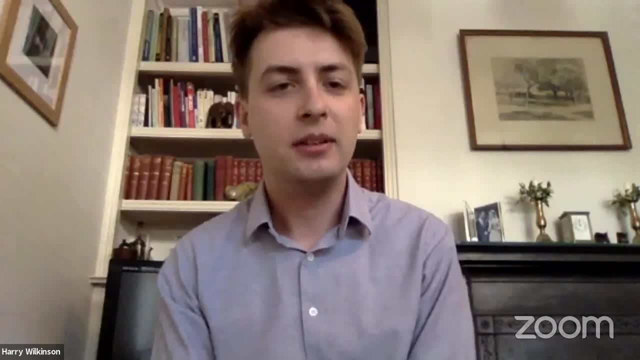 good sense and practice, and we've got a very eminent economist with us to discuss mathematical models. He's an emeritus professor of economics at the University of Edinburgh and indeed he worked with the World Bank for many years, working with them on energy and the environment. 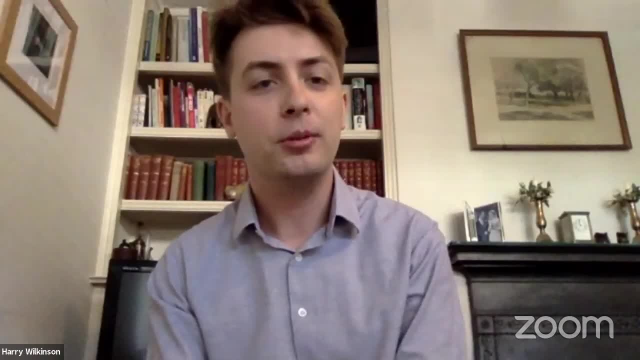 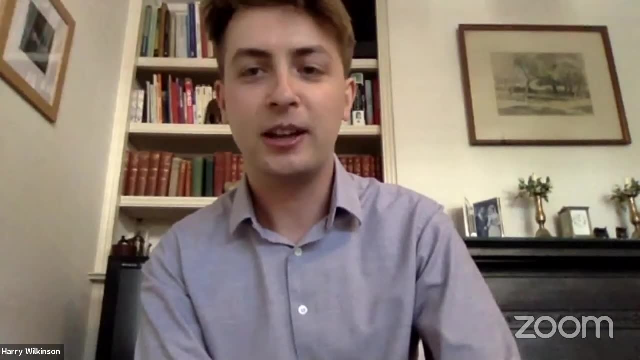 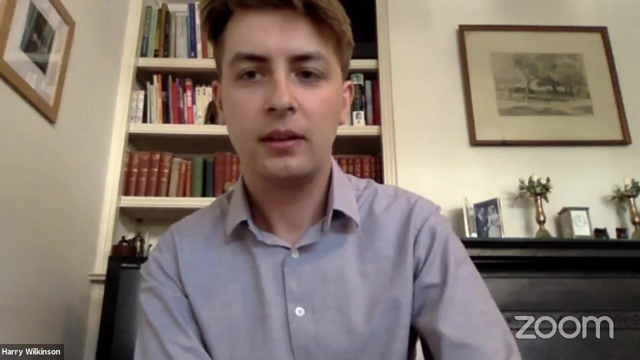 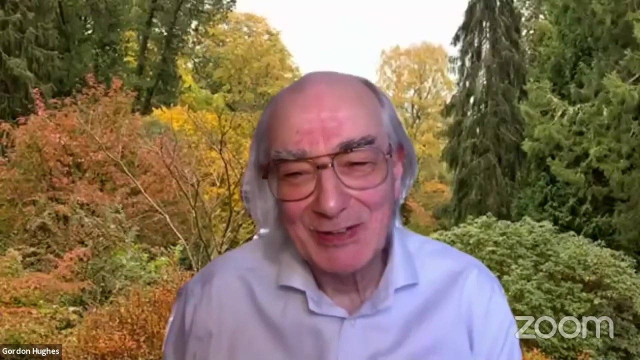 and was responsible for influencing many of their important environmental policies. So, Dr Gordon Hughes, thank you very much for joining us and I will hand it over to you for your remarks. Just a word about background, since I noticed some of the comments on Chris's thing. I'm not 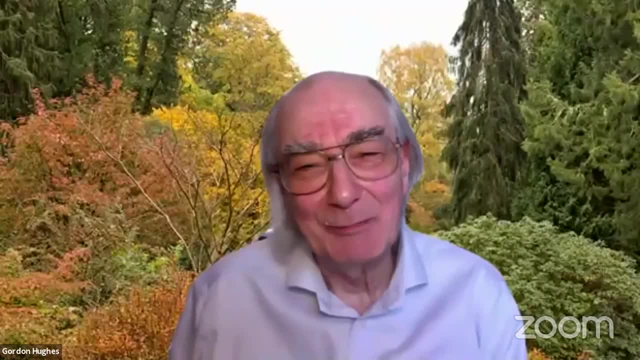 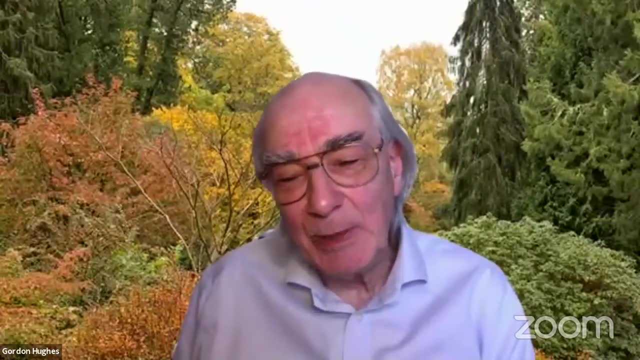 sitting in the garden with trees. I'm sitting in the garden with trees. I'm sitting in the garden with trees behind me. I too have a background set to advertise where I live in the Scottish Borders. Let me give you first of all a little bit of background to myself, in other words the kind 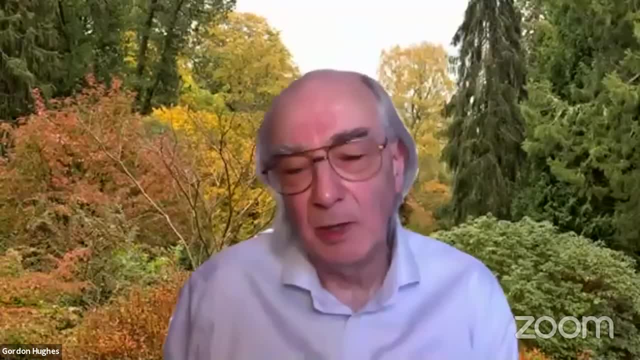 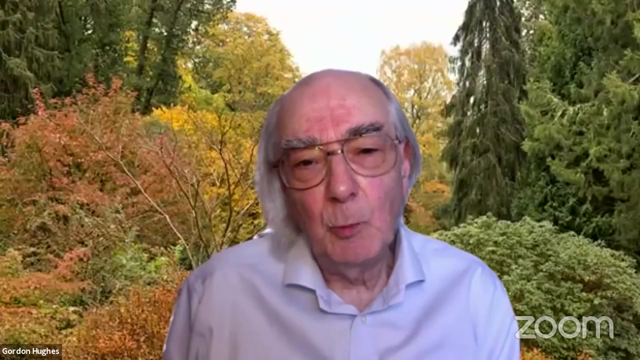 of ways I've used mathematical modelings in policy, and I'm going to speak specifically about my involvement in Eastern Europe and the former Soviet Union from roughly 1988 to 1993, where, for those whose memory is short, the economic changes that occurred with the 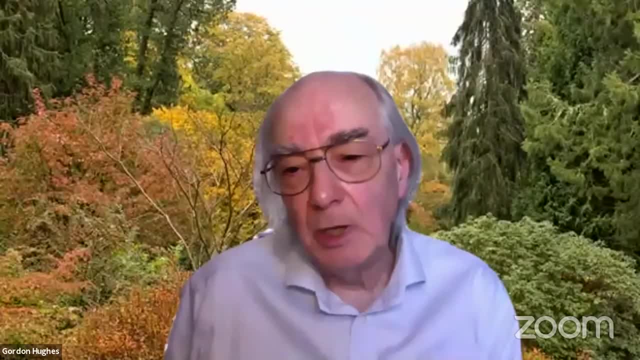 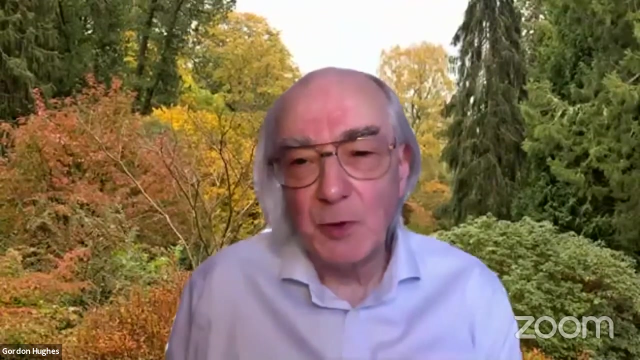 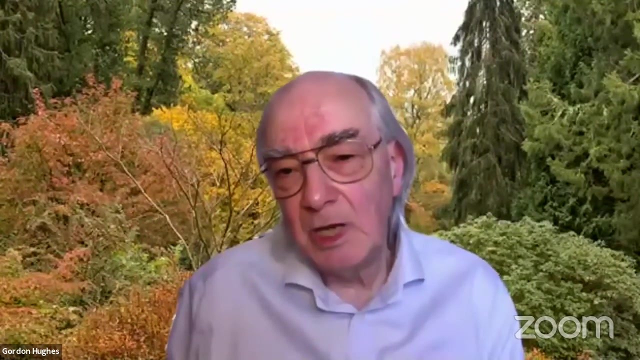 collapse of the former socialist system were as traumatic and as large as we are currently going through, and indeed, in many respects it was even more upsetting for large parts of the population because the prospect of emerging from it was a great deal further off than we are currently living through. and I was involved because initially I had been working with 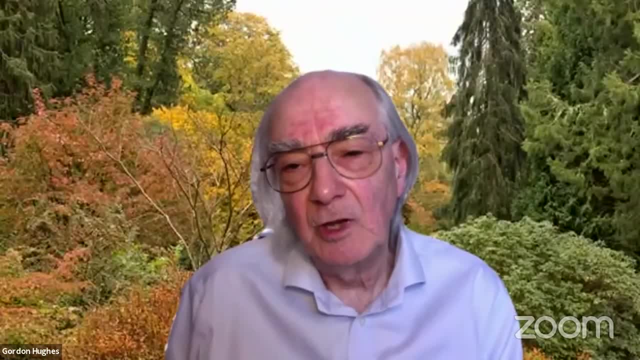 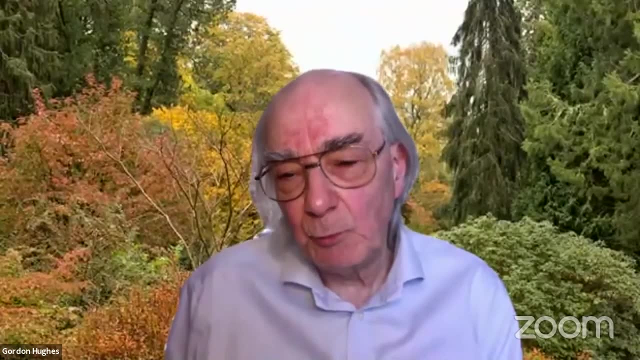 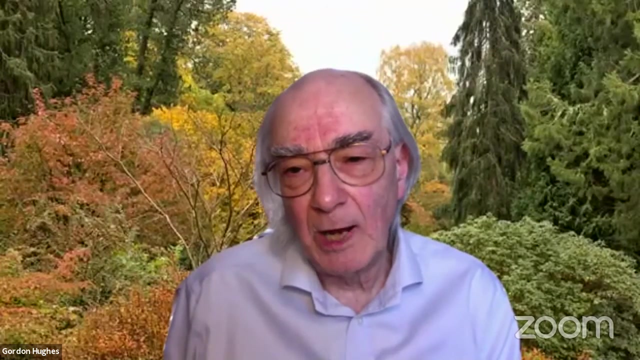 the Academy of Sciences in Poland on energy and other related matters, developing some models, because it was becoming clear that things were going to have to change. this was in 1986, and we worked together quite closely for a couple of years when suddenly it all broke up and the next 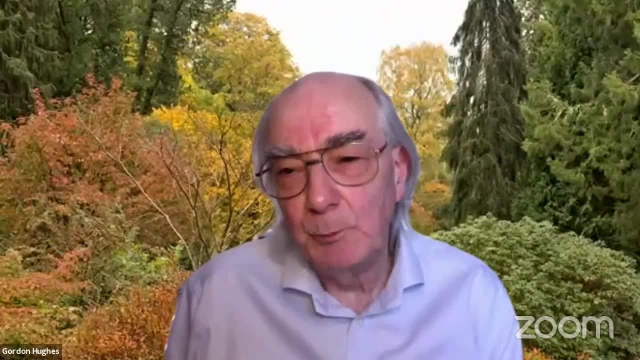 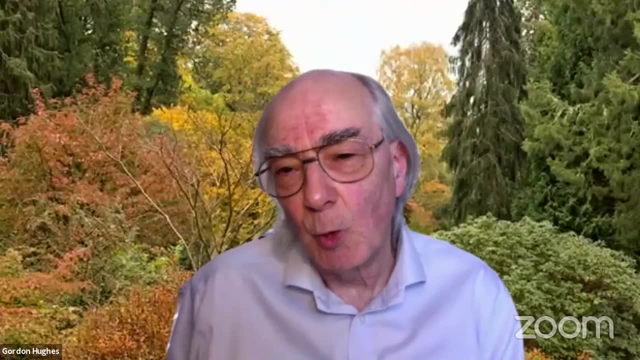 five years were, from my point of view, both extremely exciting but extremely demanding, because essentially, the whole region changed almost out of out of expectation, and it so happened that I had built with my colleagues models which were actually went to the heart of a lot of the changes that were occurring: the collapse in trade, the very 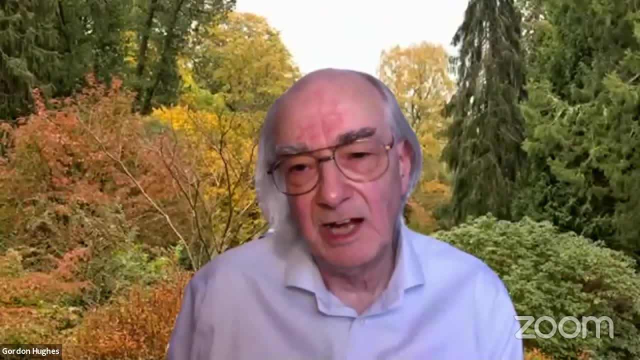 radical rises in energy prices and a variety of things like that. now, there were a number of lessons that came out of that. first of all, forecasts directly were not the main product of the models. it was an understanding of the links within the economy which were likely to be. 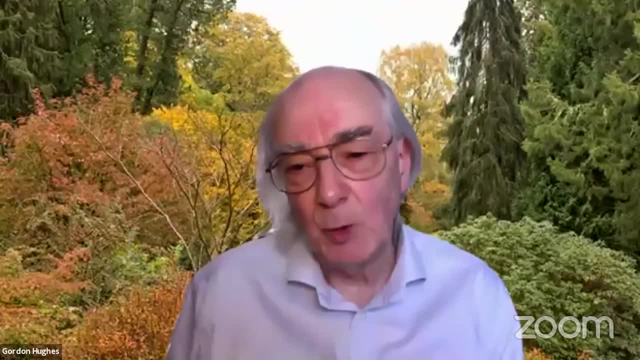 important to people's incomes, to employment and to a variety of other things in future. the other thing that was important was the closeness and consequence, the trust that was built up between me and the people that I was working with and, later on, the politicians that I was advising, that essentially, I both understood and sympathized, and 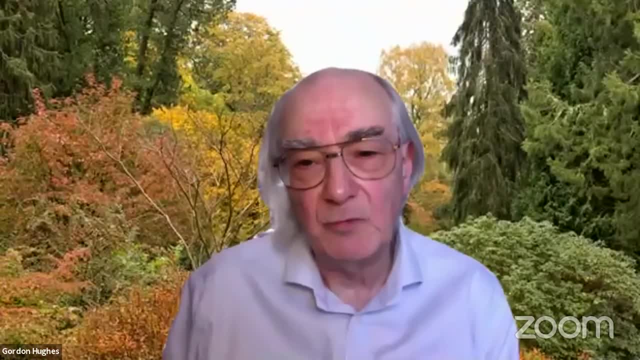 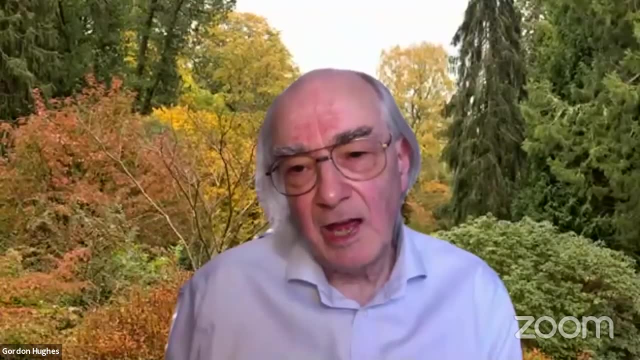 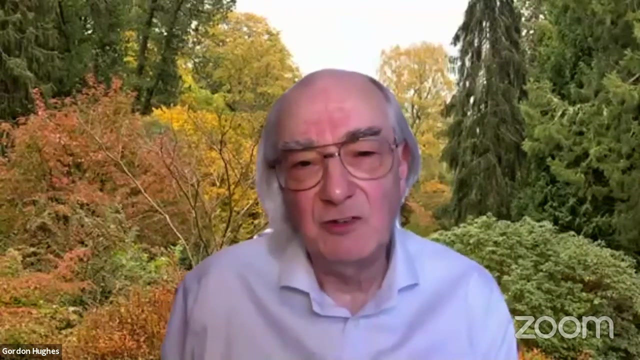 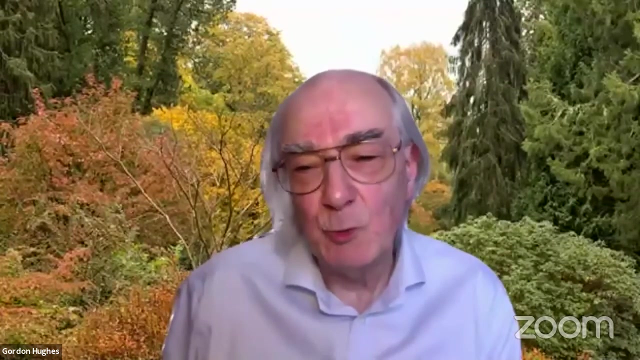 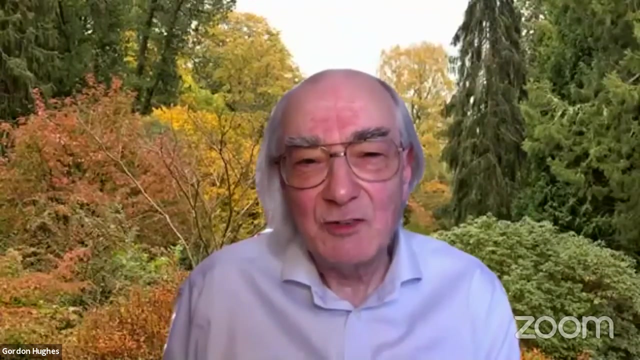 was responding to what they saw as their problems, and I think that's a very important thing, and I think it is also to be than the piedующ or the 15 00, to some extent is klima as well. well, One of the things about history is that the advisor to the king is an easy target to be. 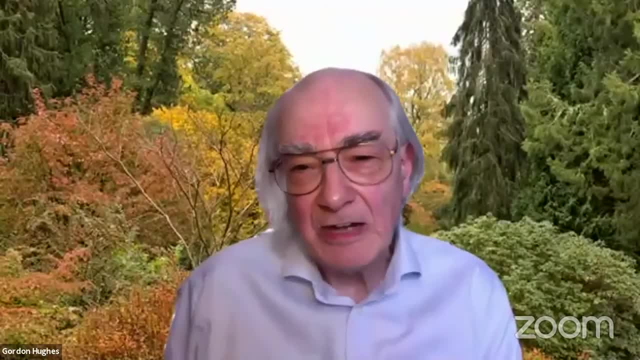 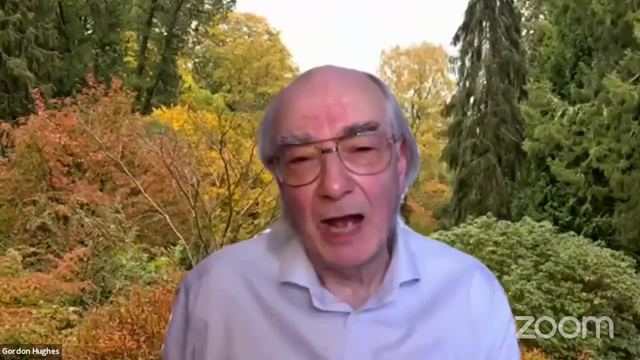 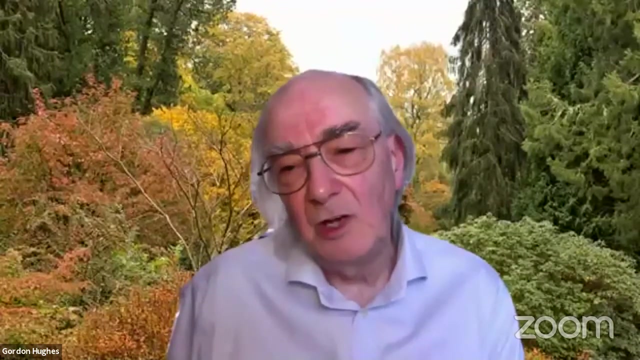 blamed for things going wrong, And so eventually, sooner or later, any advisor is either kicked out or pulls out of his or her own volition. Now there are a variety of things that come out of that, which is trust, and then subsequently, honesty, are key qualities that there must be. 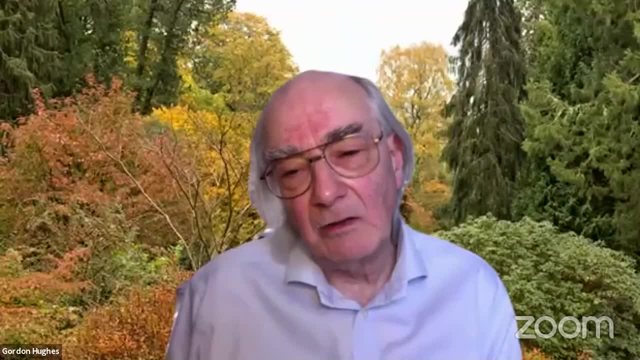 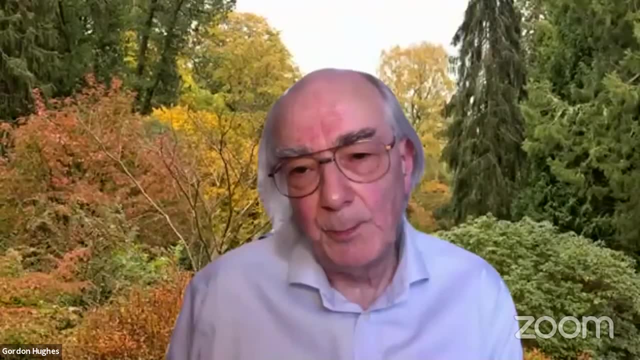 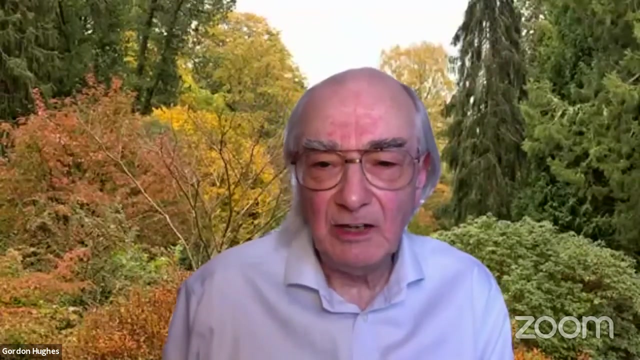 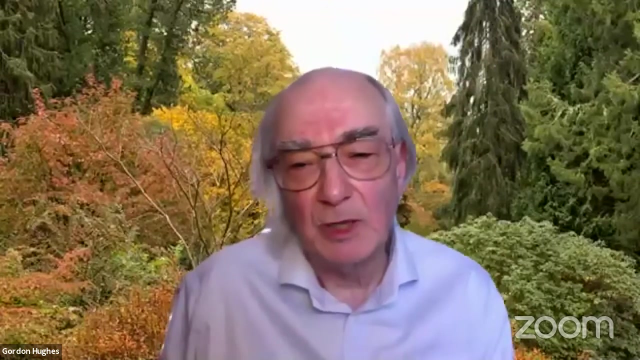 in any advisory relationship And an advisor who is constructing models has got to basically think about the person he is working with rather than thinking about the academic kudos and all of the other things which may have influence. I think there is a lot of evidence starting on that line of work initially. Actually, it is a reality which is that there is no academic rewards from getting involved in modeling for policy purposes. 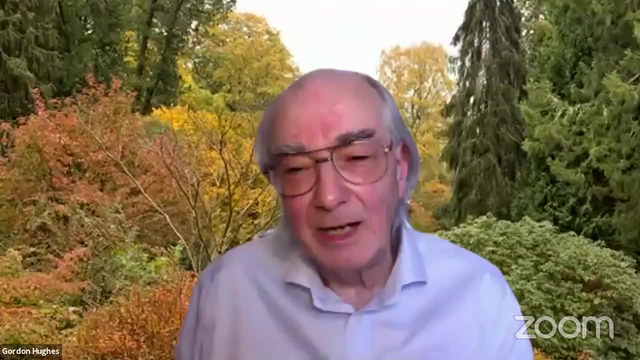 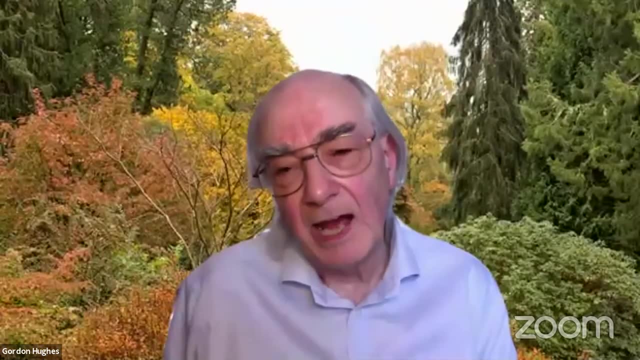 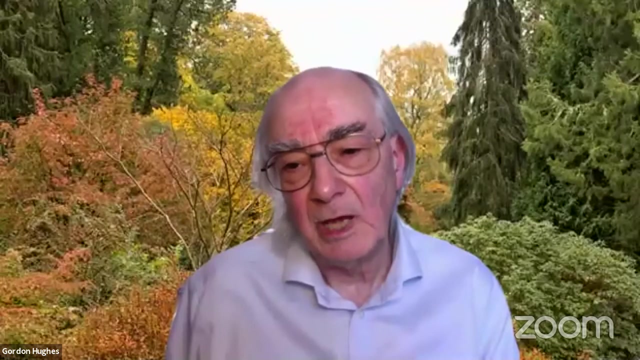 The only thing you get are brickbats and very, very little academic recognition. And those people who see that their modeling work is primarily academically oriented rather than primarily oriented for advisory purposes typically distort their models to meet the requirements of an academic community rather than to meet the needs of the people who are. 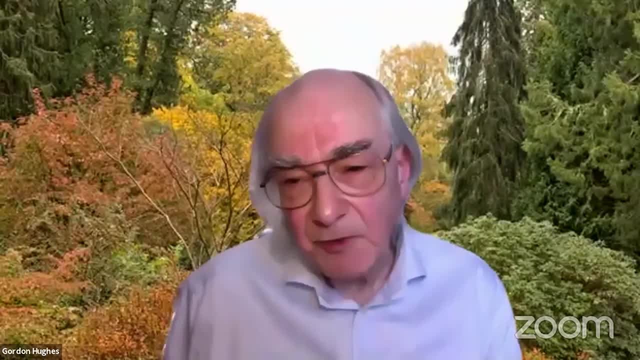 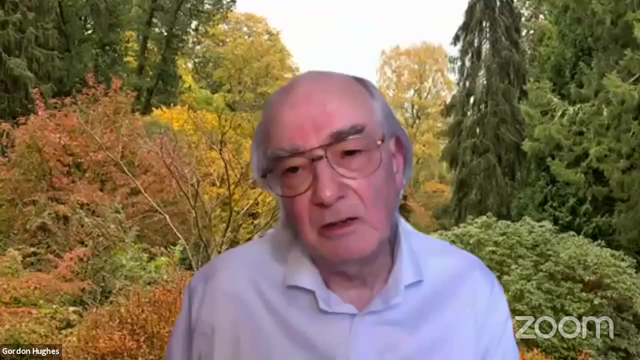 being advised. Now, if you understand that, the next thing is: well, why have models at all? And Chris has in part provided an explanation. Models, mathematical models, all kinds, are cartoons. they are highly simplified representations of particular features that the advisor, the modeler, thinks is important to answer problems which he or she has been presented with. 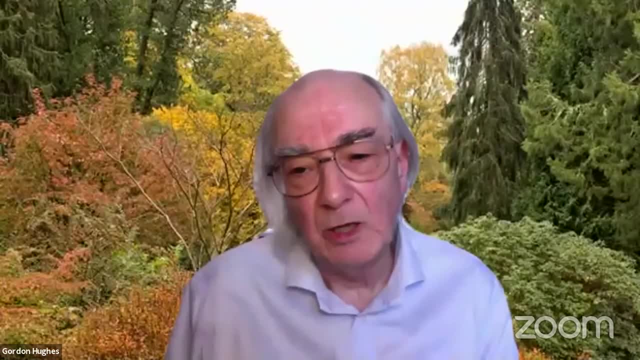 they are not an attempt to describe the whole world, because the whole world, well, the only model of the world is the world itself. so, essentially, your choice is: what is it that you choose to focus on? What are the issues that you see as being important? and then, what can we? 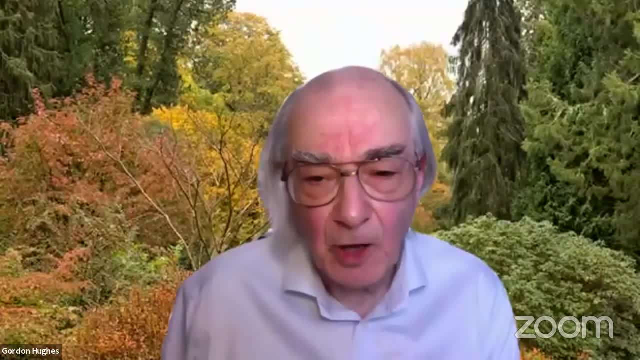 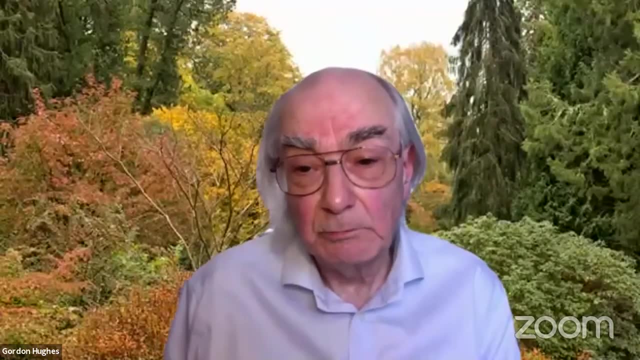 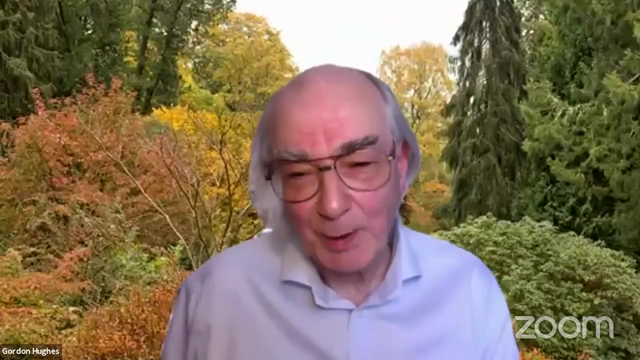 learn from those issues. The follow-on from that is therefore: how do you test whether your models are any good? How do we learn what are good cartoons and what are gross misrepresentations that we're interested in? and the answer is that we do have to test our models against. 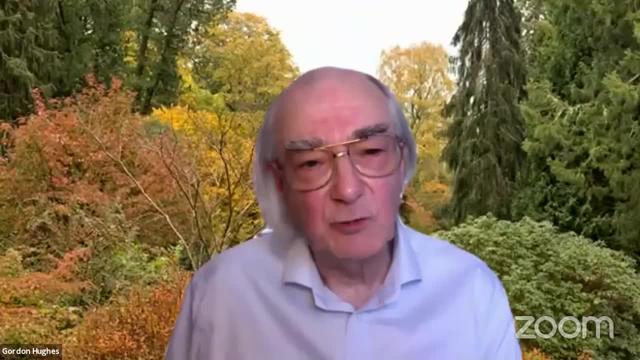 what are the issues that we see as being important, and then, what can we learn from those issues? reality, in some ways- and forecasting is one of those ways of doing it, but also ways of doing it are, you know whether the inputs appear to be sensible and valid and whether the intuitions? 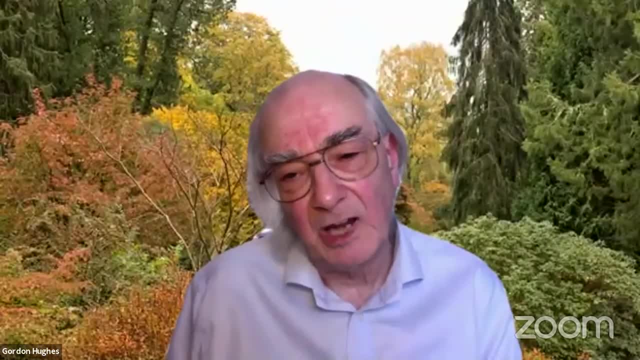 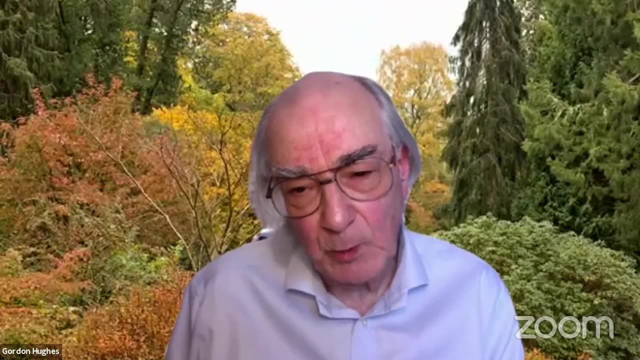 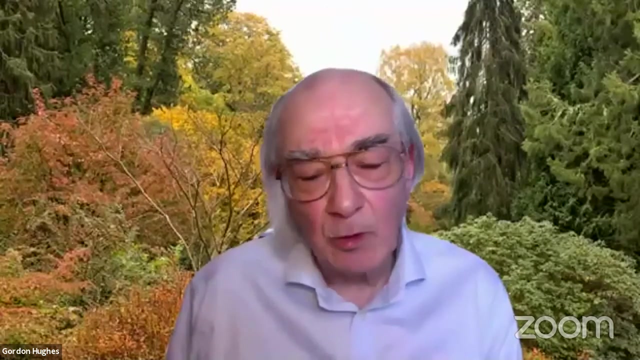 make sense in terms of a broader understanding of the systems that you're trying to model. Now, when we talk about models in the way that we are here, we must bear in mind that all of us have representations of reality. All of us have ideas about what affects what and how and by how. 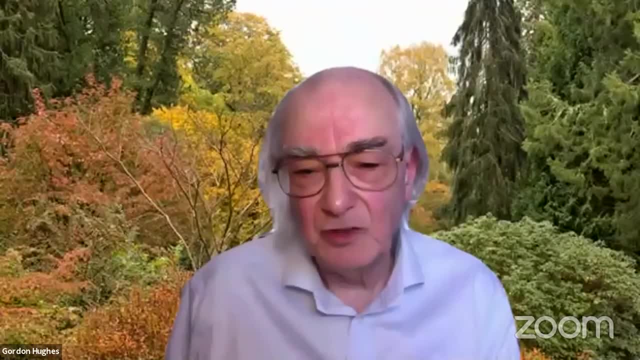 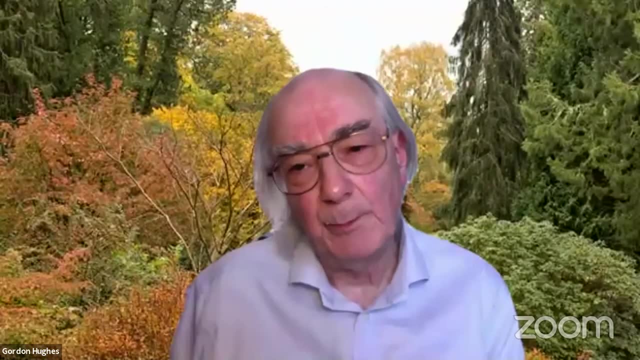 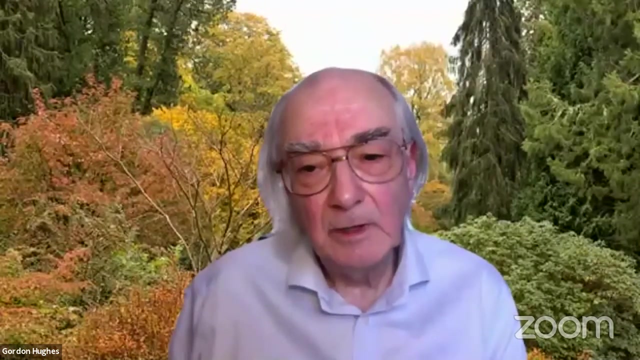 much. The only advantage- and it's a big advantage- of doing it by mathematical mechanisms is essentially by introducing two things: One, rigor, so that you don't believe things which essentially are not true, And the other thing is that you don't believe things which essentially are not true. 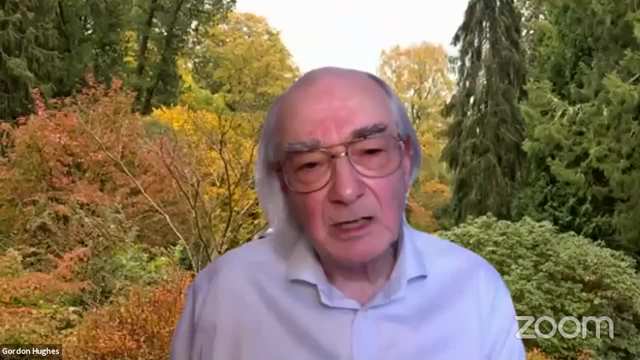 Don't follow logically one from the other. And secondly, to introduce what are often constraints, for example that certain things have to add up, that there are certain laws, whether it be of economics or physics or whatever else, that can't be departed from. So there's no such thing as a 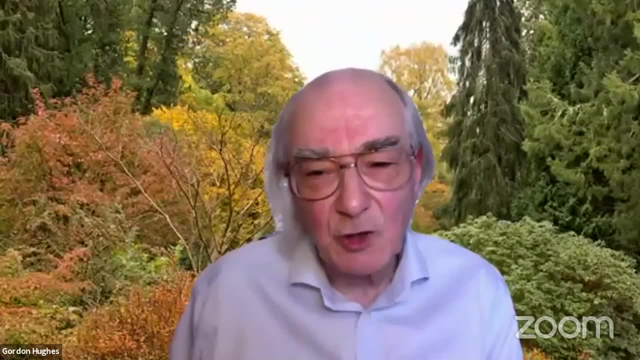 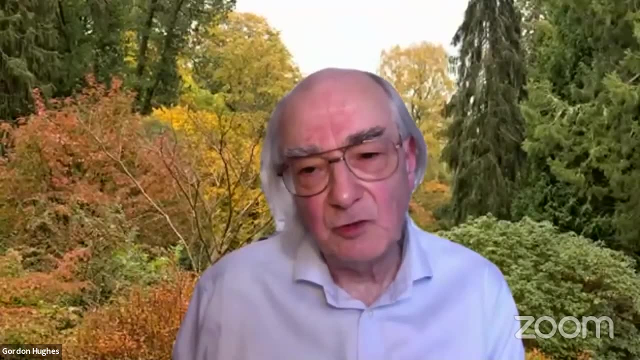 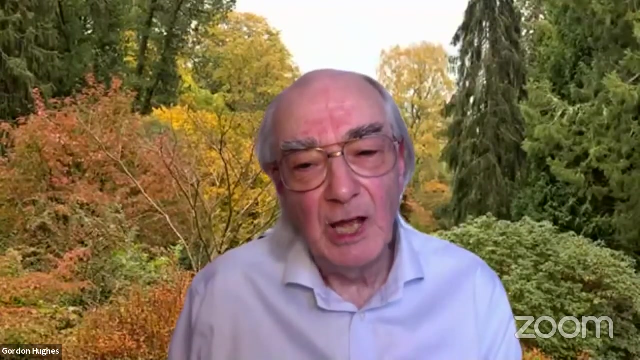 perpetual motion machine, And introducing those two requirements actually constrains what models can do and it constrains the kind of outputs that can produce. Chris referred to exponential growth and the point that exponential growth almost never, indeed never, continues indefinitely. Well, the reason is that they run into constraints of one. 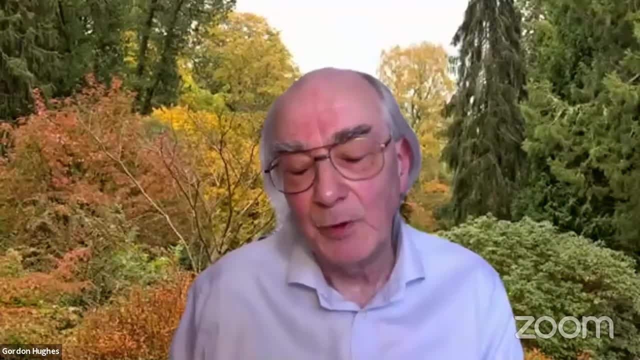 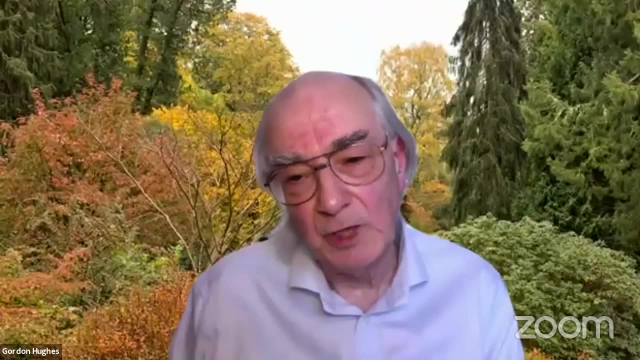 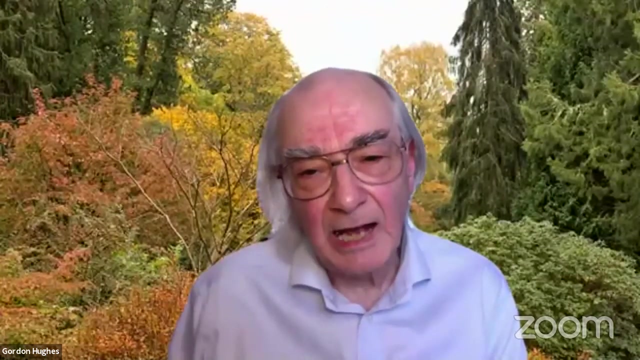 kind or another, and it's essentially picking up that kind of constraint. that is part of what a good model does for you. But then the other thing is: what about the forecasting side of it? And here I'd like to draw on a view. 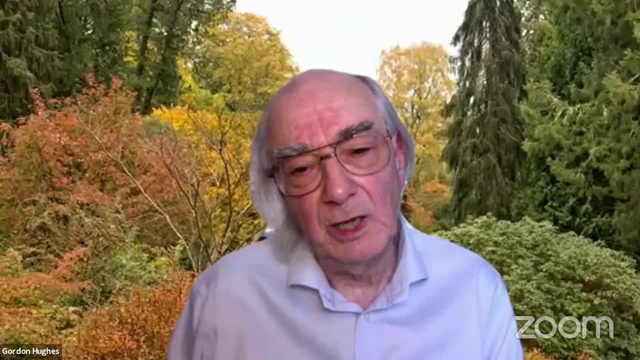 where there was a radical change in economics during the second half of the 20th century. Originally, economists thought that by building more and more elaborate models of the economy we could produce better and better forecasts of what was going to happen in future. 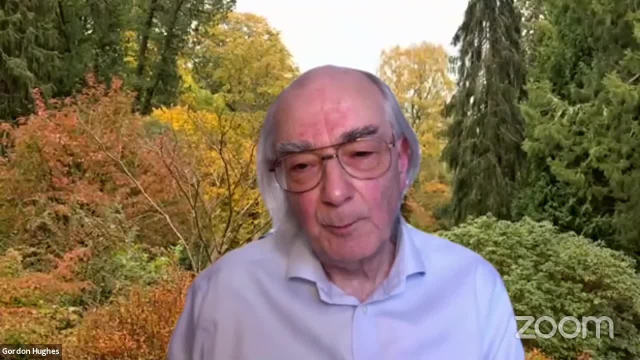 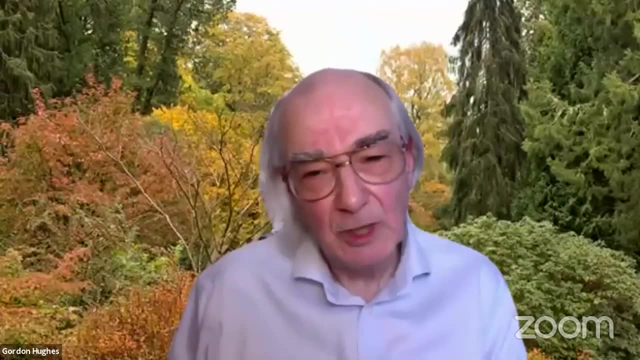 So essentially, the idea was: let's build everything in, and we're going to build everything in. let's disaggregate, let's make them bigger and more complicated, and surely the resulting forecasts will get better. They got worse, They got worse because essentially nobody could. 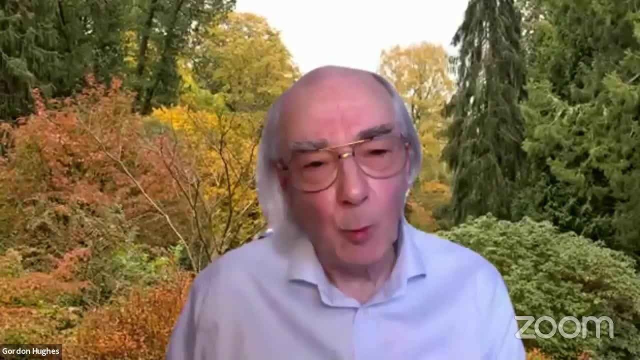 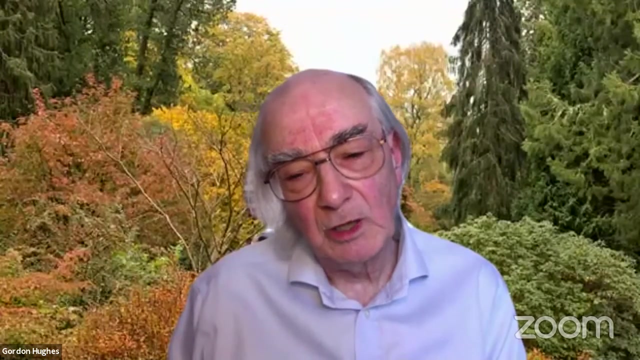 understand really what was going on in the model, and also because they became increasingly incapable of taking account of the inherently random nature of an awful lot of what was going on. So then what? So what the modelers learned in economics was to ask the question: does my model do any better than? 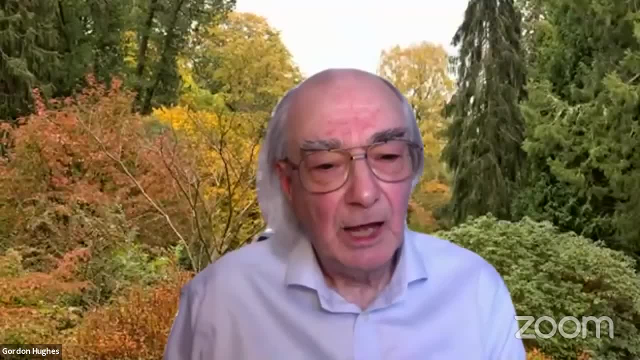 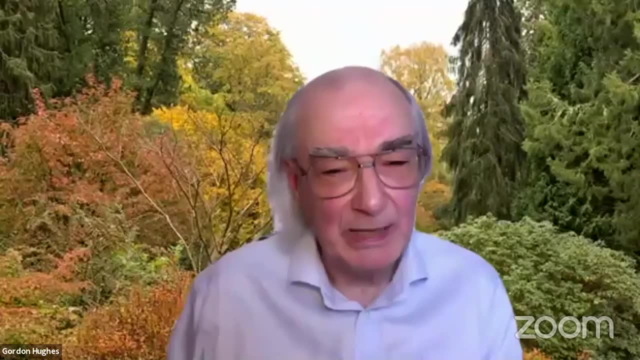 some very naive and very simple model. One of the most naive ones is: next year is going to be like this year, or next year's growth is going to be like this year's growth, And essentially those are in the jargon, time series, models of a very simple kind. And the question is, do they do any? 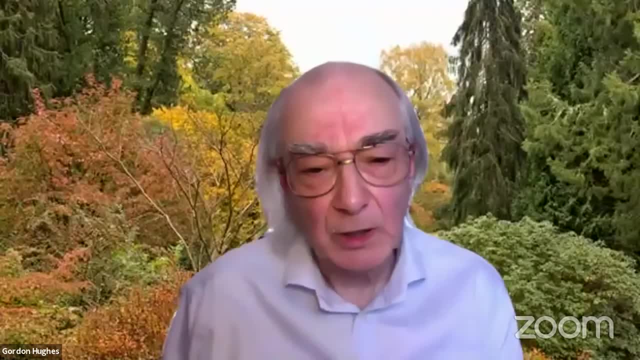 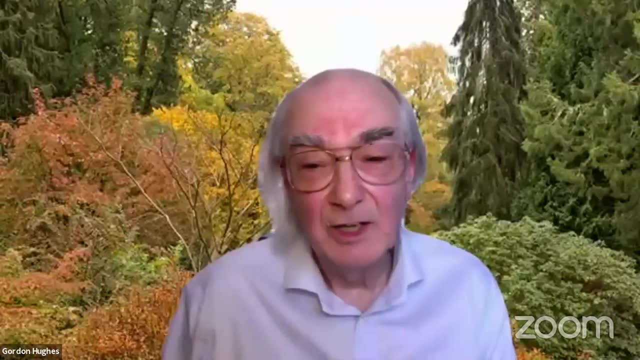 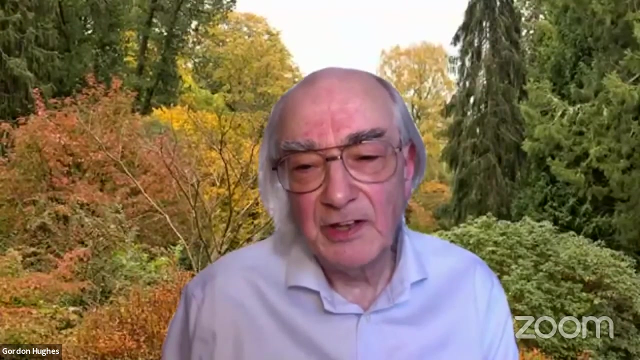 better than I'm sorry. Does your model do any better than a very simple naive model? The answer that economists found mostly was no, they didn't. Now, one of the standard thing against economic models was they never predict the next recession. That's actually unfair. In some cases they predicted. 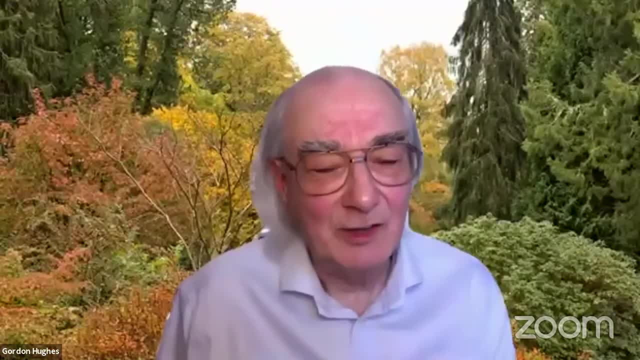 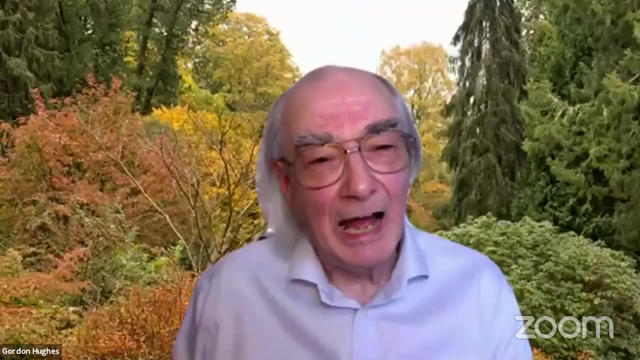 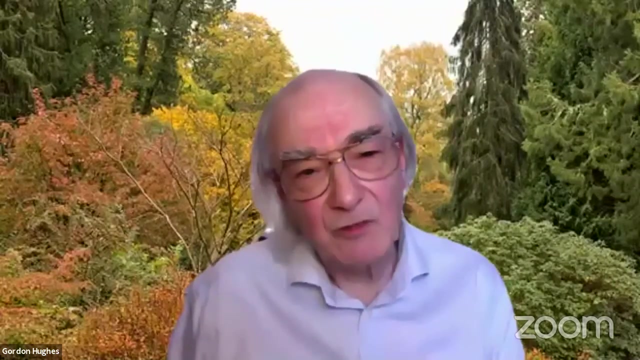 far too many of the next recessions. The classic joke is that they predicted 15 of the last five recessions And they were too sensitive and they were too prone to tip over in a way that led to a recession. The problem is, there's a very fine line- And that's, in a sense, Chris's fine line- about chaos. 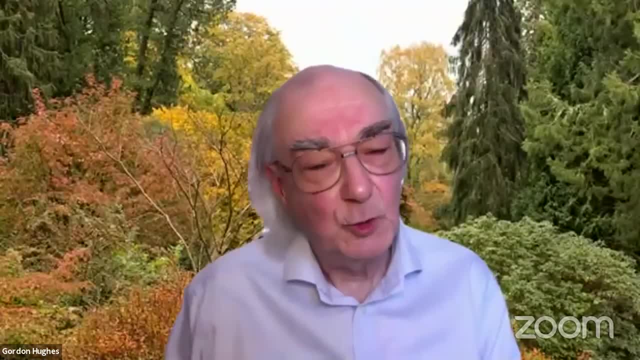 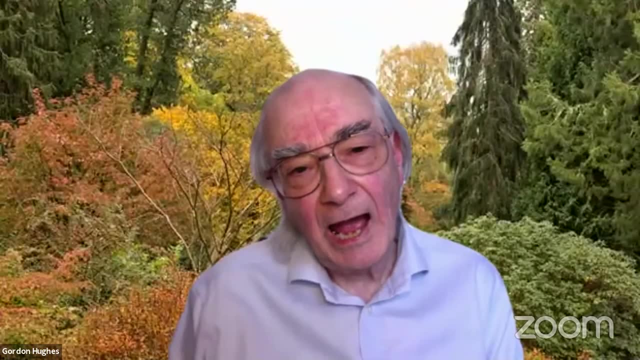 where something is stable, too stable and then too unstable in terms of the way in which it behaves. And all of that is telling us that as we get more and more complicated in the way we try and model, the less we understand about what it is that's going on and how it's going to change. 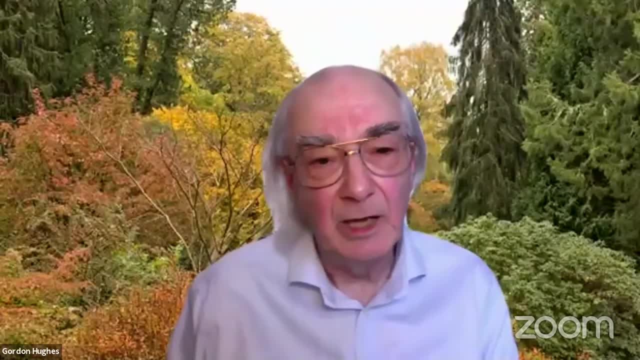 the less we understand about what it is that's going on and what's going to happen. And then this is going to be a very, very complex model because we're going to be looking at things that are going really driving the key things that we're interested in. So, ultimately, when modelers 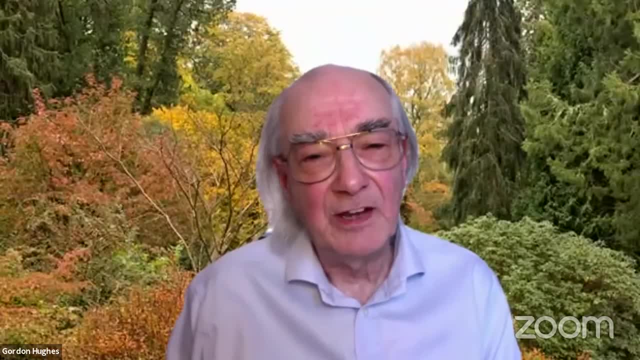 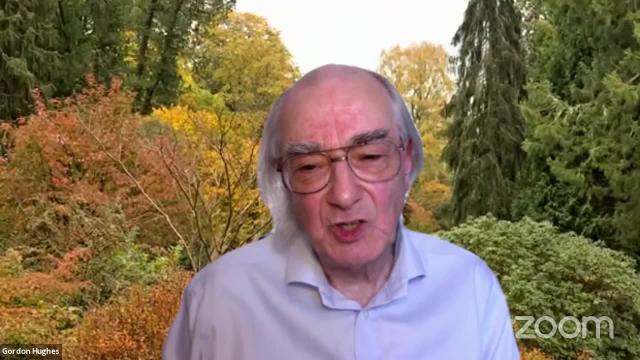 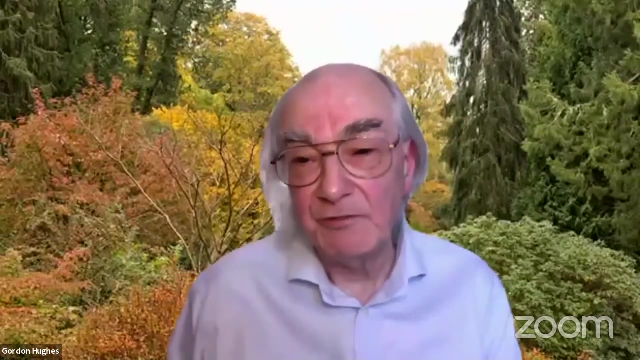 constructed those kinds of models. they looked at them and they said: do we believe it? And in effect, what they were doing was saying: actually, does my intuition, my experience tell me that these results are plausible? To what extent are they plausible, Or do I have to modify it? And 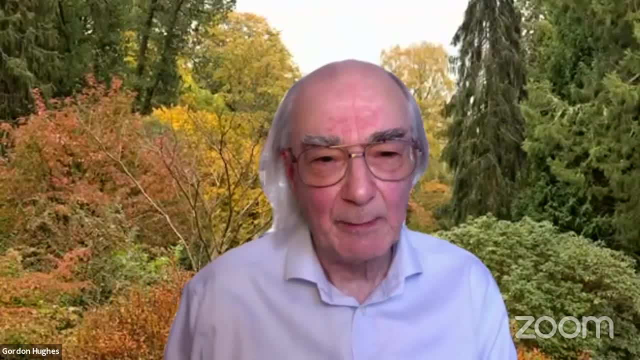 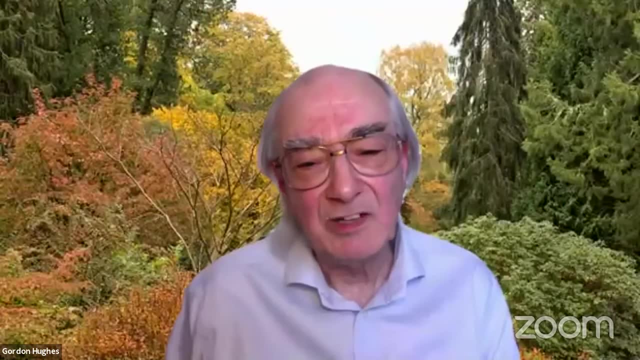 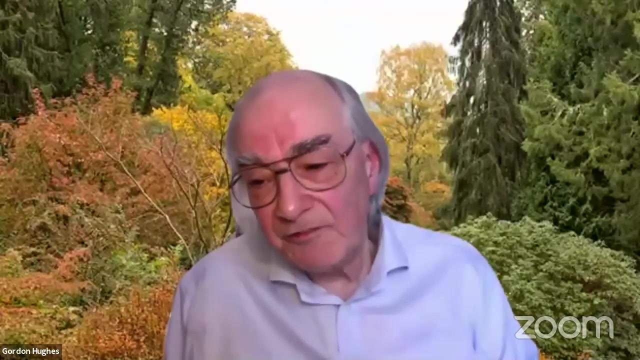 what they would typically do if they didn't believe it. they'd go back and change the parameters in some kind of way. Well, that's not really modeling, That's just essentially fitting a mathematical framework to comply with your prior assumptions. Now, the final thing that I 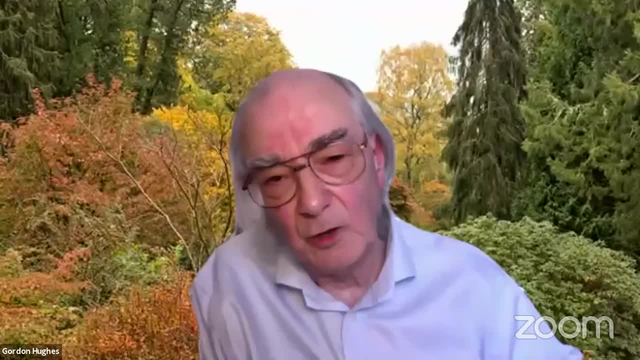 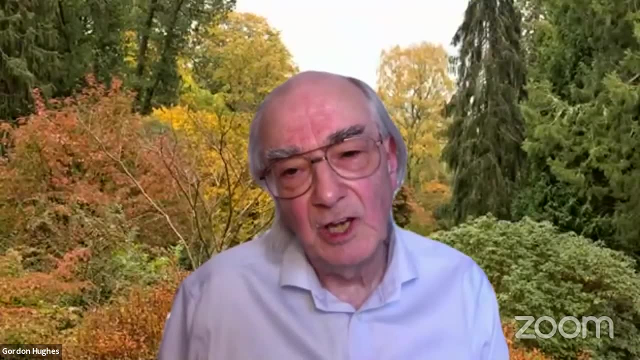 want to bring in, because it's very important in the current context, is about risk, Because one of the things that good modeling can do for us is actually provide a framework for analyzing risk, A distribution of outcomes rather than a certain outcome. Now let's take a particular example. 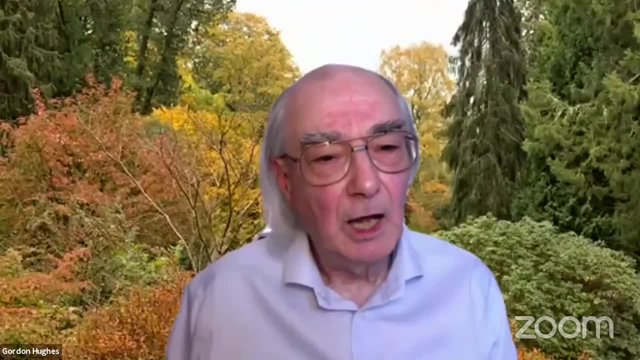 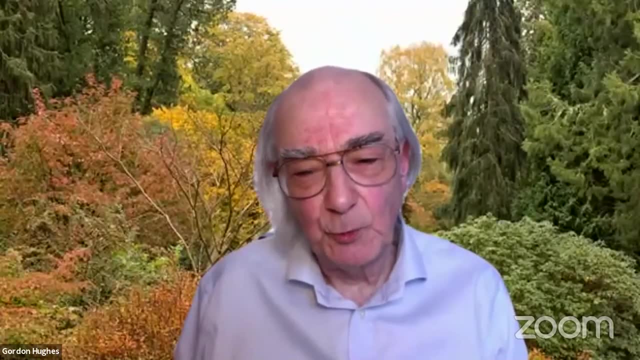 which is widely quoted. The WHO has people who are widely quoted as saying that there is a risk that changing lockdown policies will lead to a second wave of infections and more deaths and so forth. Well, from one point of view, that's an utterly trivial statement. 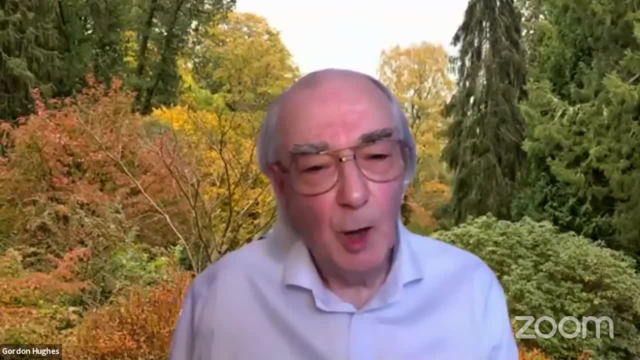 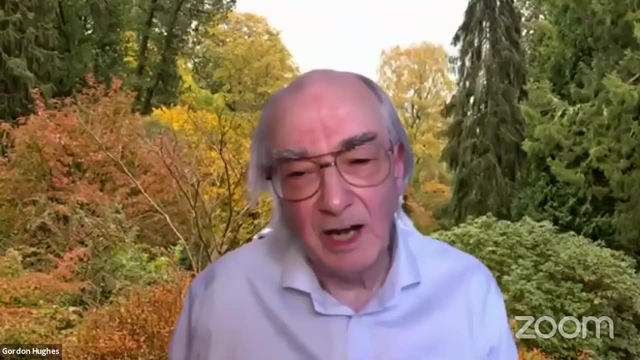 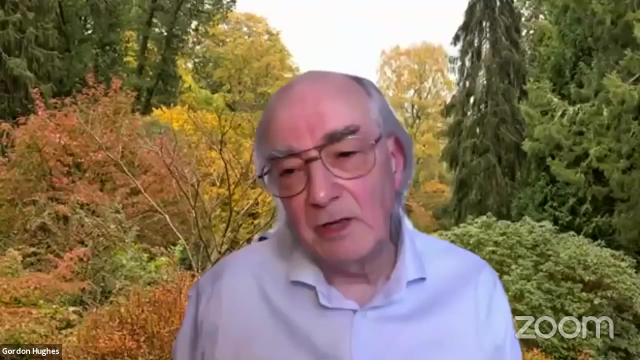 Of course, there's a risk that that might be the case. What matters is whether that risk is one in a hundred or whether it's 25 or 50 in a hundred. In other words, it's not a general statement that something is possible. Rather, it is a statement about probabilities of some kind that matter. 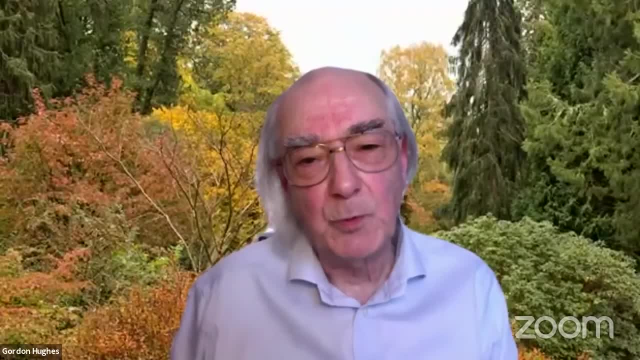 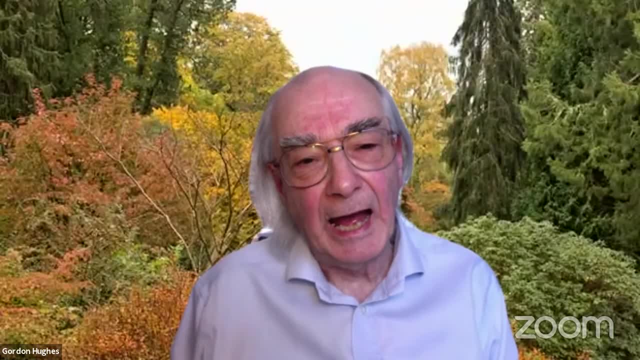 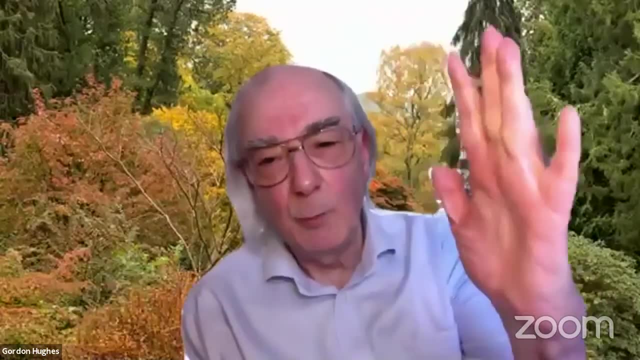 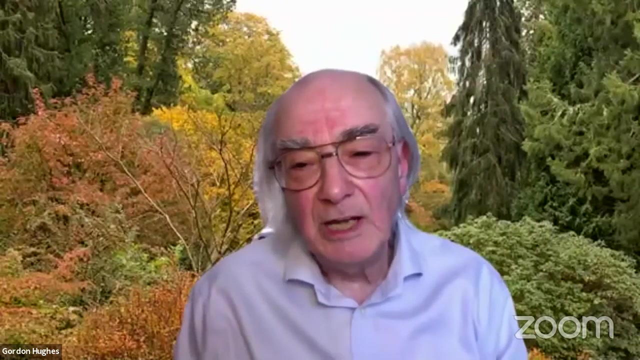 And you finish up with a distribution of outcomes, And the Bank of England does that. when it makes an inflation forecast, It produces what's called a fan diagram, which is essentially a range of increasingly improbable outcomes around a central point in terms of the way in which it thinks that. 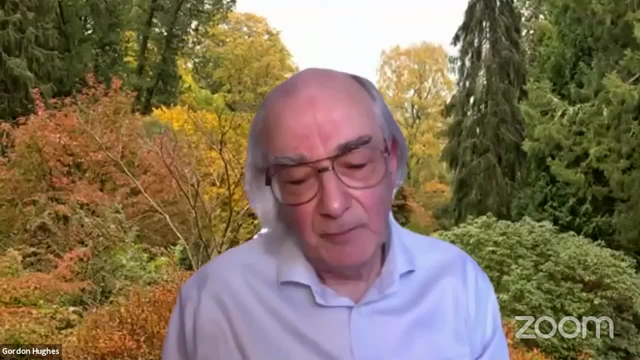 inflation is going to behave over the next year, five years, whatever it may be. Now, that kind of quantification may be a little bit more complicated than what we're used to, But it's a little bit more complicated than what we're used to. But it's a little bit more complicated than what we're used to. But 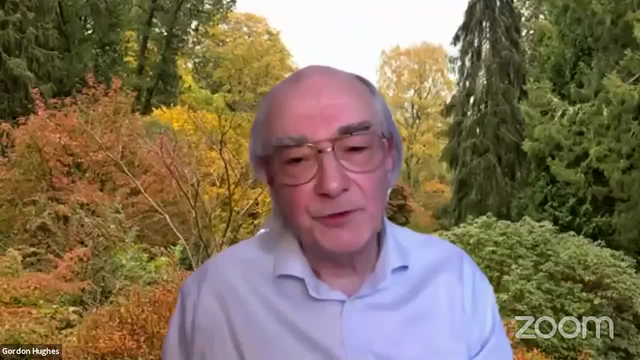 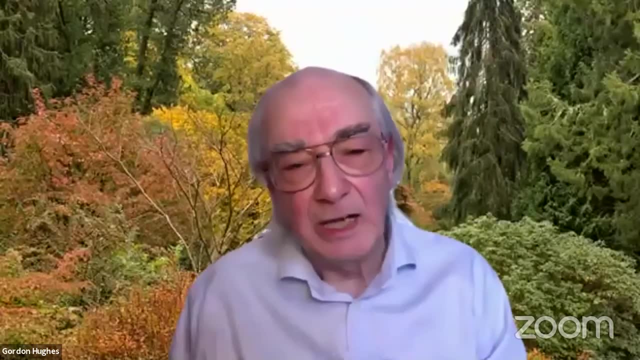 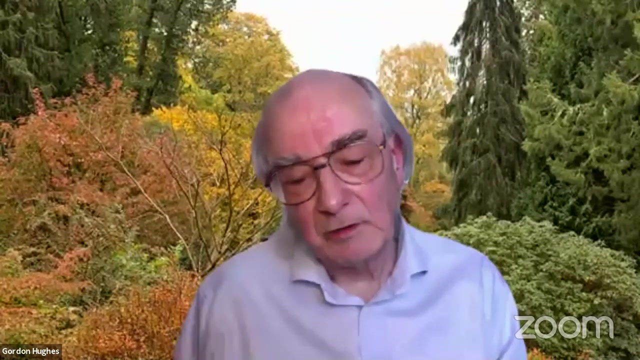 it's a little bit more complicated than what we're used to, But, on the other hand, it's important because it's saying what are the probabilities that are governing the choices that we may need to make as a policymaker. Now, this is very important, coming to the current crisis, because 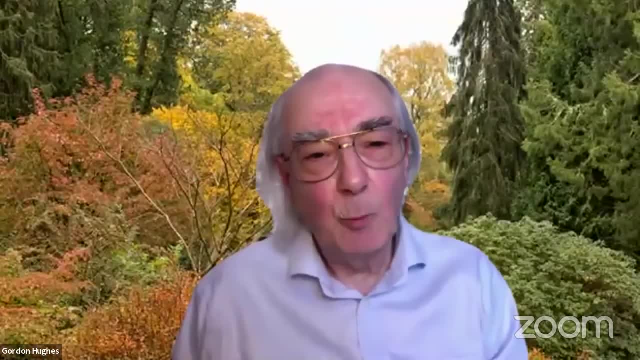 we are told that one of the things that happened was that a particular story was put around that if the policies weren't done, we wouldn't be able to do anything, And so it's a little bit more complicated than what we're used to. But, on the other hand, it's a little bit more complicated than what we're used to. But 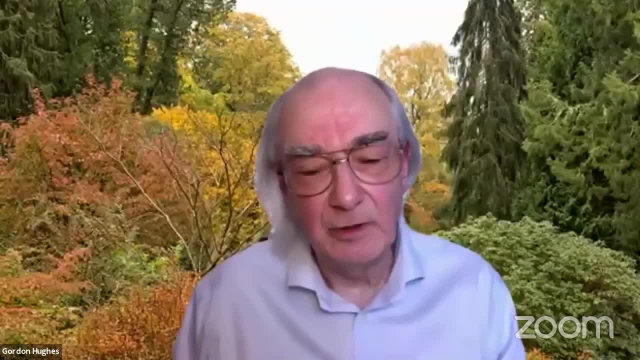 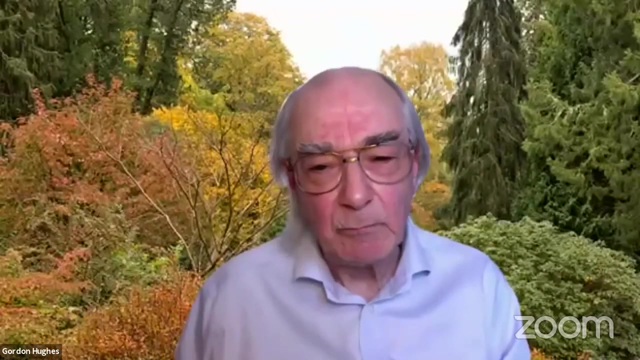 changed, there would be 250,000 deaths. Now, that wasn't the central forecast of the model. That was a worst-case scenario. Nobody is too clear about how it was derived, But the point was that it became the focus, almost as though this is what is going to happen if we don't actually change the 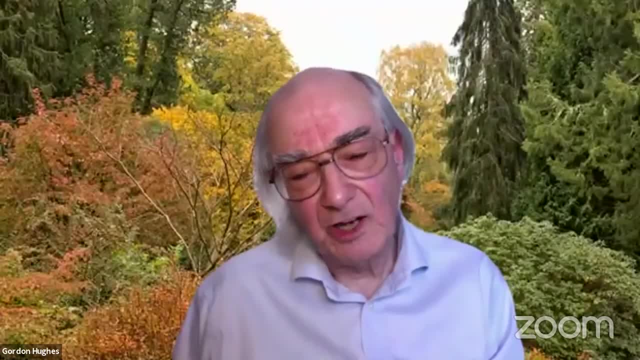 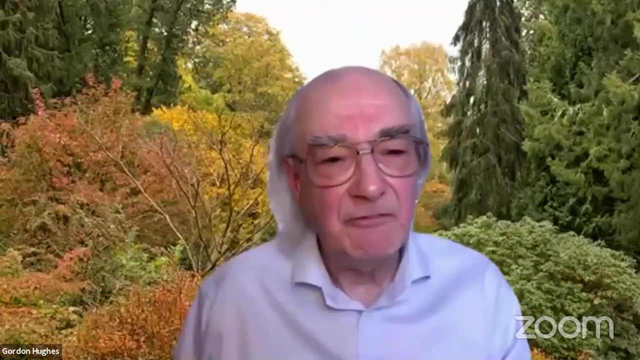 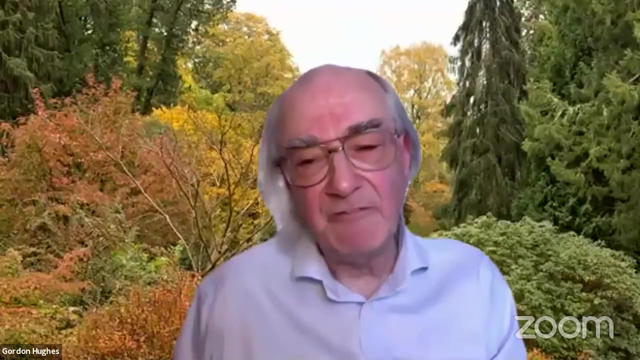 direction of policy That illustrated two important things, Which is one that we live in a society which is very, very naive and ignorant about probabilities, And that causes enormous problems because it very easily leads to either a concentration on this kind of extreme outcome, in other words, one worst case, or it leads to. 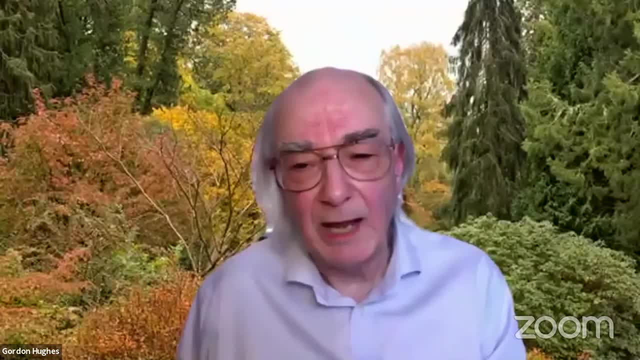 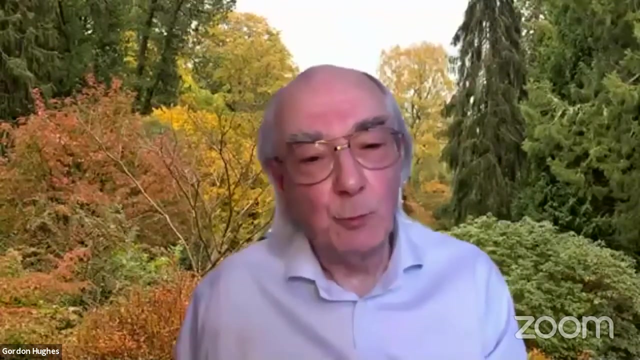 people, just ignoring the distribution of possible outcomes. So, for example, in Britain we have an example of costs that were put on building a high-speed railway which everybody knew, based on experience, were almost certain to be wrong. The range of costs was probably very large. 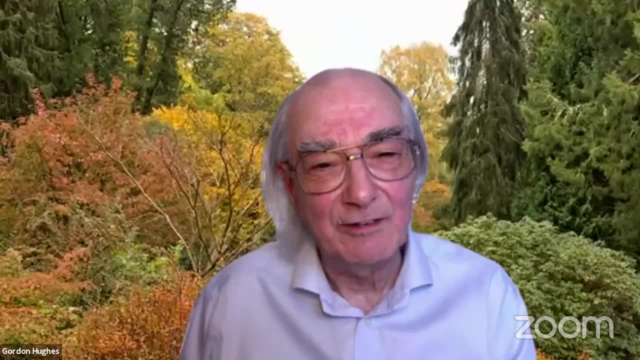 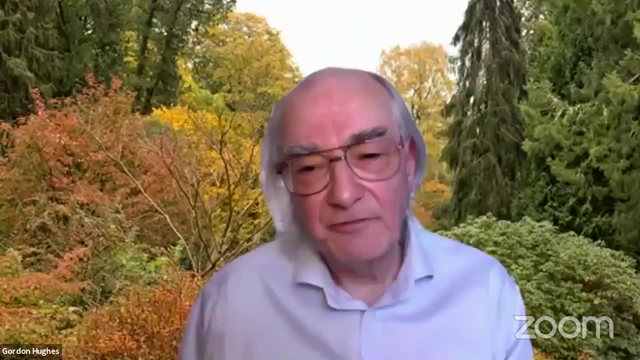 and has subsequently been tripled since the original figures were put around. There was a case where people took the original numbers and ignored the fact that there was a large range around those numbers And actually that range was an upward range, not an upward range. So it was an upward range And actually that range was an upward range, not. 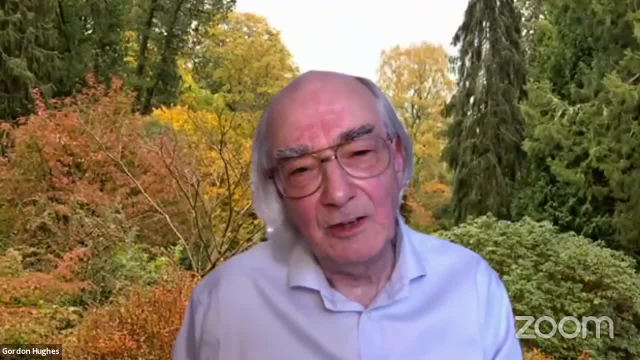 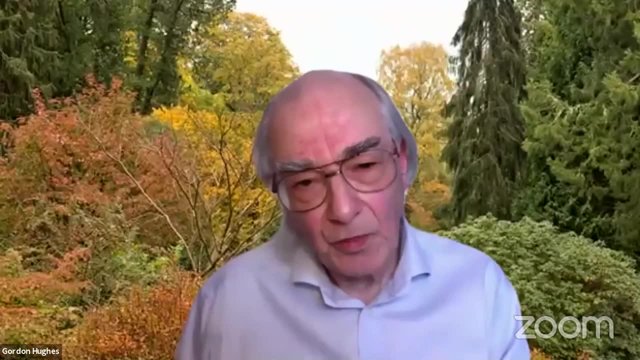 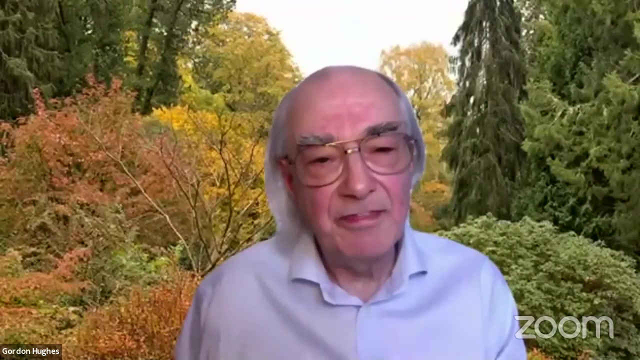 an upward range. They were never going to be less than that. It was likely to be very much larger than that, And so, from the point of view of giving policy advice, the point that I'm trying to make here is that policy advice, ultimately, is not about there is one right thing to do. 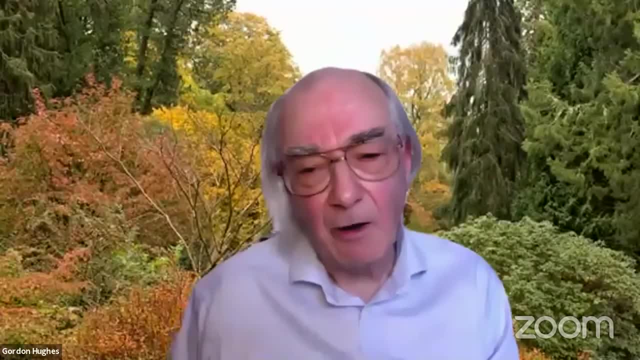 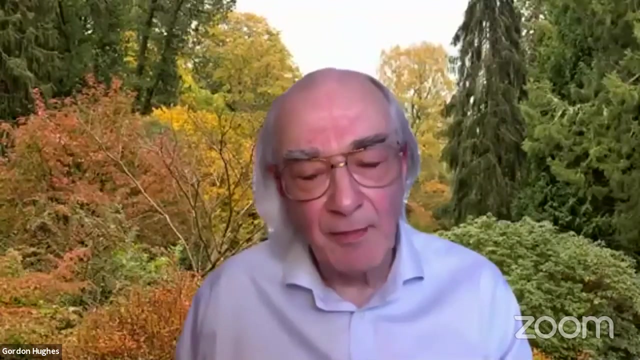 There are a range of model outcomes, There are a range of things that could happen. Many of them are random and we don't fully understand them, And actually what we need to get is not a fixed policy for the next month, three months. 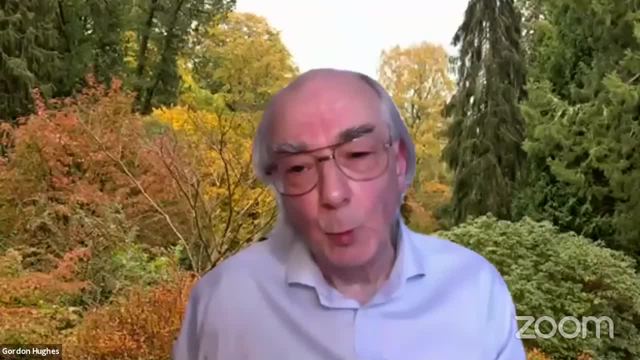 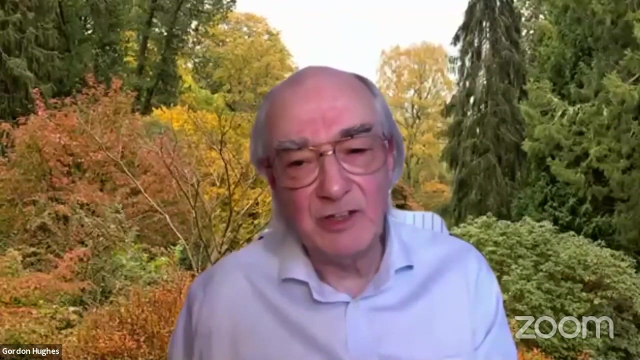 five years, but rather a set of rules by which, as we collect more information, we adjust the policies to take account of the extra information that we get and we build into our policy the collection of the information necessary to inform the improvement of our models and the development of a better idea of the direction of policy. 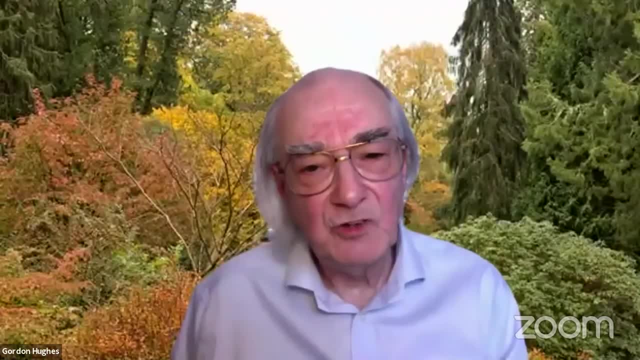 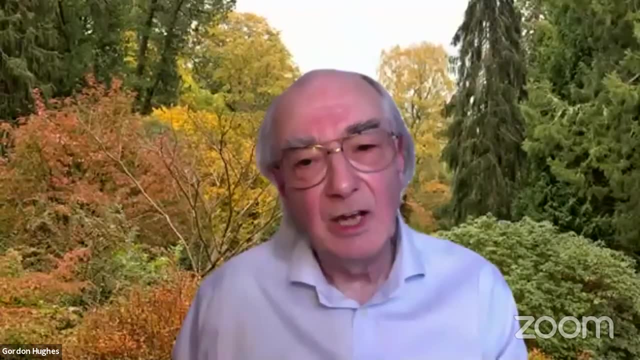 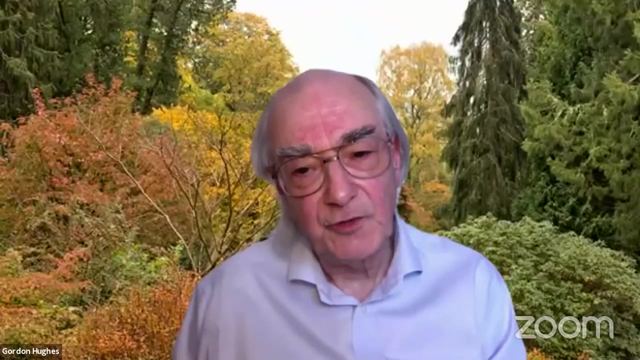 And that is where I'd like to end, which is with respect to the current policies. the big, big mistake that's clearly been made is essentially the failure to systematically appraise, as you go along, the models that have been made that underpin policy, and then to have a feedback. 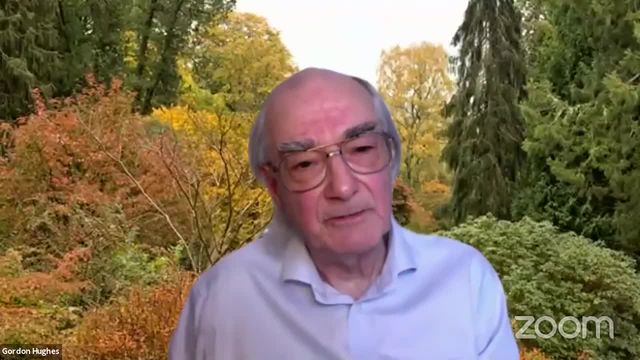 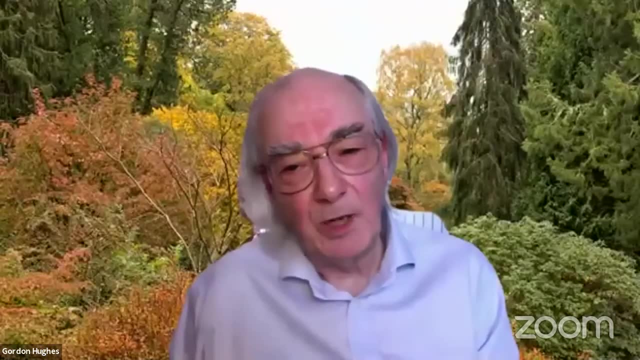 between the construction of those models and the development of the policy, because the two have to go hand in hand. It's not. there is a model and this is what the policy comes out of it. It's a continuous iteration and it is the way you build on that iteration that is crucial. Thank you. 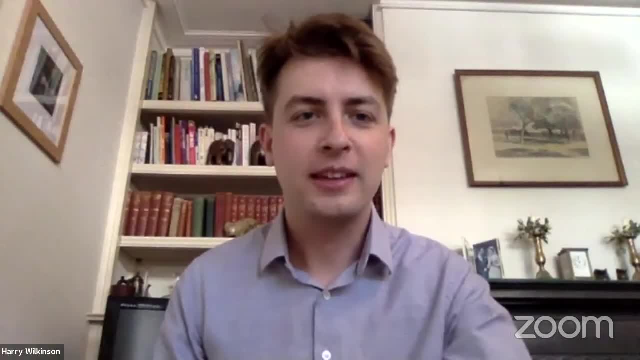 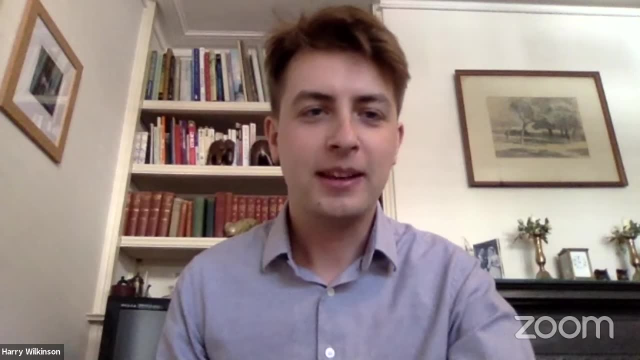 Thank you very much, Gordon. I'm sure there's a lot of things that we will come back to from that when we have the question and answer session later. My next guest is Dr Benny Pizer, who I'm sure many of you will be familiar with. 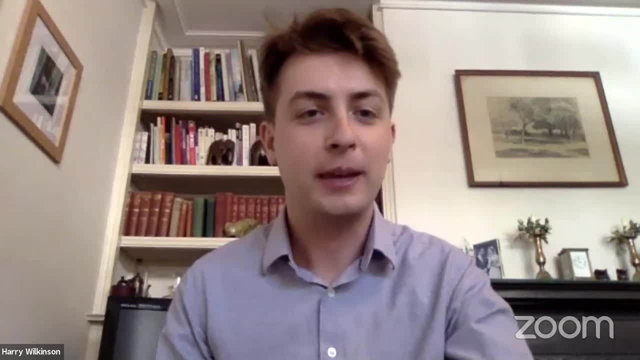 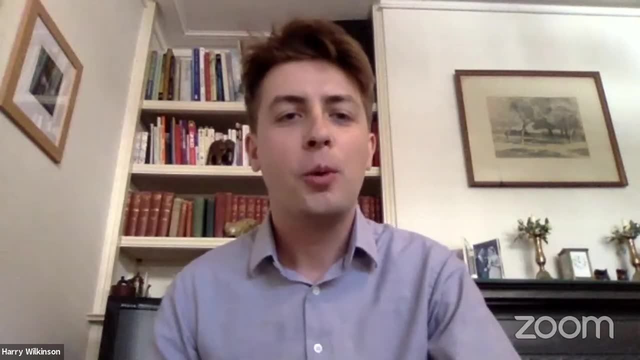 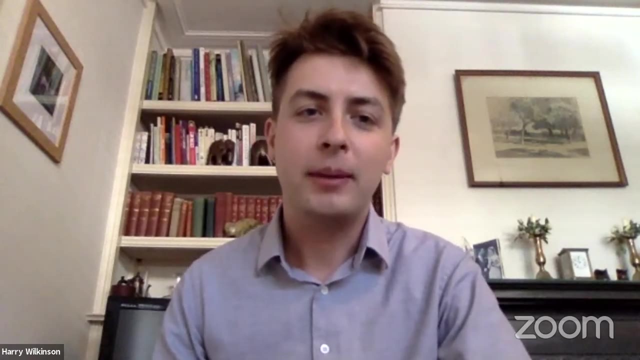 He is my wonderful colleague and director of the GWPF And, of course, one thing I thought would be important to mention was when he set up the CCNet newsletter. it was indeed looking at the public perception of risks and, in particular, asteroids. and then that conversation. 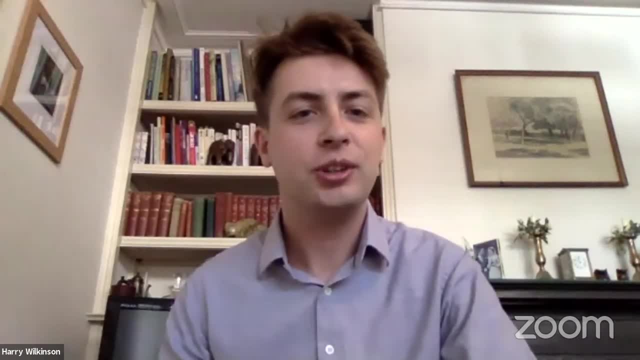 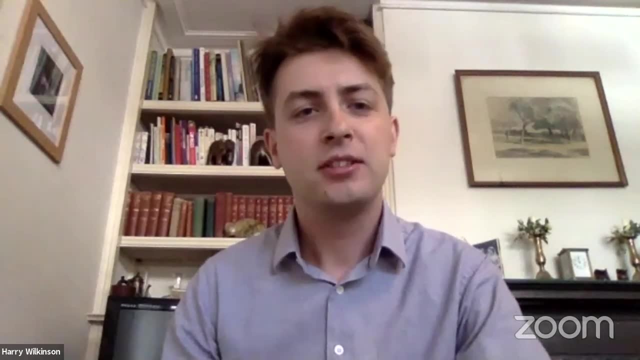 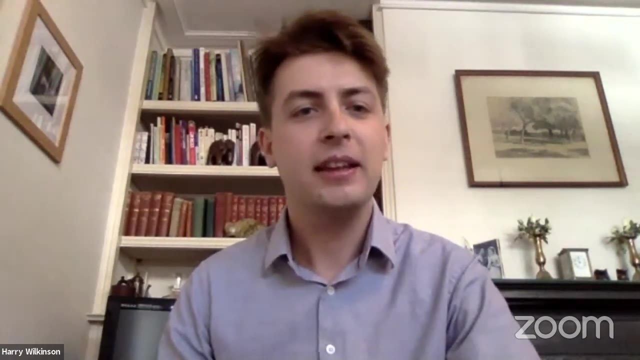 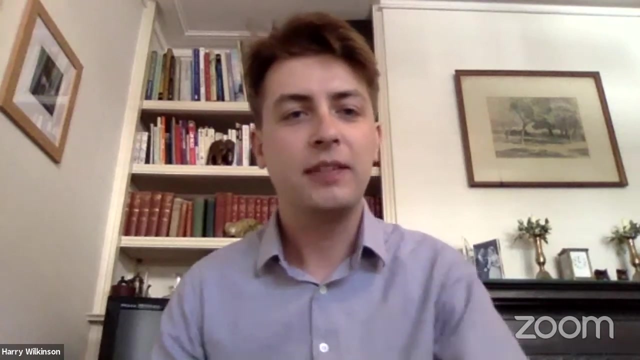 moved on To become about climate change, And now today we have the GWPF newsletter, which is the successor to that. So risk has always been a key element of models and how they interact with public policy, And I thought Benny would be the perfect person to give us now this more political context to how. 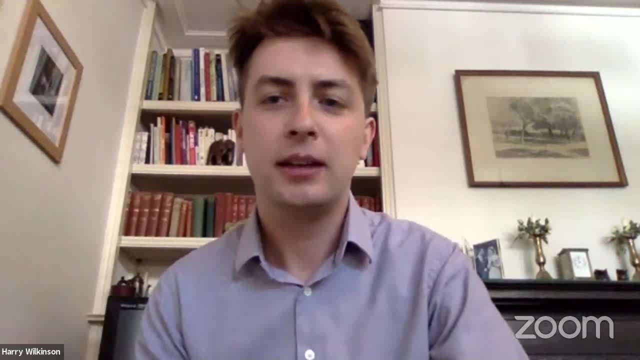 governments around the world and the world as a whole are going to be able to take advantage of this. And this is this broad discussion around the impact of models on climate change. So if you were me, we'd like you to share your thoughts around what the GDP model looks like, and 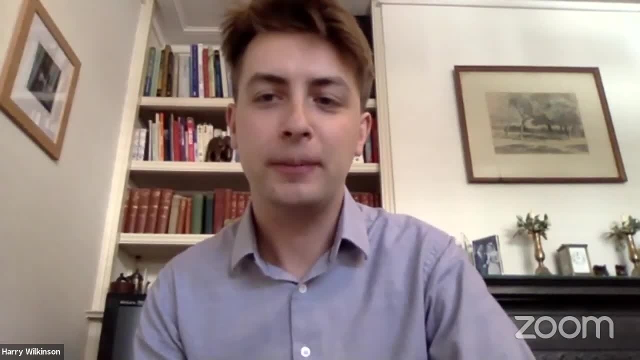 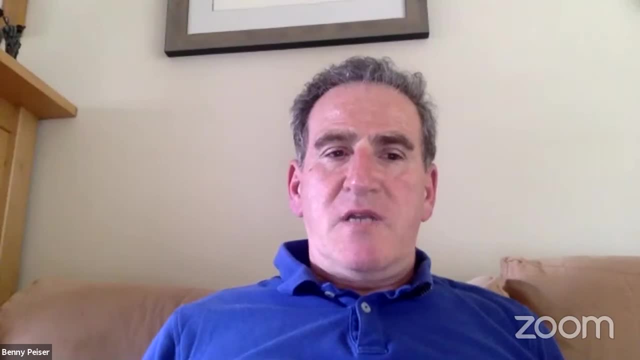 how the grand plan is going to affect climate change at a global and international level. And then we will pop back to Mr Pizer Great. So thank you very much. So, thank you very much, Thank you. So I'd like to just touch on the issue of climate change and what you are saying. 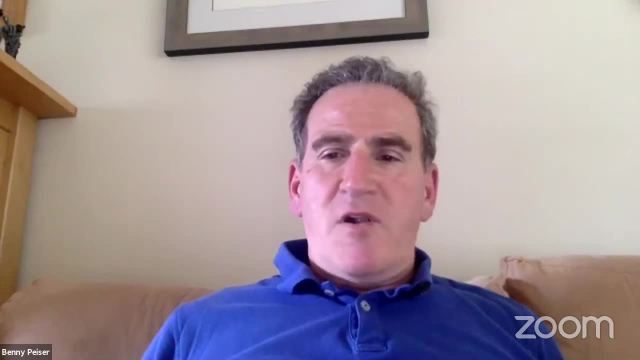 particularly in the context of the climate, Because you're a part of a world that has been really doing the climate change, and the climate change phase of the world have been interacting with models, particularly in climate. Benny over to you. Thanks, Harry. 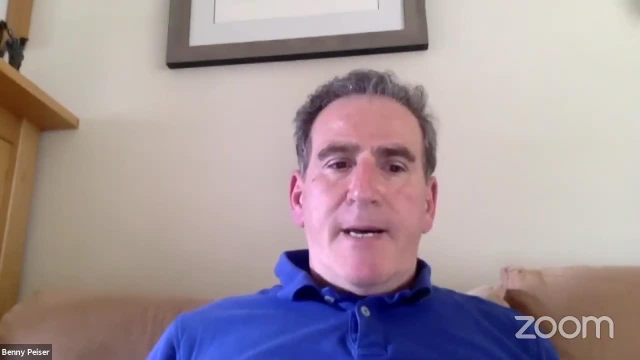 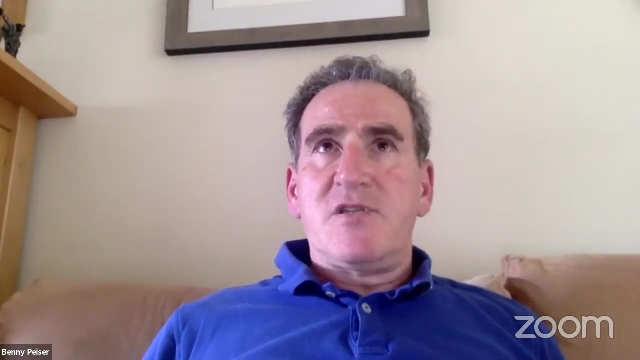 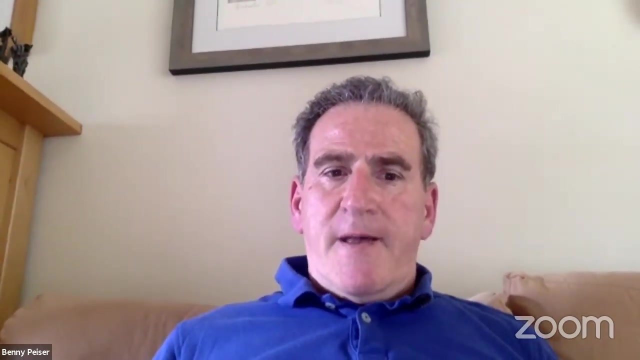 So I don't intend to discuss the COVID-19 models and the discussion about the models was the right decision or not. I also don't want to discuss the failure of some of the models. My main interest today really is in discussing institutional failures- flawed. 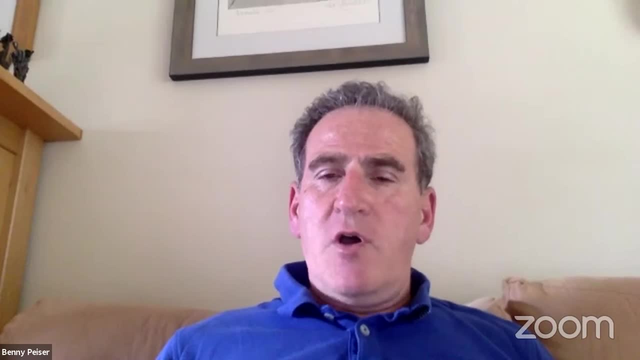 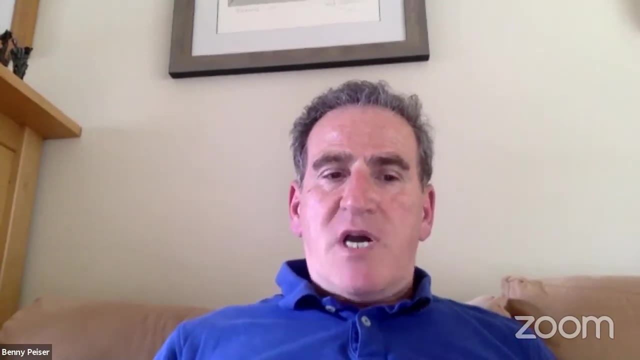 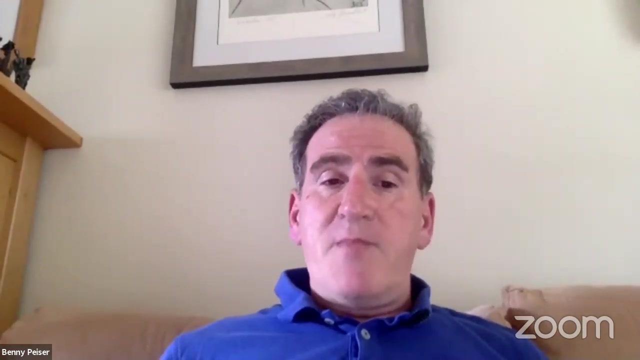 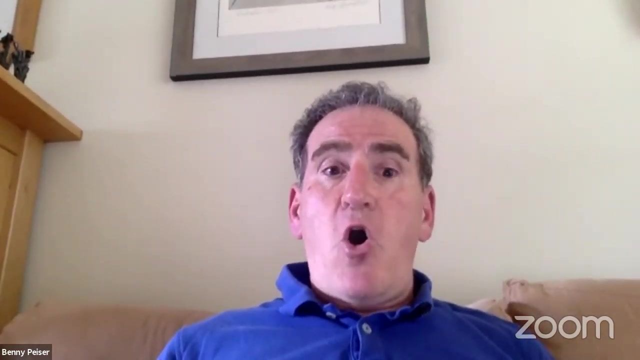 organization and the lack of quality control of scientific government advice and its evident contradictions and shortcomings. We've known for a long time the flaws of environmental and economic and energy modeling. How do we know that? Because there's a long, long track record of failed. 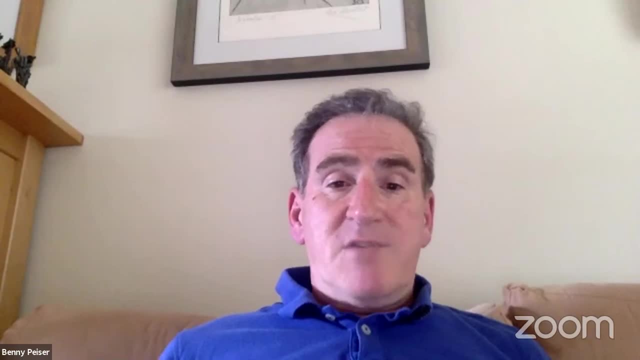 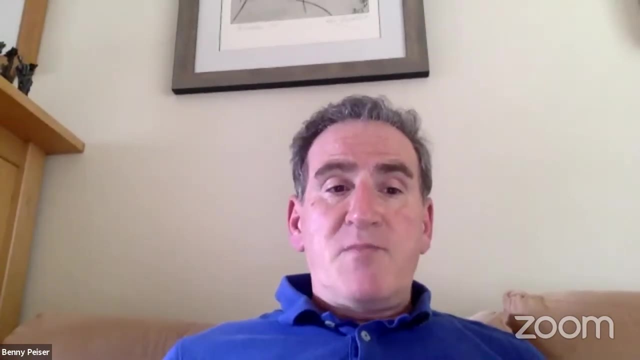 predictions based on flawed modeling. You know the Club of Rome with their doomsday predictions: the failure of the population bomb scare, the peak oil models failing to anticipate the shale revolution, the failure of the economic and statistical risk forecasting models that played quite a significant role in the financial 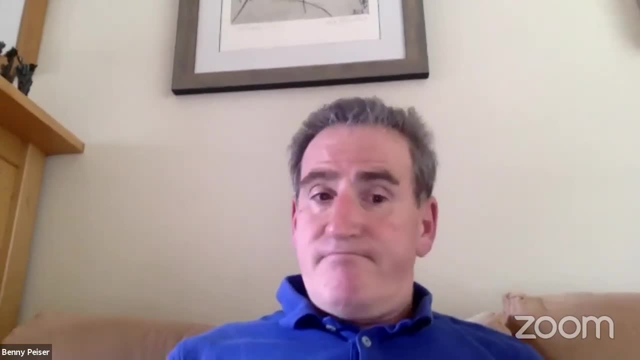 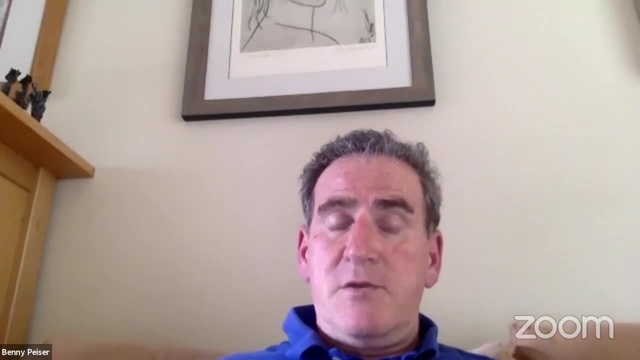 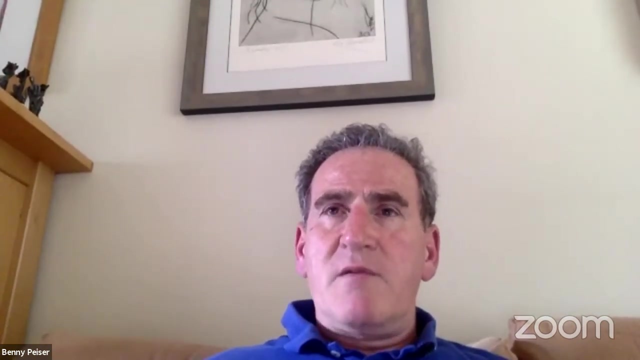 crisis in 2009,. and perhaps, who knows, the perhaps biggest risk modeling failure with the models of, you know, the COVID-19 crisis. When it comes to climate modeling, perhaps the most prominent failure was 30 years ago, when the 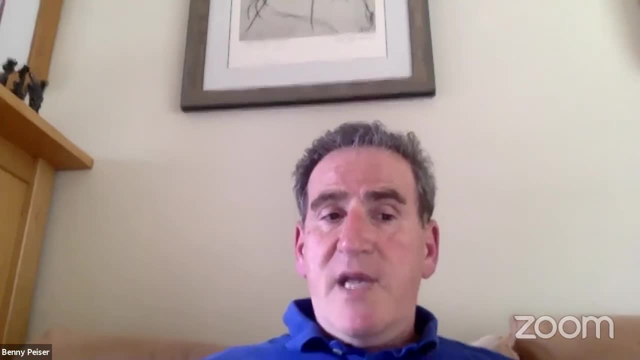 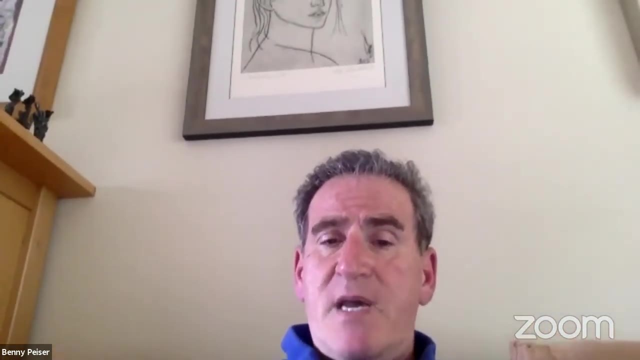 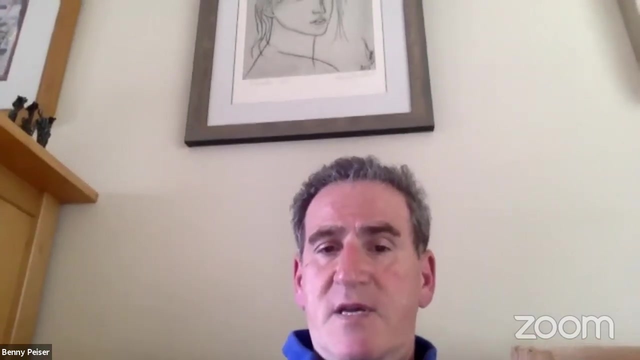 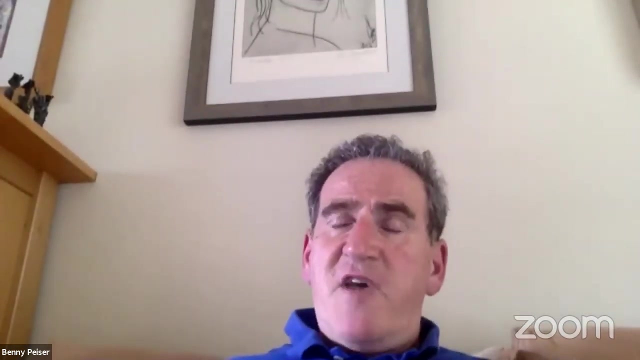 IPCC published its first assessment report and predicted a warming trend of 0.3 degrees Celsius per decade. Of course, in reality, global temperatures have only risen by about 0.5 degrees Celsius, so about half What most of the models predicted. And in fact, this is the problem of 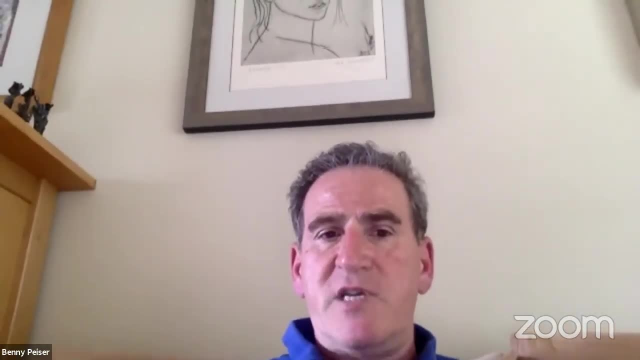 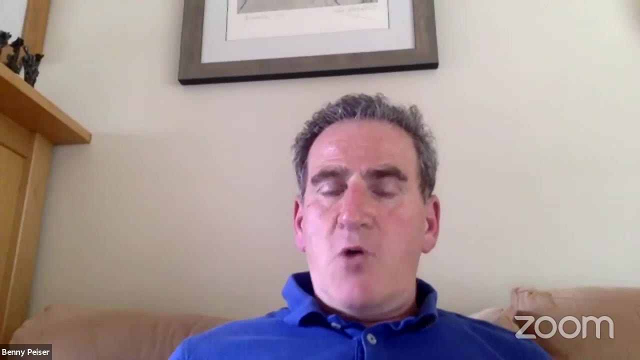 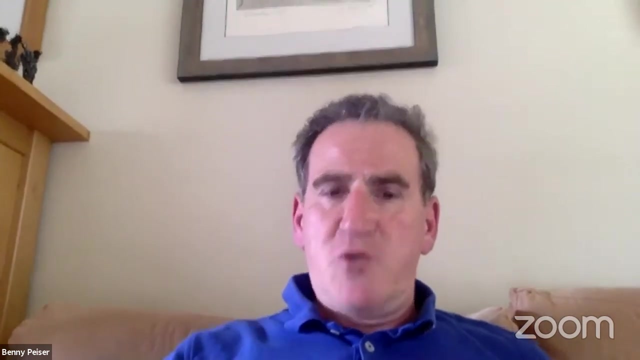 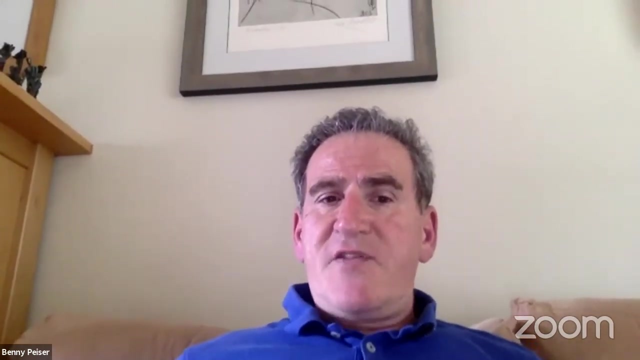 models, of politicized models, is that almost the entire alarm about global warming is purely based on predicting future disasters, future events. If you simply look at the chart that's on the right, you can see that over the last 30 or 40 years, nothing spectacular. 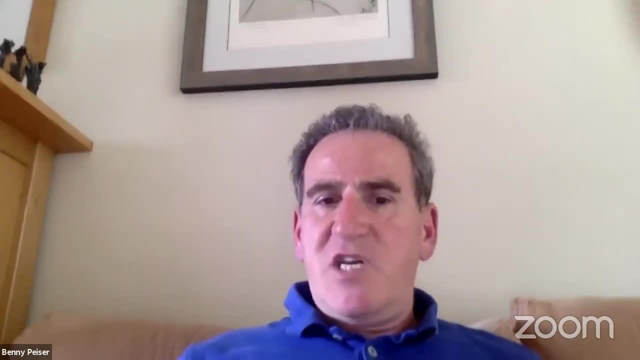 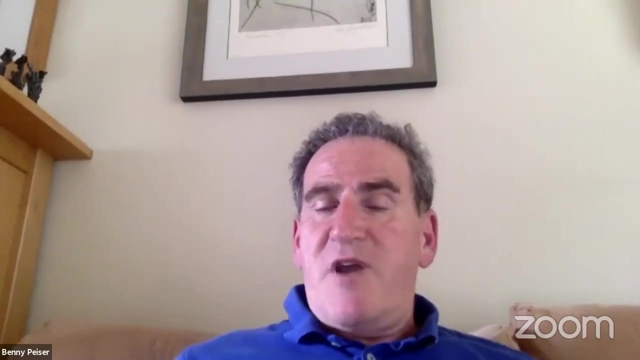 has happened. The warming has been very slow, has been very gradual, and there is no signal or sign that it will accelerate. It might, but there is, you know, nothing in the data to suggest that suddenly it will accelerate or double the rate of the trend of the last 30 years. So in this case, 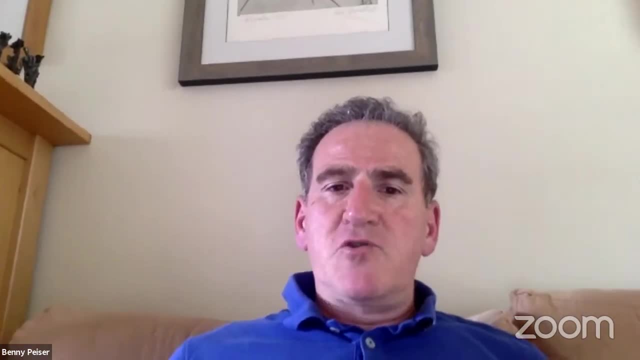 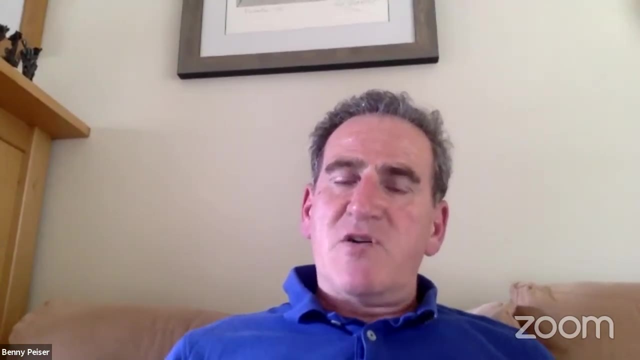 So the problem is that most of the news reporting is based on these models. They are not based on what is actually happening. They are based on people predicting that it's getting worse and that it's going to accelerate and that what we're seeing now will not continue. 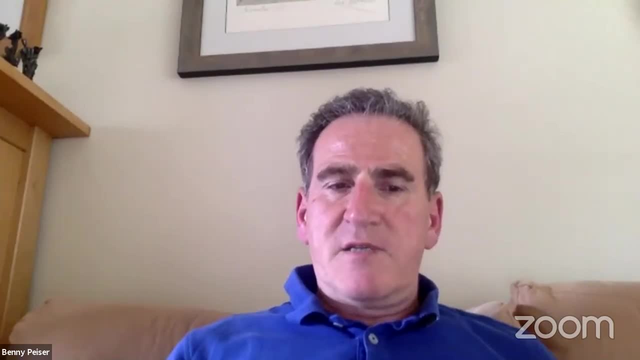 So we know there's a track record of failed modeling, which raises the question why scientists and governments and the general public continue to accept these kind of worst case doomsday modeling, unchallenged, uncritical, Why the news media is falling for these predictions, oblivious of all the failed modeling. 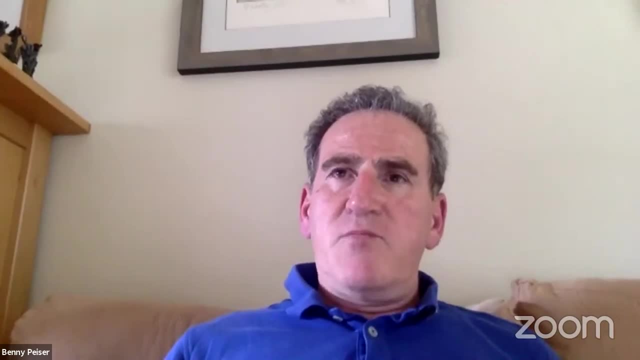 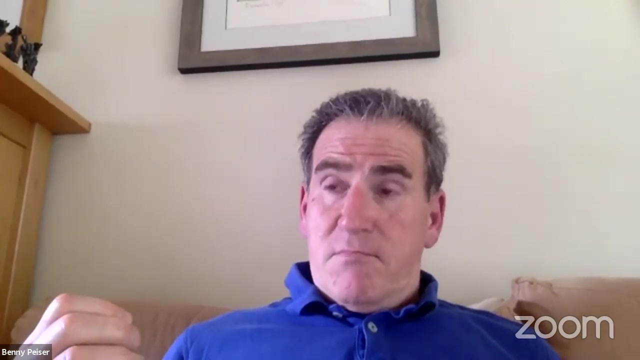 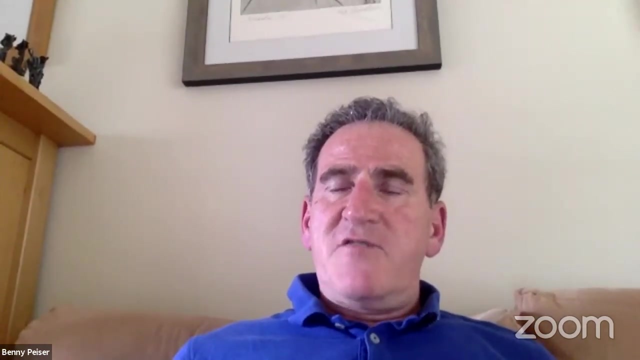 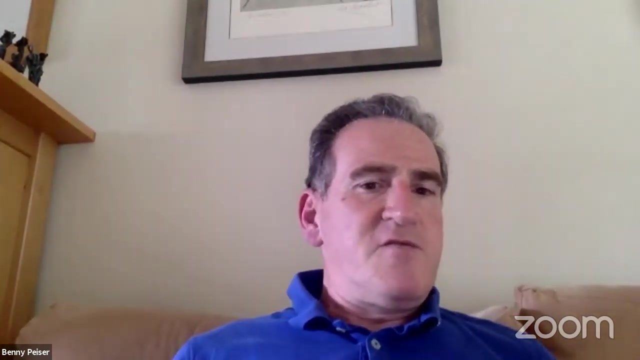 And one of the most important things in psychology in recent years. one of the most important discoveries or realizations is that humans suffer from what is called a negativity bias. This is a very important new acknowledgement of our human nature in that Because negative information and threatening information is much more powerful than any positive or reassuring information. 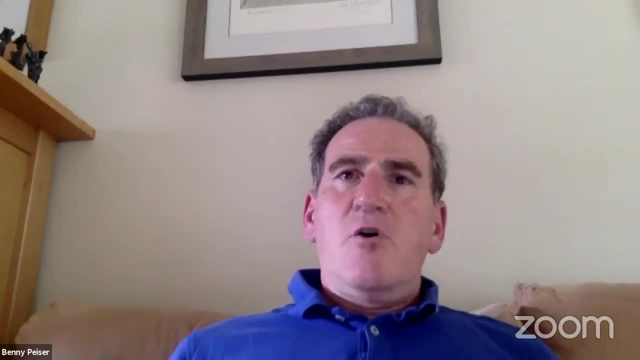 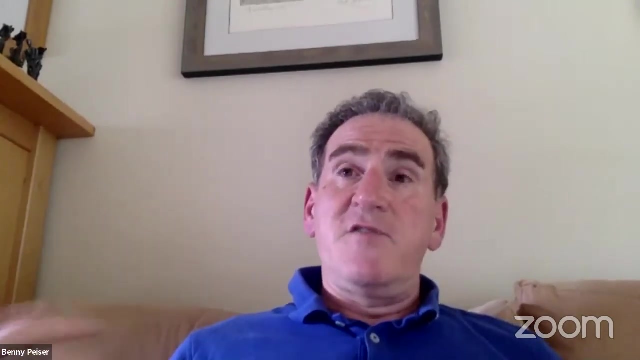 It's not as if we are rational beings who weigh up the positive and the negative, the pros and the cons. We don't do that. by and large, We are much more focused on the negative than on the positive, And so any negative information, any negative news, any negative models. 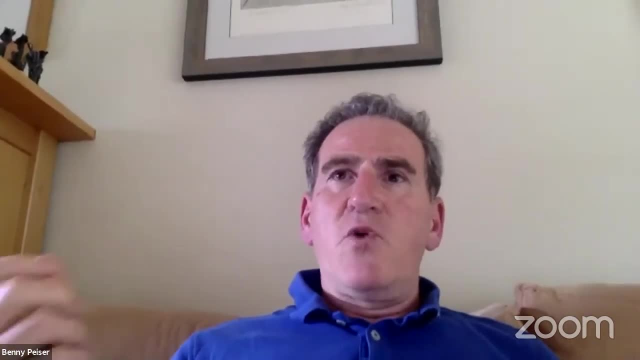 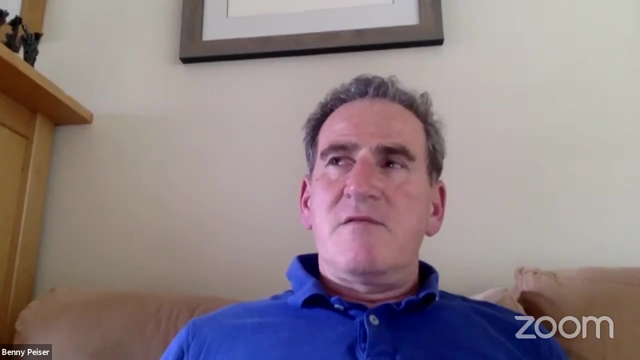 Modeling will draw much more attention and will actually cause a very deep psychological response, And this is not something you know. when we criticize people from being alarmist, that's very often not because they do that intentionally, but it is part of human nature of misreading information because the negative is so overpowering. 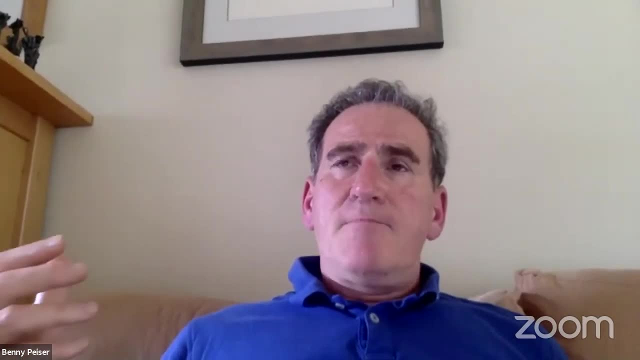 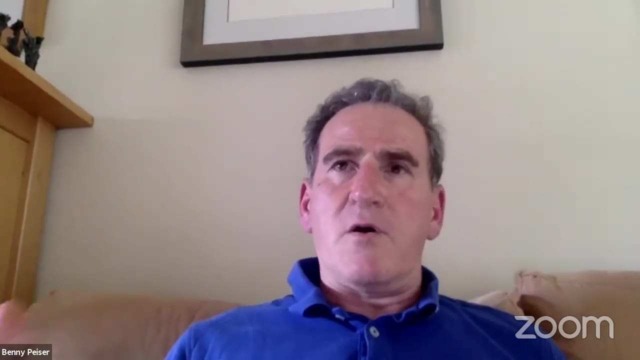 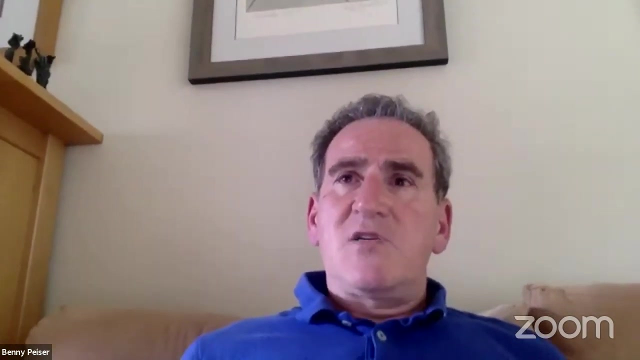 But this negativity bias, which has a deep and lasting impact on human judgment, on modeling, on policymaking, is something relatively new And I personally think is one of the reasons why we've seen this, what I regard as extreme overreaction to a disease that is severe, that is. 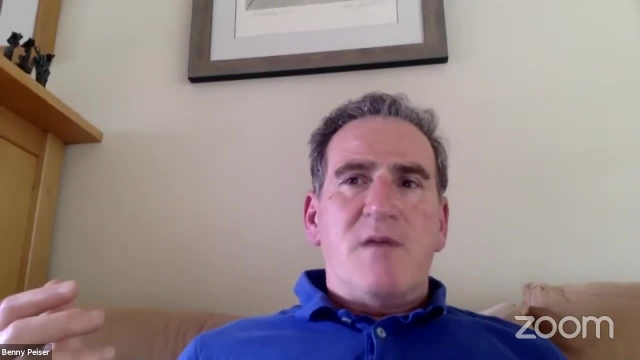 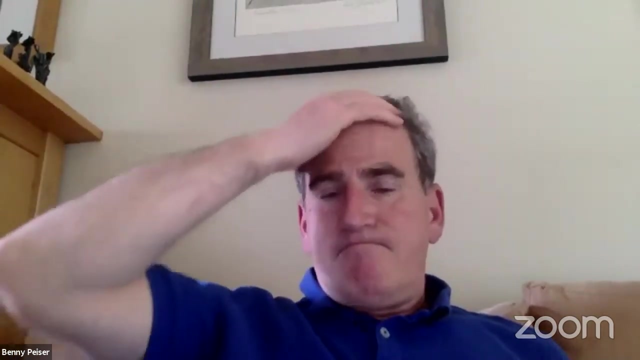 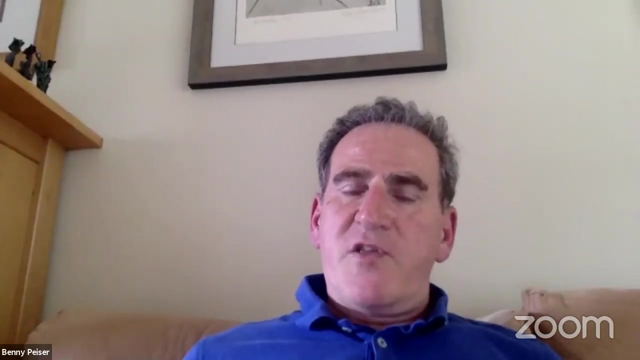 Certainly very genuine, but which is perceived as a risk much, much more significant than it actually is. So when the government, scientific advisors, the SAGE group, when they modeled the health risk of COVID-19, they didn't take into consideration 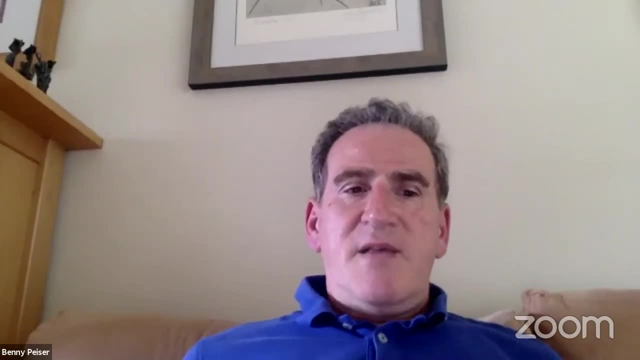 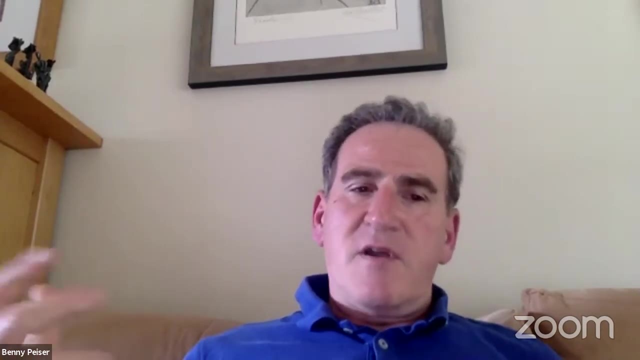 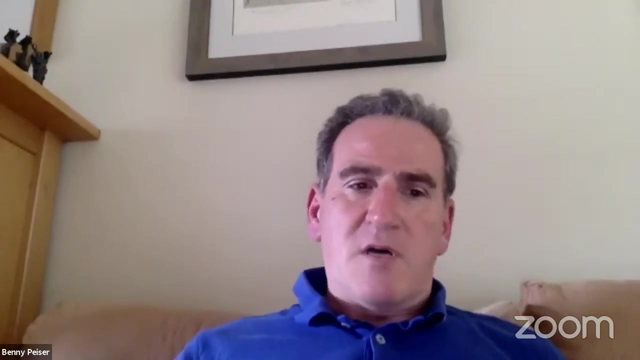 And that was one of the Criticisms by critics- the kind of health and economic risk of lockdown. They only looked at the risk of the virus and not the risk and the health risk and economic risk of the policies adopted, the lockdown policies. 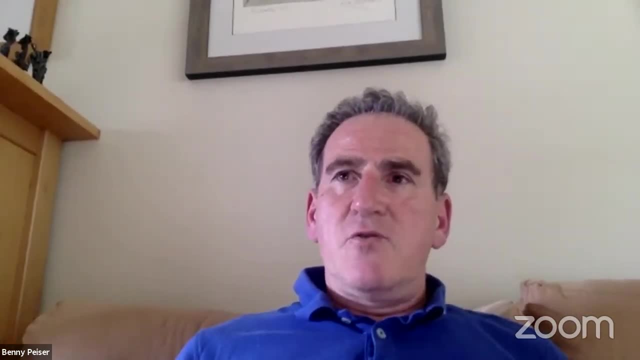 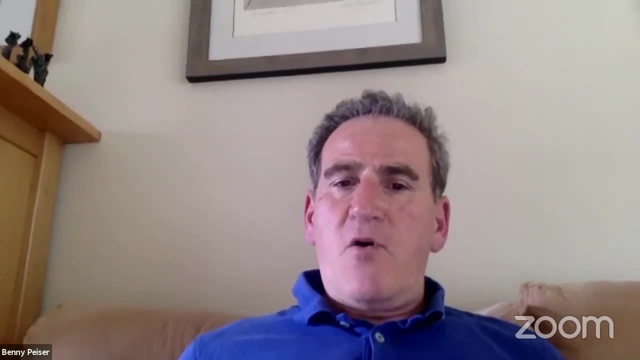 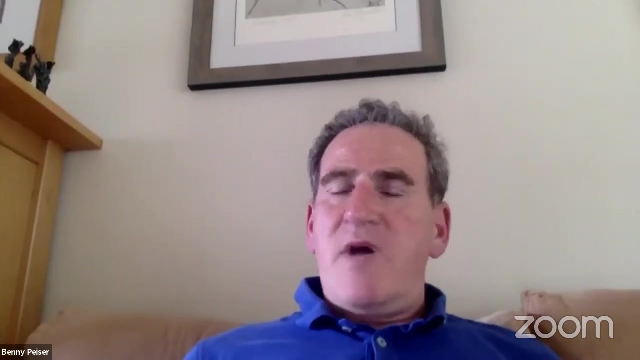 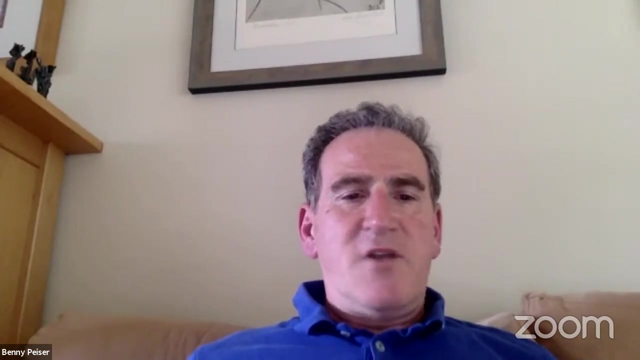 But including economists into a scientific advisory group in itself wouldn't have solved that problem at all, Because most economists- Economists- are just as crazy about modeling as scientists And many economists are just as naive when it comes to modeling. Just to give you an example, I recently read that a new study by US economists suggested that the lockdown measures saved the US economy up to $8 trillion in saved lives. 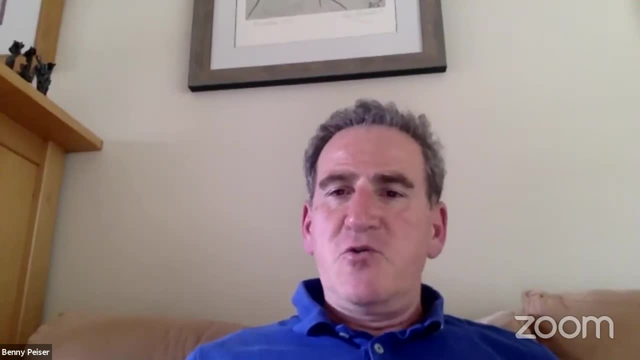 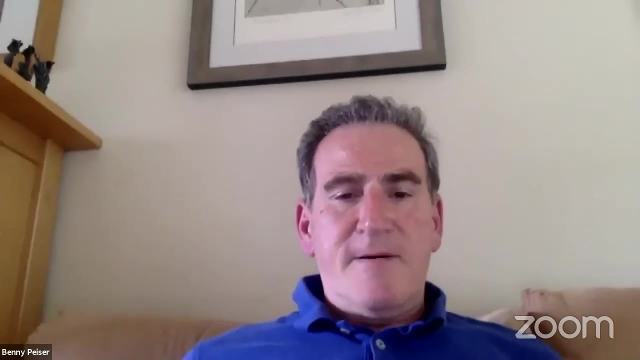 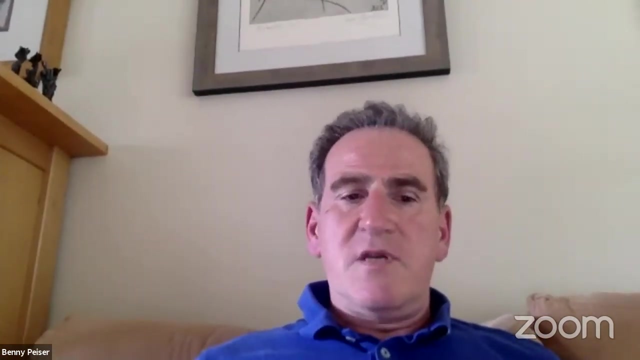 And how did they Managed to come up with this huge benefit of lockdown? They used the infamous Imperial College model and said: well, the lockdown has saved 1.7 million people. And you calculate the saving of saving 1.7 million people and you come to $8 trillion saved to the economy. 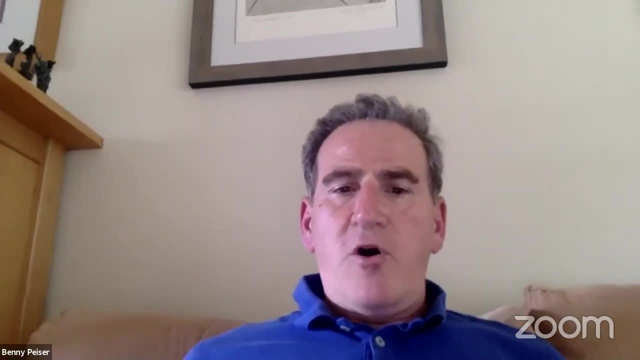 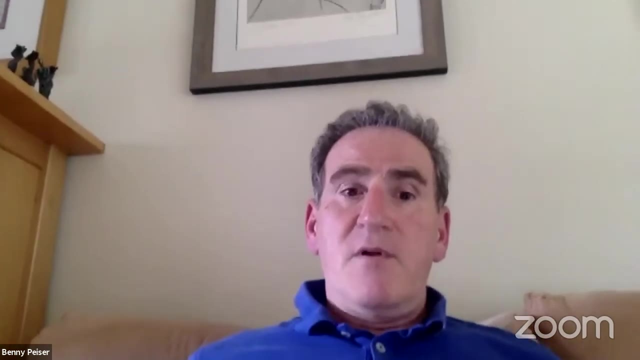 But in contrast to this model world of modelers in the cold reality Of the real world, there are now a growing number of people claiming that the lockdown might actually cause more deaths overall than the virus itself. Now, of course, the jury is still out on this, because the worst consequences of the lockdown are still ahead of us. 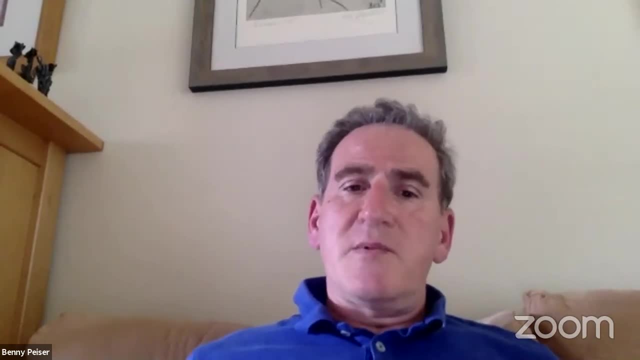 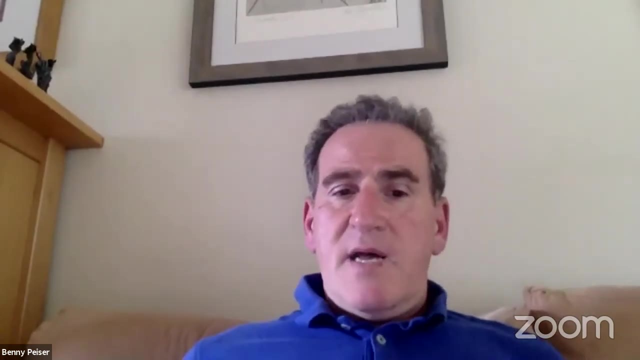 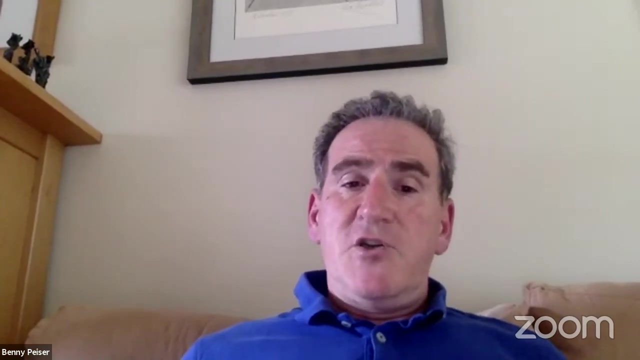 And we don't know just how deep the economic crisis we're facing will be, How many million people in the UK and world Why it will become unemployed modelers. at McKinsey, the consultancy, for instance, they estimate that up to 60 million people in Europe are at risk of losing their jobs. in Europe alone, 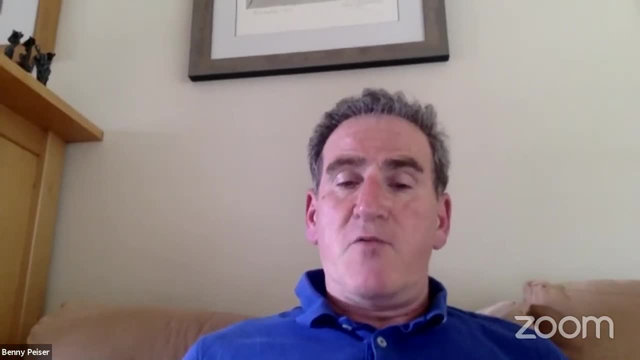 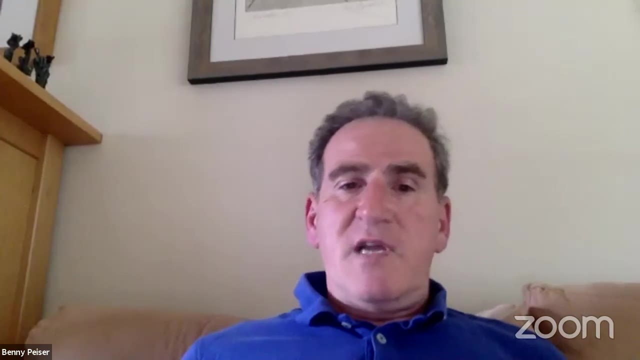 And we know, in the US, I think, 40 million people already have been made unemployed. So there is this looming economic disaster. No one, obviously, as I said, when these policies work, When these policies were adopted, took into consideration what the impact of the policies they recommended would be. 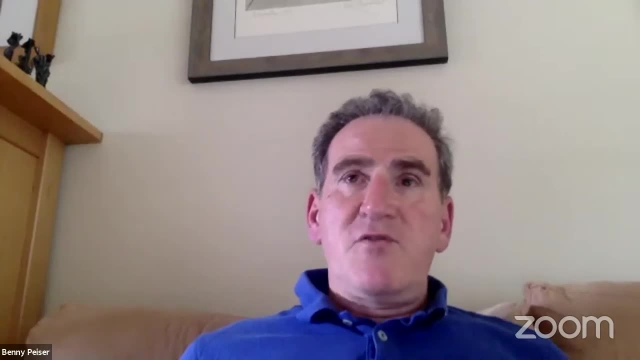 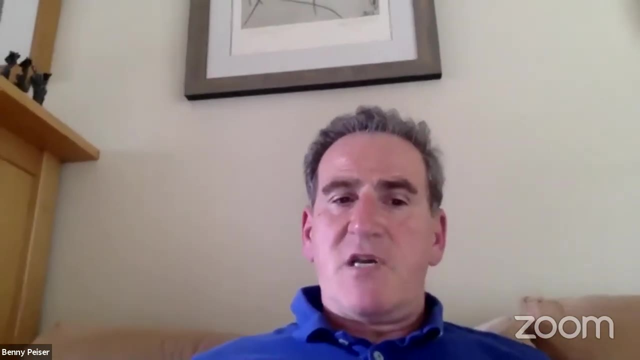 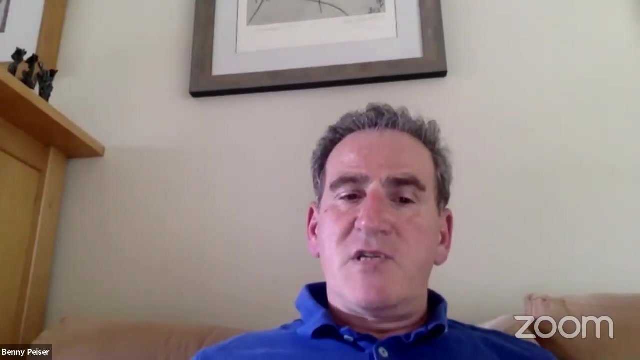 So, in short, this crisis has, in my view, caused the biggest economic and scientific crisis, at least since the end of the Second World War, And I personally think there will be very important lessons to be learned as a result of this crisis. 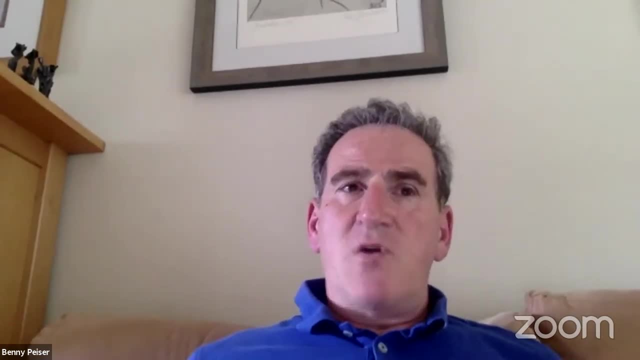 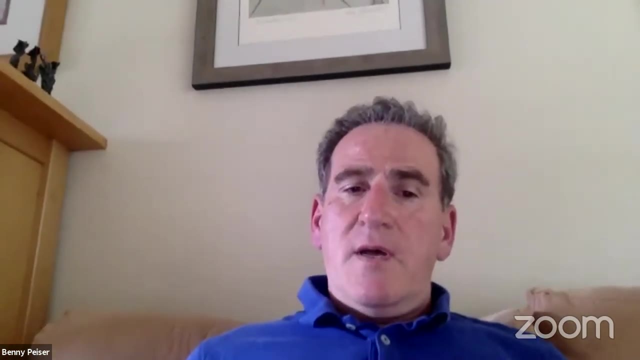 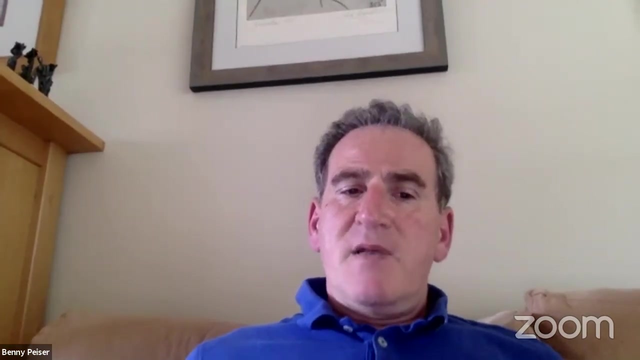 Not least In the way governments organize scientific advice. There are growing calls to provide governments with a broader spectrum, perhaps a full spectrum of advice And not just a narrow group of people- that the advice very often given is too narrow. We obviously have now a competitive system. 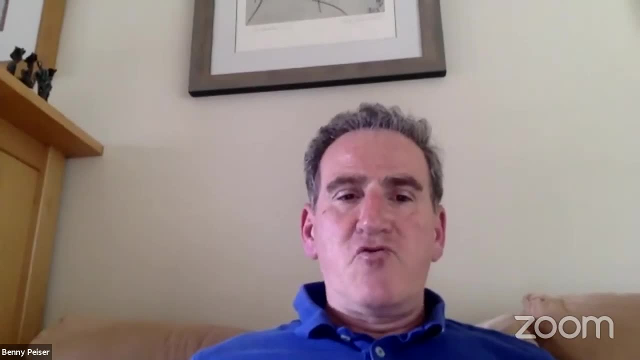 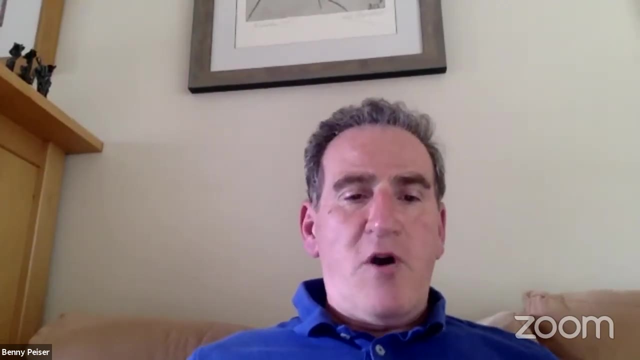 We have a competitive scientific advisory group led by Sir David King And interestingly enough, they today warned that the policies of the government to open schools on the 1st of June is unsafe. They couldn't rule out that people could get infected, of course, as Gordon just said. 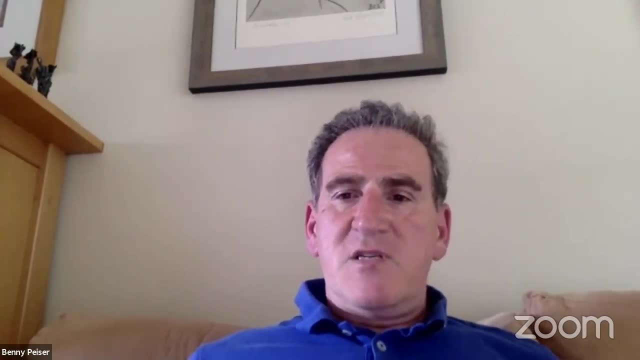 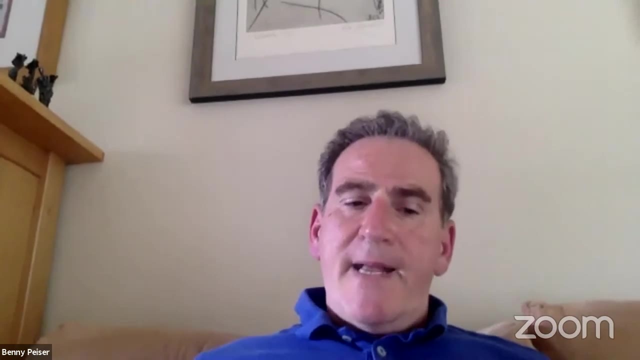 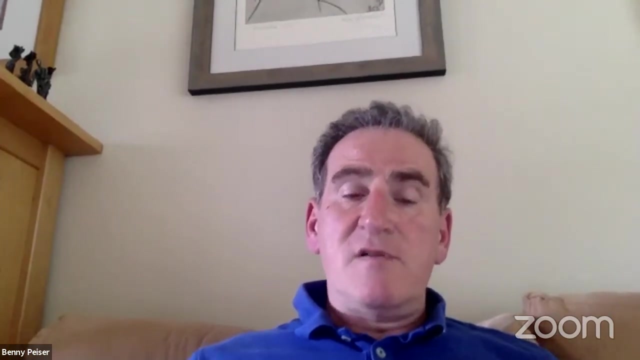 Of course you cannot rule out anything. The question is just how big the risk is. But we have now completed. But we have now competing scientific advisory groups And that in itself isn't bad, But they are adversarial rather than collegial. 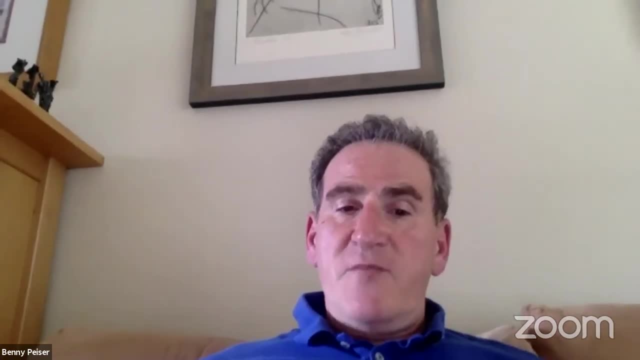 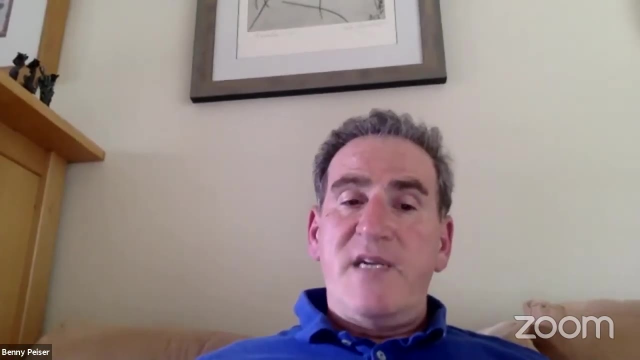 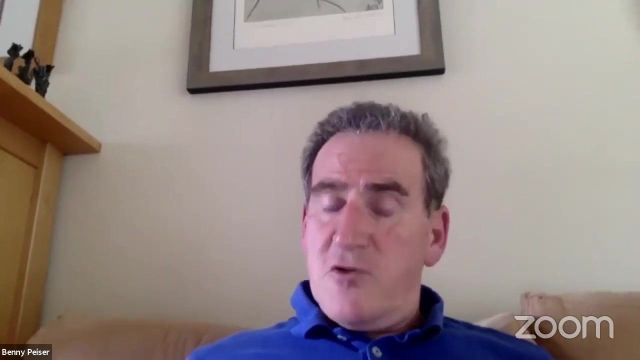 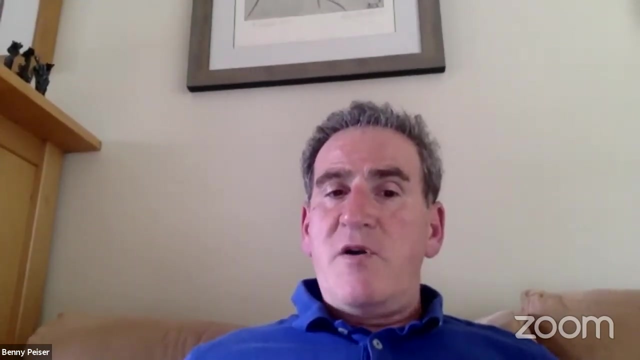 And it might be much wiser for governments to have competing scientific advisors and advisory groups in the tent and providing them with a full spectrum of advice. But that in itself will be contentious because we, the scientific organizations around the world, unfortunately have portrayed in recent years the way science is organized as one of consensus versus dissent. 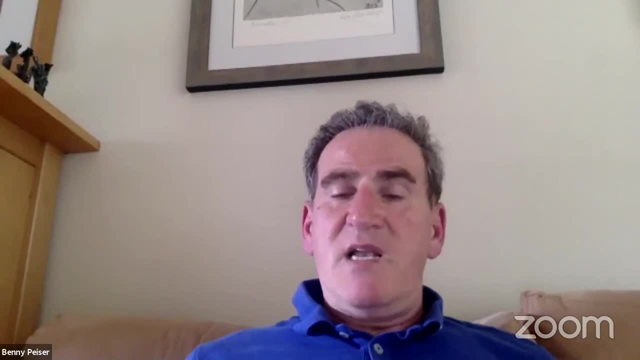 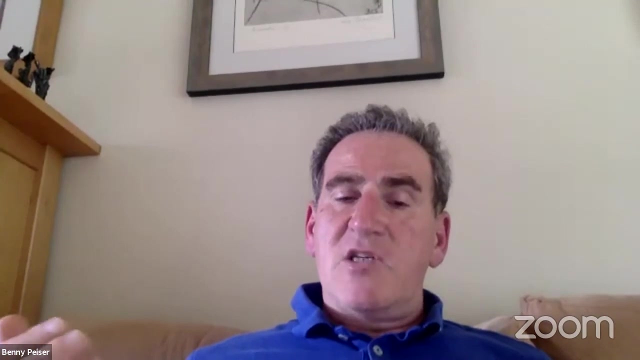 As if science is based mainly on majority view And anyone who falls Into the group of dissenting voices shouldn't be heard. That is not how science progresses. So I think it is very important that we realize that as long as scientific advice is narrow, isn't challenged and isn't scrutinized, there will always be the problem of getting it wrong. 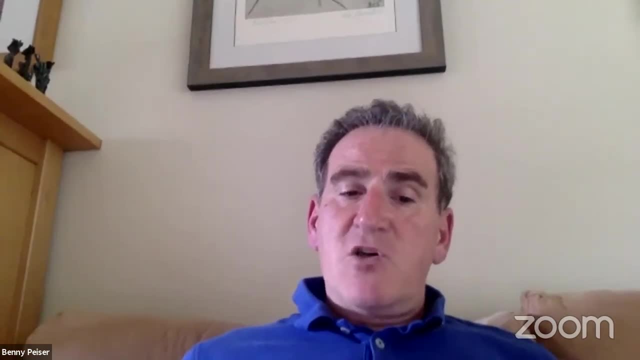 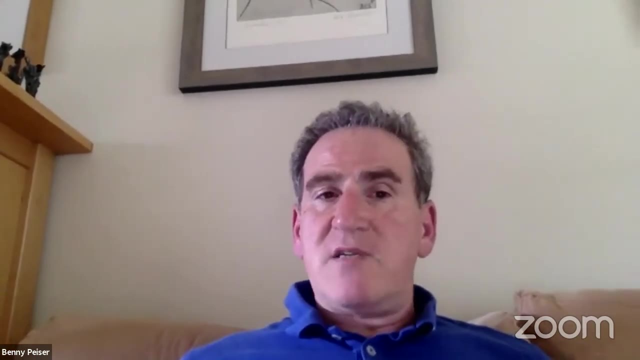 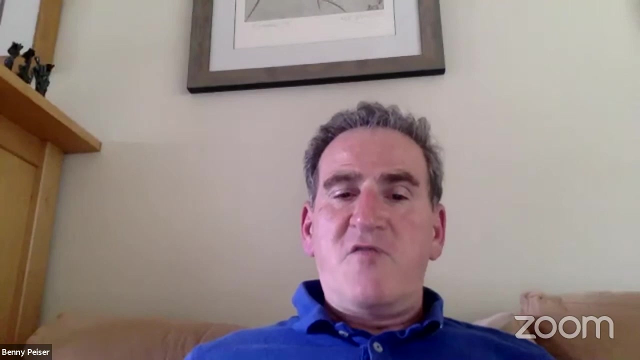 And making big mistakes. So I personally have been advocating the introduction of institutional red teams. The military does that habitually. obviously They want to find the loopholes, They want to find the flaws in their own models, in their own strategy. 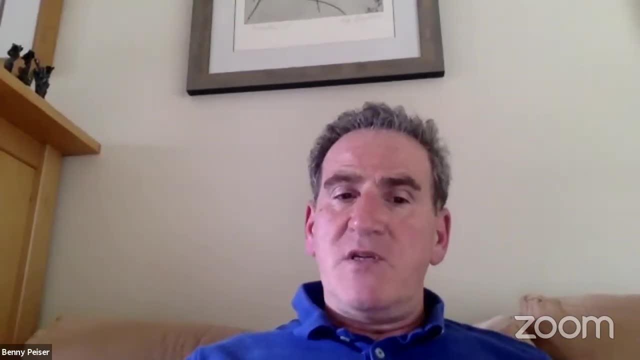 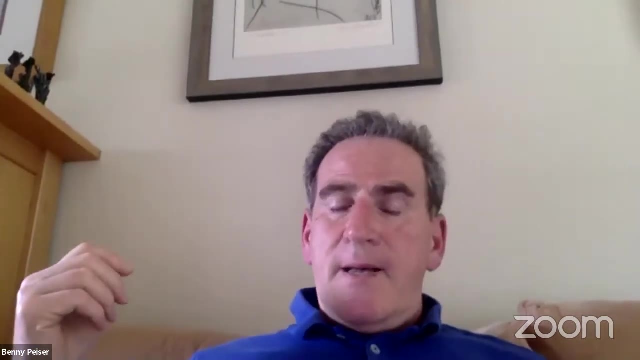 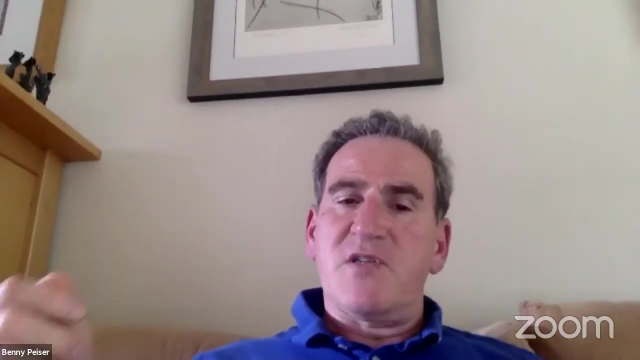 And the best way, and a lot of technology companies do the same. They want to make sure that they're Software and their programs are secure, So they will recruit red teams to challenge their programs to find problems, because they want to close these problems. 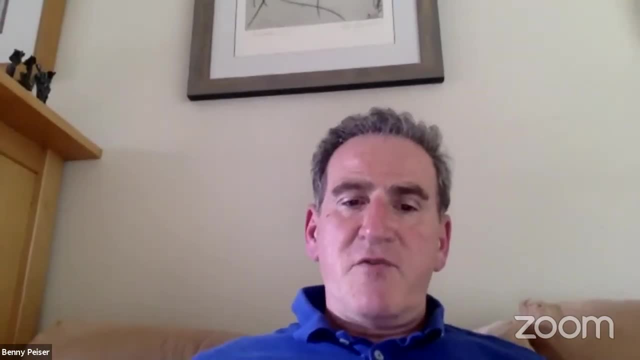 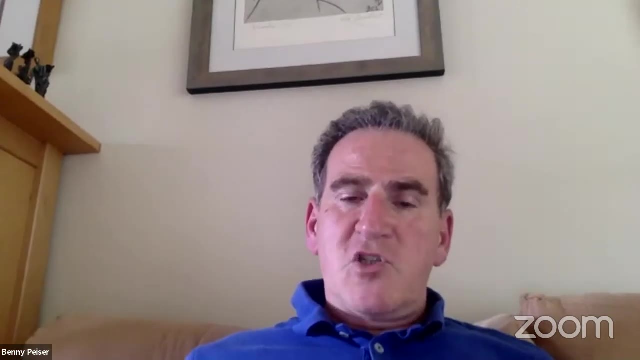 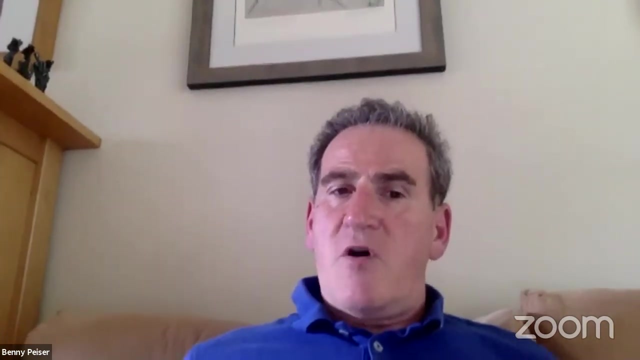 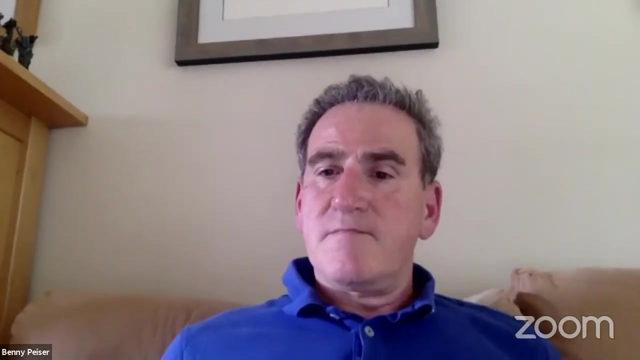 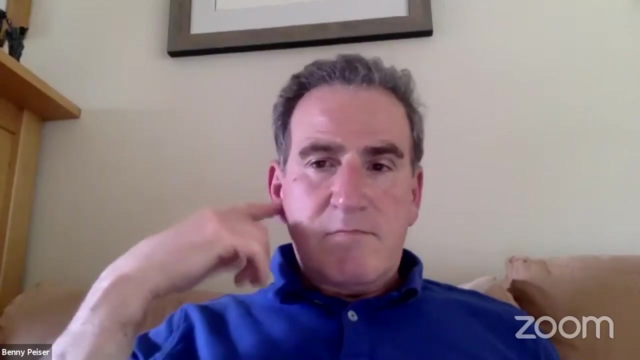 And I personally think we need this kind of scientific reform so that the government advice is really much more solid, much more scrutinized And the government has the full control And the government has the full spectrum of views of reputable scientific advice. Thank you, Harry. 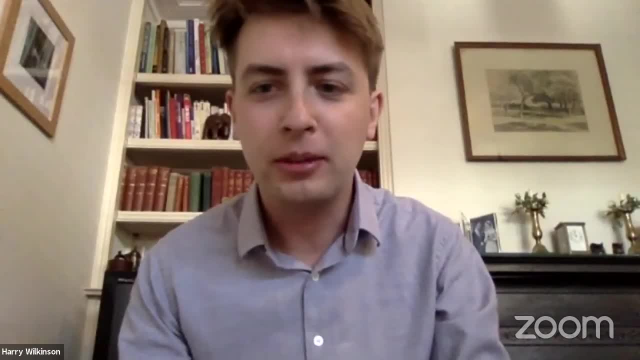 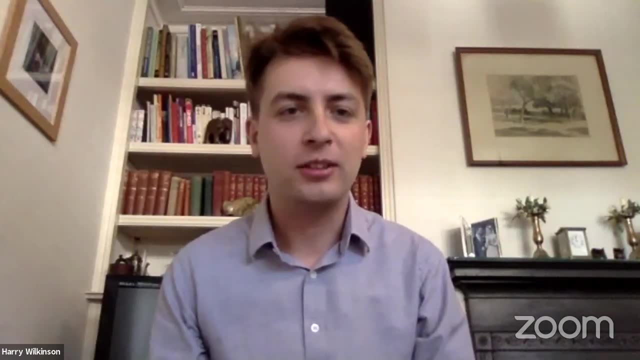 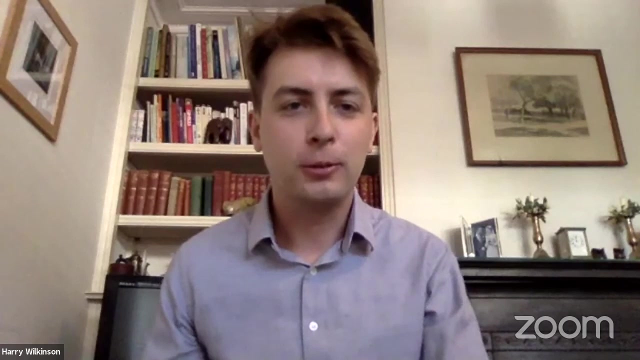 Thank you very much, Benny. I will just unmute everyone now And we will enter into a Q&A session. We've had lots of interactions from people following in And I've been seeing that the chat has been very active. So thank you all for engaging with this discussion. 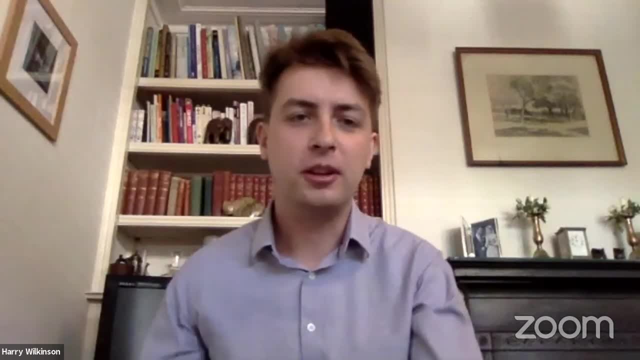 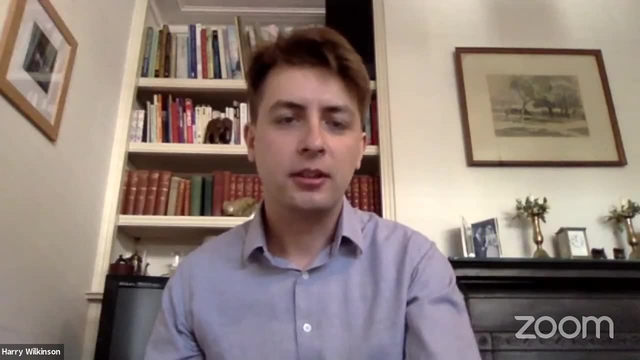 I think the first question just follows on a lot from what you were saying, Benny, which was: why is there this huge focus on the worst case scenario? And I mean, if I might just offer my own comment, I think we've seen: 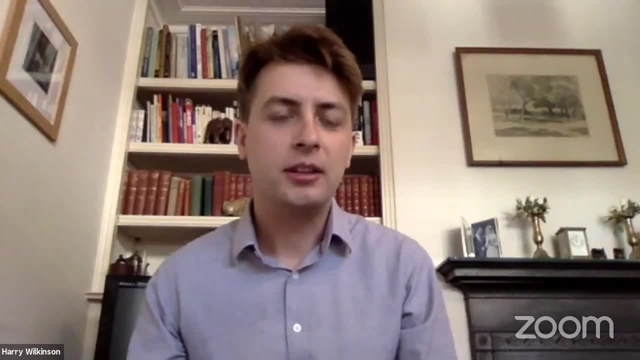 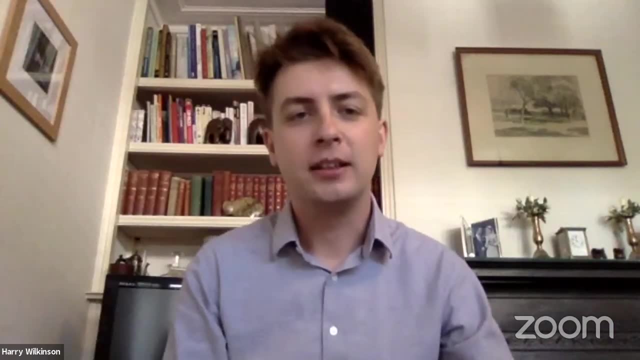 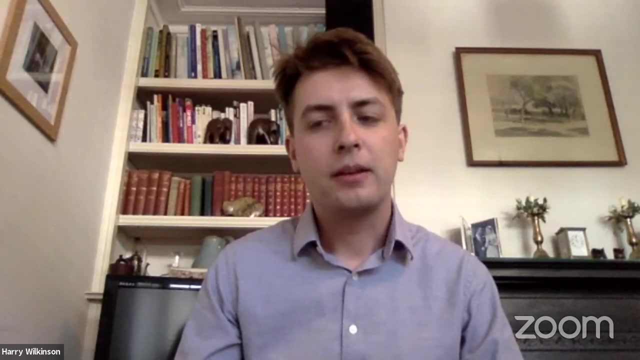 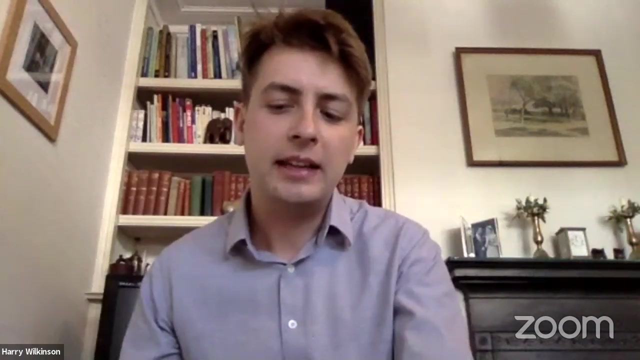 I think we've seen a narrowness of focus in that. we've seen Neil Ferguson's model, Regardless, even if he was correct. we're looking at deaths from a disease, But we've seen there's so many other consequences of lockdowns that needed to be considered and perhaps weren't considered in the initial moments when they were devising the policy. 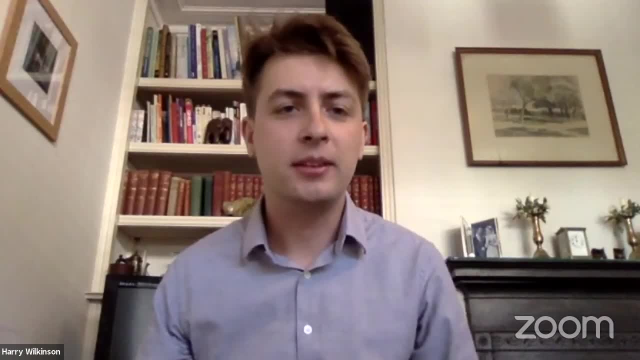 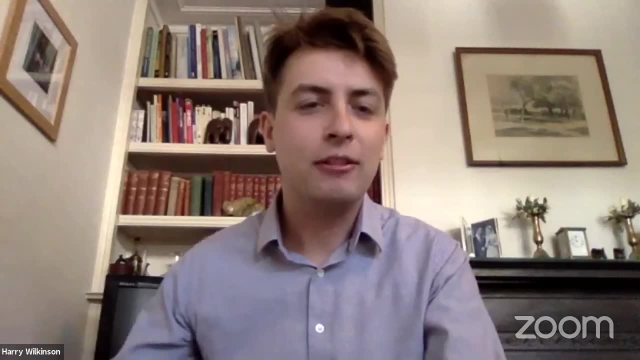 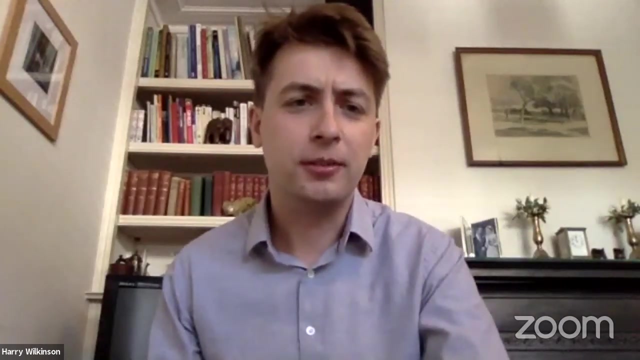 And we see in climate policy. we see climate scientists shouting: here's a big risk, It needs to be controlled, And there isn't on their mindset whatsoever. well, what might be the unintended consequences of those policies? So there's a need to be broad. 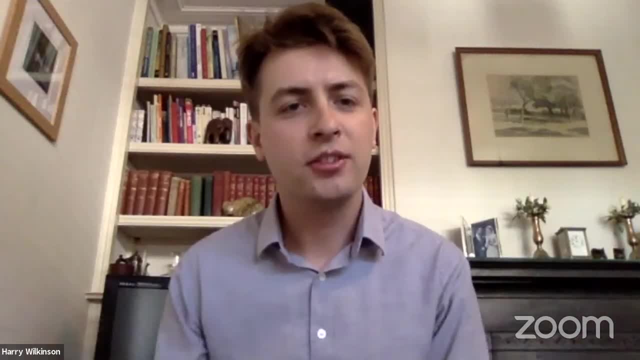 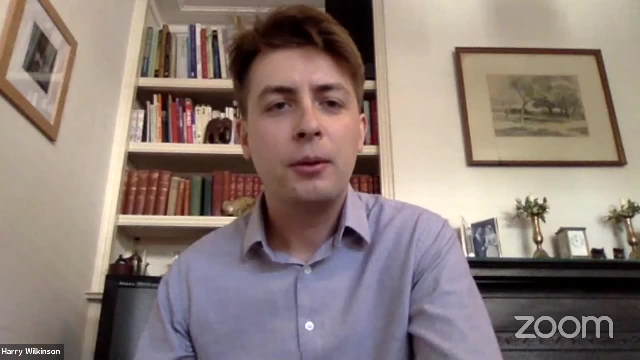 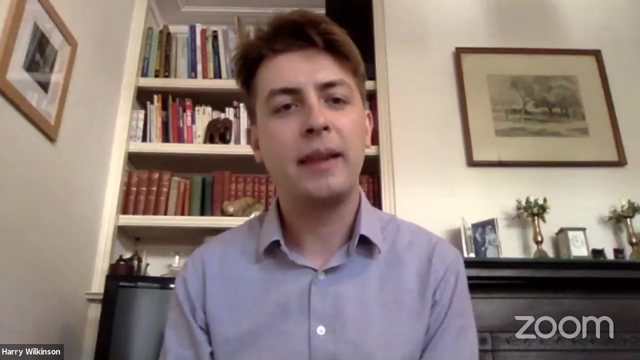 But there's also a need to actually answer specific questions. You can't be endlessly broad, Because that would just sort of leave you nowhere whatsoever. So how do politicians and scientists balance that need to be more specific and to have a broader balancing of the risks? 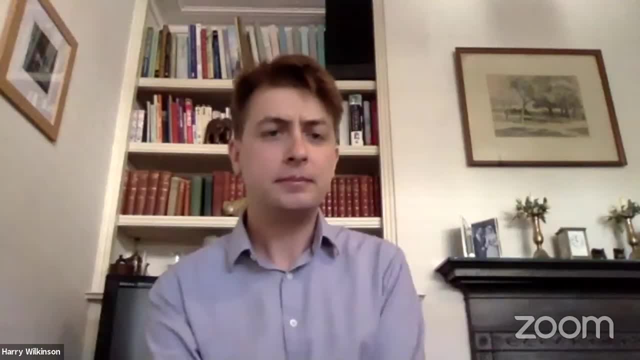 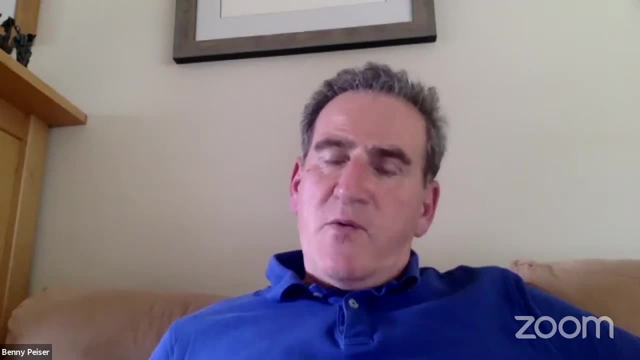 So, Benny, would you like to pick up on that first? Well, I tried to highlight these new psychological understandings of the way we tick And unfortunately. I mean you could ask why is there so much negative news on television? 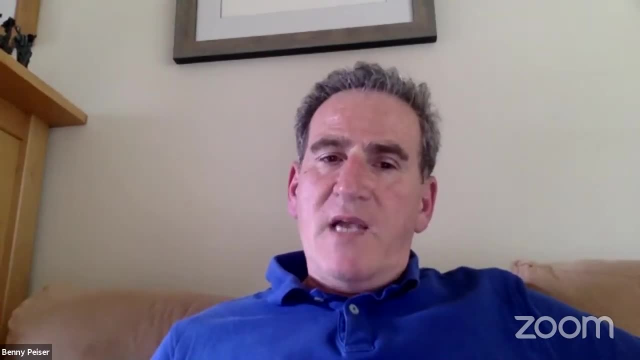 On television and in the newspapers. The reality is that we are much more alert and much more anxious about potential risks, And that we believe risk mongers more than rose-tinted optimists. That is just the reality, And it is very, very difficult to change. 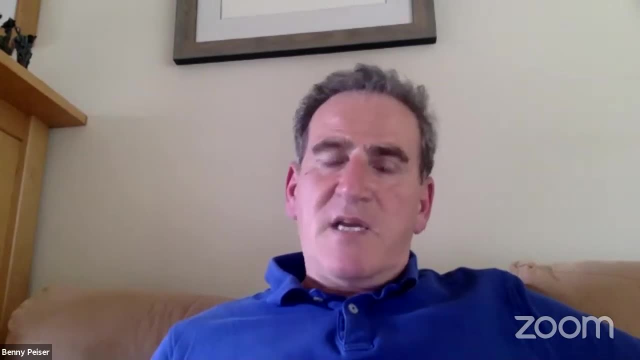 So change that mindset extremely. And in a crisis and in a situation of mass hysteria where the media screams at you 24-7 and shouts at the ministers, you have to do more, You have to be stricter, You have to lock down. 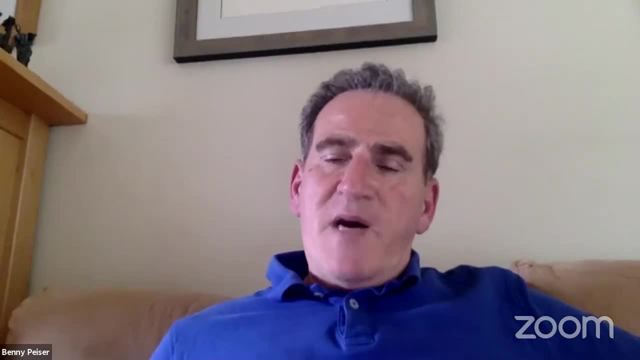 And you don't allow people out And in a climate of mass hysteria, it's almost impossible to weigh up, To weigh up in a rational manner The pros and the cons, The costs and the benefits. It's very, very difficult. So we have to accept that this is not just a political game by people who are using fear as a weapon- That happens as well- But in reality, people are genuinely risk adverse. They are genuinely scared, Particularly when experts or governments tell them to be scared. 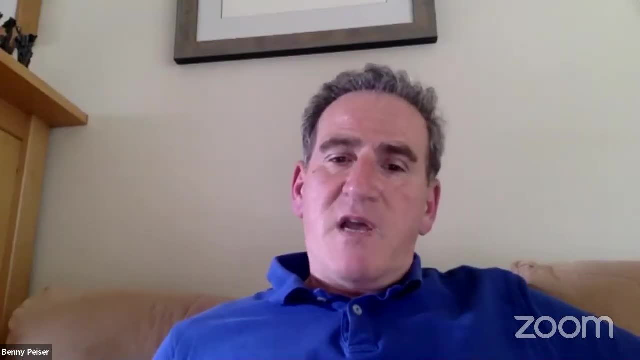 Which is, you know, on climate, environmental issues and COVID. it's the official party line, It's not just a few modelers saying that It's. then the government adopts these kind of scary scenarios and tells people: you stay at home for the next two or three months, because going out is a huge risk. 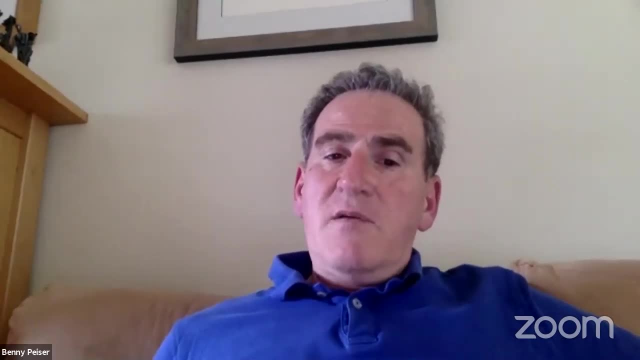 So unfortunately we have to accept that human nature is susceptible to risk or threat inflation. How to overcome that is a task for governments to look into it. I think we really need very, very serious inquiries into the way, Because governments don't know. 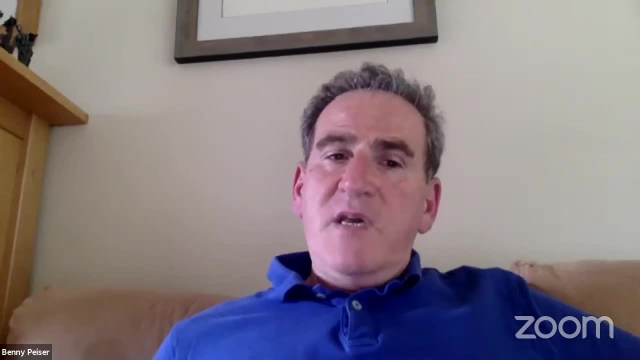 They don't know. They just don't want to fall into the trap of being basically pushed into a policy they don't want to adopt. Remember, the government for quite some time tried to adopt a policy that was more closely to what the Swedish government did. They couldn't sustain that in the face of huge public outrage By the media and by journalists who shouted at them that they were killing the public with their- you know, kind of restrained policy. So it's a tricky issue. There is no easy solution. 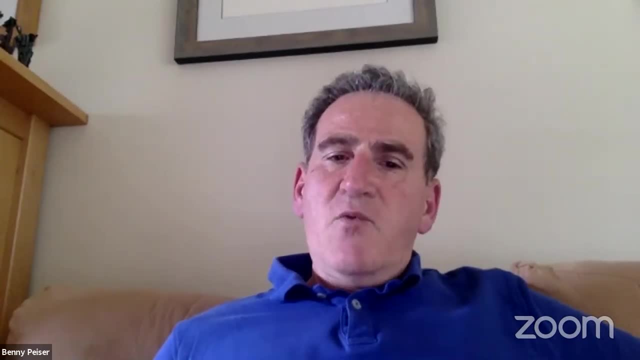 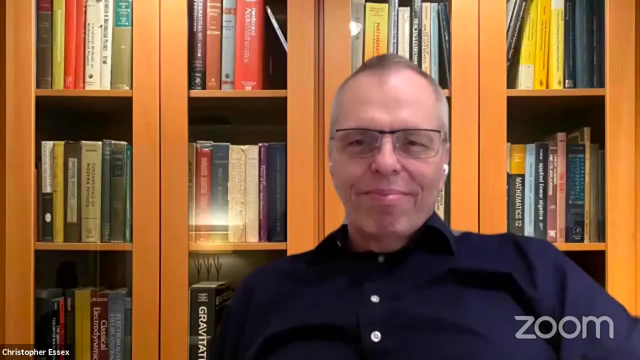 But governments will have an interest in looking into how not to fall into the trap of scaremongering. Chris, would you like to add something? Sure, Sure, Chris, would you like to come in on that next? Well, there are a bunch of things I'd like to comment on, but I don't know if there's time. 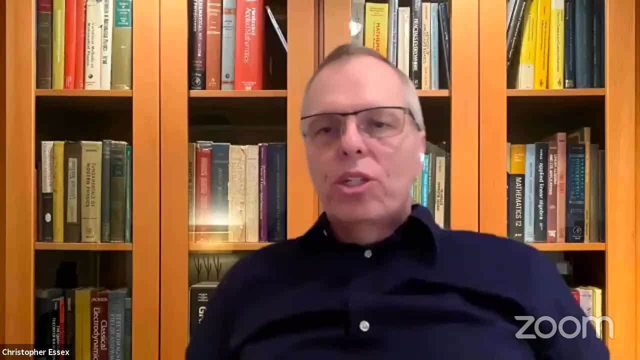 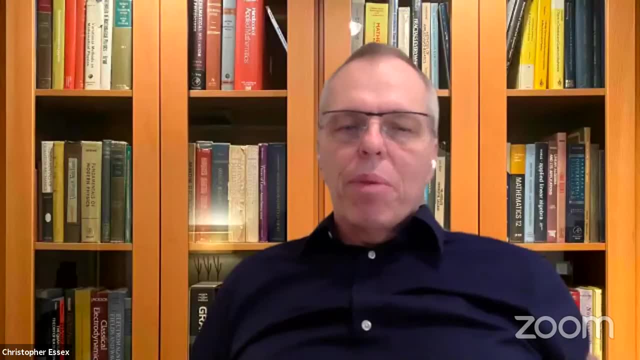 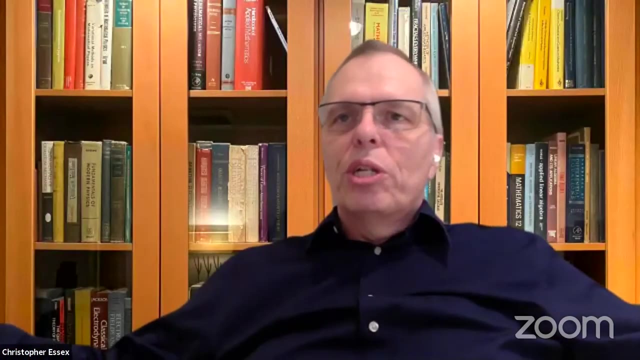 The basic issue of policy is that decisions have to be made with incomplete information. So one can't make the ideal decision because the real world is happening now And, while we might have an opportunity in the future to contemplate what's going on, you have to make the decisions. 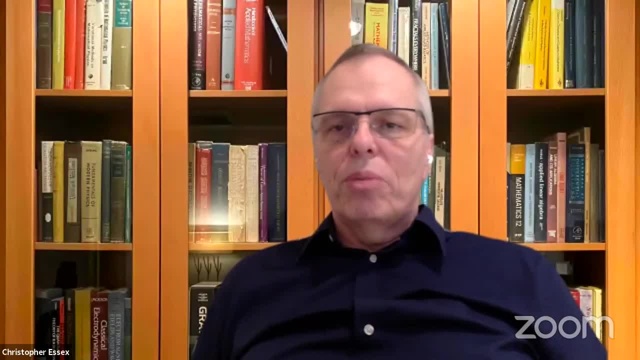 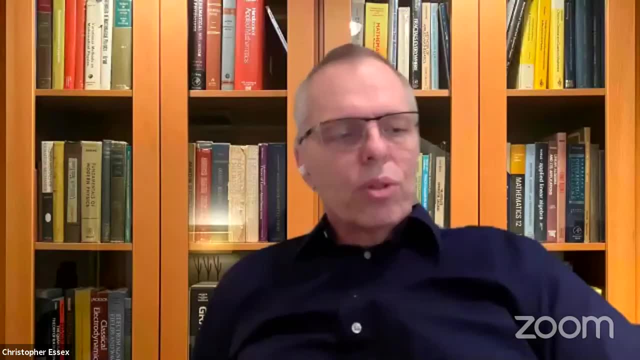 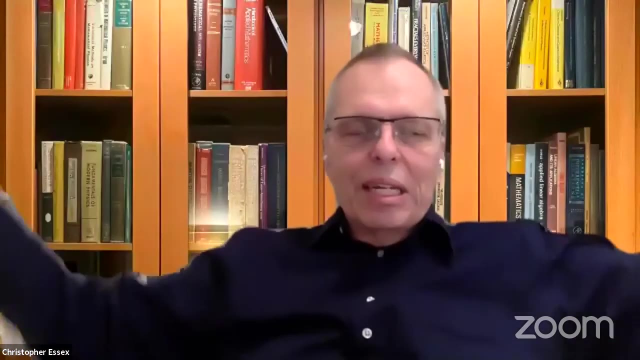 And so one has to be a little bit sympathetic to policy people who make these decisions, and they probably are going to get it wrong. But the part that I'm most concerned about particularly- and I agree with what Benny was saying about people being, you know you have to be really flamboyant to get attention. 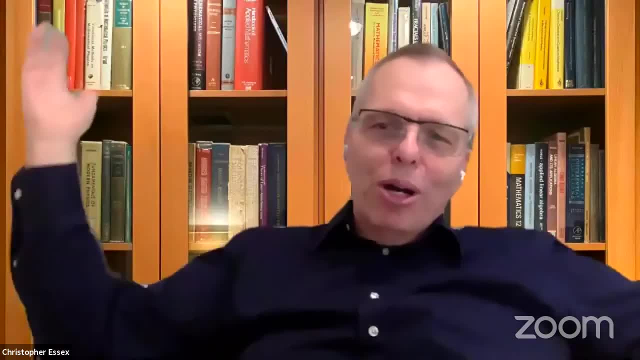 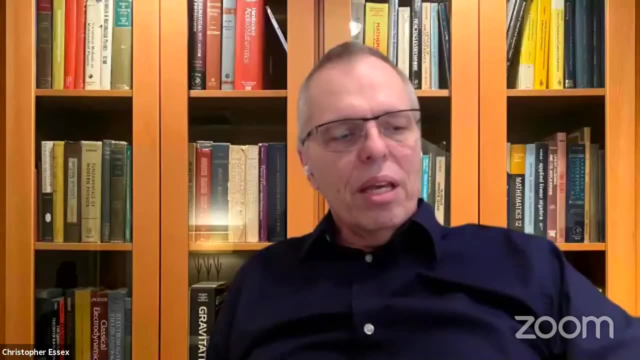 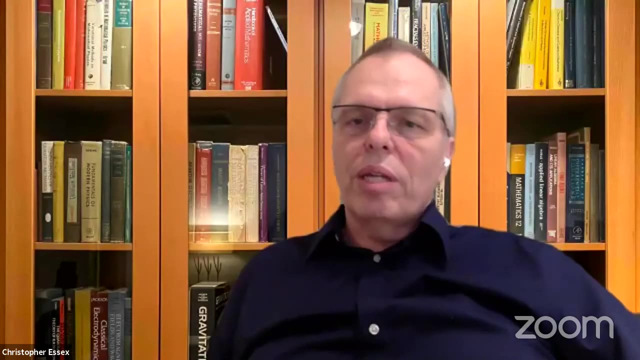 And usually it's negative and scary and the apocalypse and Ragnarok and all this other stuff. People love their apocalypse, But the thing I'm most concerned about is policy. The thing I'm most concerned about is not that policymakers listen to scientists per se. 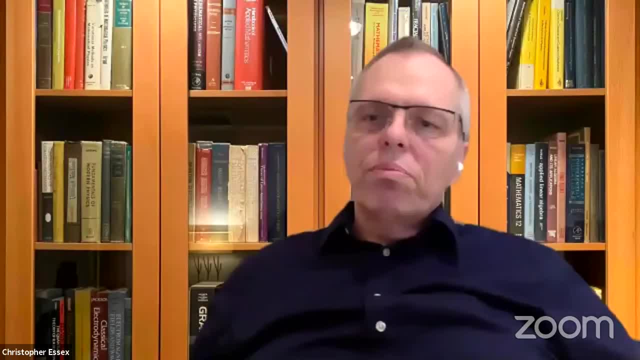 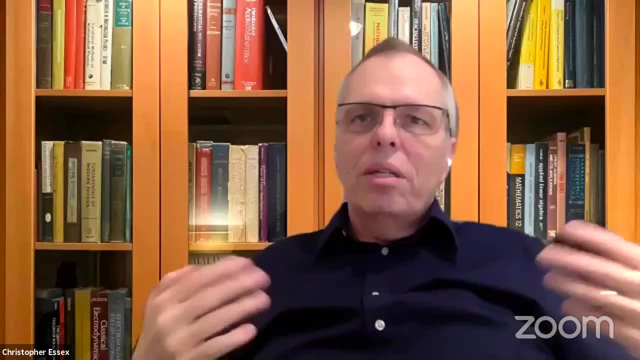 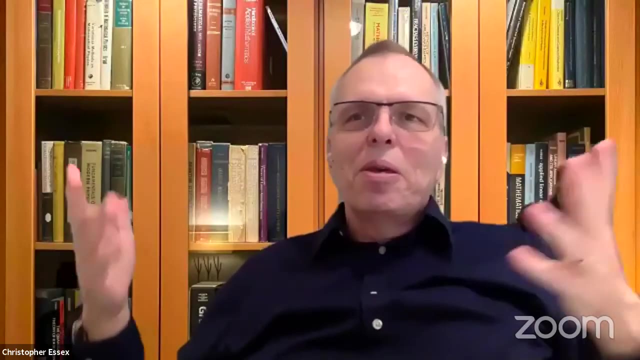 It's that they want to look at the scales the scientists have been looking at and they want to put their finger on it to adjust things. And that leads immediately to something that Gordon said, which he suggested: that there were no payoffs for advising. 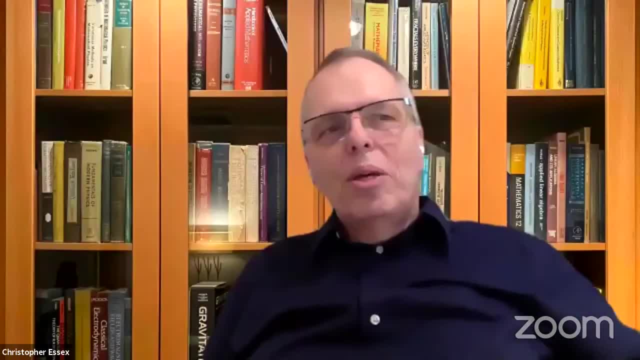 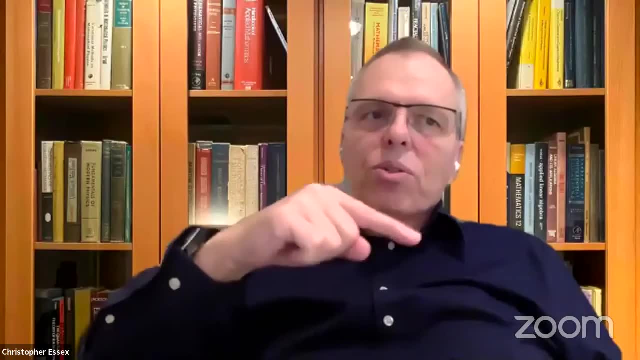 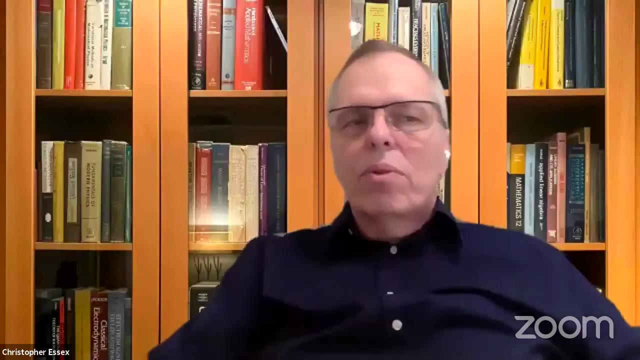 Well, yeah, probably as a courtier. That's probably true, But when it comes to what's happened, certainly in connection with climate, there's been a lot of fingers there And it's affected the whole social dynamics of the field in a way that has distorted how we think about things. 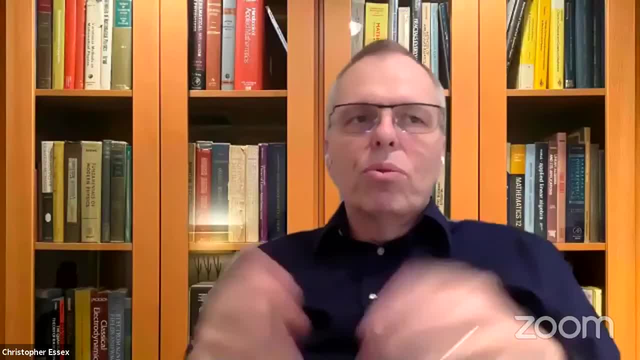 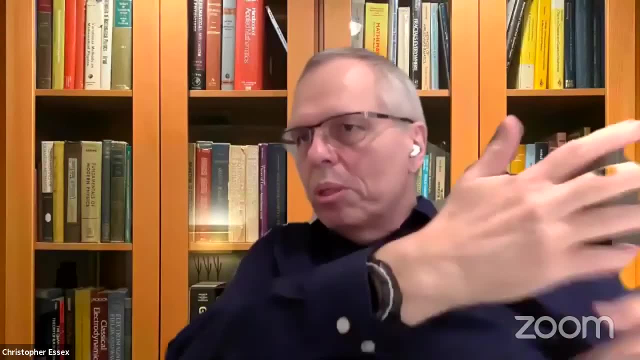 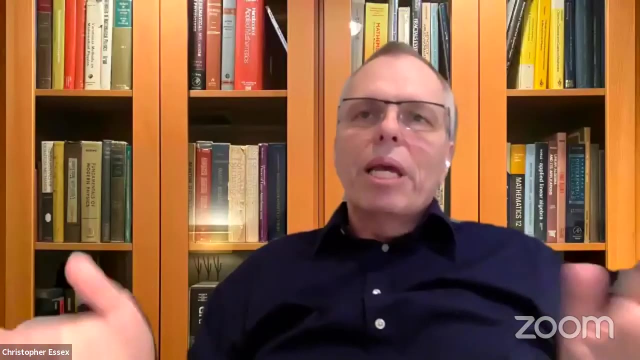 What should be done is it should be completely separate rooms. There's the policy people and the science people And the science people And the science people. People should have a red team. There should be some collection of a spectrum of positions, And then the policymakers can make a decision. 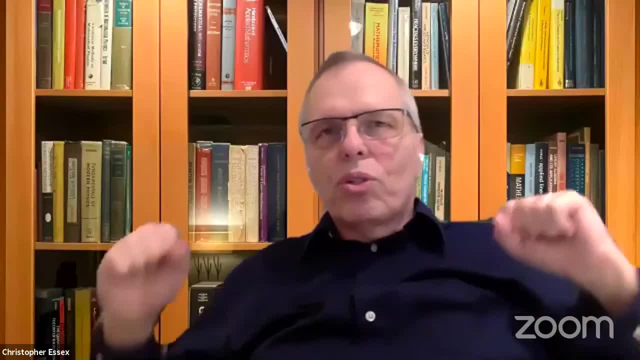 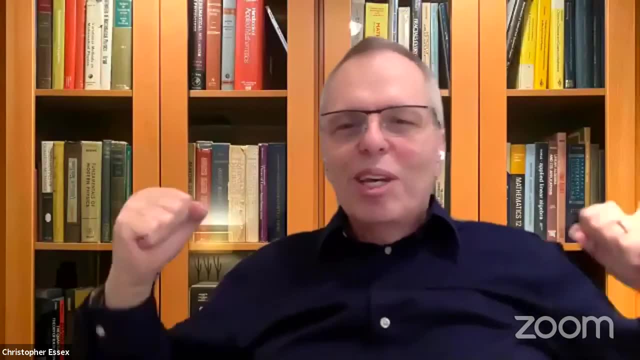 But what we have now is we have this. I don't know if you know this comedian from the 1970s, this American comedian called Flip Wilson And he always with his catchphrase with the devil made me do it. Well, the politicians have a devil. 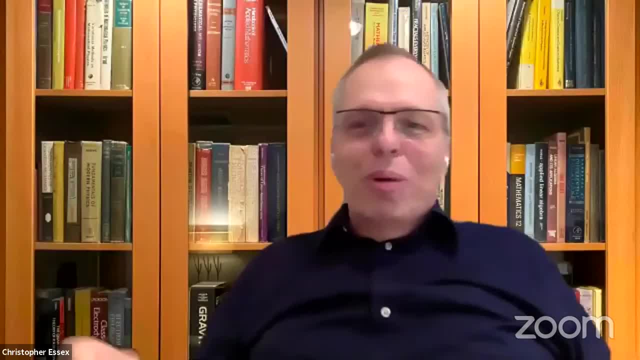 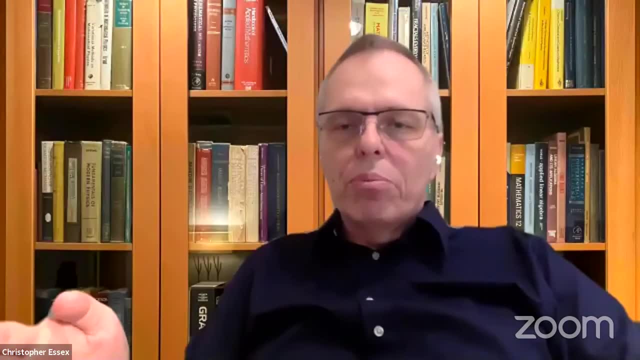 They say: the scientists made me do it. I don't know what to do, but the scientists made me do it. And that can't be. These people are in a position to make decisions with incomplete information. That's their job And they shouldn't be saying: well, the scientists are the ones to do it. 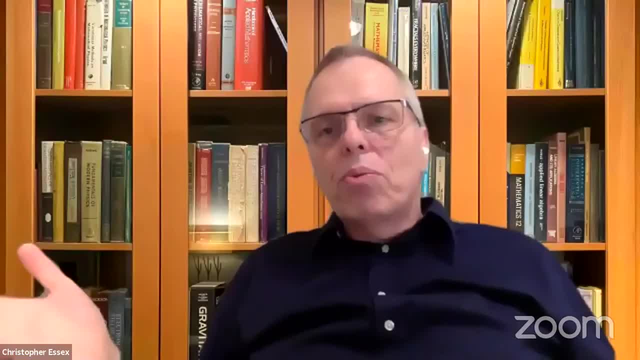 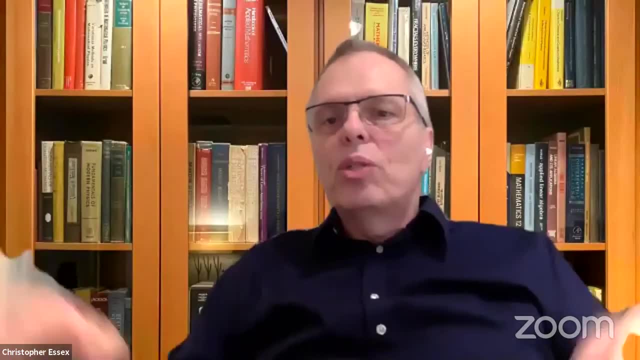 And then I'm just a puppet and I do what they tell me, And that's, I think, one of the problems we're encountering. We have to somehow force the decision makers to bear the responsibility of the decision, given a full spectrum knowledge of what's going on. 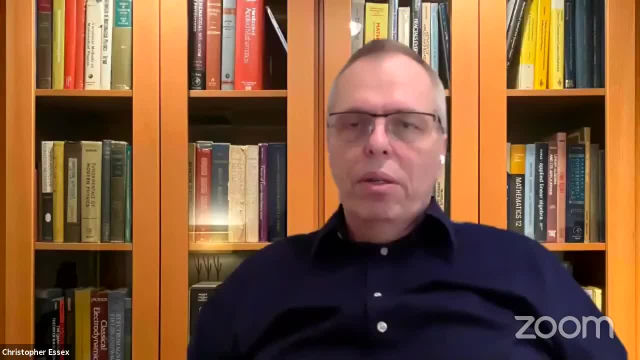 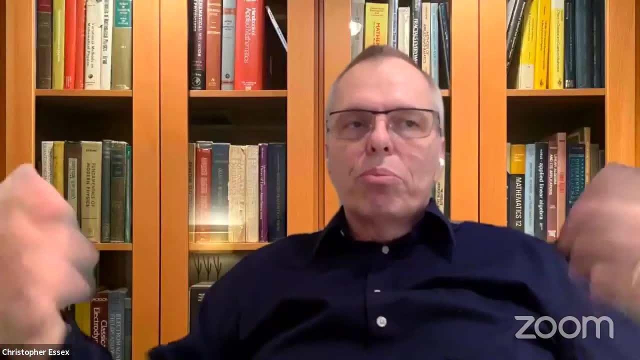 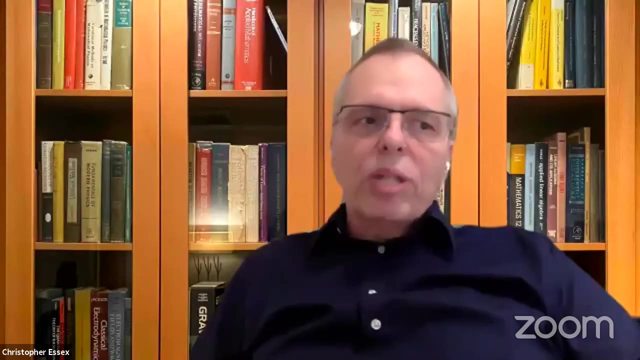 And that's what's not happening on any of our scientific discussions. OK, The other thing I wanted to follow up on was this business about using models to predict the future, And then one of the things that people will find a little bit disturbing is that climate models are actually pretty lousy about. 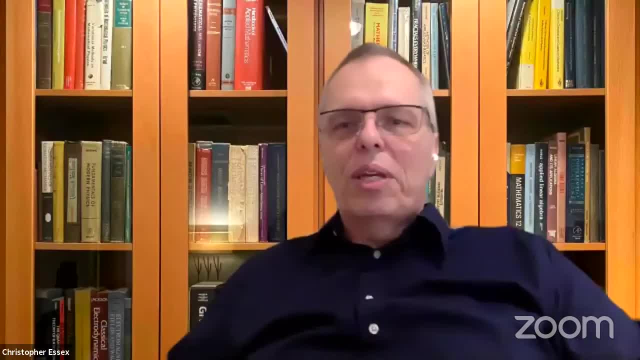 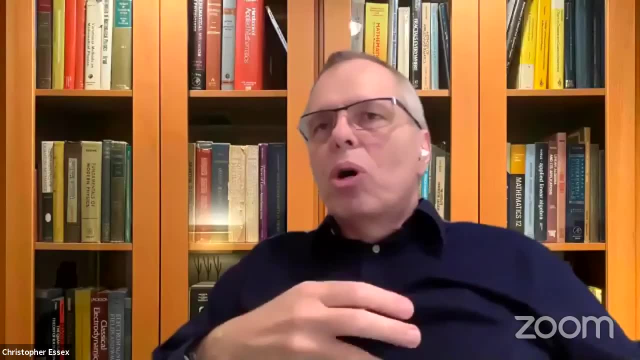 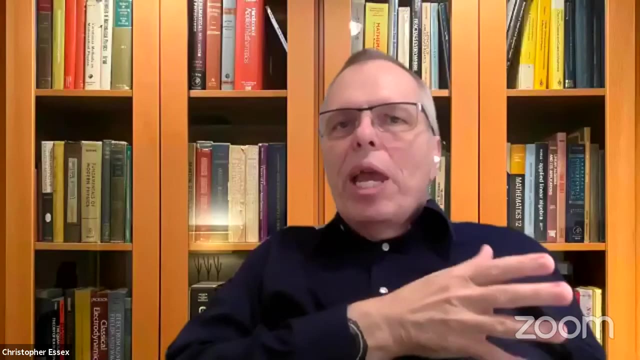 They don't really have really great forecasting skill because they are, in the end, cartoons. And while you might, we might learn something from the models. from a physical point of view, there's academic merit in them In terms of projection, In terms of projecting into the future. they don't have the weight of a meteorological model which constantly is being corrected by how badly they get the weather done. 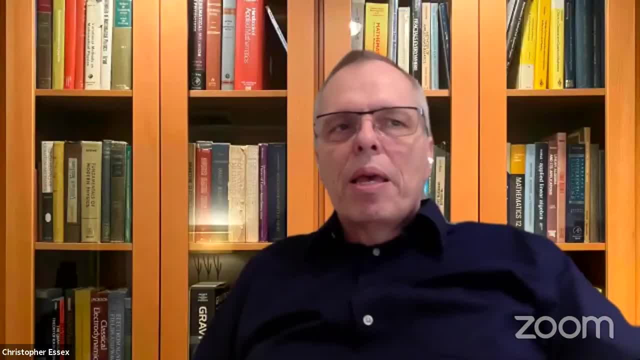 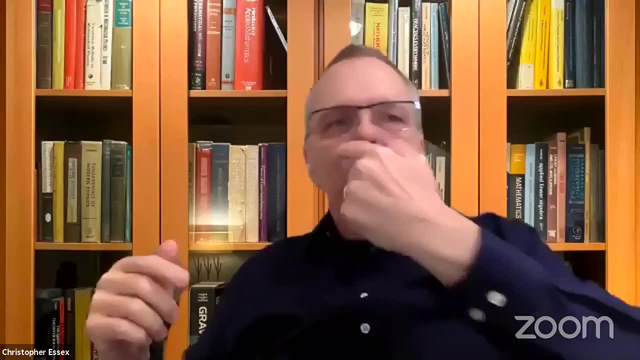 But we only get one shot at climate. We don't know what's going on, And the problem is that someone will say, oh, the climate models got this wrong. You know, if the analogy is? well, there's this cartoon of a face and there's a mustache that's missing. 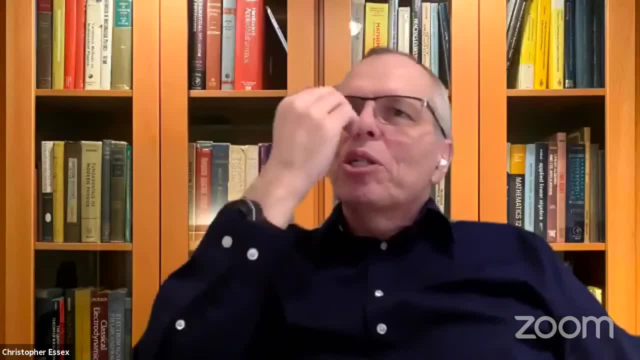 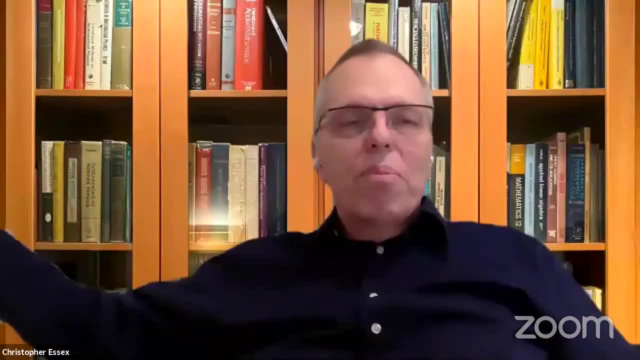 Oh well, we'll bring Leonardo, the modeler, down and we'll bring his paintbrush And he can just paint that mustache, Mathematical mustache, in, And so these models can always be corrected to match what, whatever you see, But that doesn't give them any predictive power. 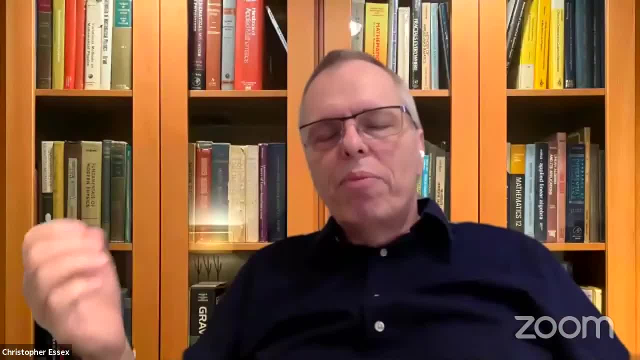 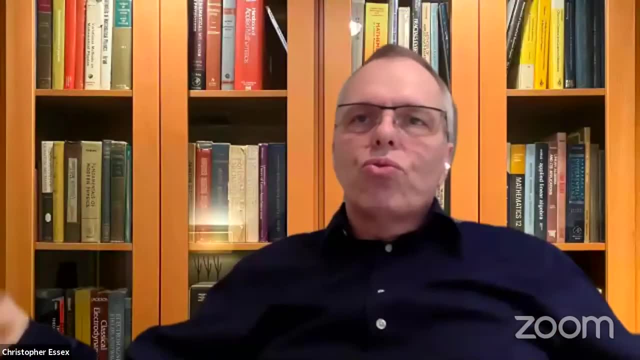 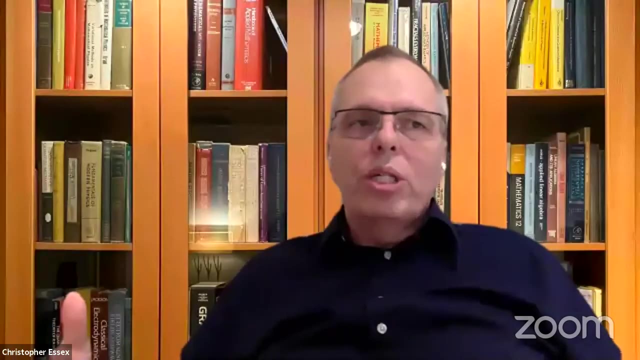 And so in that sense it's not really like theory and experiment in theoretical physics and experimental physics working knit and glove together, because you can't do controlled experiments on this And so you can't exclude other kinds of behaviors being involved. So it's a very different situation. 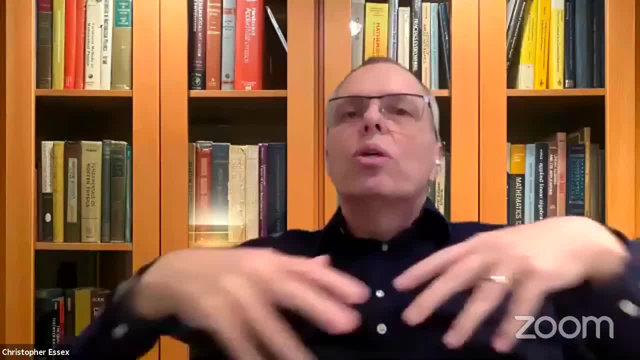 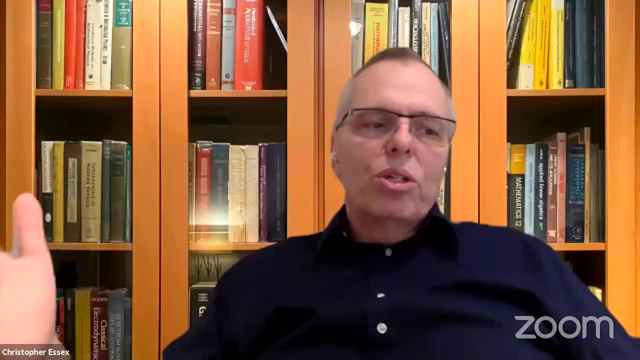 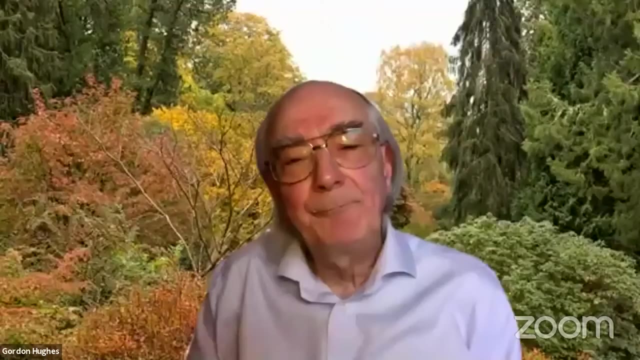 It doesn't mean we don't have to make decisions, but we have to make decisions without full knowledge of what's going on, And there are better ways to do it than others, And we're not doing the good way. Thank you, Gordon. 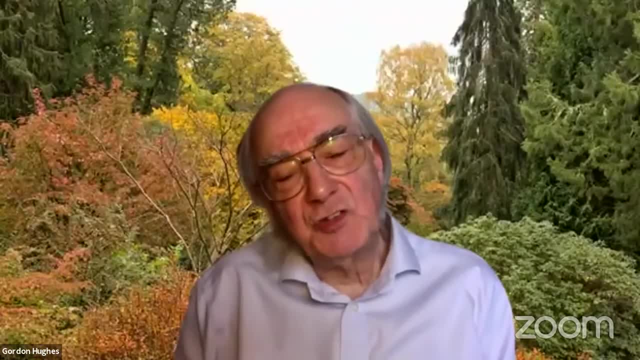 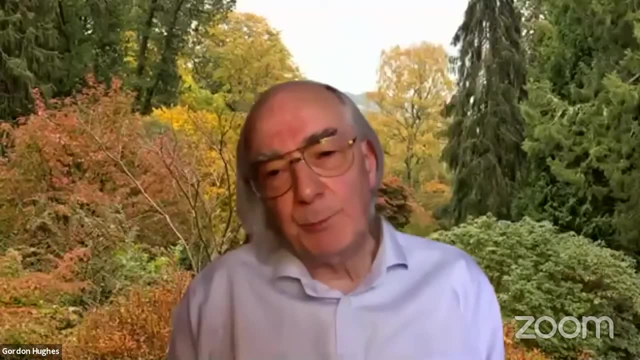 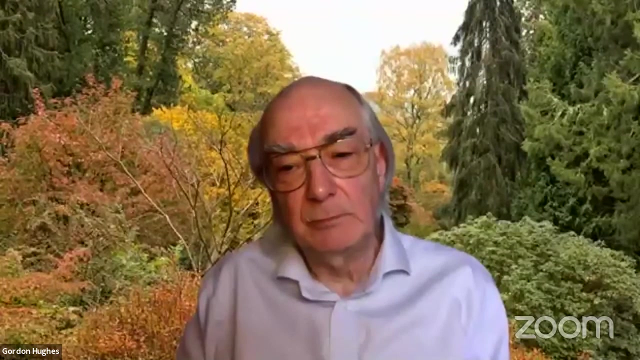 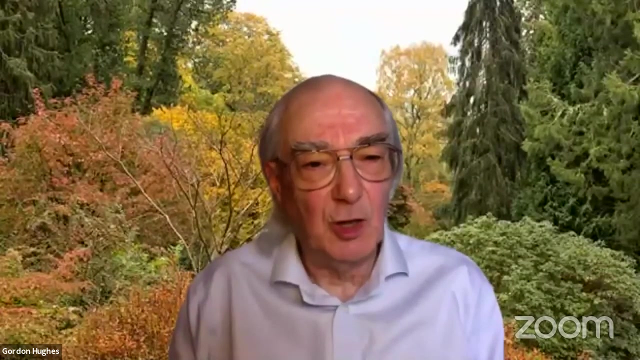 One of the things that I think politicians have done- and they've done themselves great harm by this- Is give the impression That more things are in their control than is in reality the case, In other words, in the past, a century ago, even perhaps 50 or 60 years ago. 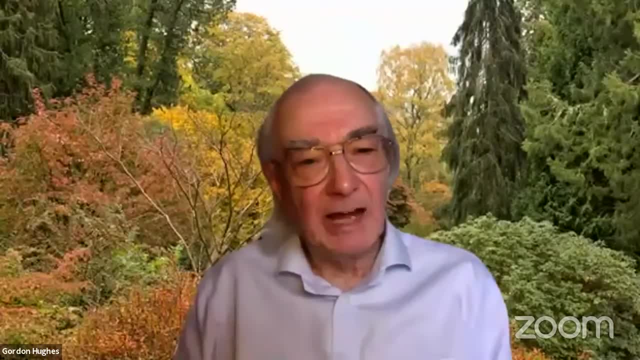 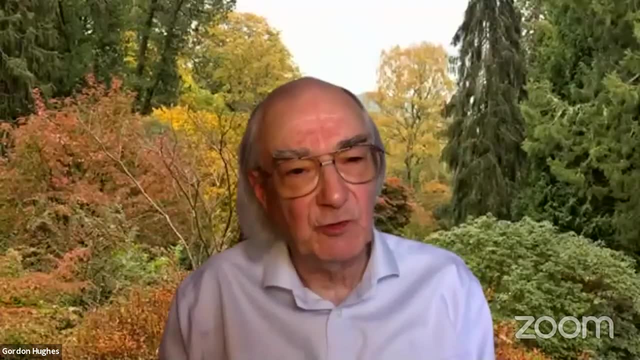 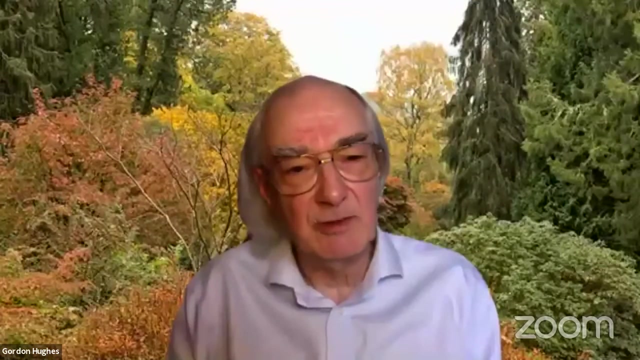 It was not expected that a government could necessarily do very much about a pandemic of the kind that we're experiencing. It certainly wouldn't have been thought that there was a great deal That could be done about climate or about a variety of other things. 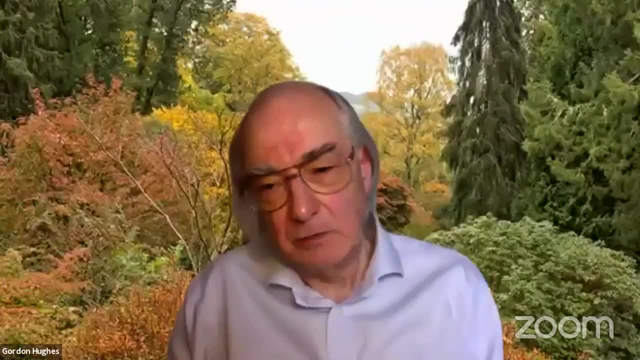 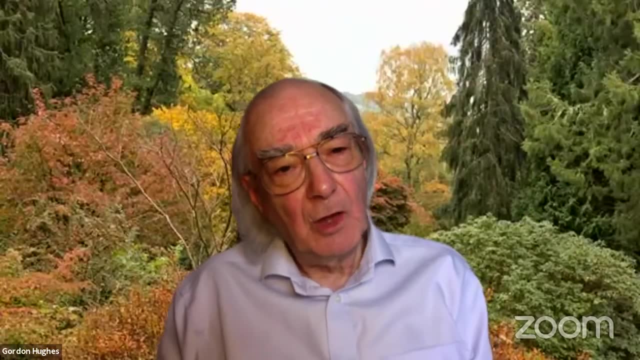 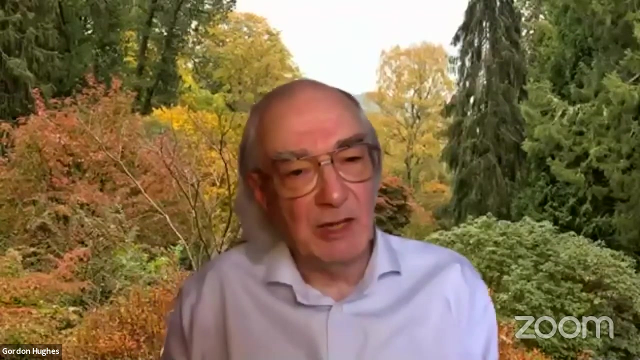 These were in a sense outside the control of action that was likely to be effective And over time. and this has been prompted partly in response to a demand from the population to reduce uncertainty And partly an aggregation of power or at least a claim of power. 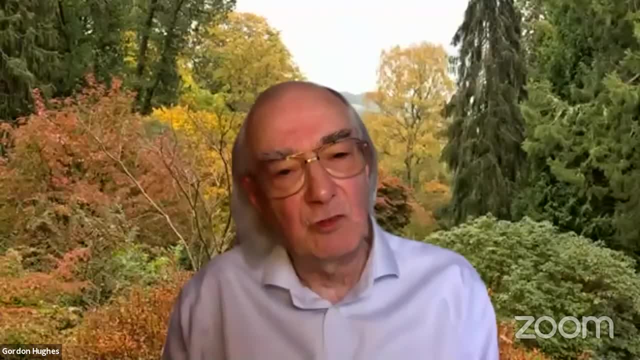 Over the economy and over other things, Which essentially leads to, On the one hand, a claim that something must be done And, on the other hand, a response, for this is something That something may not be much related to what is the real problem, but, on the other hand, 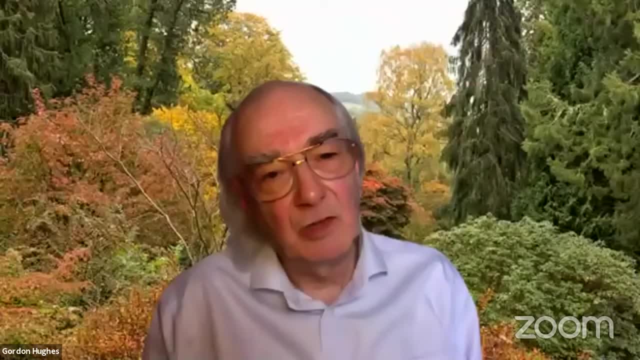 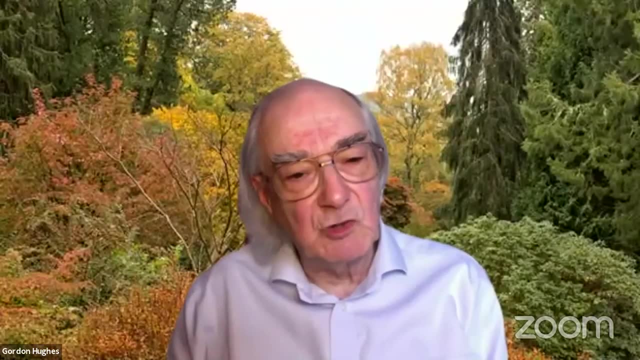 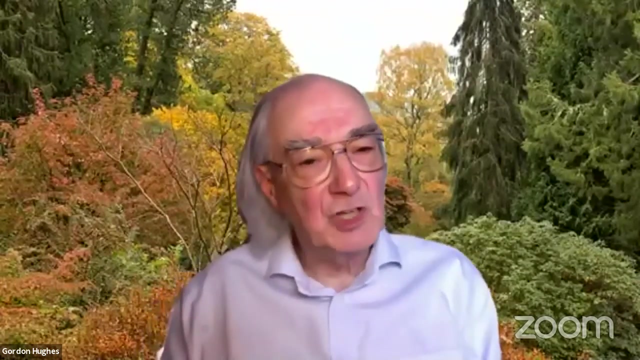 The political establishment is doing things, And I think For politicians a part of the answer has to be: government can do Less than you think, That we can do a certain amount In a certain number of areas, but we can't actually make, in many cases, fundamental differences. 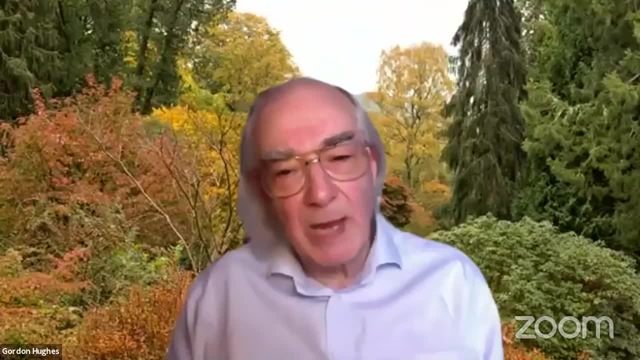 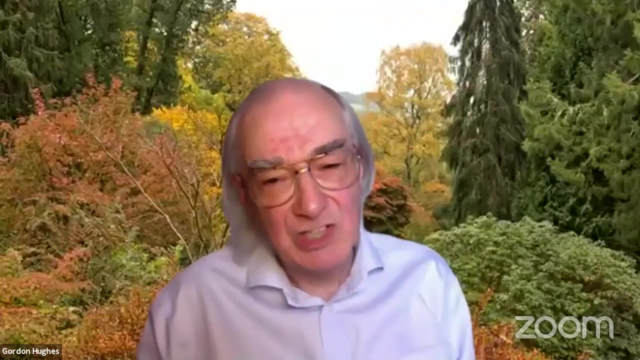 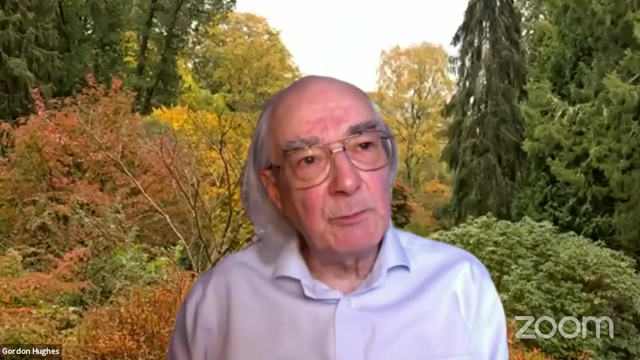 And when we can make fundamental differences, they may be actually catastrophic. In other words, the only tools available to us may be worse than the disease that we're trying to deal with, And that, in a sense, Is a lesson that Economists actually learnt. 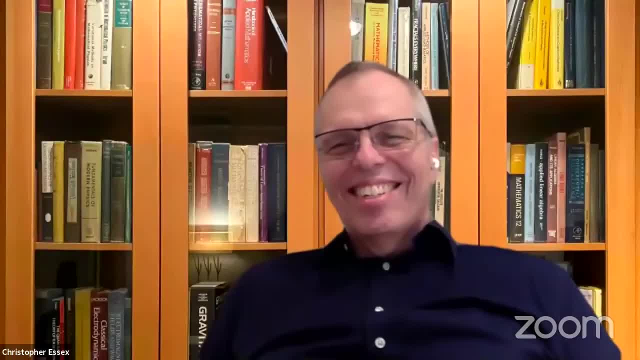 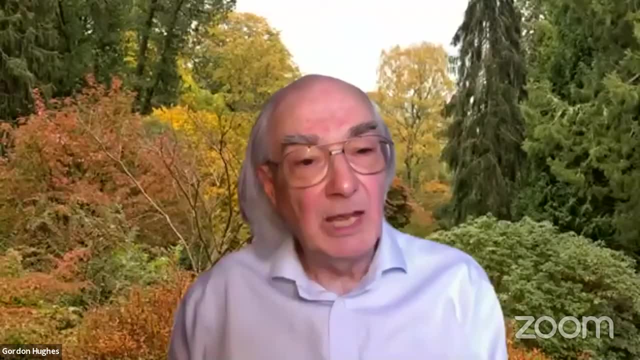 Surprisingly early, Because there was a whole doctrine Of the idea of Keynesian management of economies, of economies In the 1960s and the 1970s, When essentially politicians got the idea that they could fine tune employment By raising public expenditure or by changing interest rates. 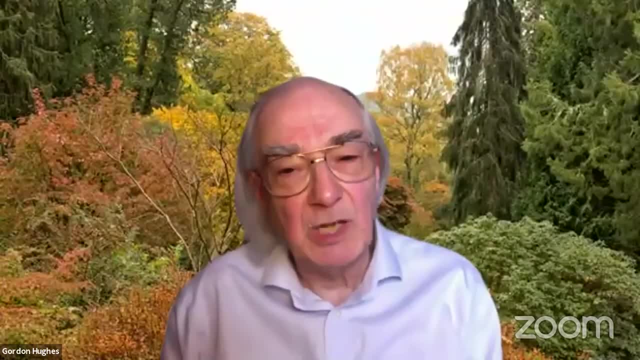 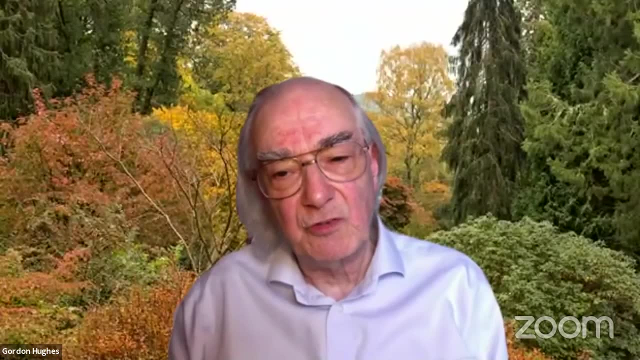 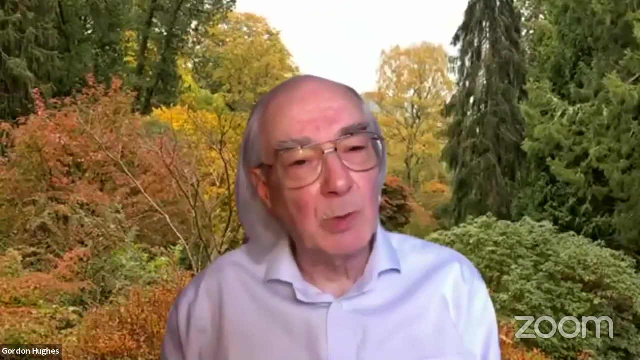 And then gradually it stopped working. And it stopped working Partly because the underlying economies changed And partly Because other things changed in response to those interventions, And economists reached the stage at which they wondered whether really it was possible, in a long-term sense, to change anything fundamental. 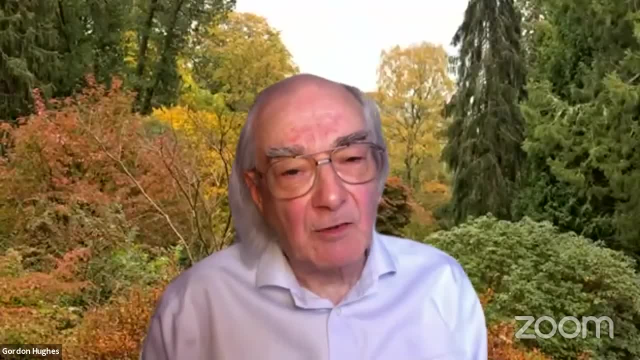 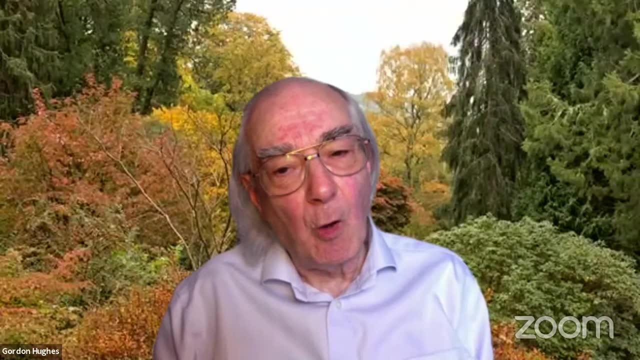 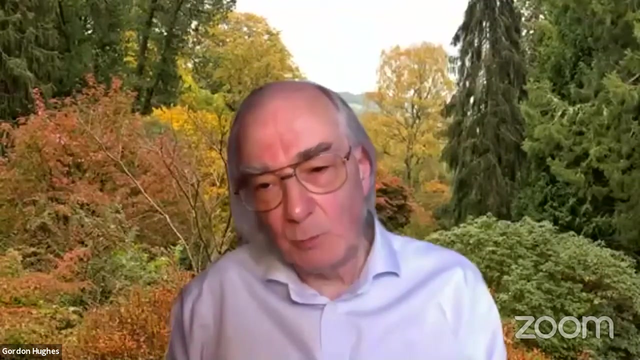 Now The People are very reluctant to reach that conclusion And it's still Heatedly debated, But we are aware On the limitations Of what actually can be done And, in part, what is needed, And this is whether it be. 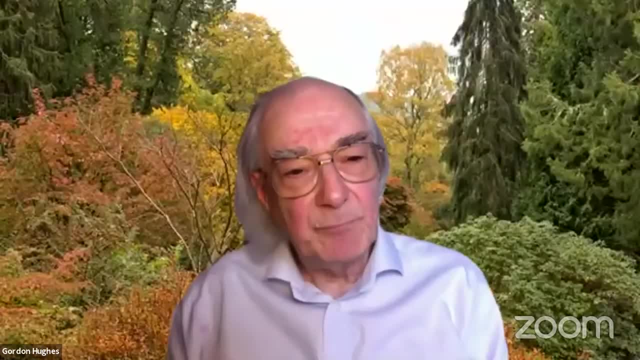 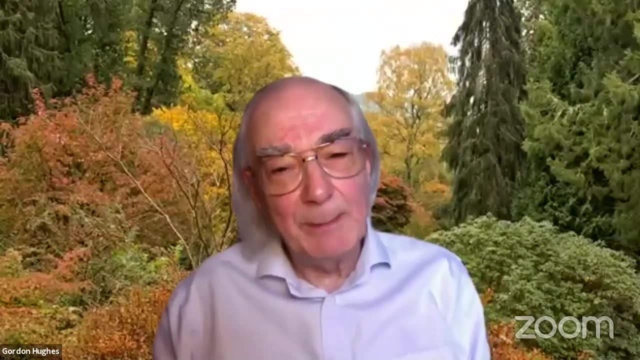 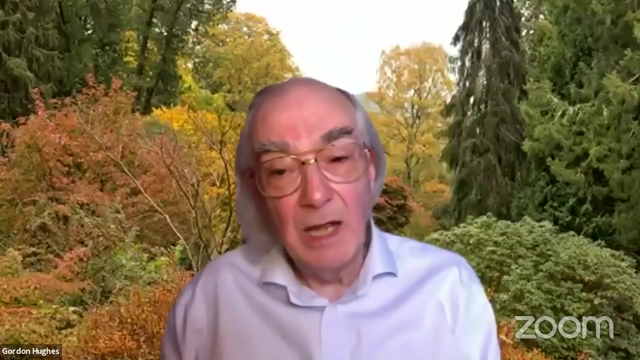 Pandemics or climate or whatever, Is A greater modesty On the part of both governments and The people who put claims on them About what can actually be achieved in any useful Way And that If things can be achieved, 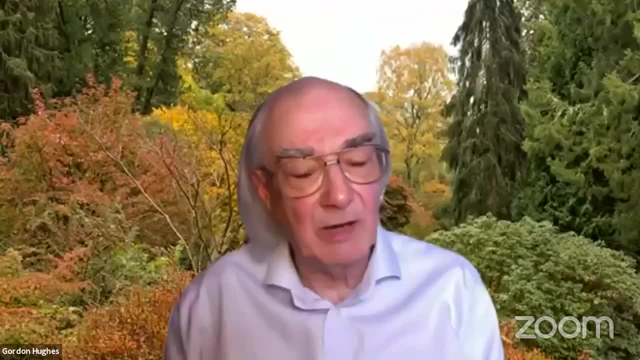 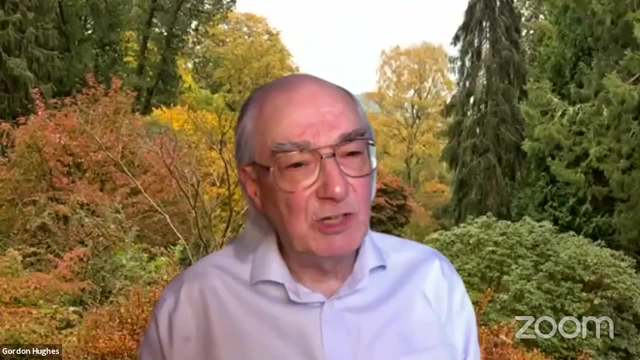 They can typically only be achieved Over a relatively long period of time, By essentially setting The context, The framework, Rather than necessarily, You know- treating the economy Or The population's health As a car that can be steered. 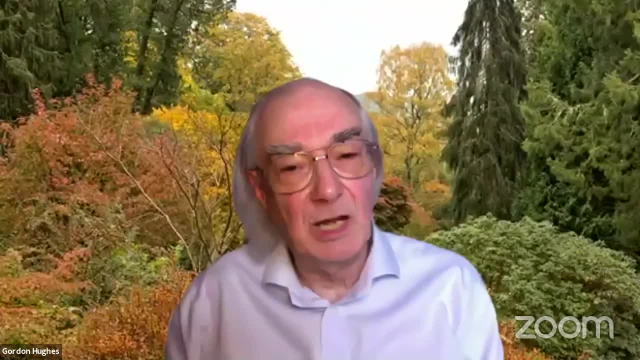 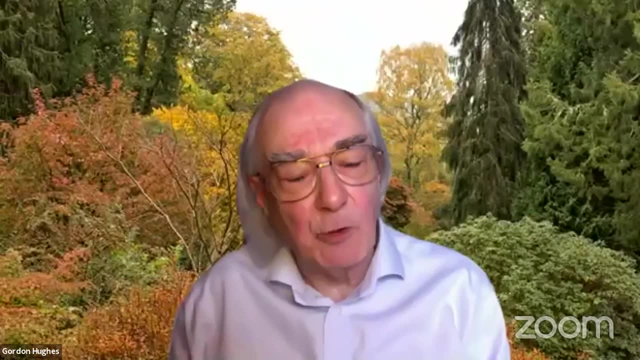 In some Rather conscious way Over time, And the implication of that Is essentially profound In terms of our relationship with The political world As well as the political world's relationship with The rest of us. And that comes back to what I was saying about risk. 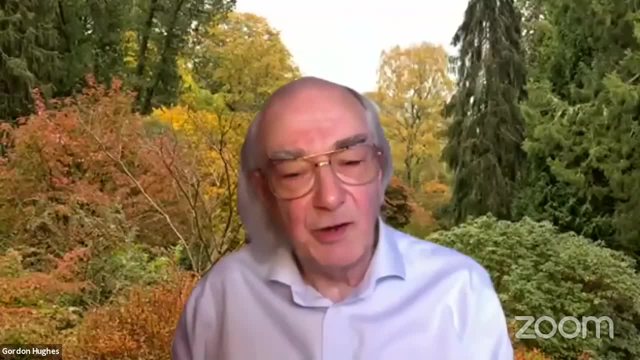 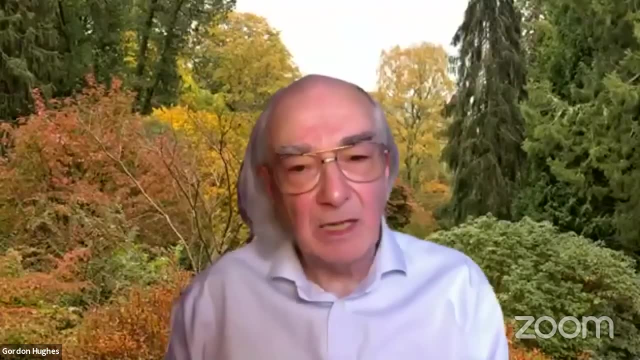 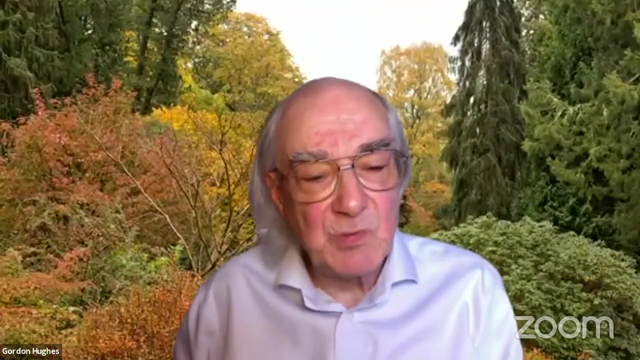 Which is there are all kinds of things That are really outside the control Of The Political Or governmental establishment. The truth of the matter is Put aside. Well, I mean, we've got a pandemic. The pandemic isn't particularly bad. 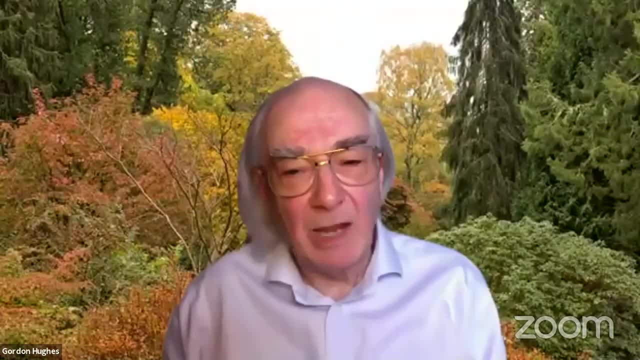 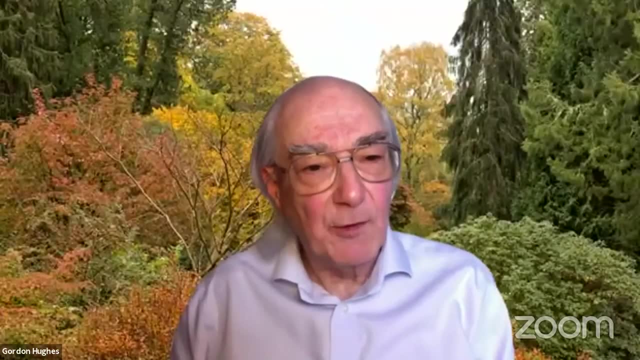 It's on. It's about average For pandemics If you look over A period of a couple of hundred years. And there are Actually a whole lot of other risks Which, In natural, Natural Hazard terms, are considerably worse. 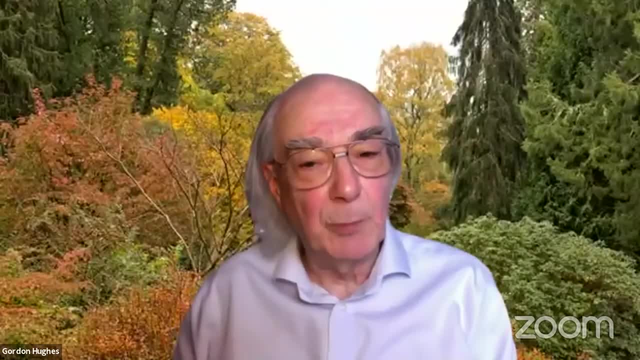 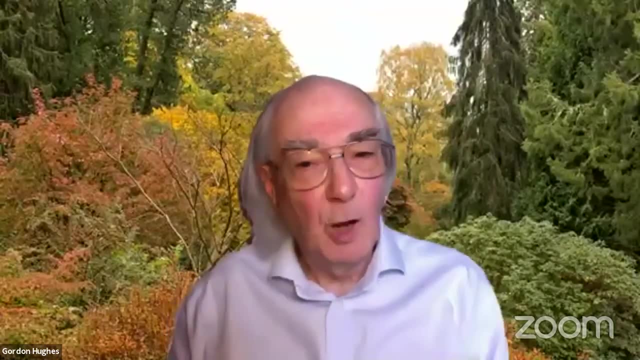 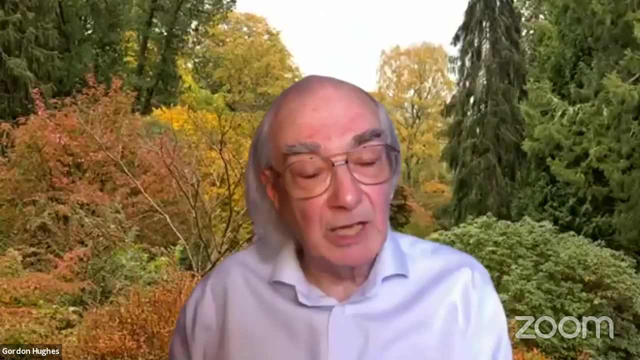 Earthquakes. I mean to take a very simple example: The death toll from the Boxing Day tsunami In what was it? 2004.. I don't remember the exact year, Was greater than The Death toll Around, At least. 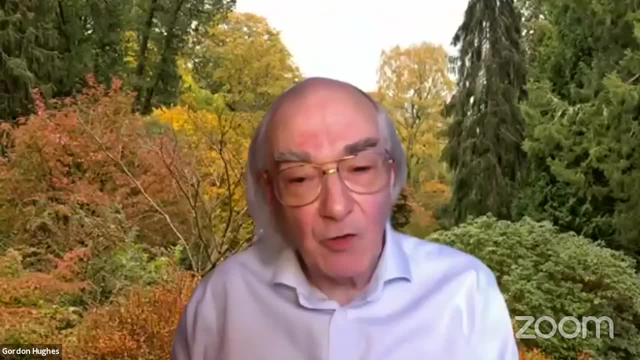 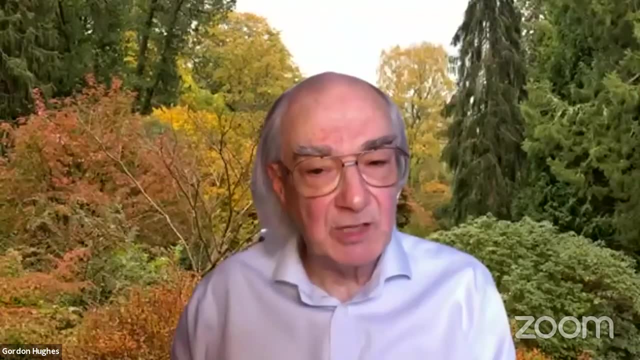 In Asia And most of the world. Now, That was A purely Fortuitous Event, Completely outside The control of governments. We could have done something To mitigate its impact In advance, But the point is: 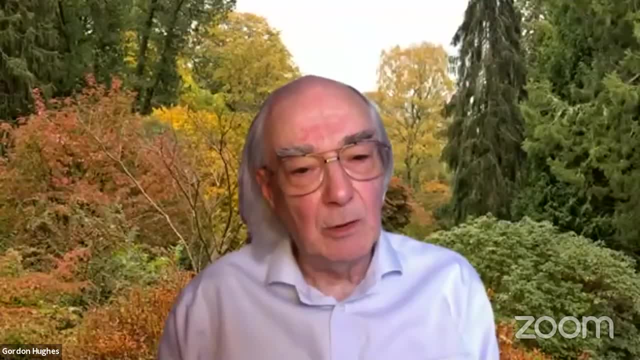 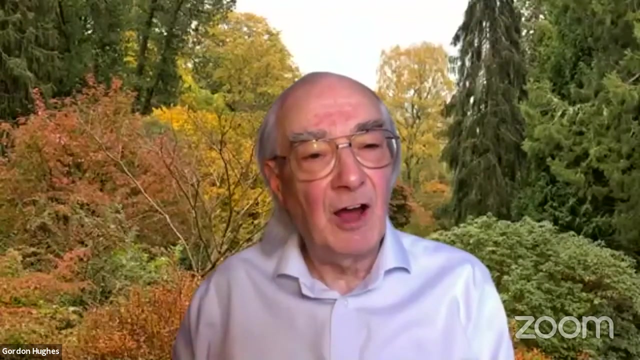 That The world Isn't a certain place And we Really need To learn To live With The uncertainty That is inherent In The world And find Ways Of Dealing With That. 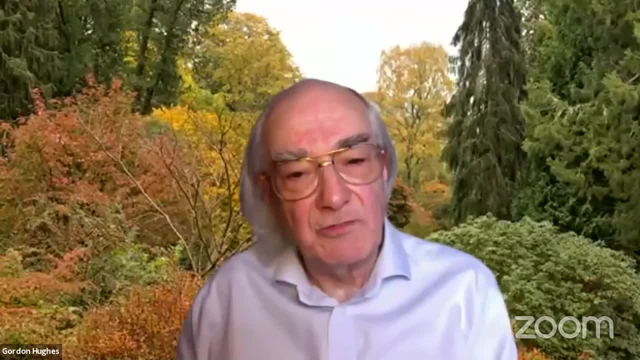 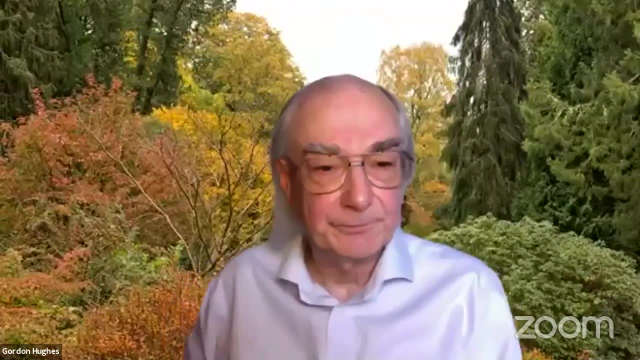 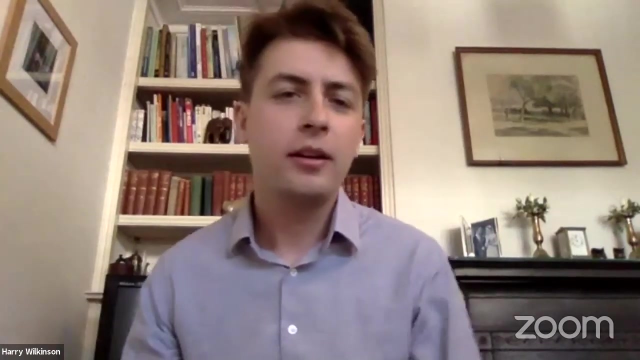 Rather than Simply Find Demanding That, Essentially, Governments Spend All Of Their Time Either Responding Or, Indeed, Preventing Things That Probably They Can Do Not. Very Much And They Don't Have The Courage Of Their Convictions To Follow Their Own Policies And To Analyze The Evidence Themselves Or 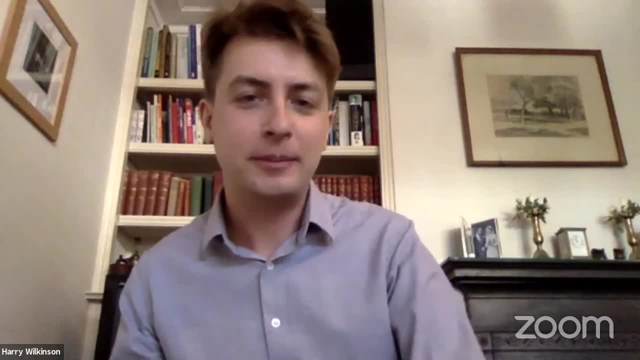 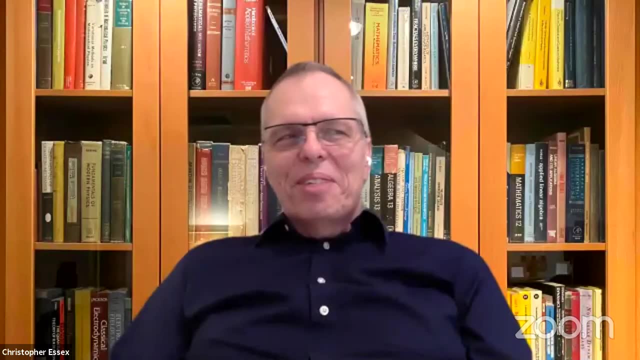 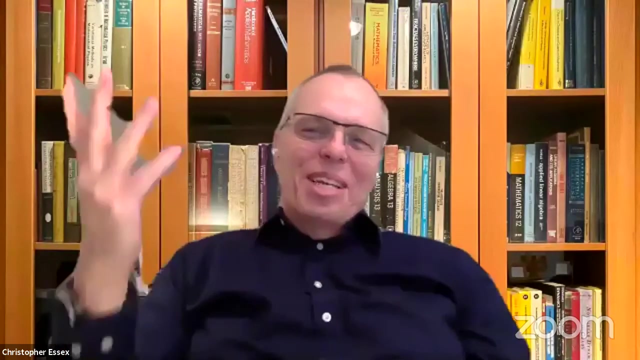 Is It Instead The Problem That Politicians Are Determining The Science? I Love It. It's Really Almost A Single Word. Now, It's Not The. 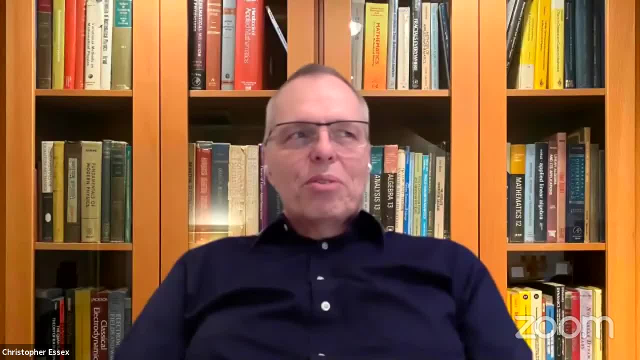 Science, But The Science Right. So Maybe Hyphenated, But I Don't Know What They're Following. That's Exactly What Scientists Are Supposed To Do. 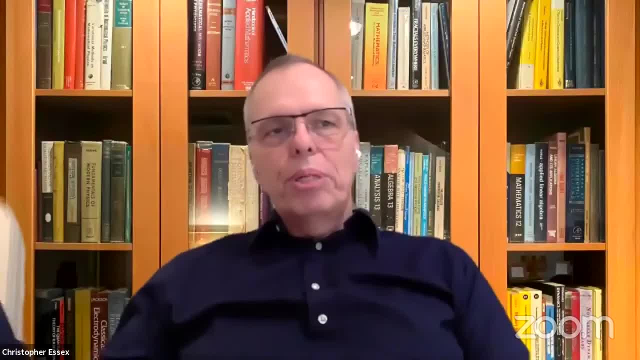 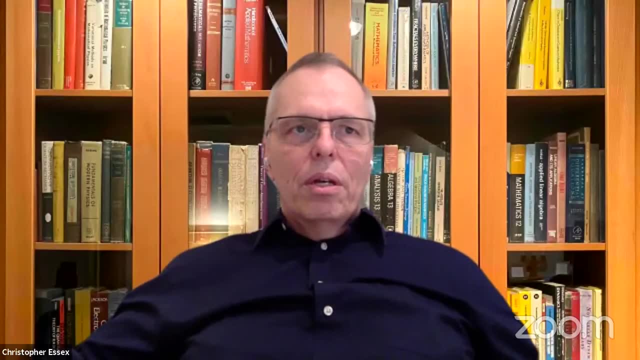 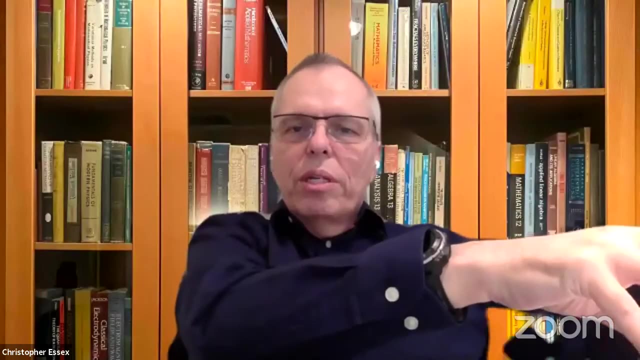 Right. So Even Though I'm Officially An Expert, I'm Quite Happy If People Are Skeptical. That's The. That's What You're Supposed. 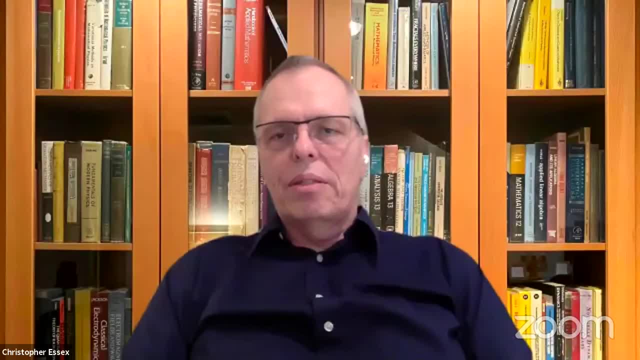 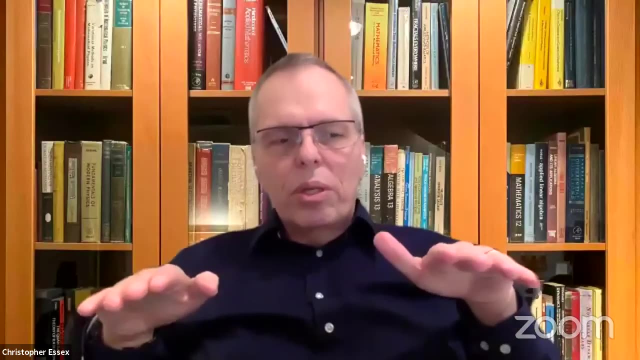 At All. You're Supposed To Be Questioning Things. That's. That's What It's All About As Far As Governments Losing Their Confidence And So. 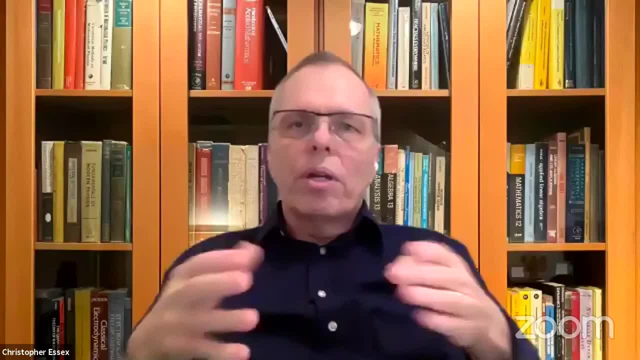 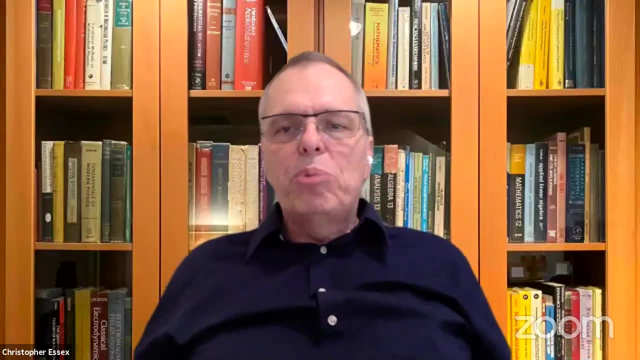 Forth. Well, You Know, I These All Of Those Holes Down. You're Going Down The Rabbit Hole Very, Very Deeply. These Are Very Deep. 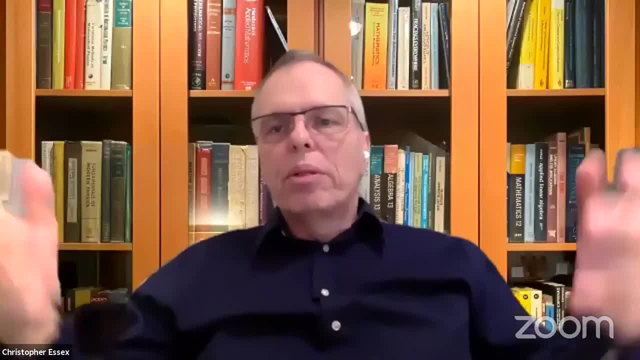 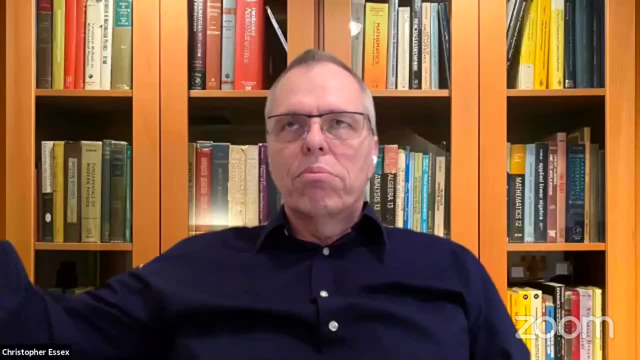 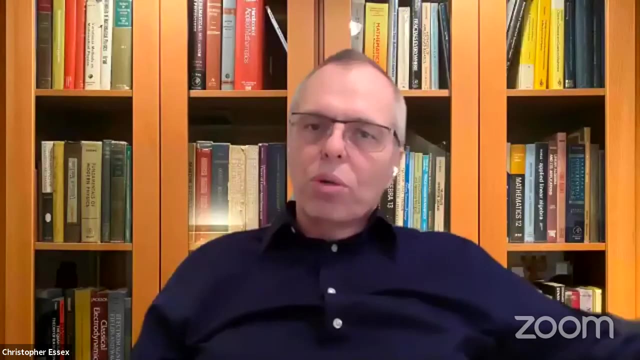 Scientific Problems, And They're Sort Of Magically Waved Away Into Being A Solid For Just Some Data. It So Most Of Those Needs. Finally, 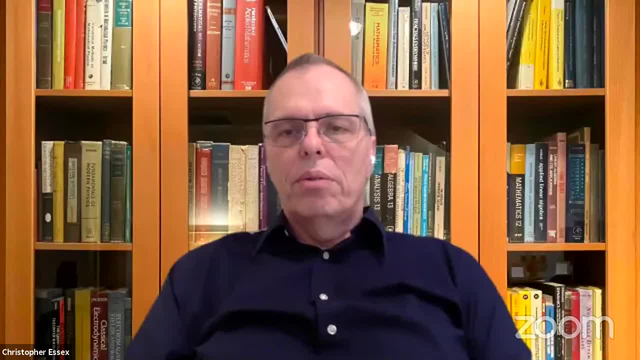 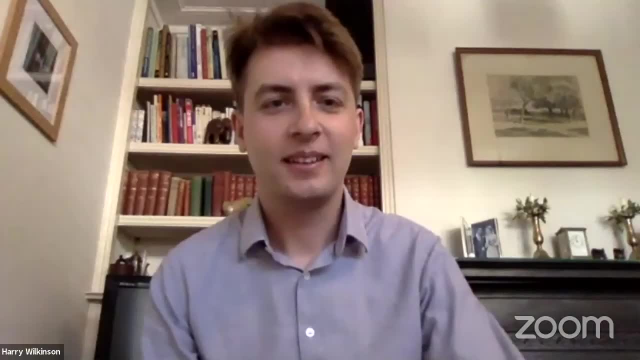 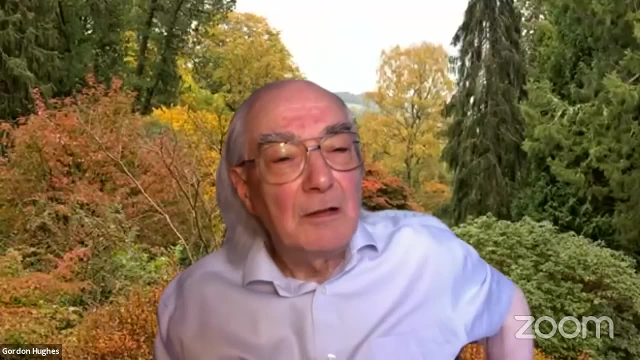 Be To Maintain That Equality, That That We Do Have To Maintain, That Then Be Normal. first of all, the science tells you nothing. There isn't any such thing as, as it were, 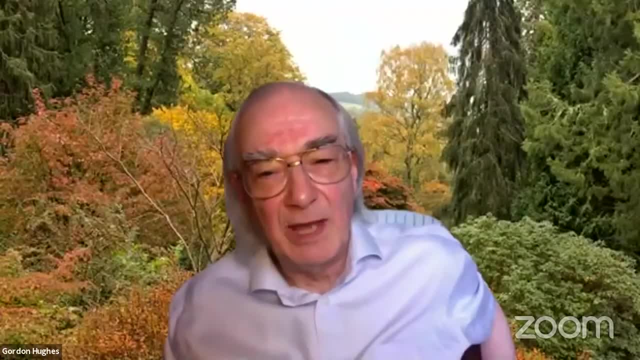 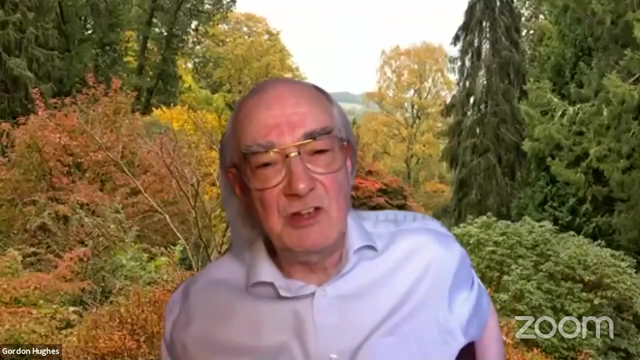 settled conclusions from science. Science, in the end, is a method. It's a frame of mind and a method of collecting and interpreting and building on evidence. What actually politicians are doing when they claim that they are following the science is essentially disclaiming their 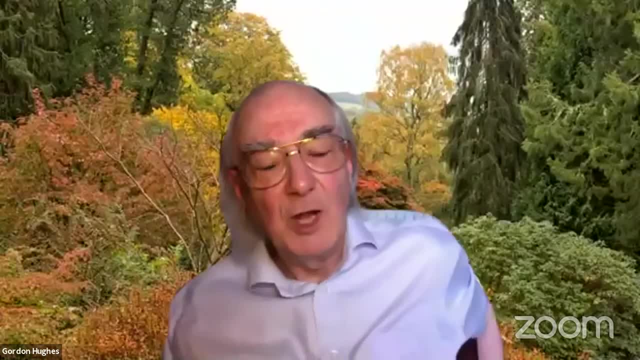 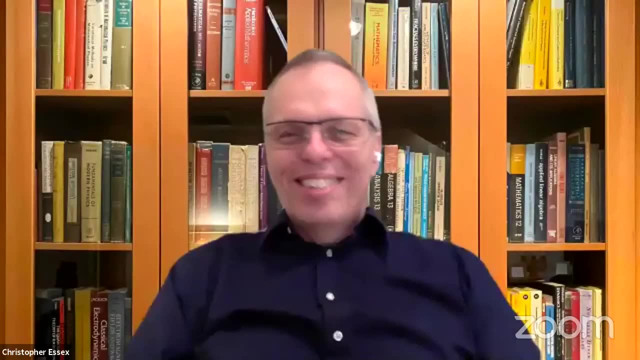 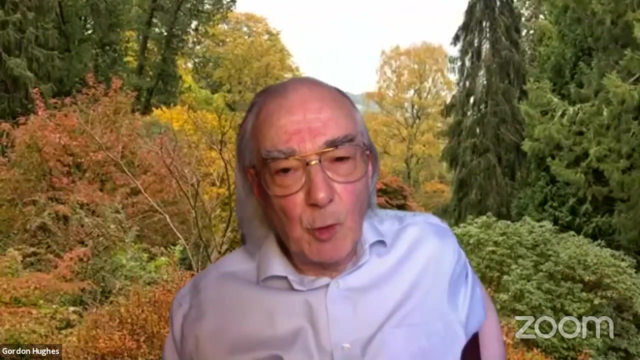 responsibility for it. They are, in effect, trying to say: oh well, this isn't very pleasant, but I didn't. you know, I'm not responsible for it, The devil made me do it. Yes, And I think to go a bit further about that. I think that the core problem is that scientists all too often allow. 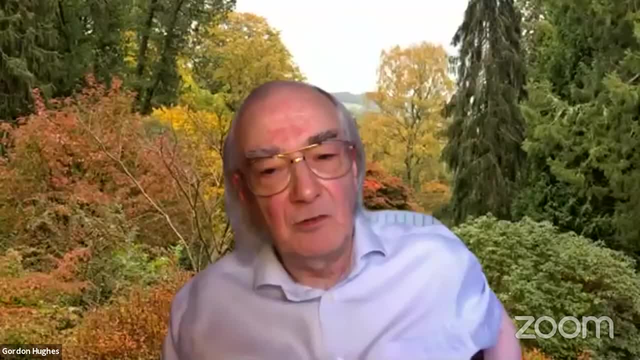 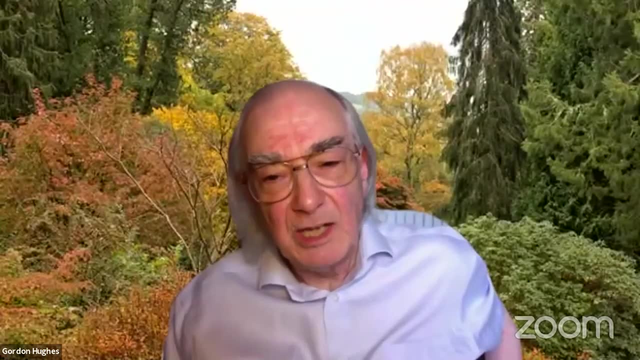 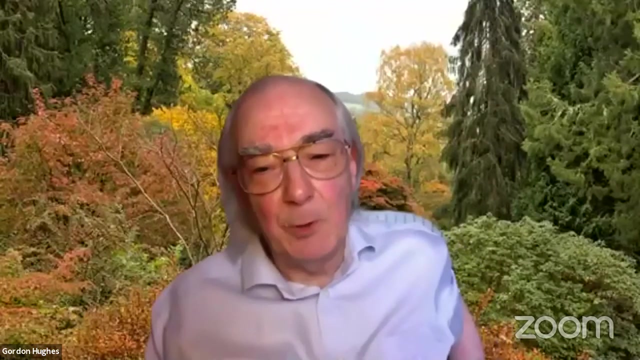 their own views about what the right thing to do is, to intrude in the advice and the science that they allegedly you know, that they claim is settled. So, in other words, we have, on the one hand, science people who want to become policymakers and politicians who don't want to. 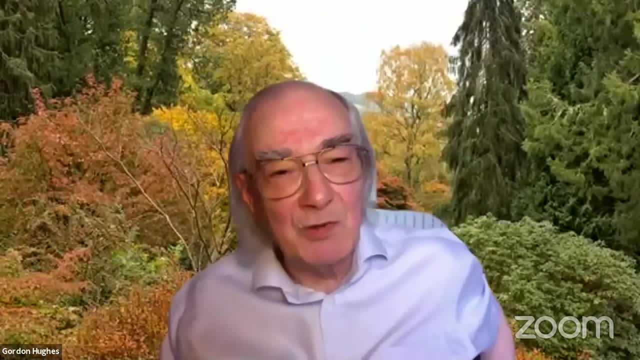 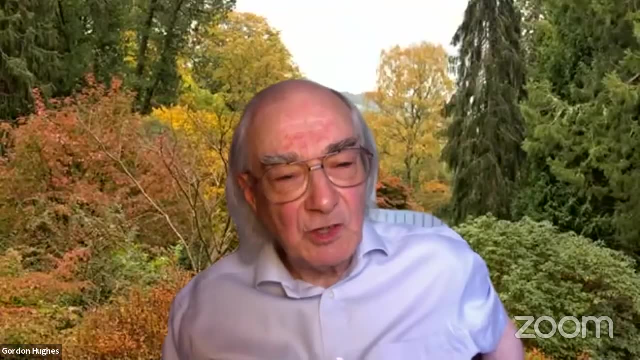 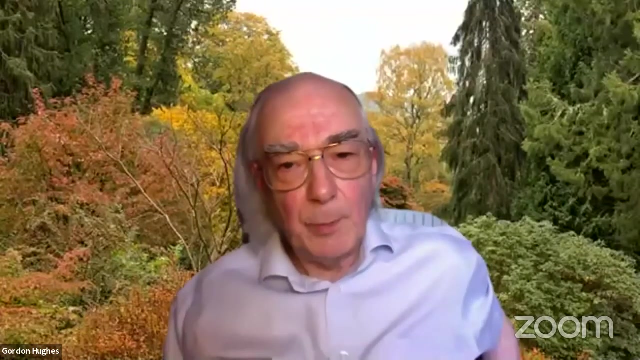 be policymakers, And the outcome is almost bound to be unsatisfactory in terms of the result. Now, I think the problem I mean- again, Chris has emphasized the role of incomplete information, The the other thing, I think, is that politicians fear being held responsible for things over which they 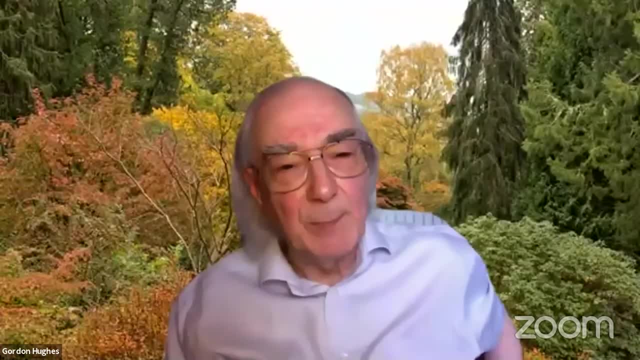 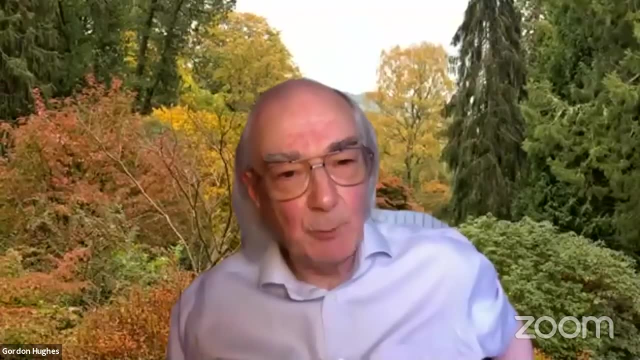 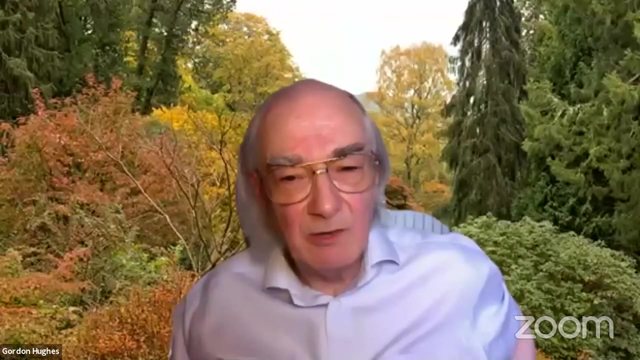 don't have a real control And therefore they're going to be blamed for outcomes which they couldn't control. Now, my view to that, and that's based on my own experience, is that's life, In other words, that essentially, as I said about my experience in Russia, 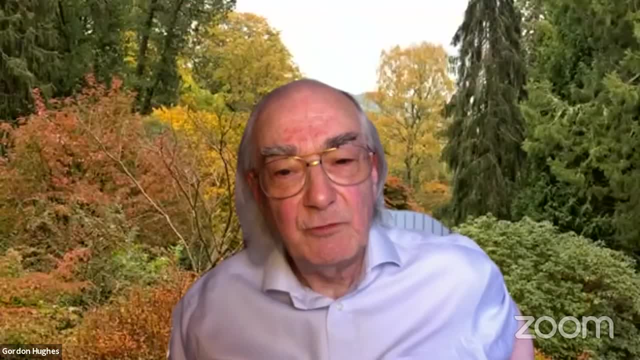 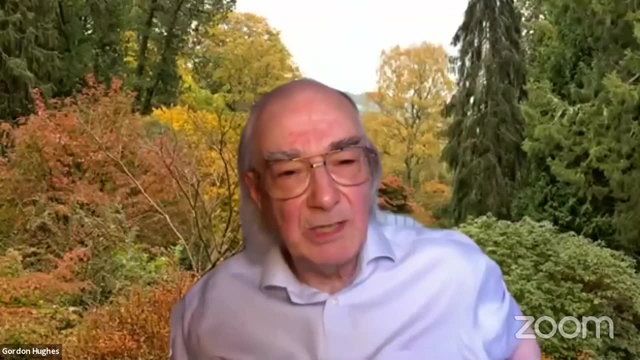 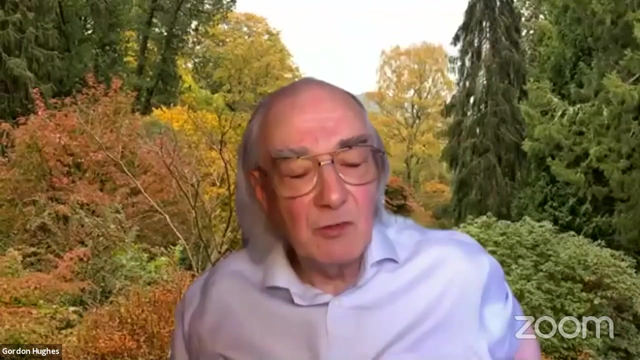 when he came down to it, none of the politicians survived. It has significant political forces after the events because they inevitably did get blamed for it, just as we, as advisors, got blamed for it and still are blamed for it. But the problem is: 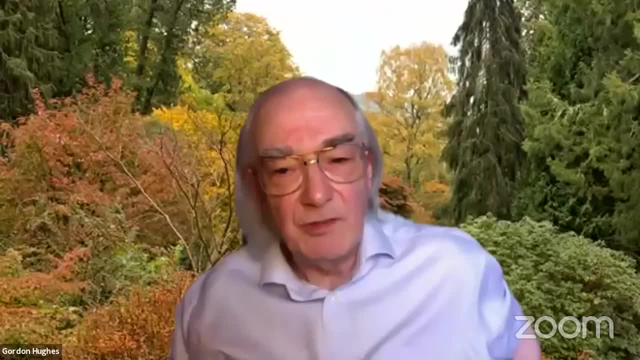 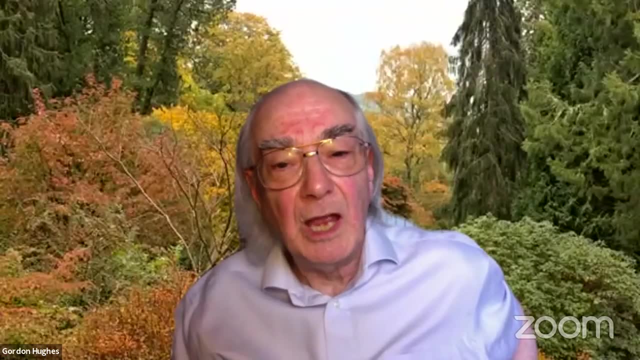 that you just have to live with that and do the things that seem right on the evidence that is available and stop, as it were, trying to protect your future career. And I think the trouble is no politician is going to ever find it easy to do that. 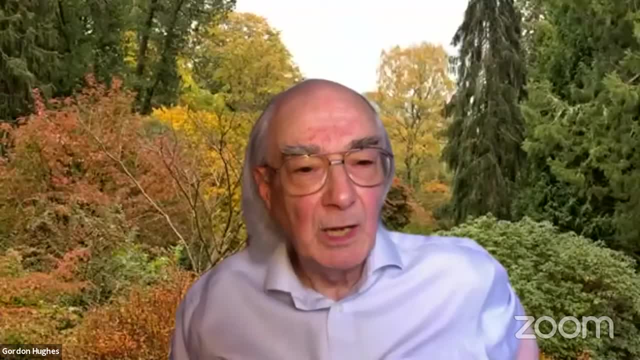 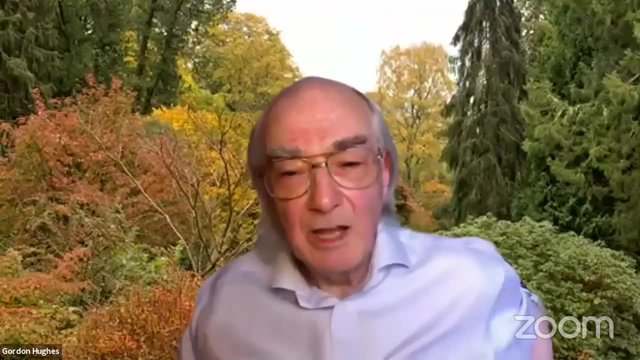 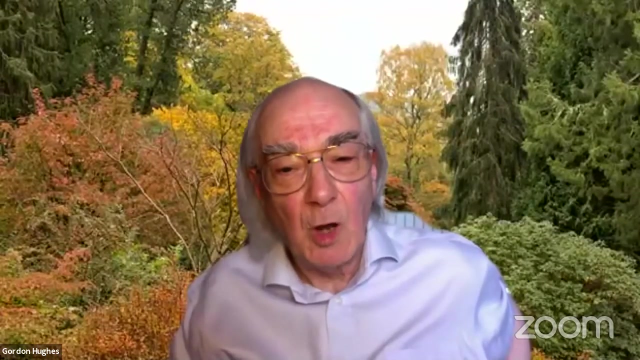 And to reconcile themselves as they should. I mean the group of politicians in the UK and so forth. I mean, in my view, their careers are over. I mean, you know, there is no way out of having had to take the steps they did, whether they were right or wrong. Ultimately they're going to 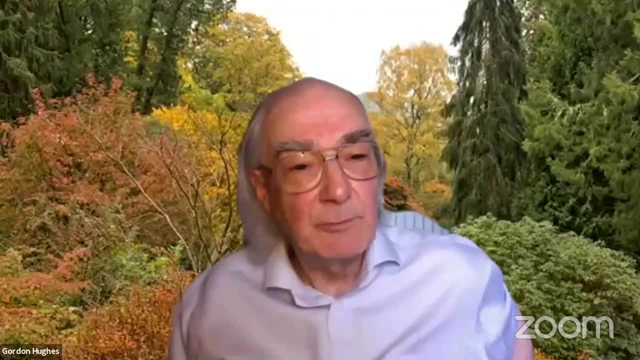 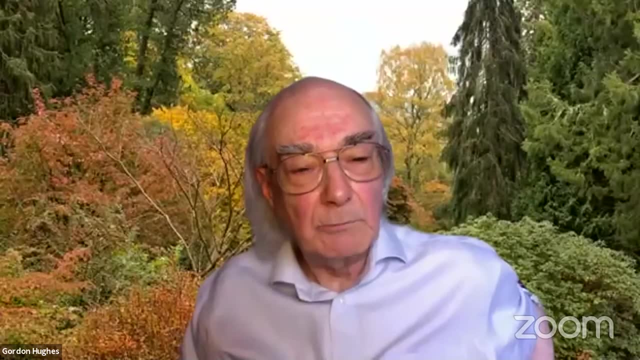 be blamed for it And they won't recover from that. And the problem is, once you've accepted that and can live with it, then you get on doing with what seems the best thing to do, subject to the best advice, and you don't worry about defending. 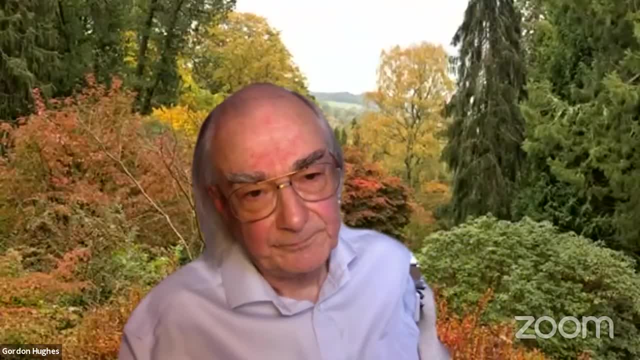 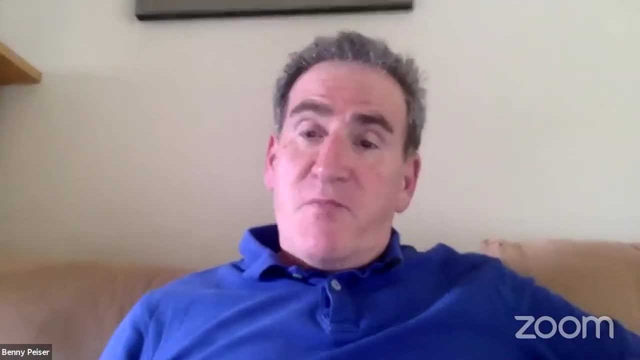 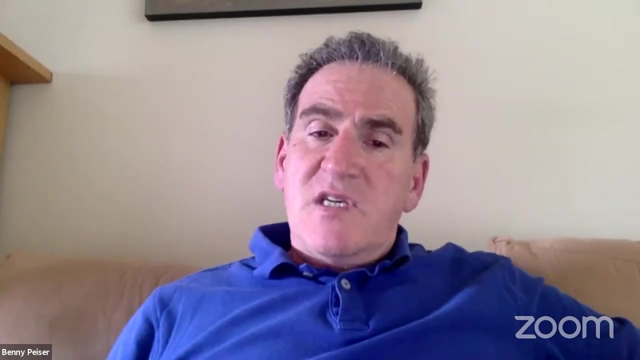 yourself all of the time. thank you, uh, benny. yeah, i, i'm afraid i think it's much worse, with both scientists, the scientific organizations and governments. the- the scientists, in many ways have only to blame themselves for becoming far too political, far too much campaigning. scientific organizations over the last 10-15 years have bombarded ministers, governments around the 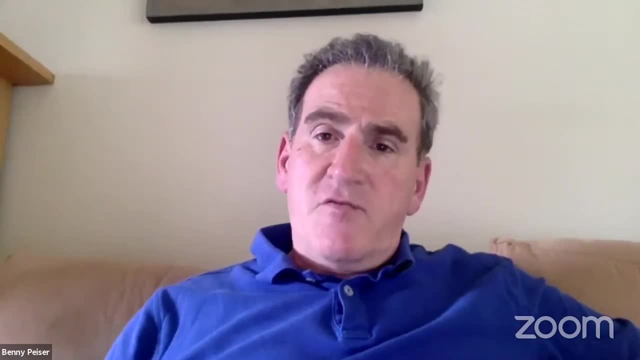 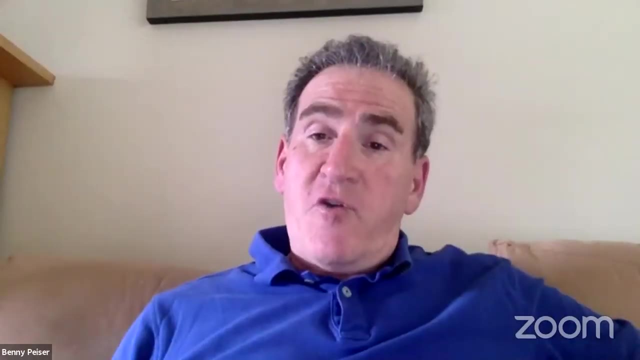 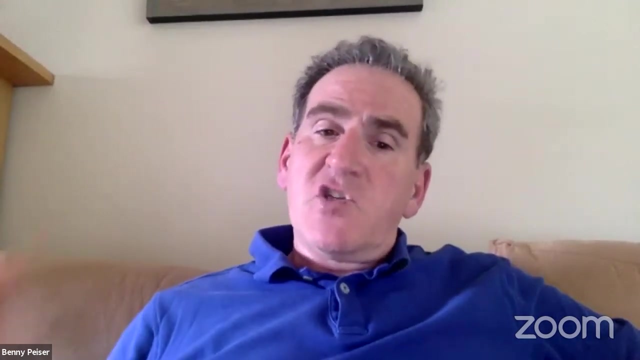 world, for you have to follow the science, you have to follow what we are telling you. if you do not- codependency, you do not follow what we are telling you, you're a denier and we will make sure that voters know that you're a denier. so the scientists have become extremely politicized. we know from: 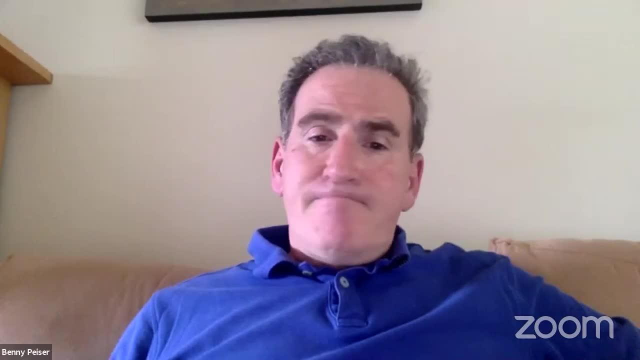 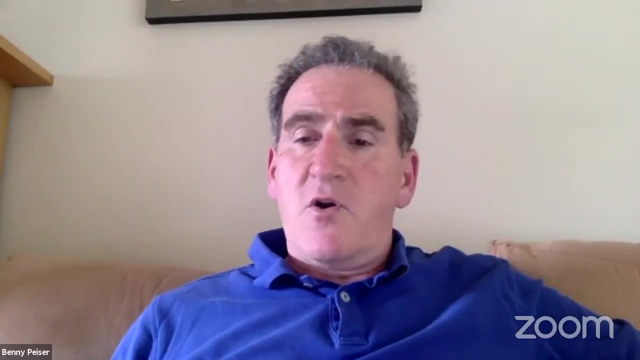 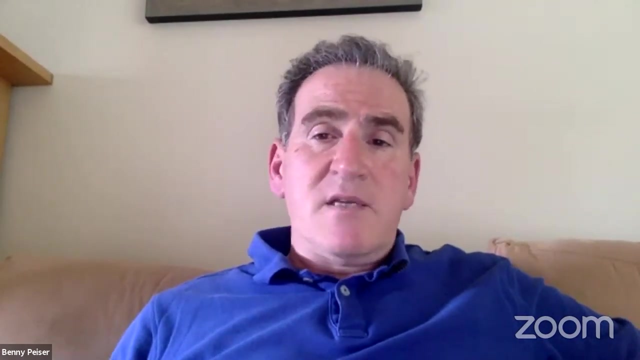 surveys around the world that on average um 60, 70, sometimes 80 percent of academics are left-wing. very few conservative scientists left in this world. sometimes you wonder whether scientific advisors will have to be selected not on their expertise but on their political outlook, because in a political in 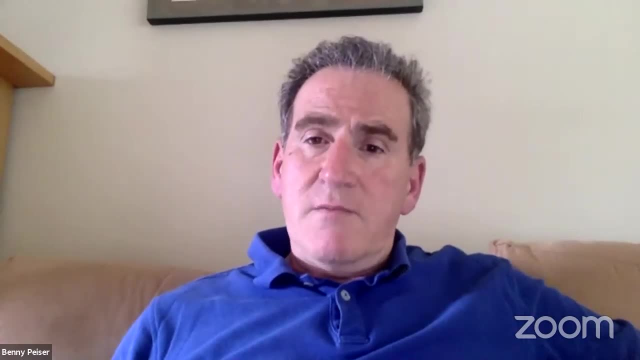 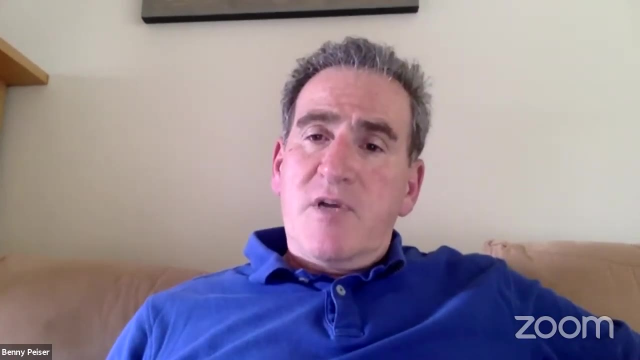 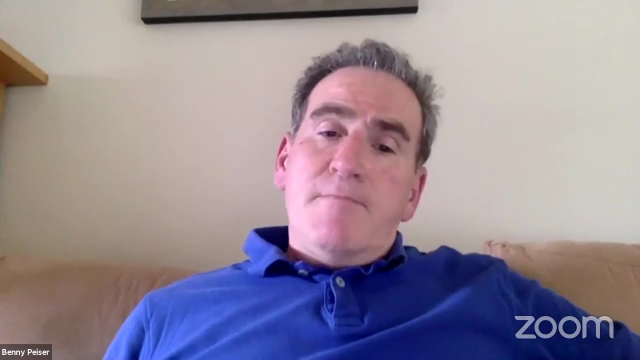 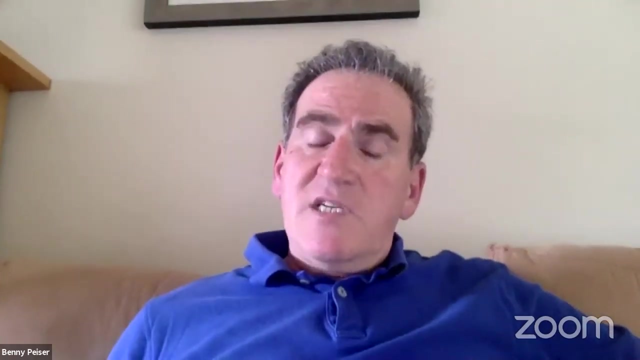 in a highly polarized society, if you have scientific advisors who are extremely opposed to government, the governments they advise, they will be not able to actually function properly. um sorry, my dog is just running crazy, so i i really think, uh, scientific institutions are just as much to blame and the gordon and 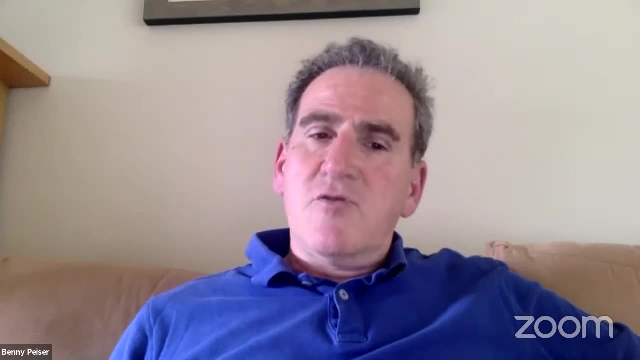 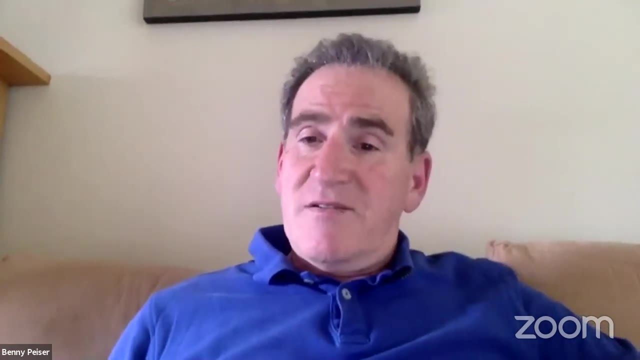 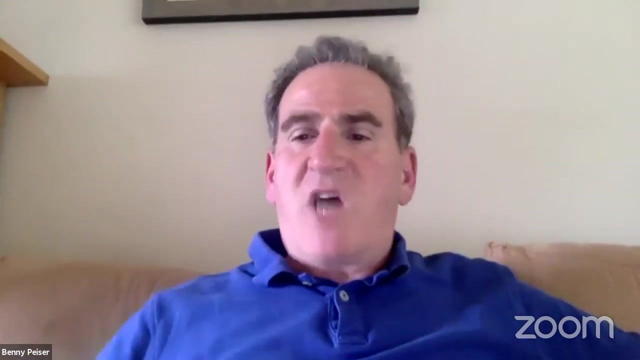 chris are right in saying that the ministers are trying to say: well, it's not our decision, it's a scientist. however, they also know that if they go against these scientists, they, the scientists, will run to the guardian and say, ministers, doesn't accept science, the signs. then the government. 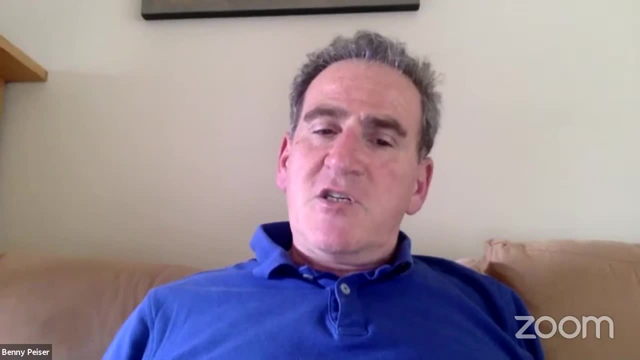 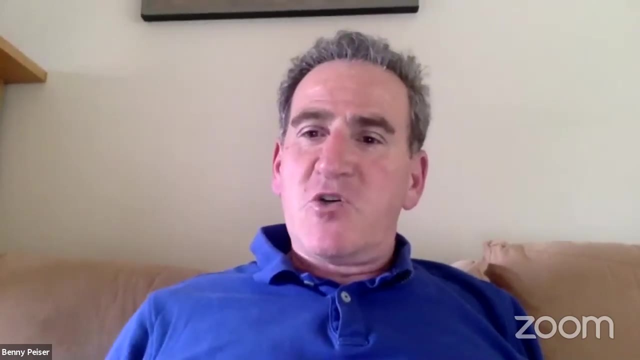 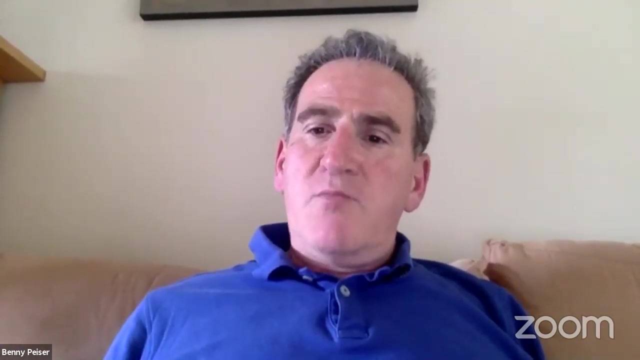 doesn't accept the science. so the, the, the politicians are in a hard place, because if they don't follow the science, they will sure the guardian and the bbc will make sure that they are sure that they are exposed as science deniers. so it's that is another reason why it's so important. 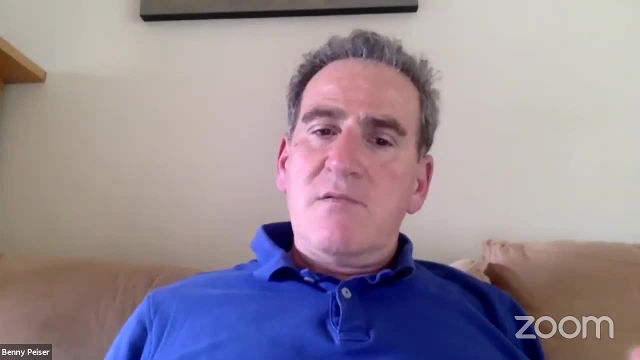 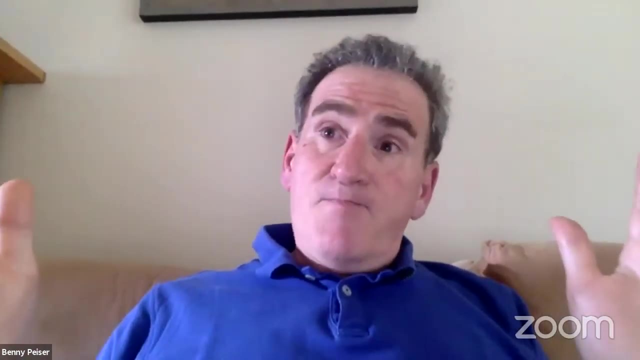 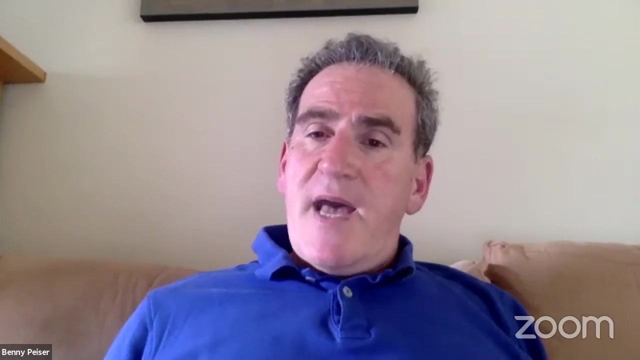 to have a broad spectrum of views in scientific advisory organizations so that ministers actually get the broad spectrum and can then assess the, you know the, the the spectrum of of uh views and weigh up the different uh views. but the scientific institutes, institutions, made the mistake, in my view, in telling governments that the science today means. 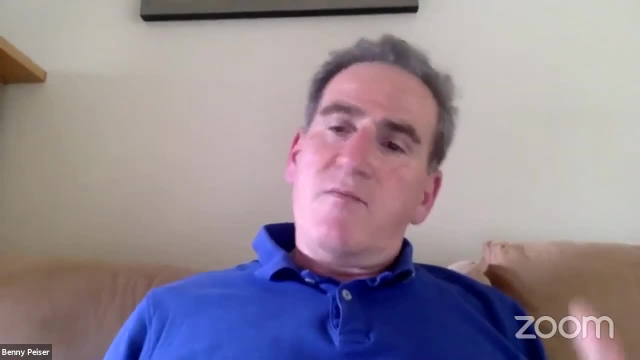 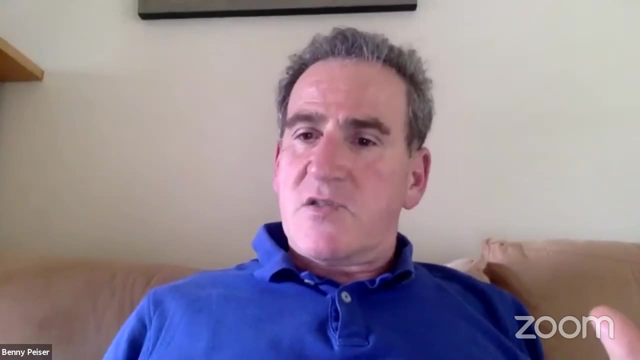 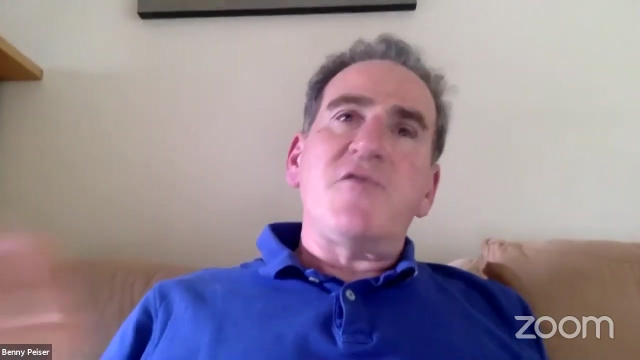 that only. what is the kind of consensus view, and what is consensus view in today's world of science? the majority view. wherever there's a majority, that's the science. that's how scientific organizations are portraying science. the majority of scientists believe this. so therefore, this must be the truth, because it's a 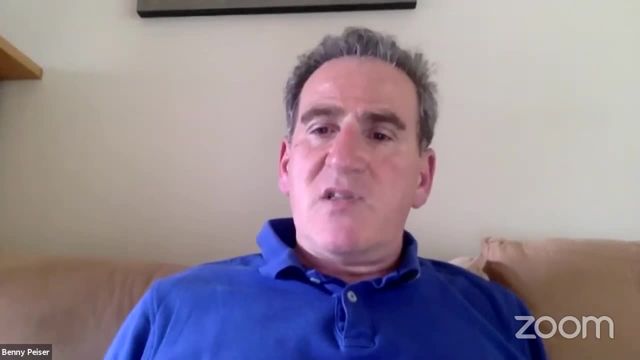 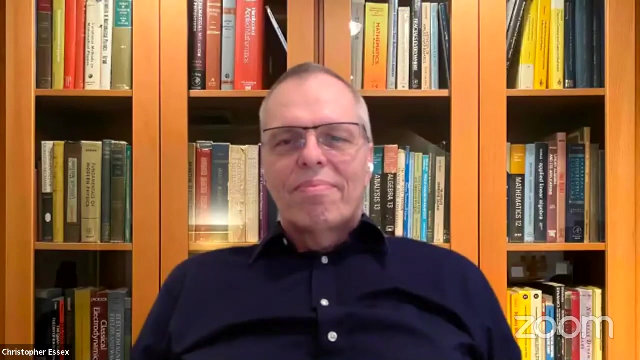 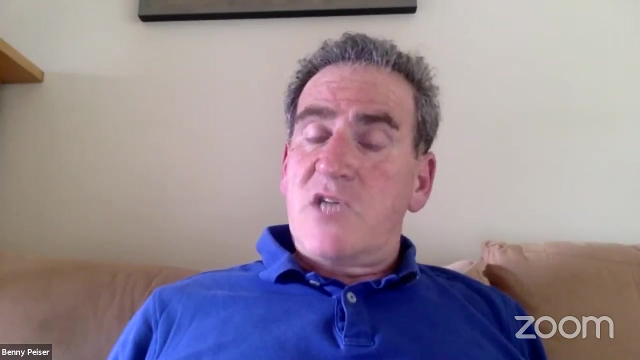 majority. i mean, that's the way people understand science, because the scientific institutions and organizations have told ministers that they know that the majority is right and and and anyone dissenting from majority view did not be included in any advisory role and shouldn't should be essentially, uh, shut down and and and silenced. and because of that crisis in scientific 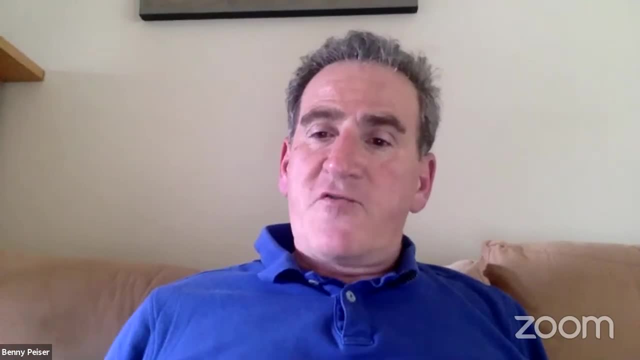 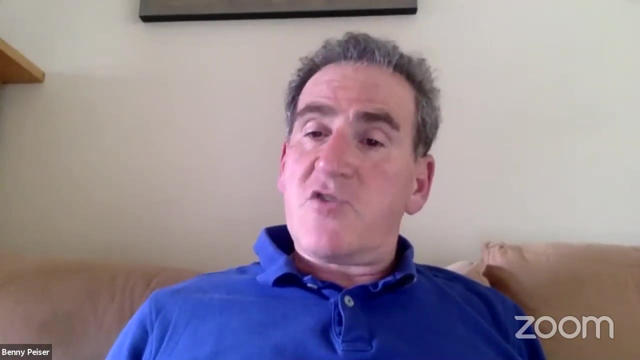 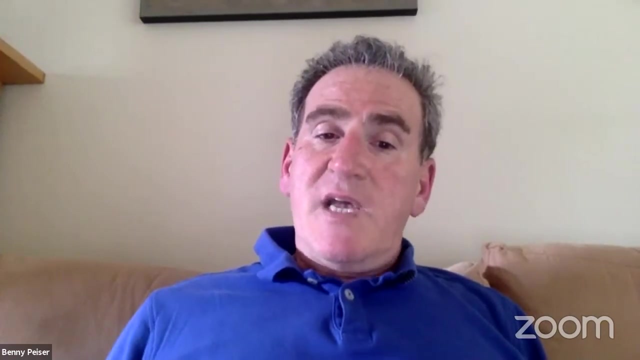 in in � there is a term called trust there's no security there is also a loss of trust in scientific advice and and the covet 19 crisis has exposed this crisis more than perhaps any other in how deeply divided the scientific community is on on this pandemic and as i said i i really hope there 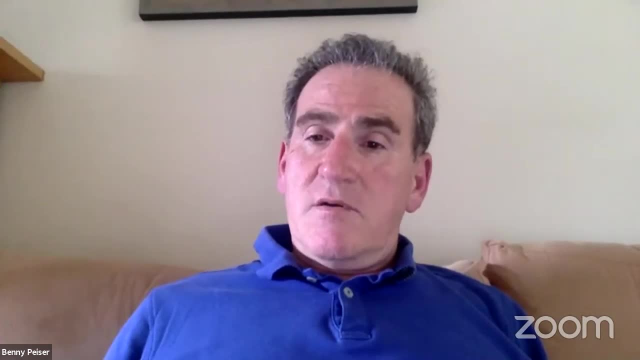 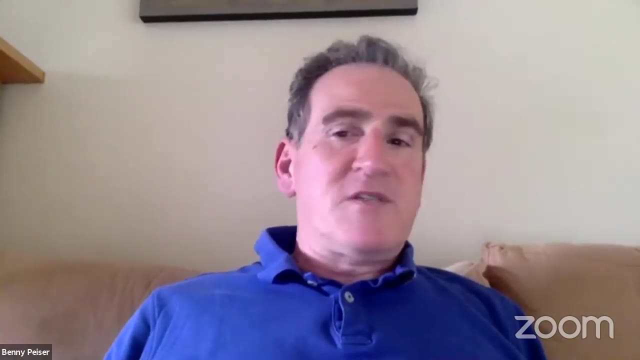 is and and one last thing: things only change change If the mistakes made are really catastrophic, after lost wars, after big natural disasters, after big accidents. only then changes are being considered. My fear is that this crisis might be such a big disaster- economic and social disaster. 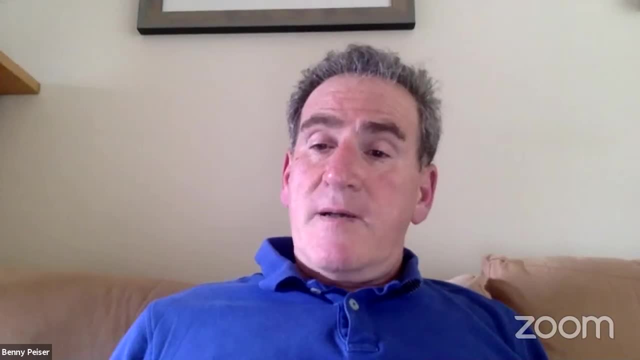 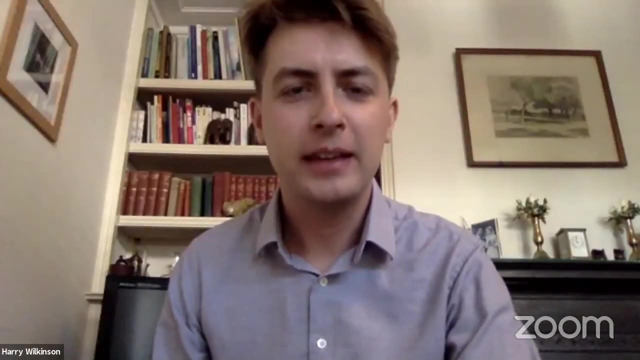 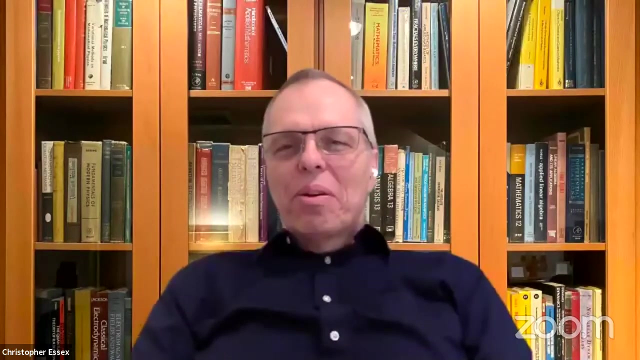 that will help to make policymakers aware that things have to change. Chris, I see you're keen to come in there. Yeah, I did. I think I have to push back on Benny here on the whole business about science. I wrote a book with Ross McKittrick on climate change and so forth, and one of the things 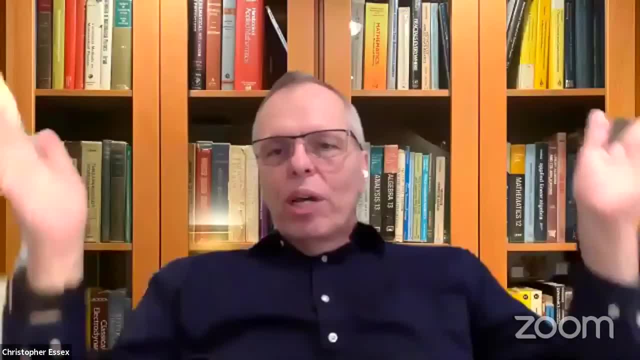 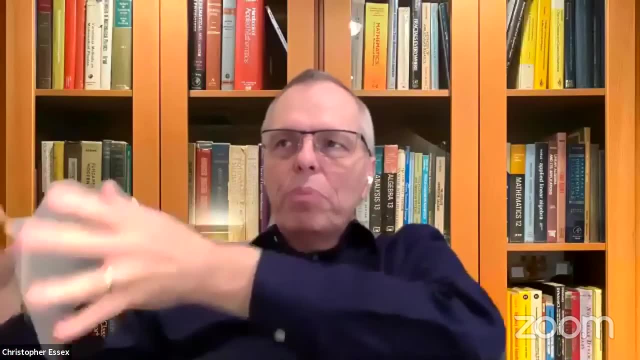 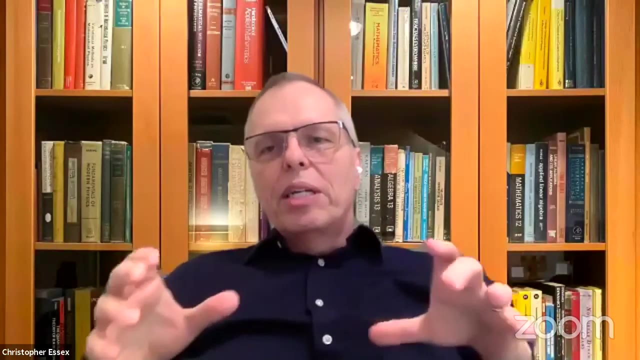 we were careful to do was not to have science as one sort of big package, But rather to make a distinction between the scientific mind and people who were acting on behalf of science and so forth. We defined a group which we called official science, and Benny is completely right about. 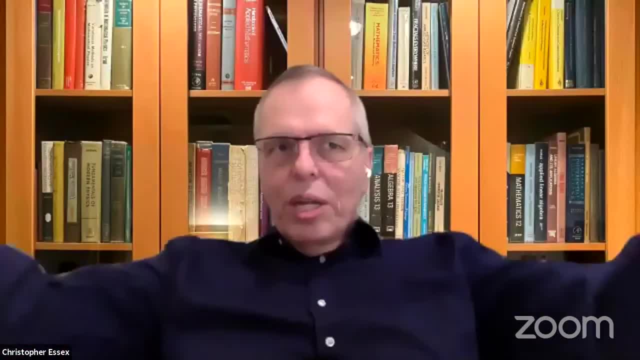 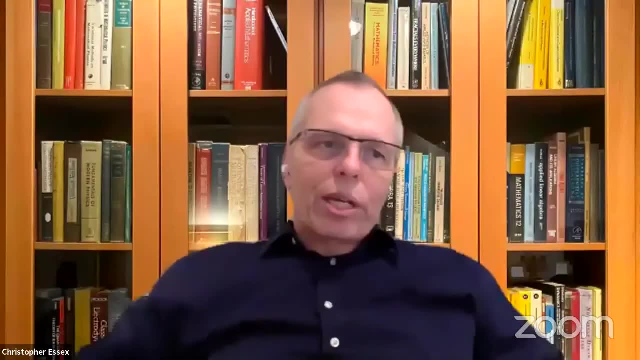 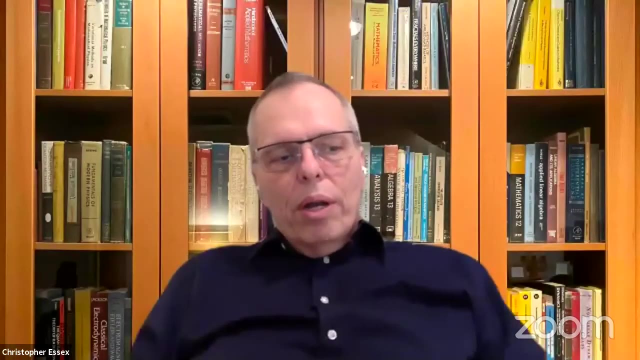 official science. I think they're the ones who are defining the science, and they include major scientific bodies, journal editors, Science advisors and so on. They have a certain kind of point of view, whereas the regular scientist often finds a lot of these things very foreign and strange. 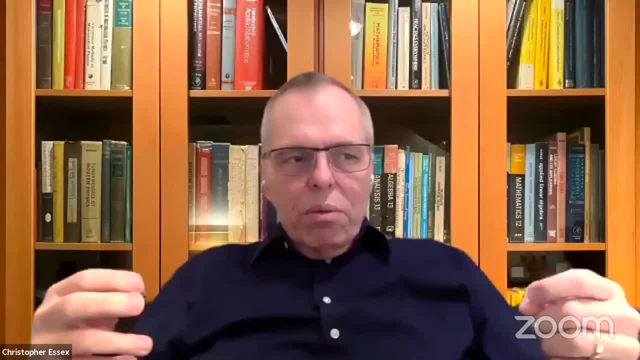 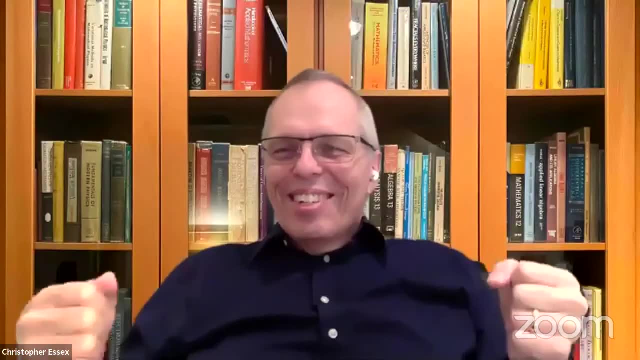 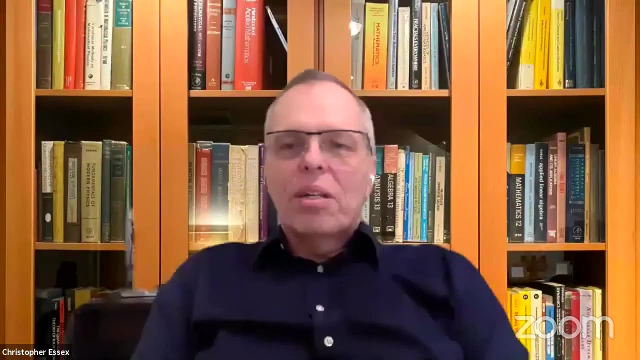 Many of us feel like these organizations have been subject to a hostile takeover in many respects. We think that that comes from the politicians and that they have their people, and so forth. I wanted to push back on that point. There is something That's very, very clear, which isn't really science at all. 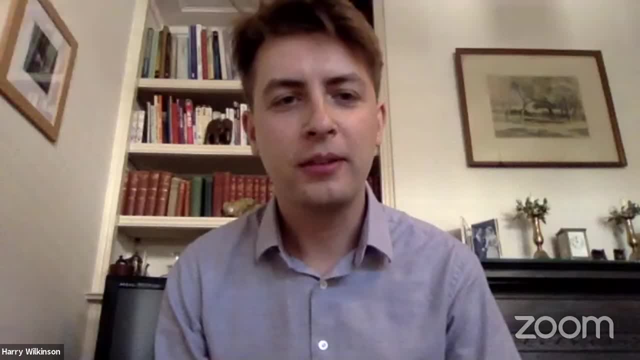 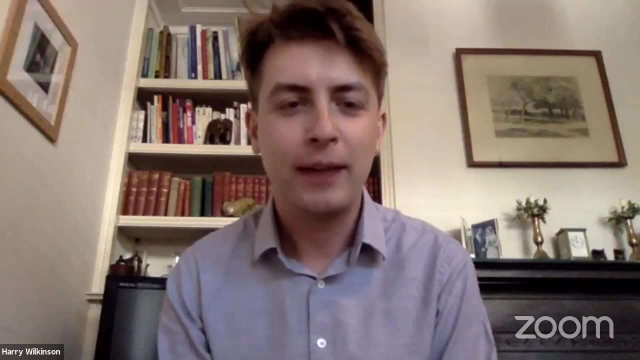 We call it official science. I wonder if you could just comment on this emerging science that we've been seeing called attribution science. Normally, we have models and they're tested by observations that are going to happen in the future. With attribution science, it seems to be the other way around. 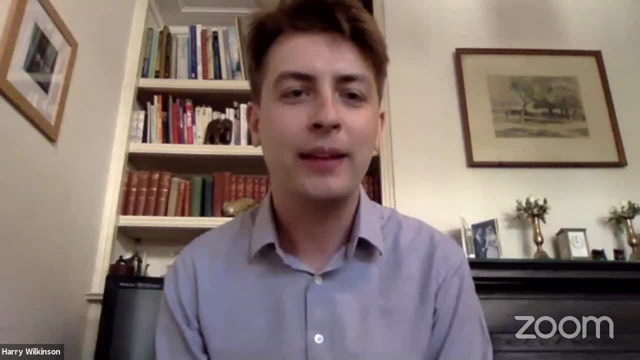 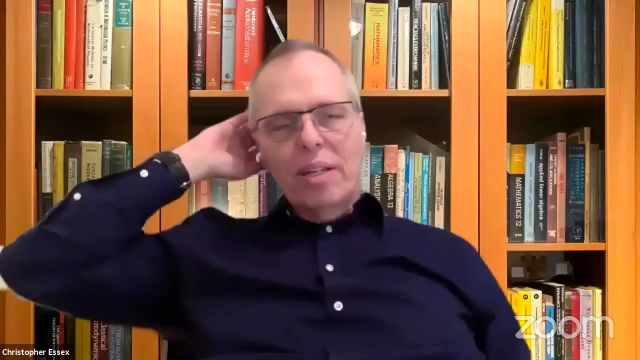 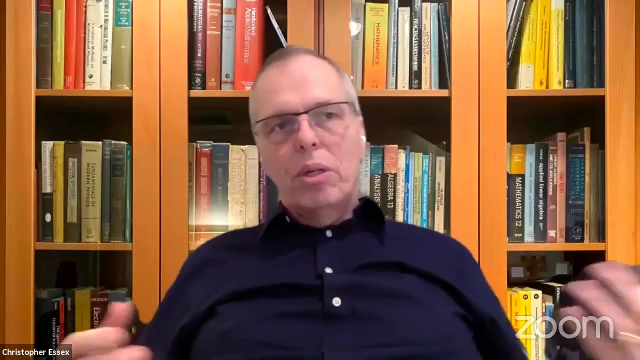 We seem to be assuming the models and then seeing how well the observations have fitted have fitted with our assumptions. The problem, as I said, with models is they can be made because they're cartoons. fundamentally, they can be made to fit anything. 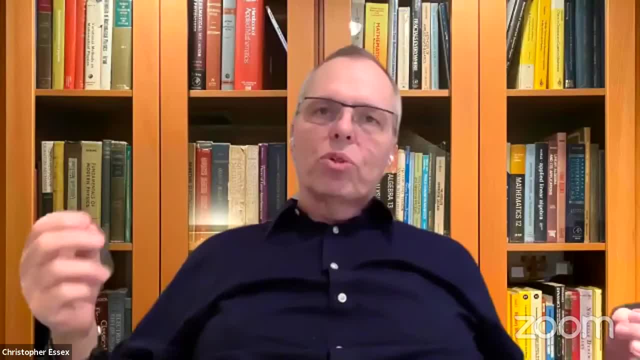 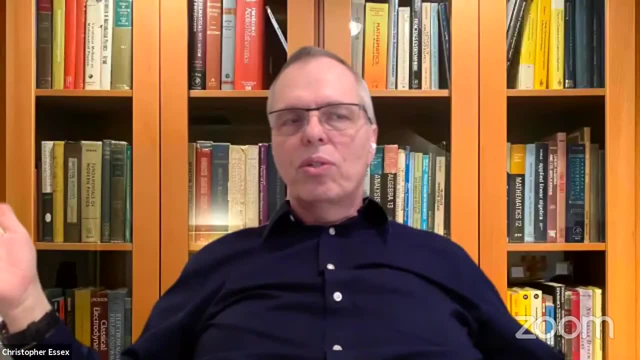 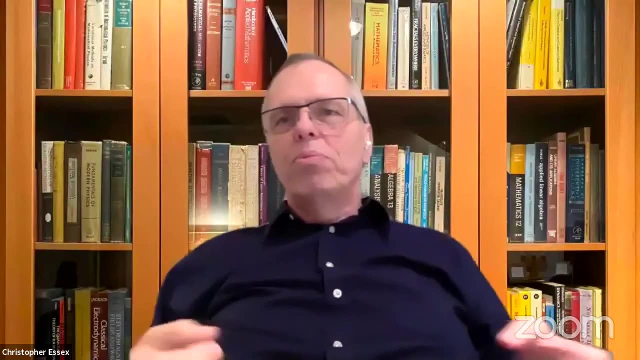 In many respects even a very sophisticated climate model for something simplistic like a time series for some average temperature field is just a curve fitting Everything that goes with that. you can just fit the curve. If you want to tweak in the bowels of a model, you can get pretty much anything you want. Fortunately I don't think serious modelers really do that, but there's no real problem with it because these are empirically based. You have to understand that when someone who is a theoretical physicist called something empirical, that's not the height of rigor, which is of course what economists think. 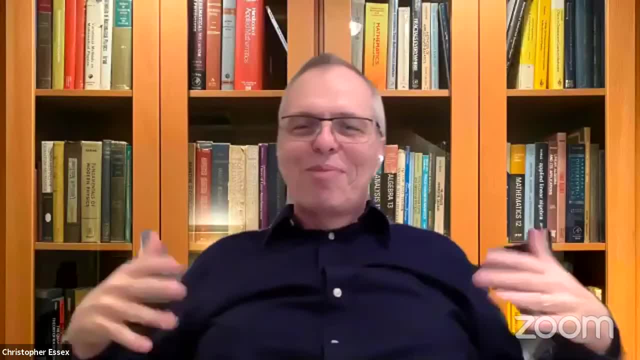 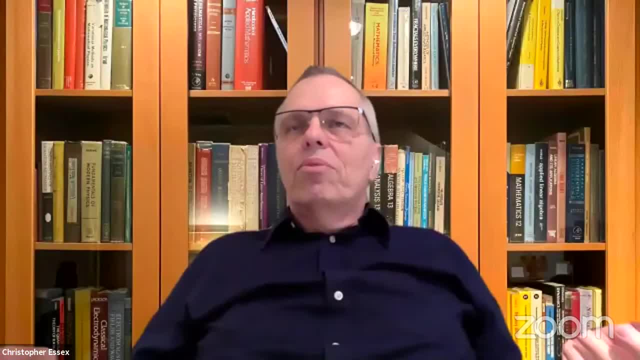 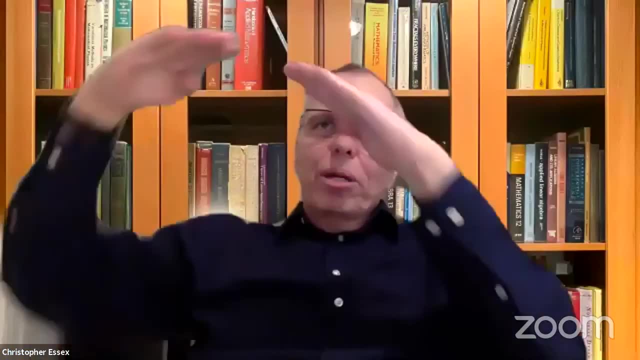 So it's empirically based. So that means that there's all kinds of straight lines through a bunch of noisy data And you have no idea that in the future that straight line might bend or something like that. So you now have to put a different cartoon in there. 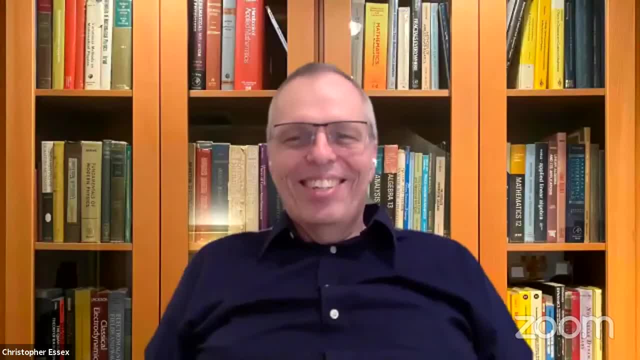 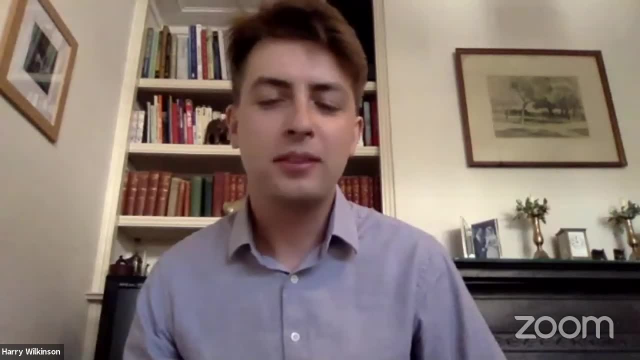 So that's my comment on that point. Thank you, And Gordon. I wonder whether you could comment on whether there's a problem with a lack of wider knowledge about statistics and about economics in the wider public. Do you think part of the problem is that the public are being led towards supporting the politicians in some negative endeavours? 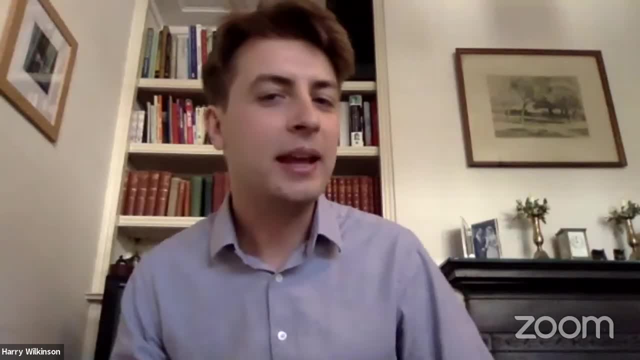 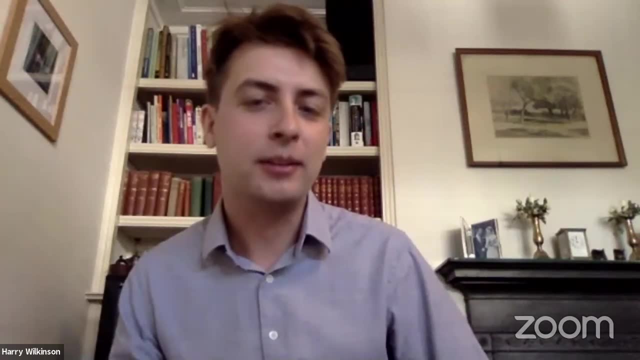 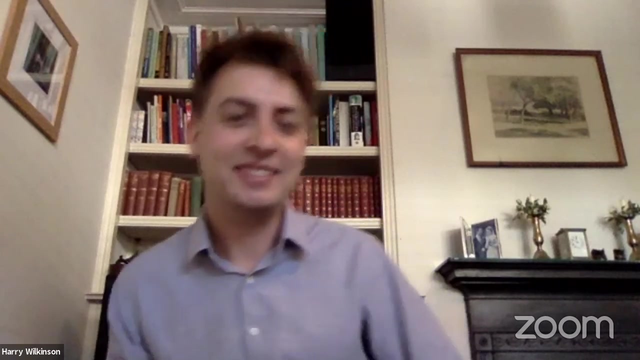 And so the public. are they to blame for what some of the politicians do, And does there need to be a better level of understanding of economics and statistics to inform a public that will support the right politicians, as it were? I mean, I think there are two separate issues there. 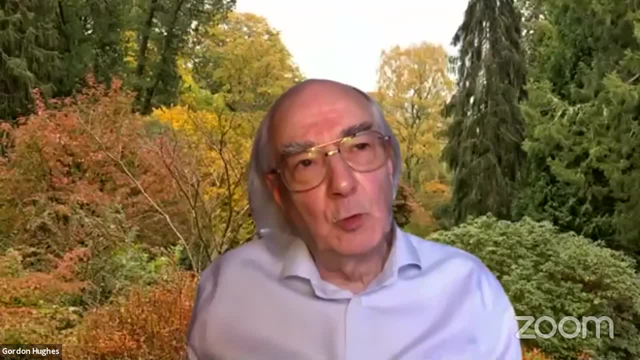 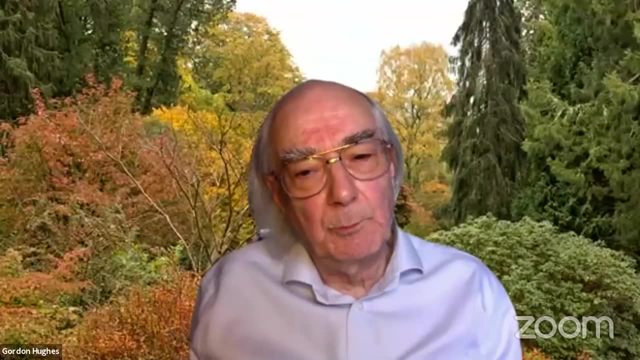 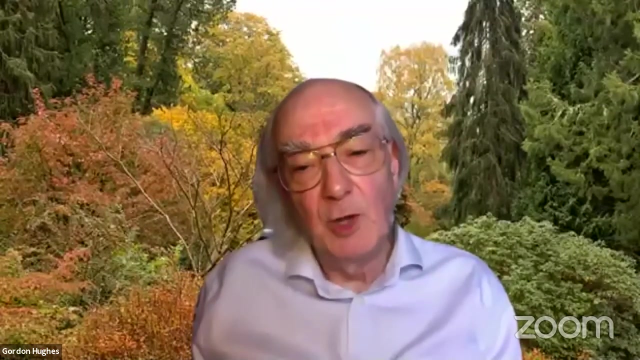 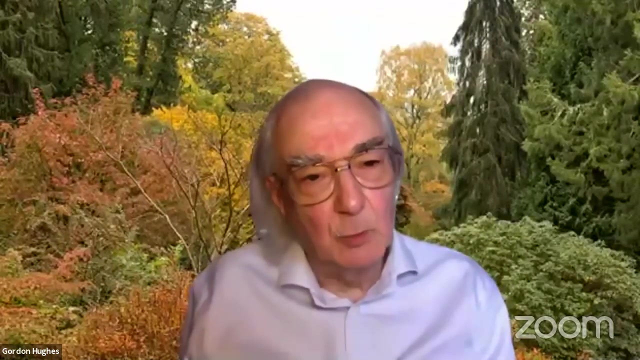 The first is that almost nobody with a serious scientific background or a mathematical background Has much interest in participating in political life, And to the extent that they do participate in it, they very rapidly lose the background, So that the consequences, as is always frequently pointed out, there are very, very few people in political or official life with a serious training in scientific or mathematical disciplines. 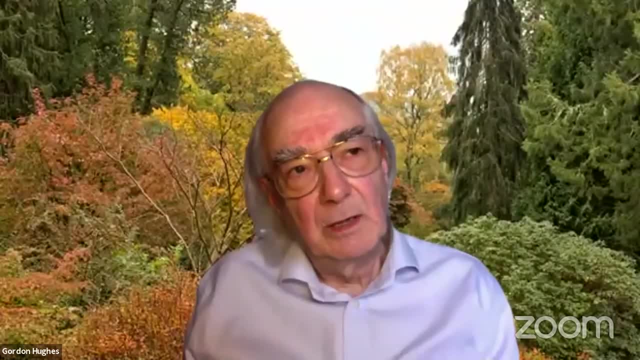 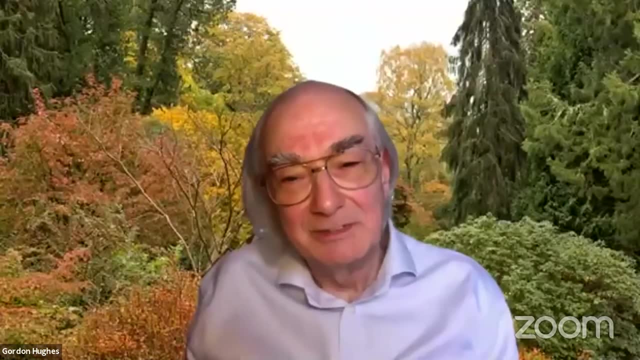 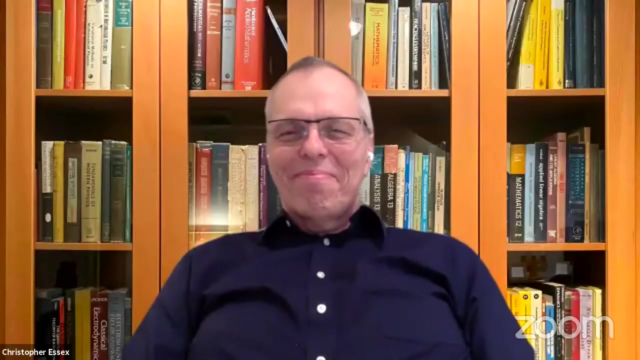 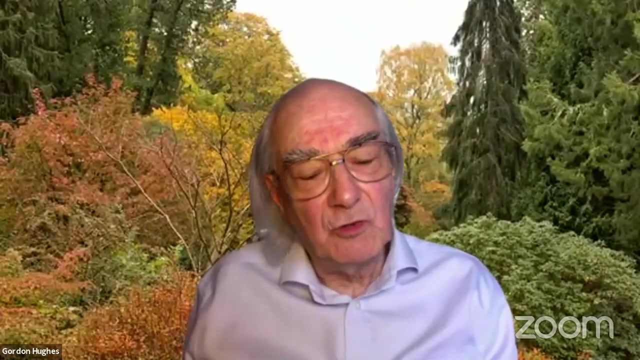 The other thing Is that politicians are rarely rewarded for having an open mind. What is expected of them is essentially certainty and predictability, And that typically means that- the kind of quote that was ascribed to Keynes, which is: when the facts change, I change my mind. 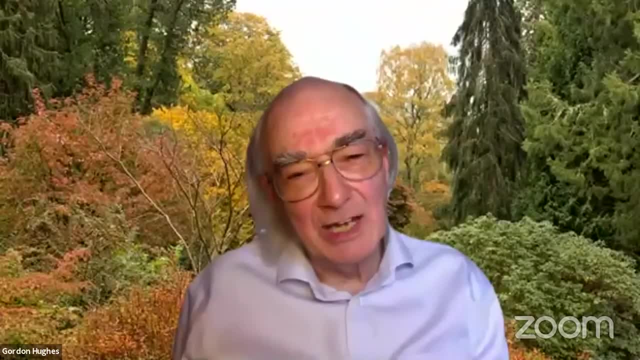 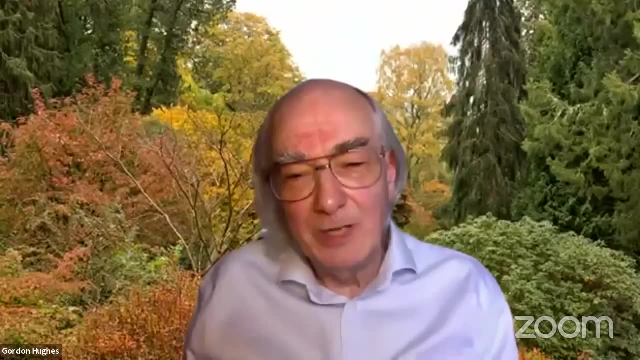 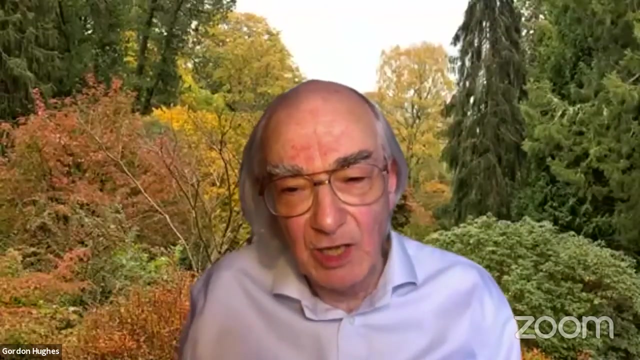 What do you do, sir, Is essentially a comment that any politician would find horrifying, because, of course, the facts shouldn't change And therefore he shouldn't have to change his mind in terms of the decision, because he'll be held responsible for making a U-turn. 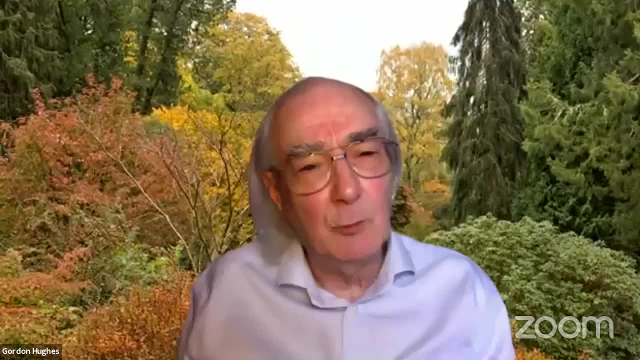 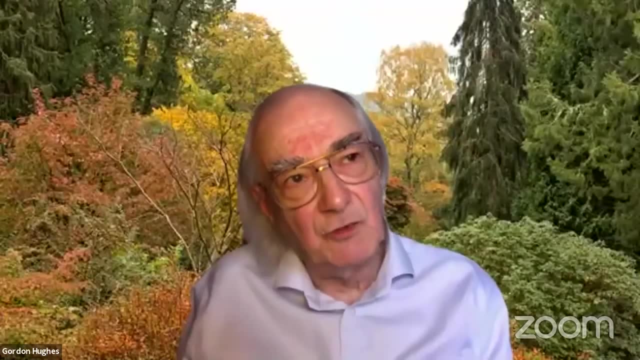 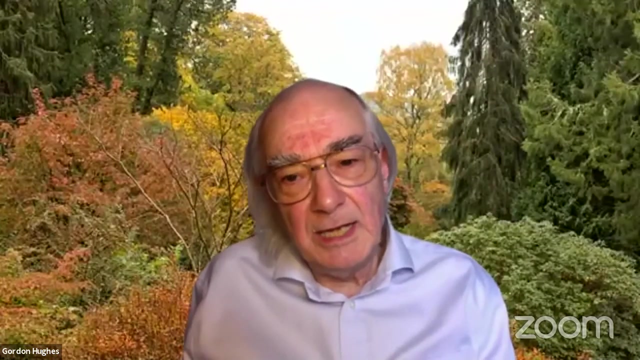 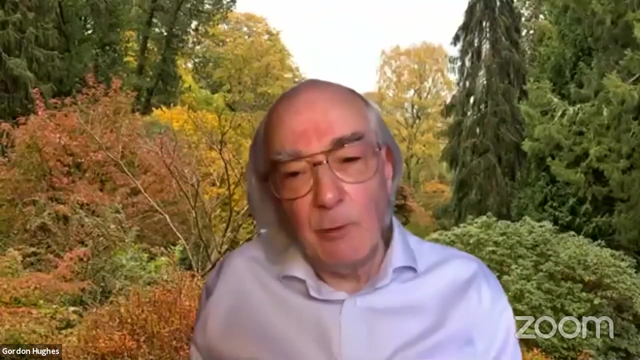 And of course that's clearly a sin of the first magnitude. The point here is that things like statistics and science, and At least Mathematical training and the like, lead to a cast and frame of mind that are very hard to reconcile with what is a fundamental political role, which is to try and reconcile what are frequently irreconcilable positions and try and find a way of dealing with a world that is messy and uncertain. 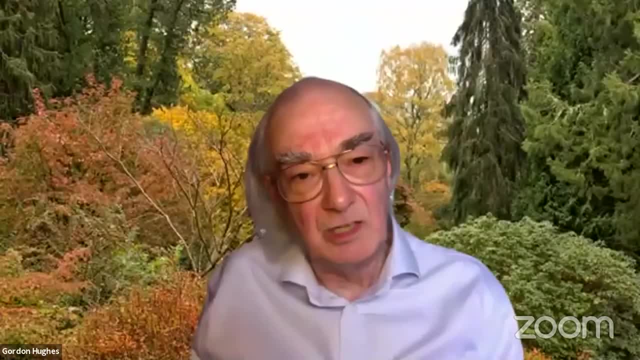 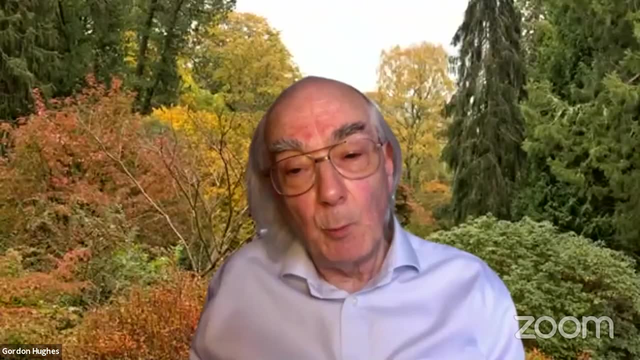 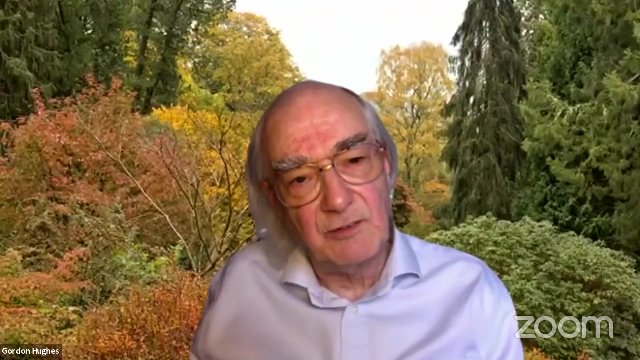 Where people don't want it to be messy and uncertain, And I think that we have to be careful about expecting more than we can really get. But we can demand that politicians- and what we expect of politicians isn't just to tell us what the right thing is- without the kind of desirable elements of both policy and a frame of mind that we've been discussing. 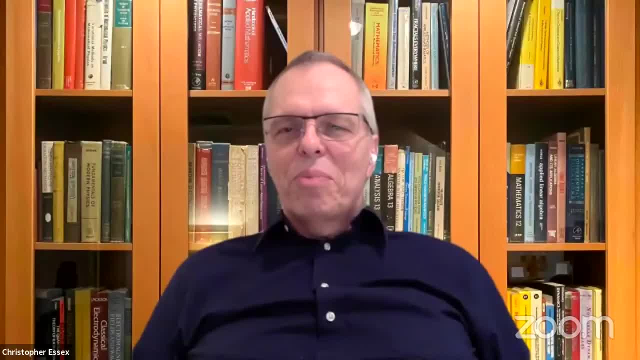 Sorry, Chris, you wanted to pick me up. Yes, I did. I wanted to reinforce it. It was a kind of a short remark when I would speak to politicians about some technical point And I said: this is really an important technical point. 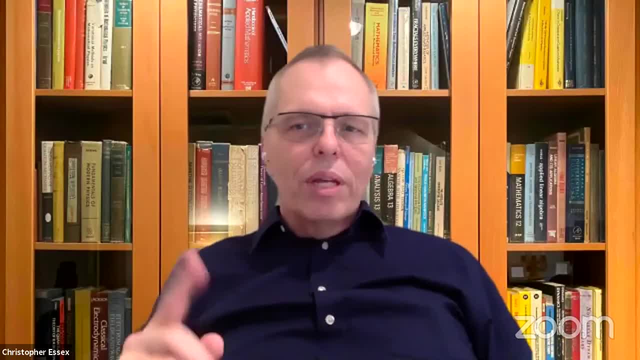 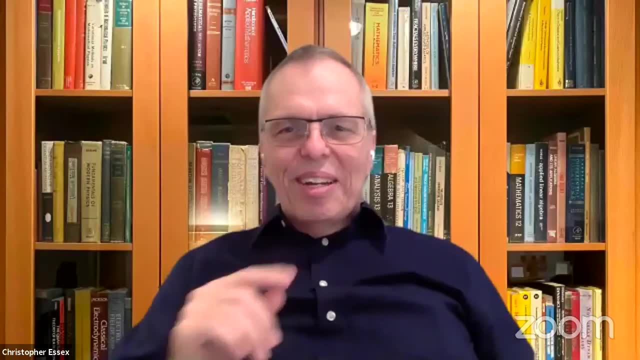 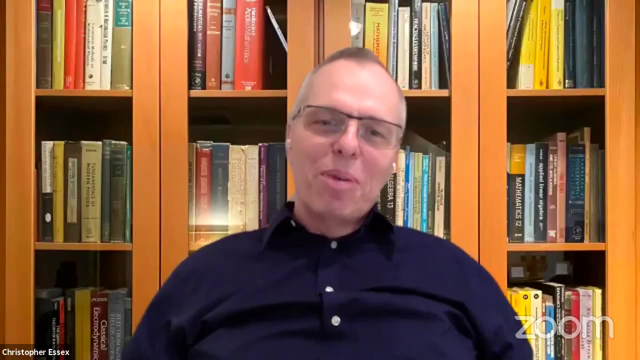 It completely changes how you think of things. And they'd say: oh yes, Chris, but you have to understand that in politics, perception is reality, And I say, well, where I come from, reality is reality. That's, in a nutshell, what the problem is. 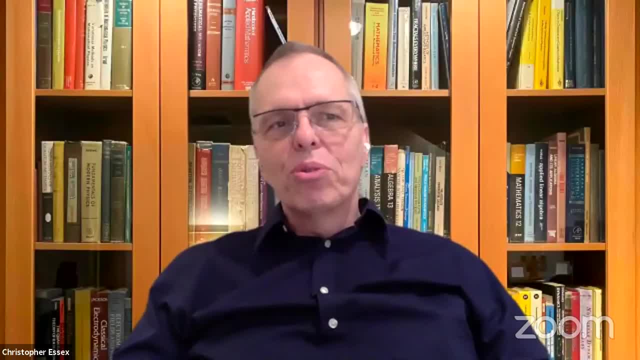 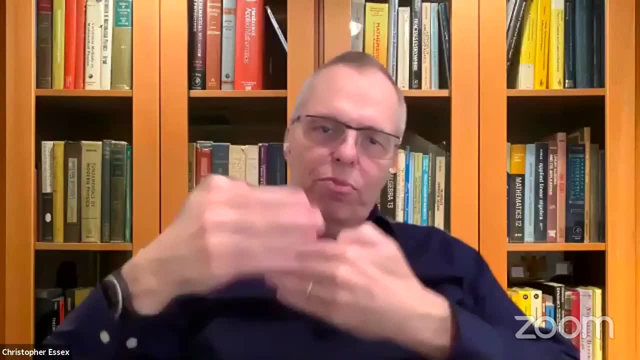 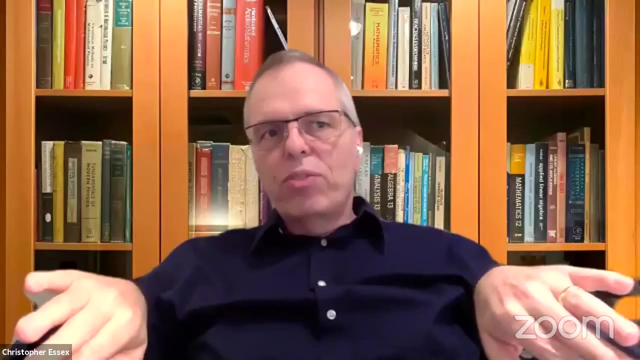 So, Speaking to people who don't really care what the truth is, they care about how it's perceived, And that immediately follows entirely with this gulf between these two different worlds, And I think if you're going to have a structure that does the best for people, you have to separate them. 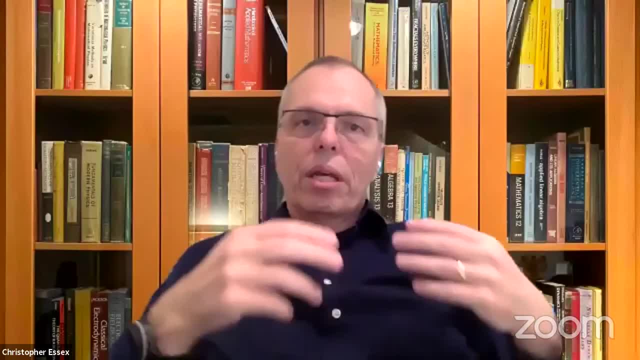 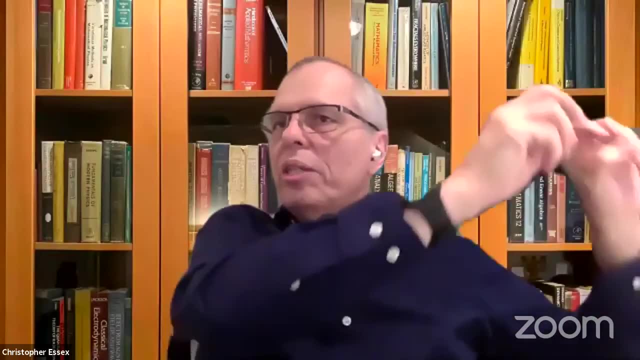 They can't be together. So you have to have an understanding that the scientists do science and they do all the controversies that go with that. You stay out of it, You don't try to define. The correct view is just to leave them alone. 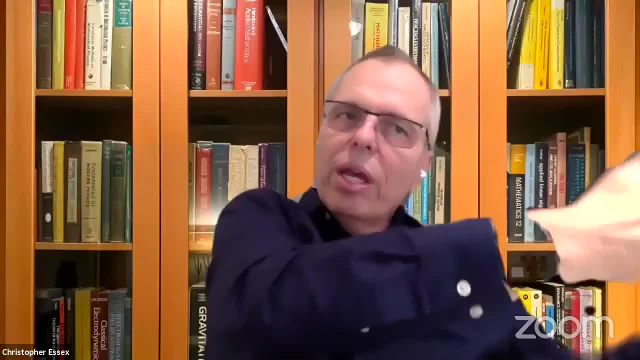 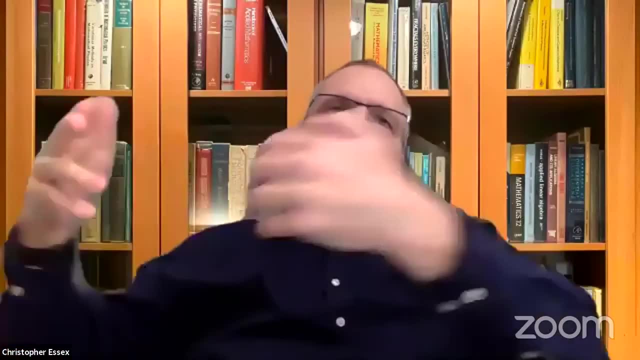 And then they peer in and look at what they're saying and they're arguing about and so forth, But they keep their hands off of it, and vice versa. Scientists don't try to become politicians. That would be the ideal. I don't know if we'll ever achieve that. 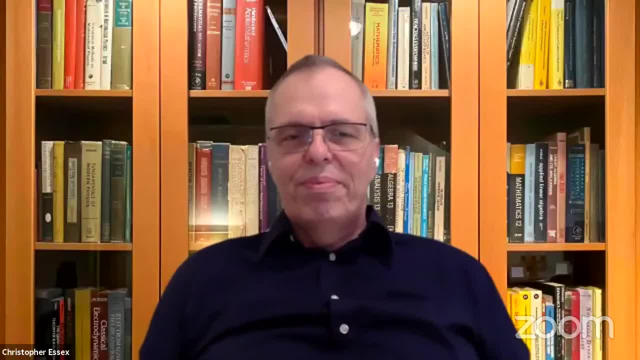 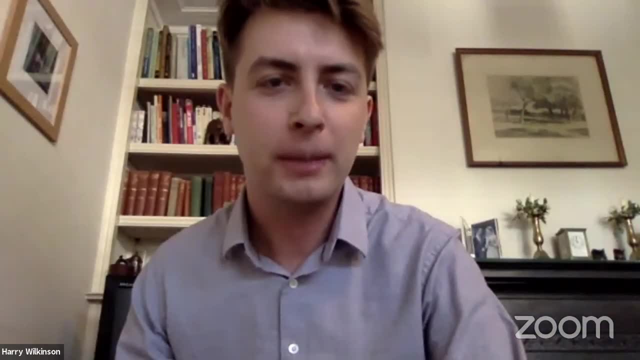 But that's what needs the direction we need to go in. Can I just? I'm going to ask Benny one more question and then we'll come back for some closing remarks from each panelist. So my final question for you is, Benny, is on the culture war. 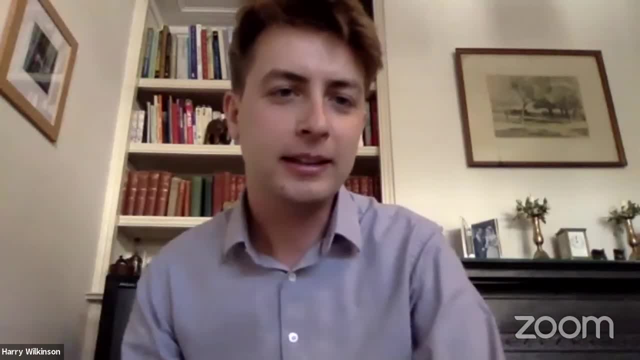 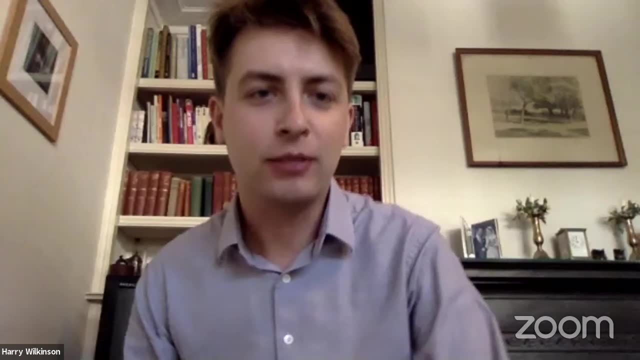 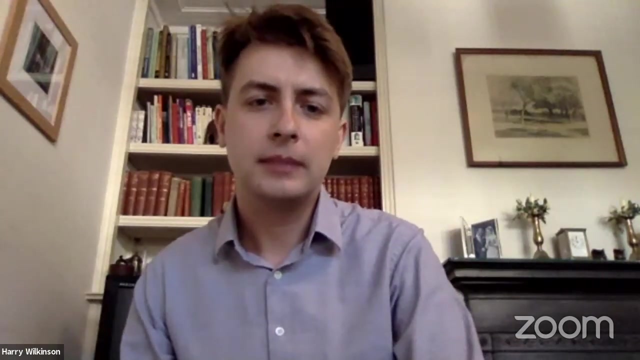 How much of these topics- and I'm thinking particularly climate- how much are they being absorbed into a wider cultural battle? And how is that disrupting a more open minded approach to the climate change debate Right? Well, it's not yet a culture war. 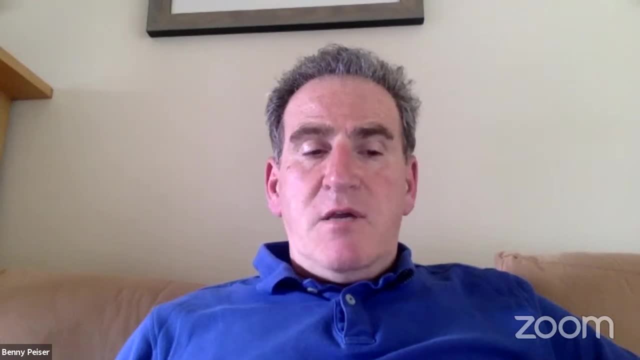 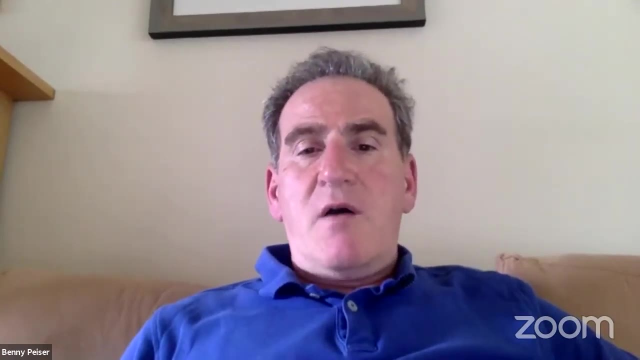 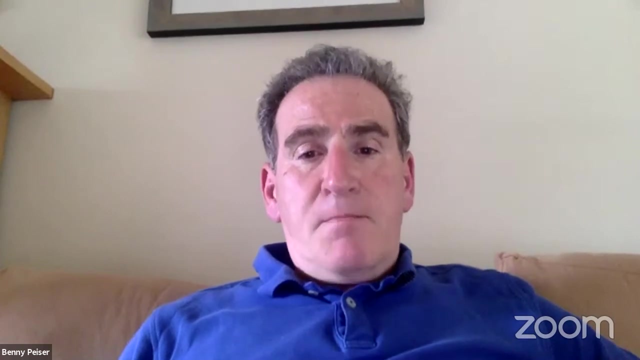 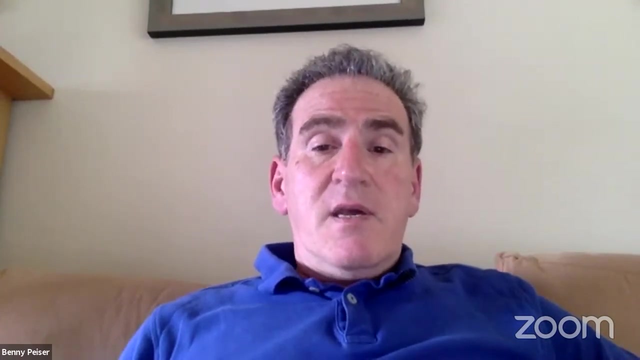 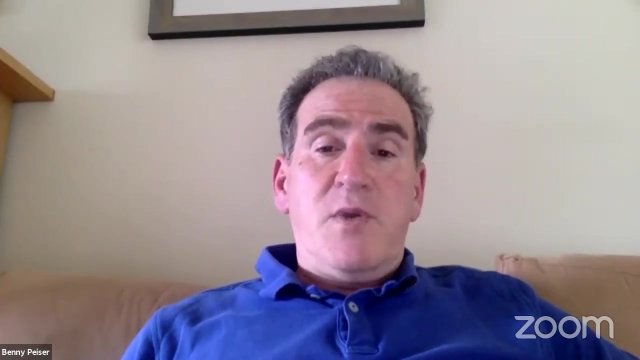 Because the kind of people who are more skeptical about the alarmist predictions are fairly a fairly small group in society where it can become or turn into some kind of clash- cultural, political- is when people will be impoverished Or fear to be impoverished as a result of the policies being adopted. 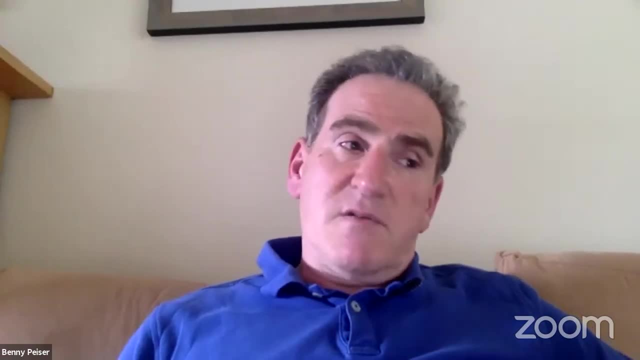 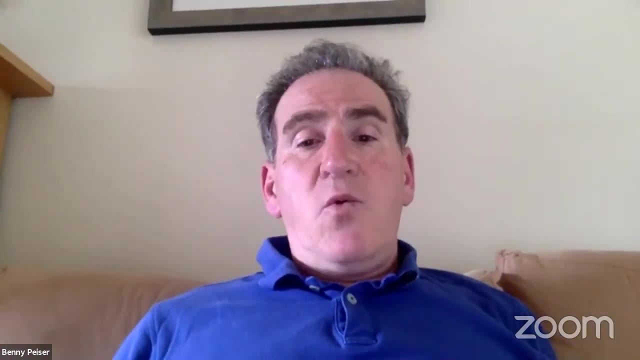 And let me just come back to what Chris just said. this kind of you know, the scientists should do the science, the policymakers should do the policy. That only works in a world where scientists don't believe they have to save the planet. 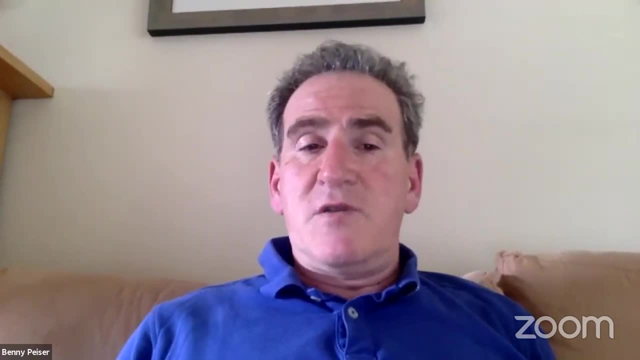 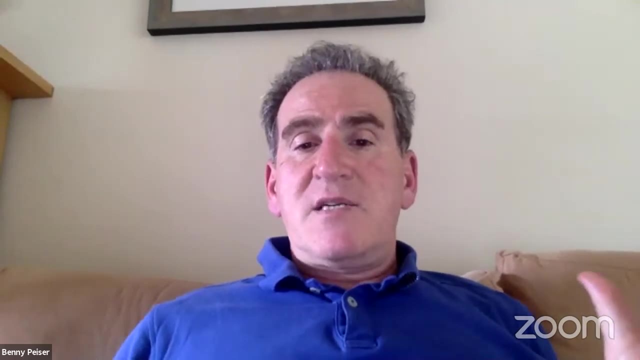 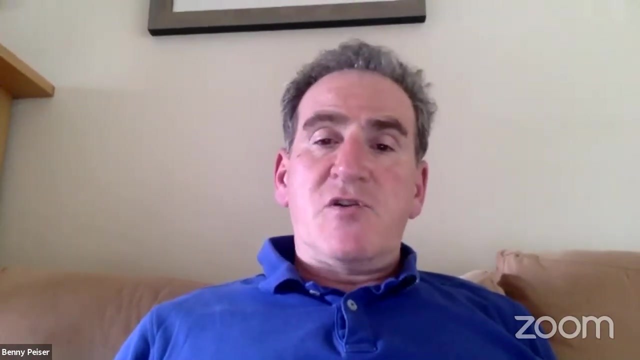 The problem we are facing and that is, in a way, similar to the pandemic. Once scientists believe that they have a kind of secret knowledge That is important to save the planet, they will do everything and anything to lobby and to campaign and to protest governments, ministers, politicians. they will attack them until they accept their view that they are right, and only they are right, because they are the ones who want to save the planet. 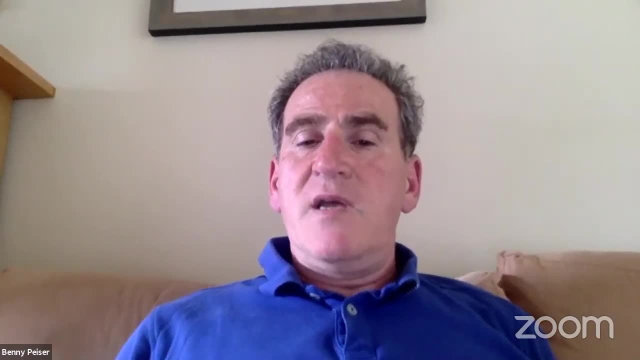 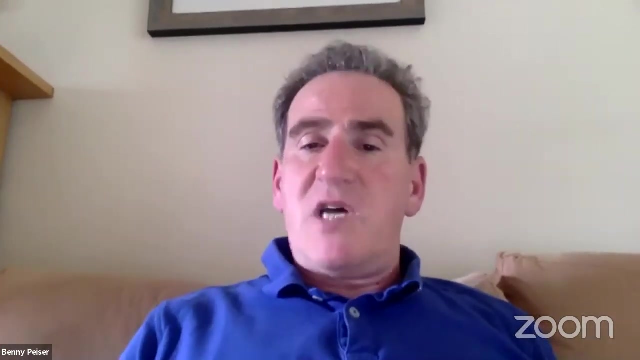 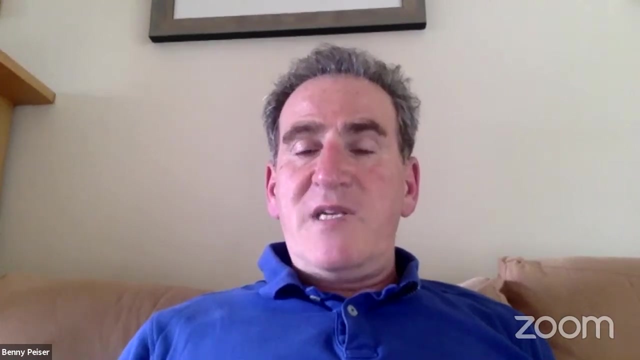 That is the problem we're facing. We're facing an almost We're facing an apocalyptic movement that believes that they have the truth and that truth has to be adopted globally by governments, because otherwise we face extinction. That is part of the problem why scientists have become activists, why they've no longer accepting this. we are scientists, they are saviors, they are people who, they have a messianic kind of mentality. 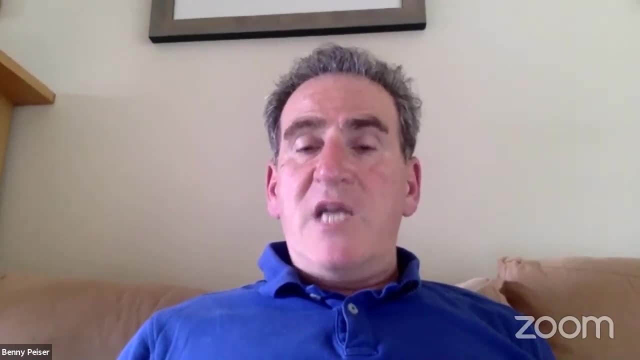 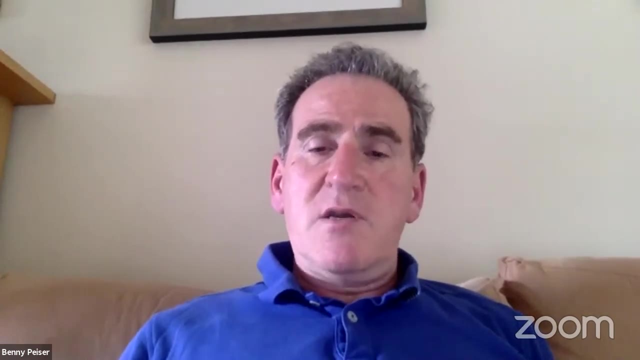 They think that politicians are. They think that politicians are Are dangerous because they are not following the science. Now, with a culture war, as I said, I don't think it will be over the science, But there is a growing risk- and we've seen it in France, we've seen it in other countries- that the policies being adopted by governments which will make life more difficult, 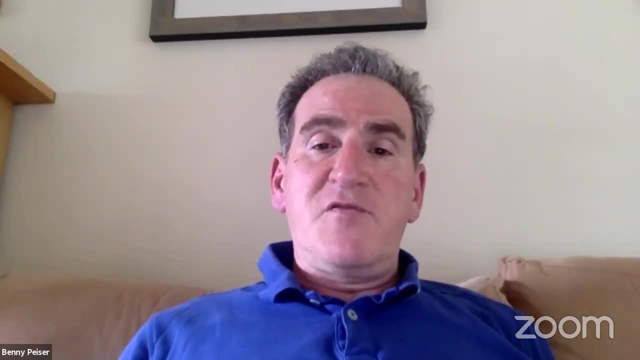 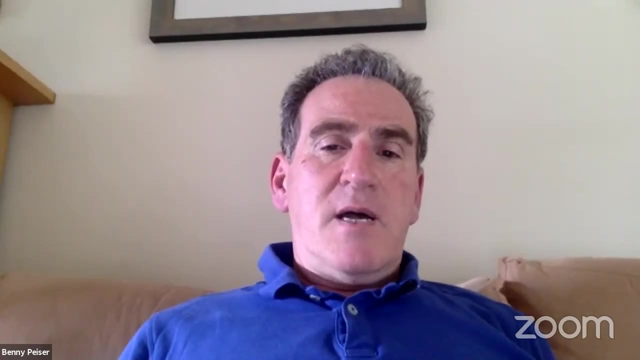 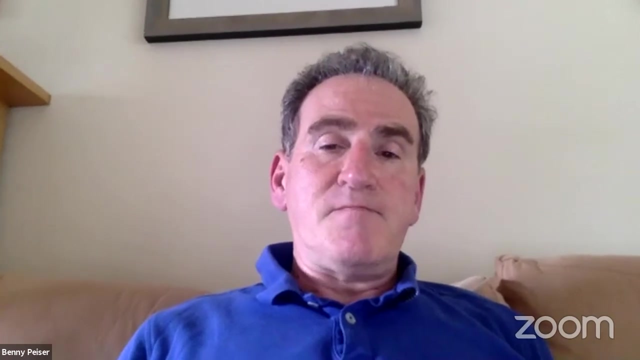 Which will make life more difficult, which will make everything more expensive. That could trigger a fight back by parts of the public who feel threatened by the government. That could trigger a fight back by parts of the public who feel threatened by these policies. that is possible. thank you, benny. so now i think we'll come to the closing. 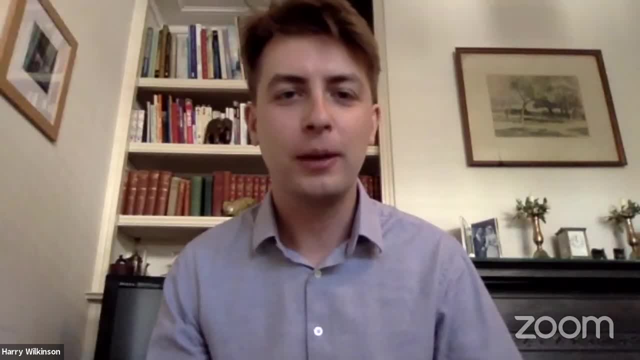 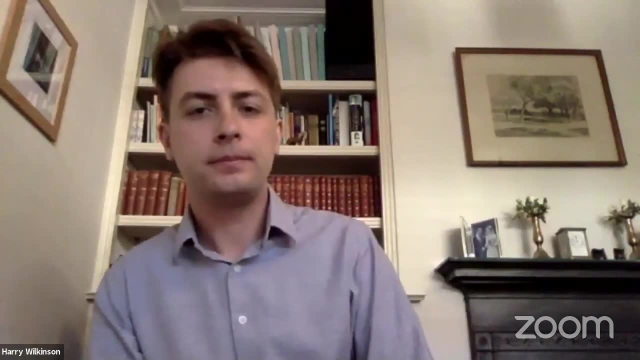 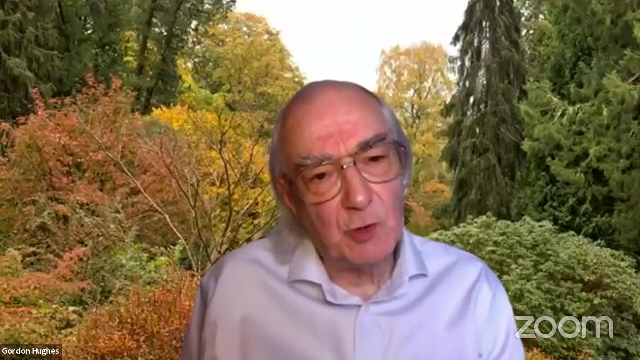 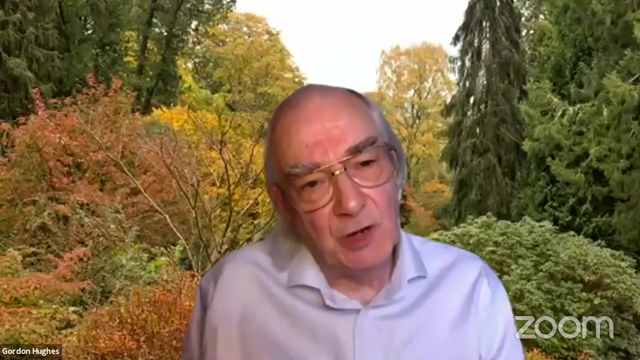 remarks. so if you could set out what your takeaway point would be to our viewers- and, gordon, i'll come to you first. um, i i'd like to pick up partly on what chris was saying, but it's it's a core part of what i think is at the heart of what benny has said and the more general. 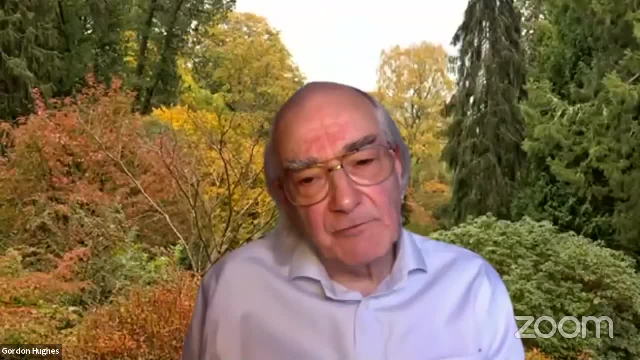 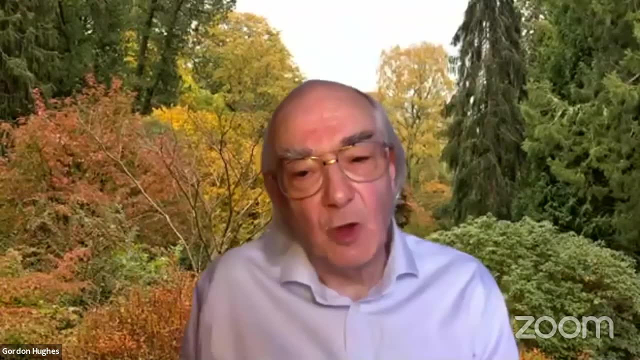 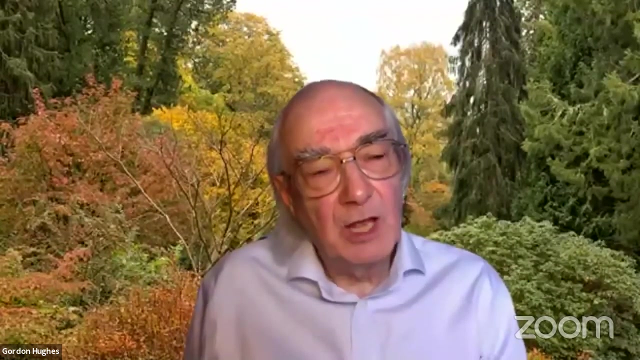 discussion, and that is: is it ever possible to believe in science as being something that is independent of, separate from policy making, and that the process of then taking that independent knowledge and converting it into views for policy recommendations, whatever, benny's core point is, in effect, that the scientists 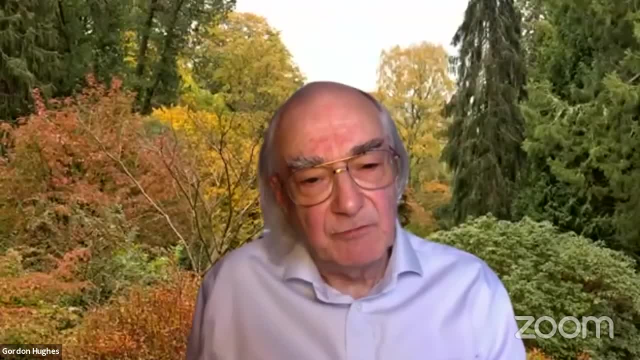 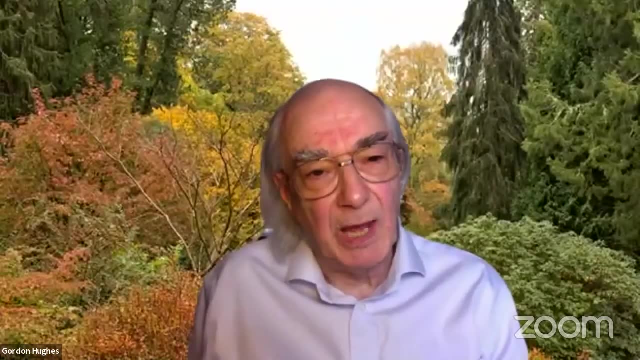 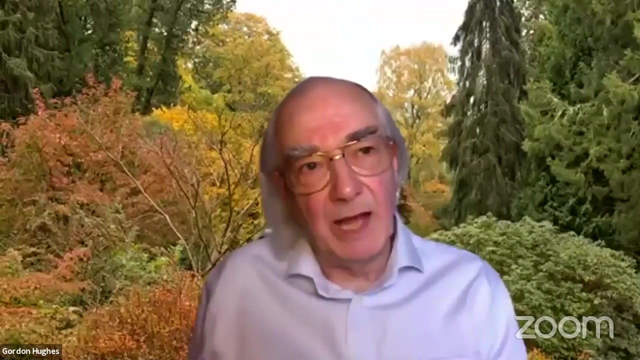 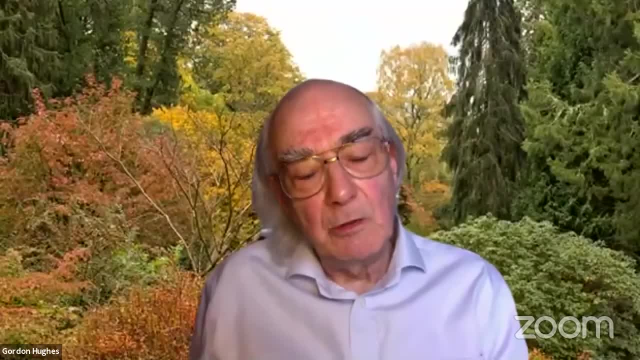 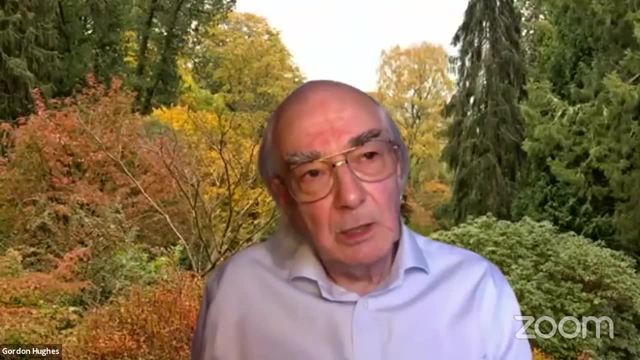 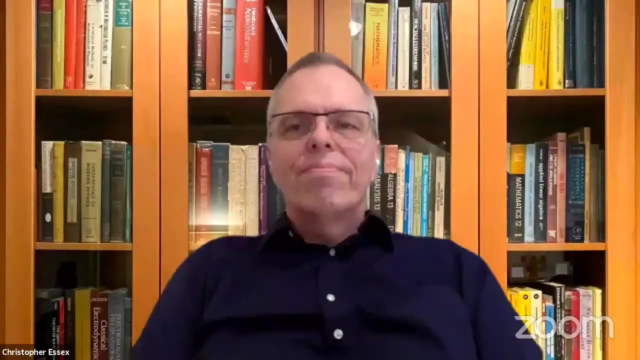 if you take that view, if you take the view that you actually know truth and that, therefore, you know what it is that you are um wanting um the society or politicians to do, you've stopped being a scientist, you've stopped being somebody who accepts the fundamental open-mindedness. 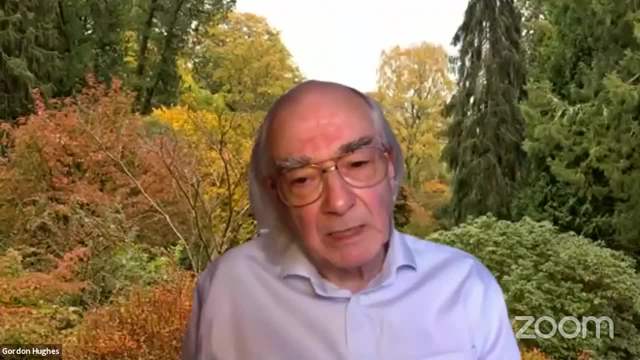 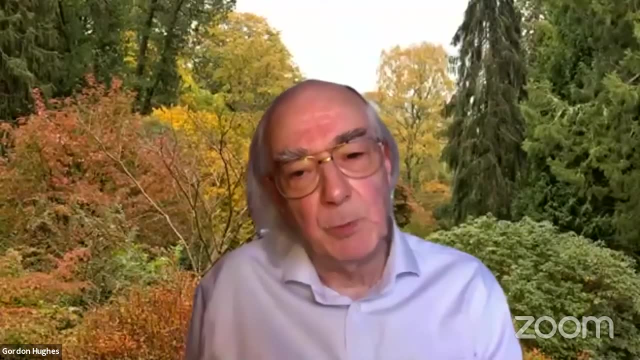 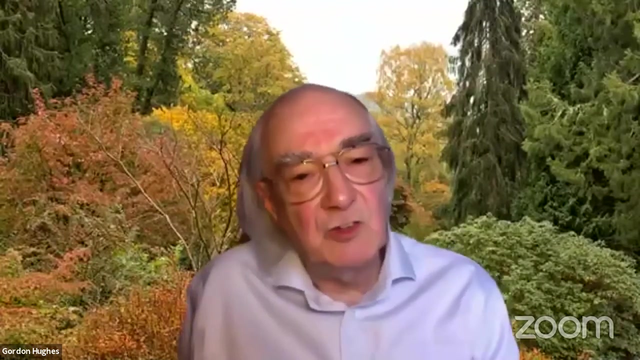 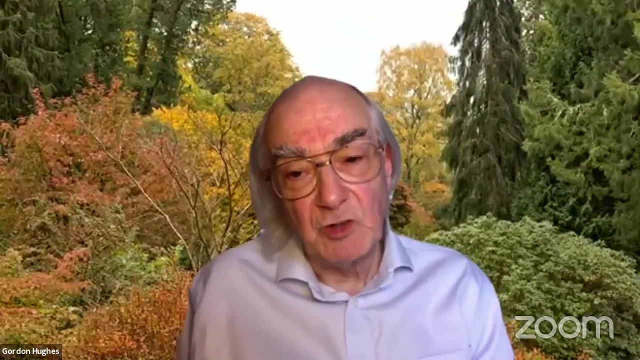 that is required and the funding, mental willingness to challenge, um even your own beliefs, let alone the beliefs of other people, and that, in a sense, i mean my analogy very frequently- is that in that case, knowledge turns into religion. it's essentially um a revealed truth which cannot be questioned, and i think the real problem is that for many scientists, 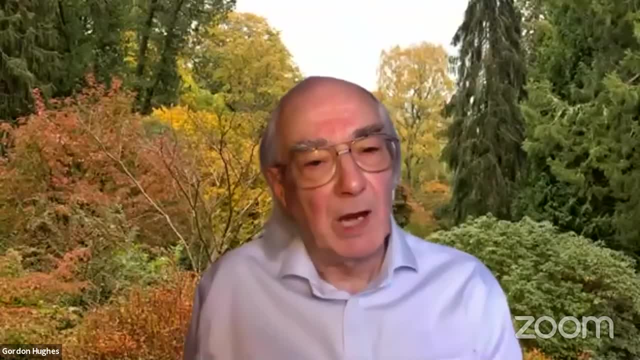 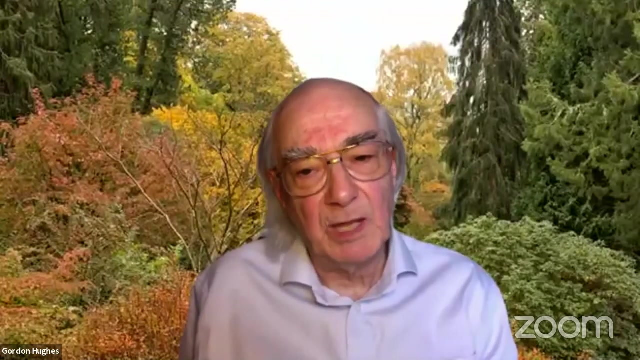 what they're doing is so important that it becomes revealed truth, and that, in doing so, they are throwing away the thing that is absolutely essential about the scientific method and the value of the scientific method, which is that it is independent of the immediate concerns, whether it be of governments or politics and whatever. and then 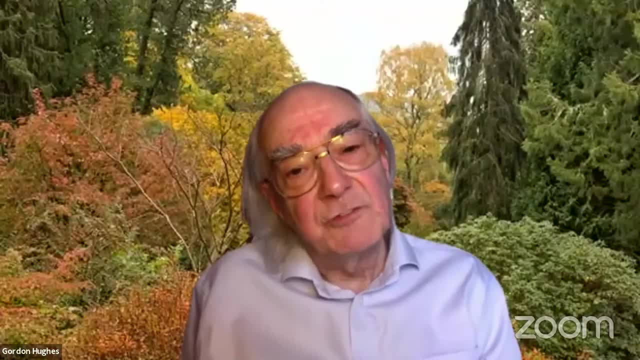 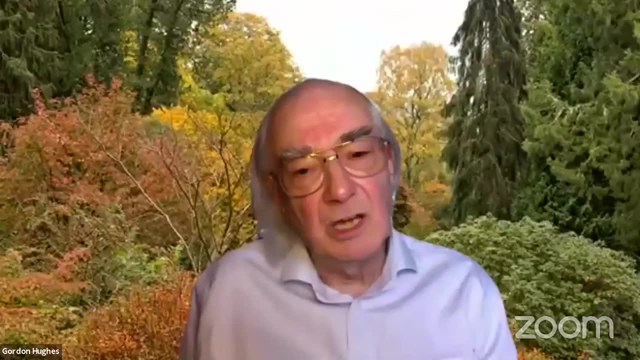 the final element to that is that we have to learn to live better with uncertainty. we have to live with the fact that we have to live better with uncertainty, and we have to live better with the fact that not everything can be certain and that it is not within the capacity of either us as 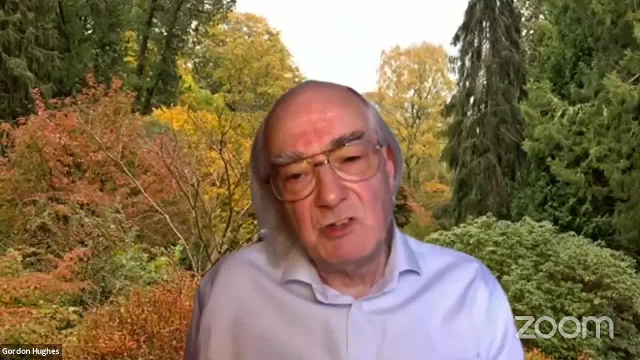 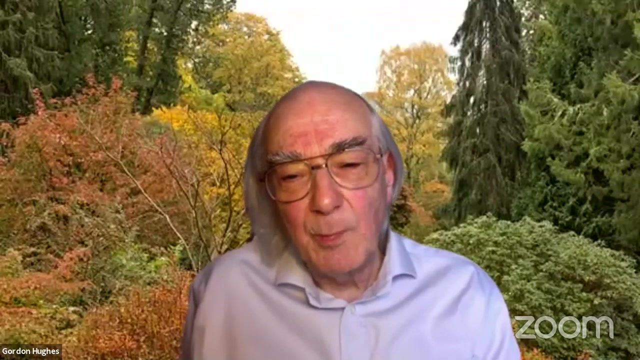 individuals or of societies to essentially offer the levels of certainty that lots of people would like? um, because essentially it means constraining ourselves and we can be certain. but we might as well go back to the certainty of the catholic church as much as any other kind of certainty. 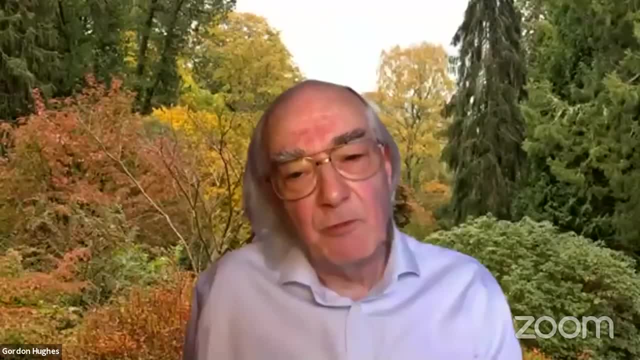 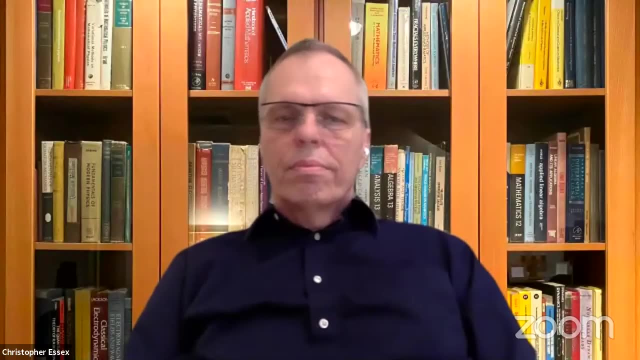 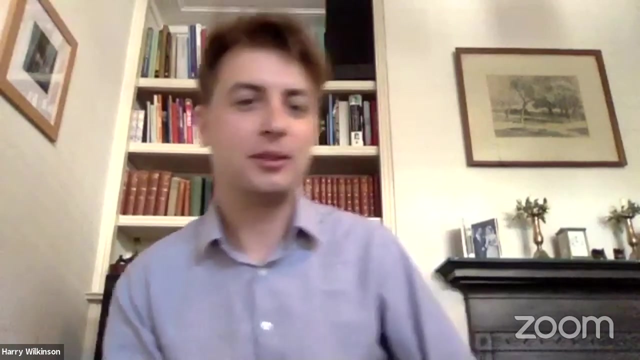 and the world doesn't allow that to us, and therefore that means we have to live, both politically and individually, with a level of uncertainty that is often profoundly uncomfortable. thank you very much, gordon and uh. now, uh, dr essex, would you like to give your closing remarks? 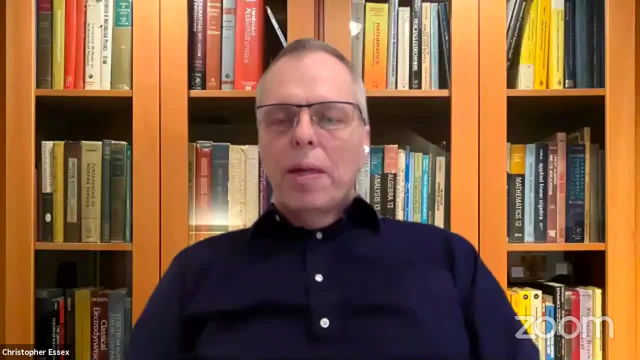 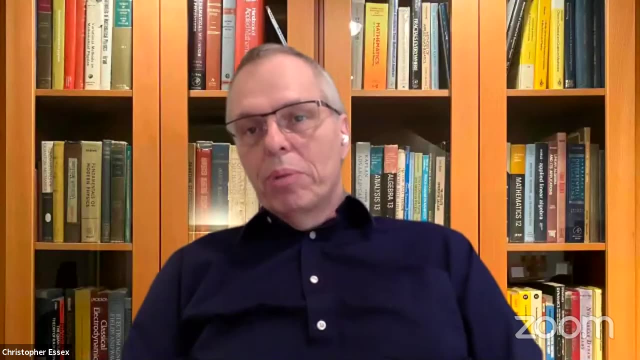 yeah, i i like very much what gordon was saying. uh, i think that it's very true that the moment you start becoming this kind of political activist, even if your phd is in science, you're not being a scientist. you've lost your scientific mode of thought, becoming a politician. 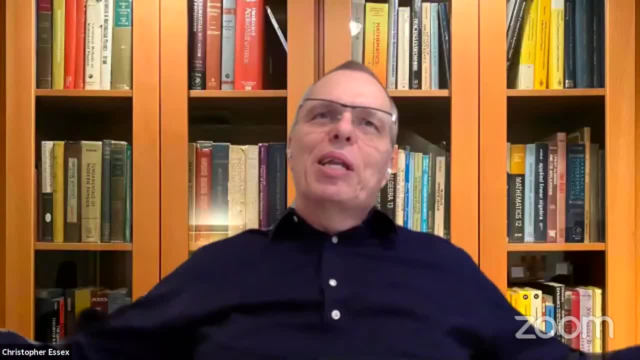 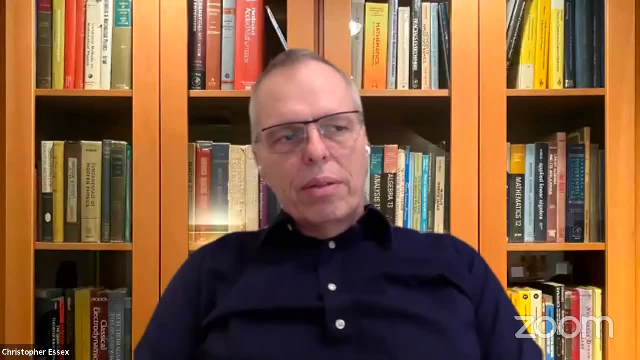 and so i sort of reject the people who do that from the scientific side of this discussion. so, uh, yeah, i i think that that it's. it's really important that we understand that science is about uncertainty. it's not knowing things fully. it's a humble activity, i mean you. 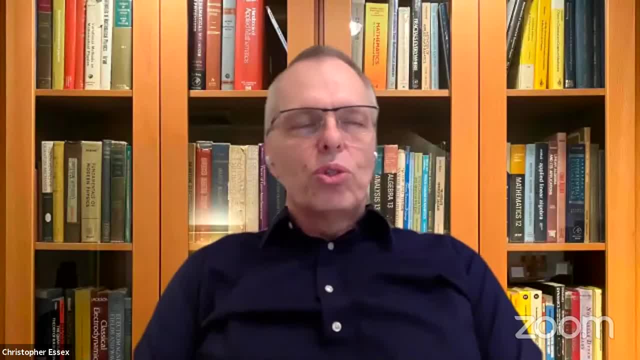 might have to be cocky and arrogant to take on mysteries of the universe, but you have to be humble, also because you have to remind yourself not to believe your own propaganda, which of course is one of the essences of the scientific mode of thought. The other one, of course. 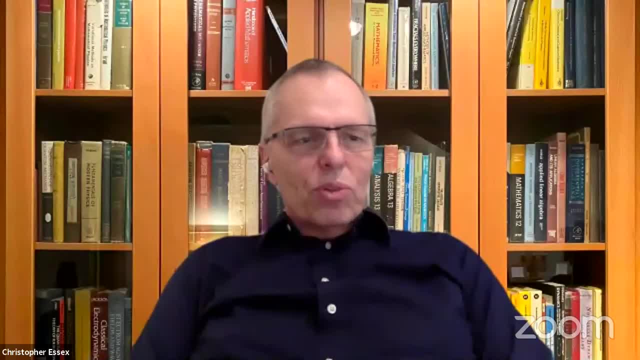 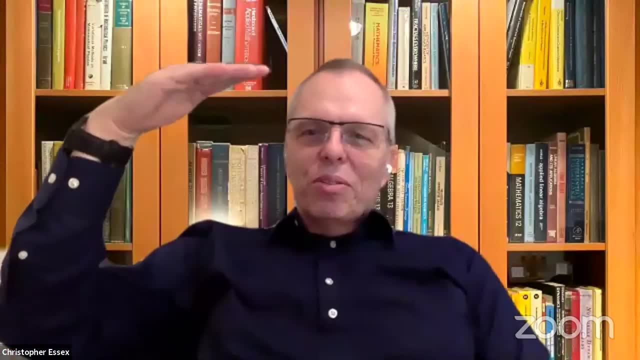 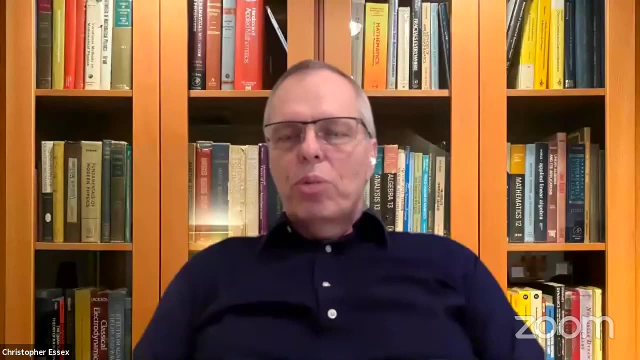 pretty, like Richard Feynman used to say, was a science is a belief in the ignorance of experts. So we can't have this kind of higher class of super experts. You have to be a little humble, because humans are very, very fallible- and I'm no exception- And you have to remind yourself of 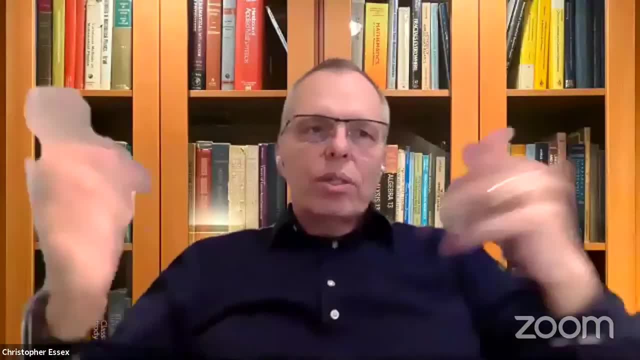 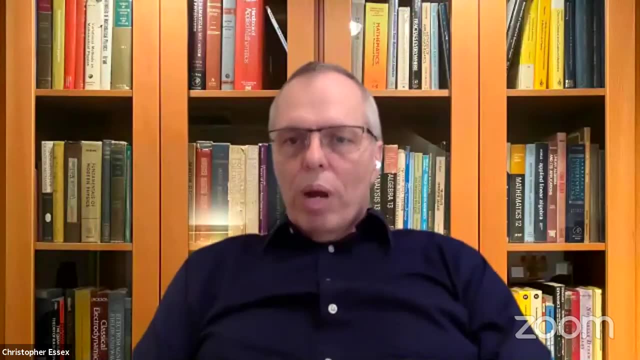 that, And once they become these kinds of infallible people, yes, it does turn in a weird way into a kind of religion, And so I think that Gordon is completely right about that. The other thing that I think that Gordon is saying, which I think is right, on the money: 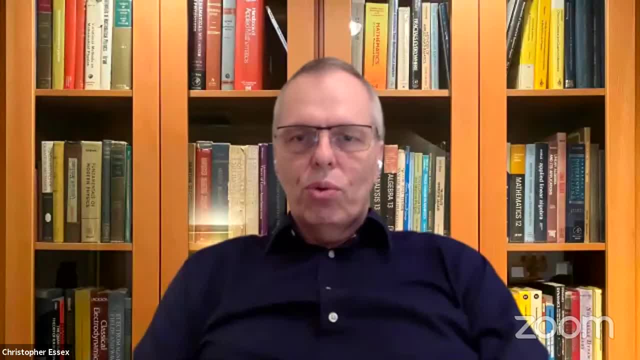 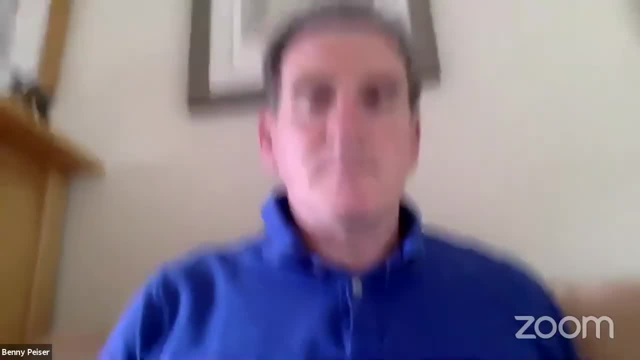 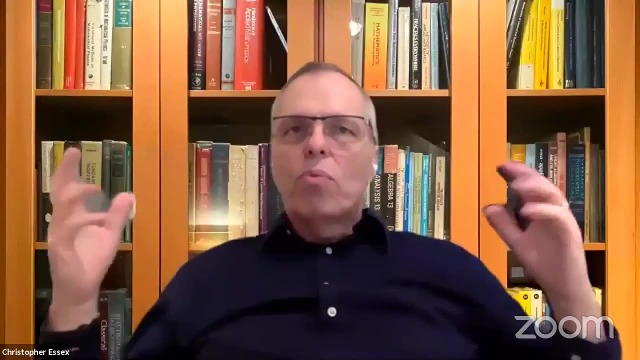 is this idea of how little we actually control things. The assumption that's built into the whole climate GARY MILLER climate business is that not only do we know completely about what's going on, but we also know how to control it, And I think that the best mental picture you might have of 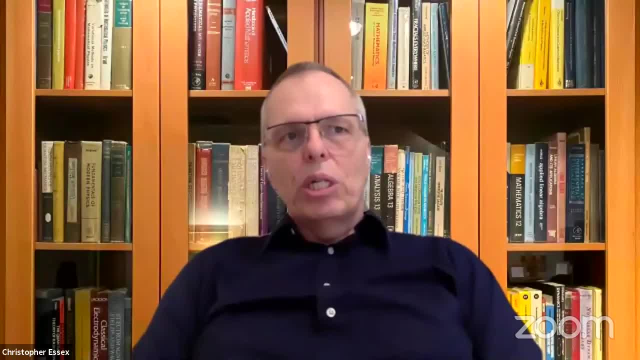 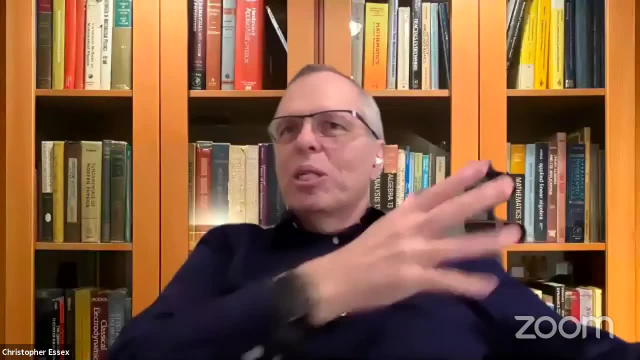 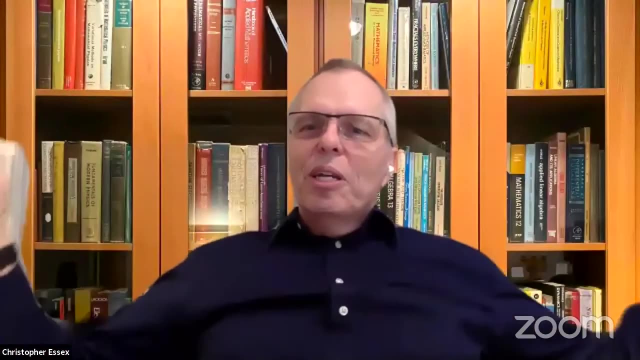 what's really the reality of how much we can control is to imagine that someone is driving a car and then in the passenger seat there's the government, And the government has control over the car radio and they can turn the music and change the stations and then claim that they're. 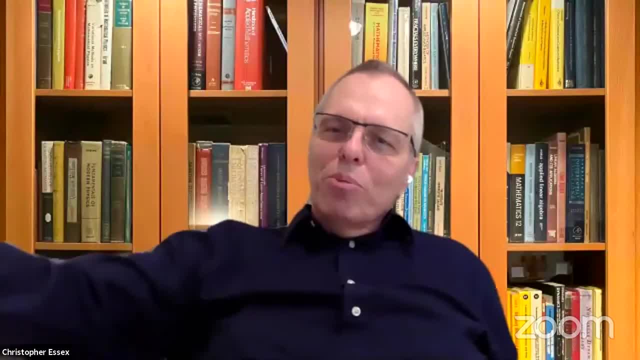 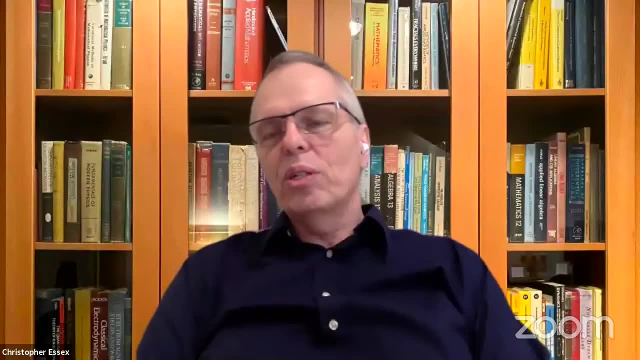 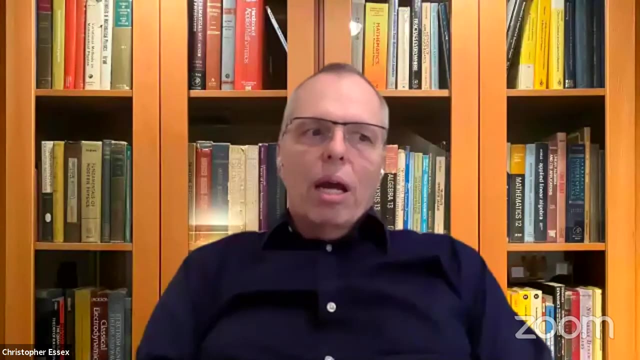 controlling where the car, GARY MILLER, is going and so forth, by turning the volume up or turning it to a country and western station and so forth, But they have no control over the actual car. I mean, that's an important thing to understand. If there is such a thing as a climate control problem. I think we haven't. 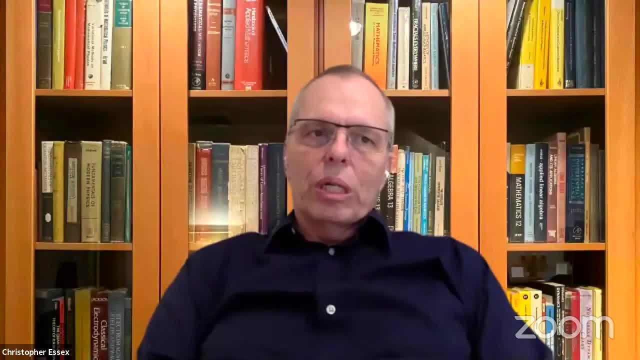 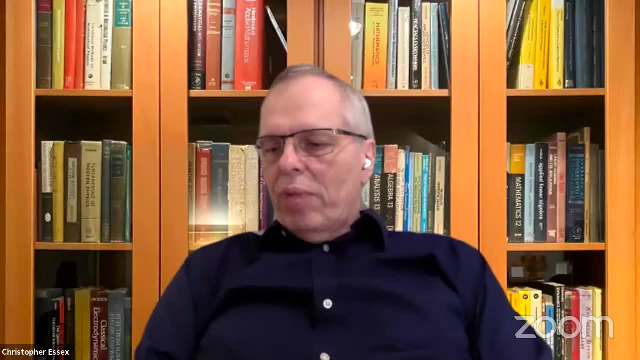 really understood where it is. It's definitely not about global temperature. It's a much more complex problem than that. So you know, if I sort of could leave anything With people about this and I would say is that in many respects, I think that the current 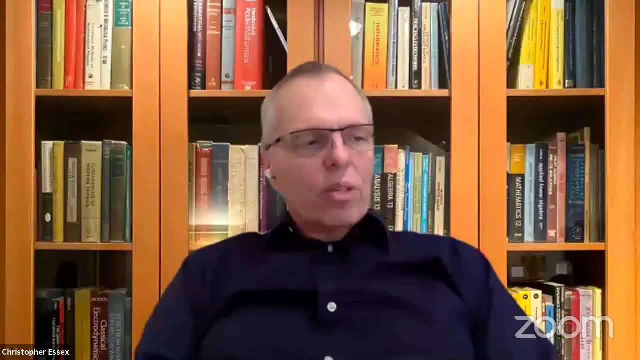 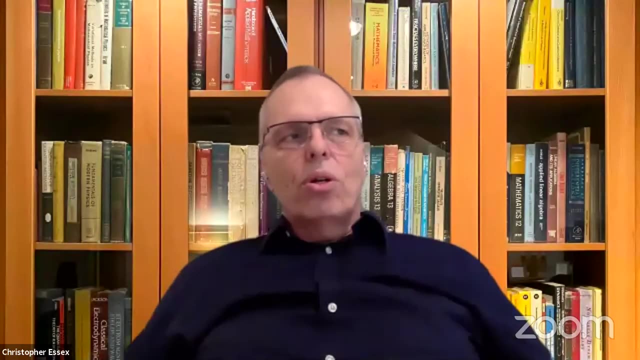 pandemic is leaving a silver lining. if there is one in which people don't feel so much like the apocalypse that's coming is of our own making. I know people are trying to make it that way, but it's still something that is external. It's the virus. It's not because people have been abusing. 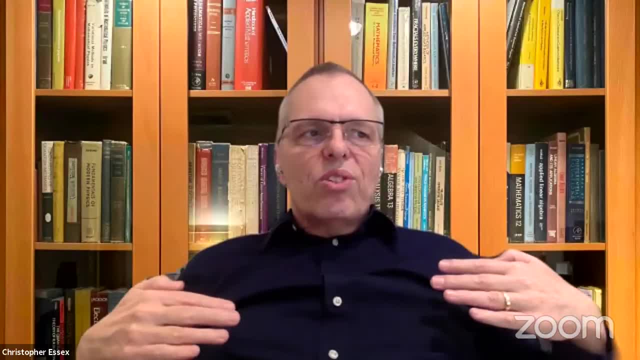 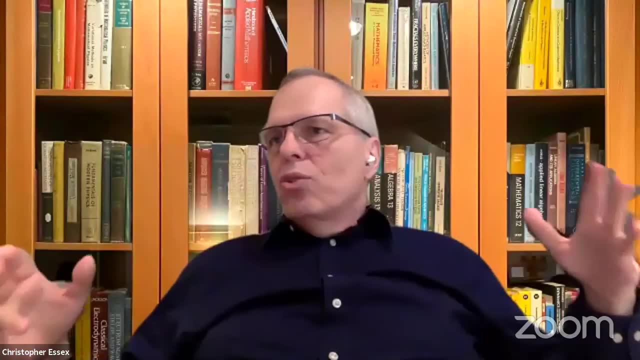 the nature and so forth. So If it could somehow help us get over the idea that we're some kind of demigods that can control the world And so when things go wrong it's our fault. If we can get over that, maybe. 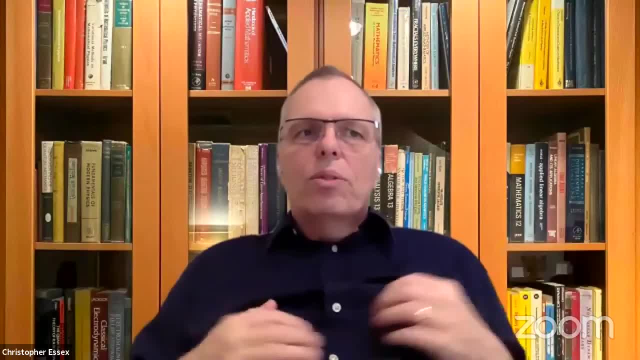 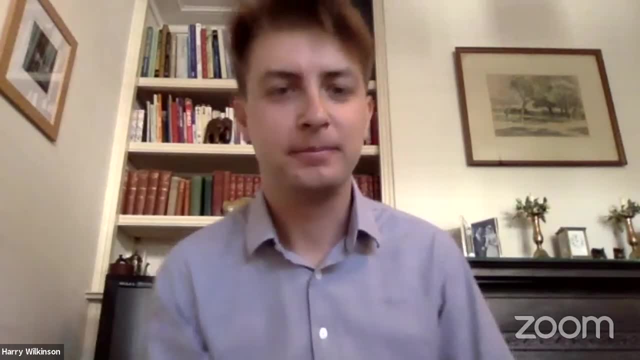 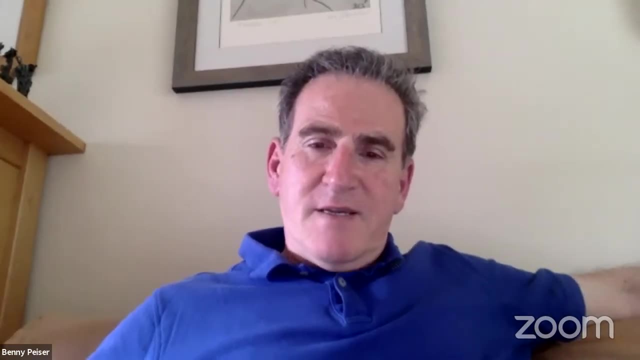 the pandemic will maybe help us a little bit with that, And so maybe that's the silver lining. Thank you, And finally to Benny: Thanks, Harry, for another very interesting webinar. You're really Growing in that role. many webinars hopefully in the next few months. 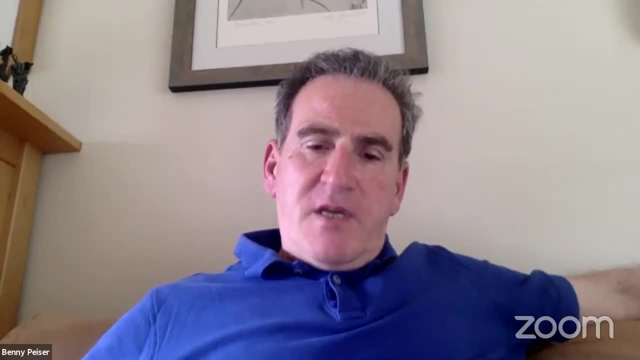 And I think, looking at the history of science, there have always been, throughout the history of science, small groups of dissenters, whether it was scientific or cultural, political, religious. Remember there were times when you were, you had the wrong religion, you couldn't even go to. 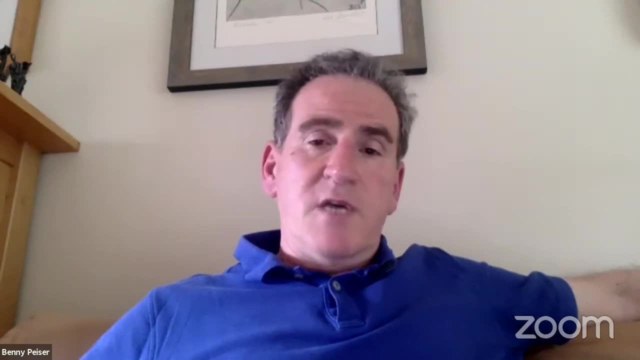 university or teach at Oxford or Cambridge. that was still, I think, in the 19th century, so we always had this conflict. this is not new, this is just perhaps with a bigger impact. I personally think that two things, hopefully, will change. one is that governments might, in response to this fiasco, reconsider how best to receive scientific advice. that's one thing. 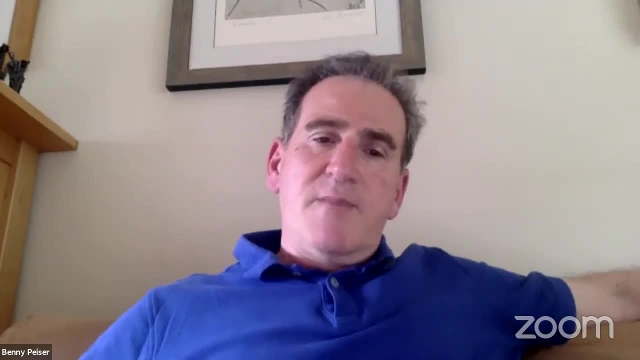 that won't change dramatically- I'm pretty sure it won't- but much more importantly, I think there is now a growing need for independent scientists, for scientists who are allowed to work independently, without the peer pressure of university administrators or scientific organizations. and I think, with the openness of the internet, with the ability of the, 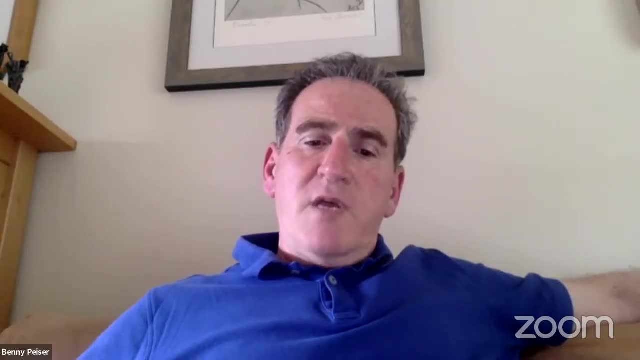 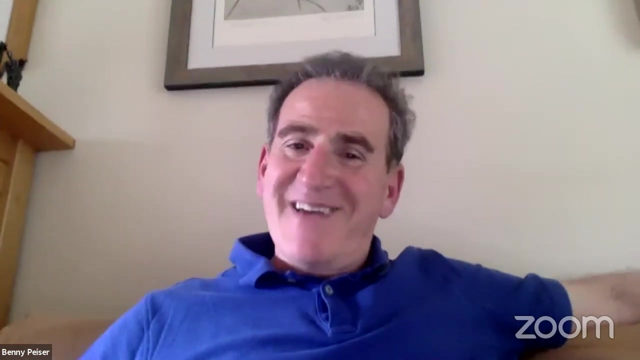 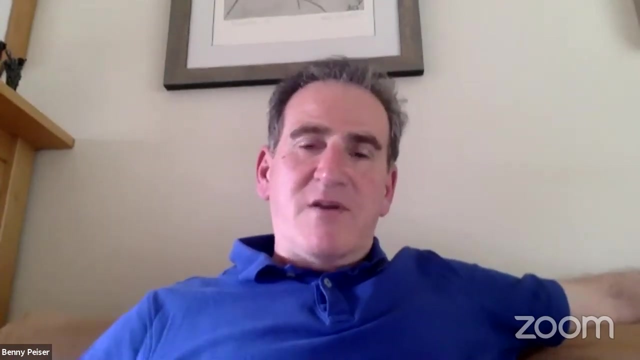 private sector, there will be growing demand for scientists to have forum, a forum where they can express ideas freely, because without free exchange of ideas there won't be any progress in science. that's how science progresses. otherwise we would be stuck to the, you know, to the consensus. 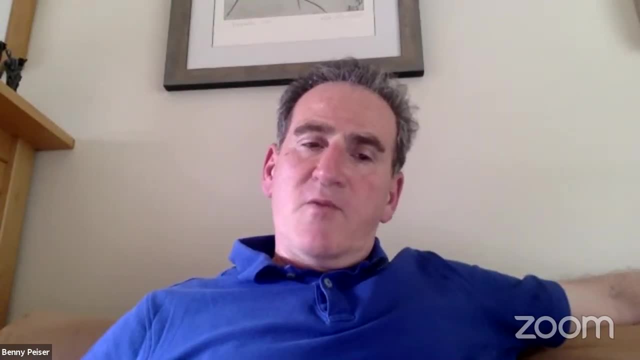 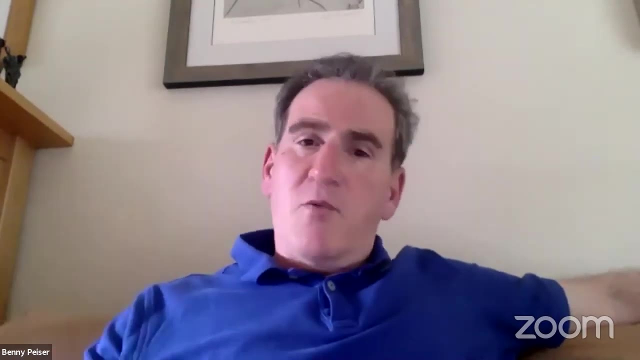 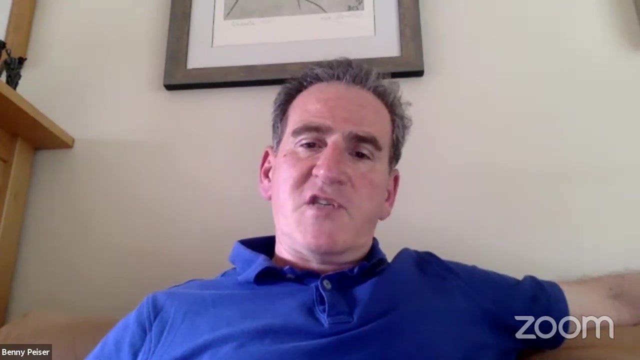 idea. so I, from all of what I've heard today and what I've seen, there is a deep crisis in institutional or what, what Chris says- official science, a deep crisis, and there are a growing number of scientists who are fed up with a kind of politicization of the science.